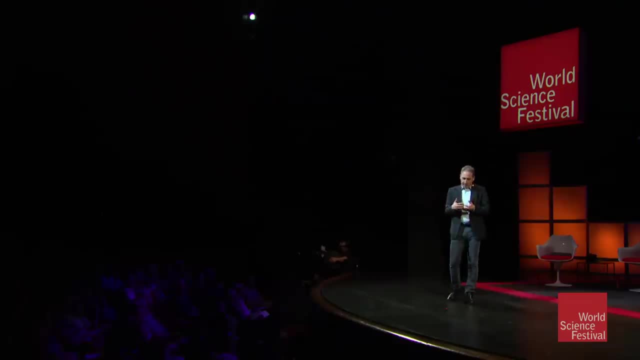 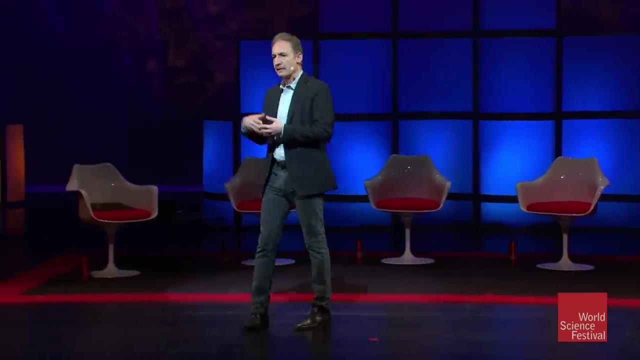 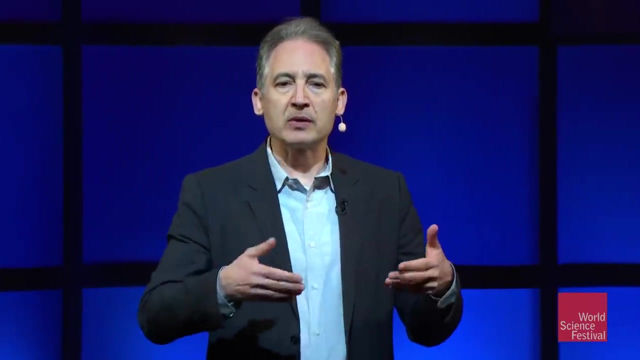 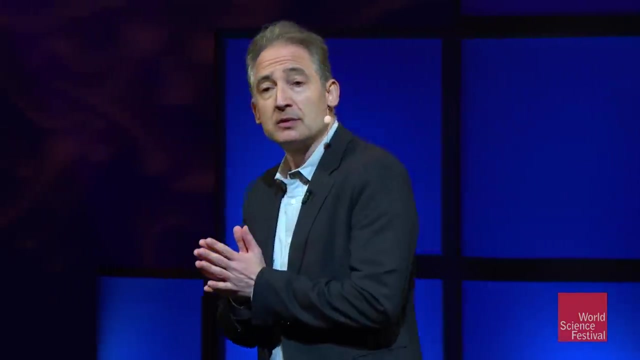 the nature of reality. But, importantly, that insight needs to come with predictions. And those predictions then can inspire other physicists, either astronomers or experimentalists, to go out and try to confirm the prediction and see whether the mathematics is actually describing true aspects of reality. Now for Einstein, it was a wonderful confluence of the mathematics. 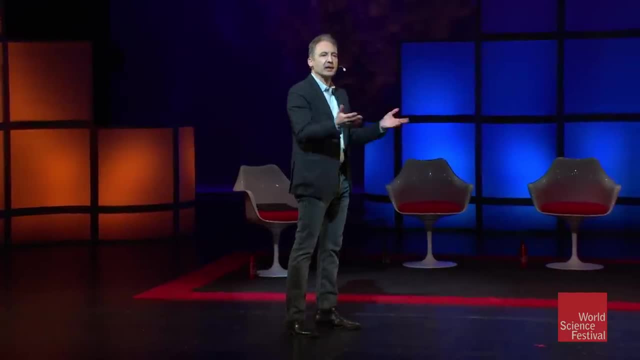 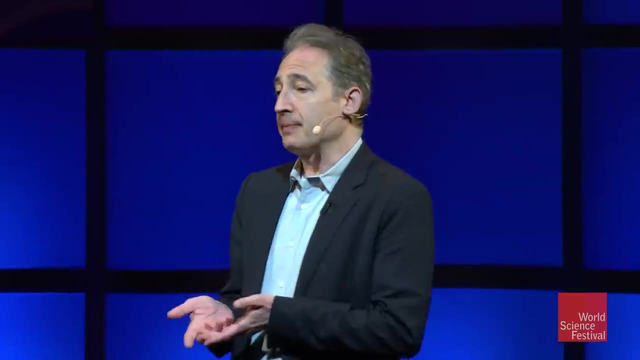 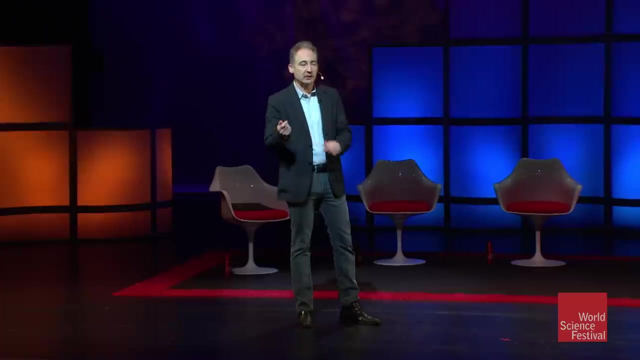 and the technology necessary to check the mathematics, because he wrote down his equation of the general theory of relativity in November of 1915, and the observations that confirmed his ideas happened in 1919. So just four years between the theory and the observation. Oftentimes, 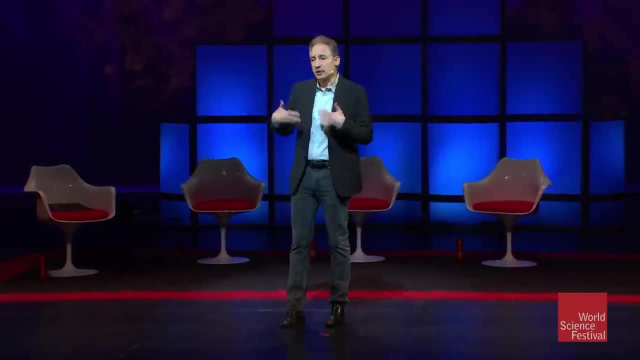 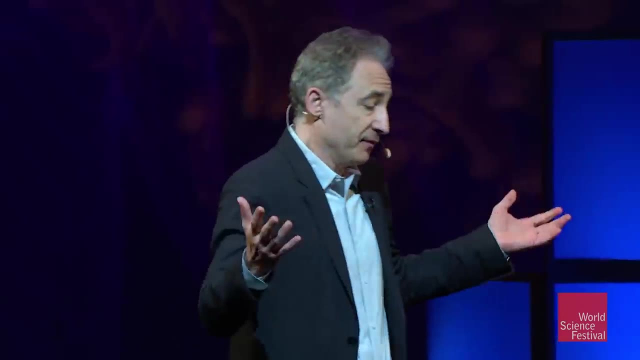 in physics the timescales are longer. The theoreticians will come up with the ideas. perhaps they're difficult to test. perhaps it will take building new equipment. perhaps it will take, in fact, countries to come together, to put their resources together, to combine. 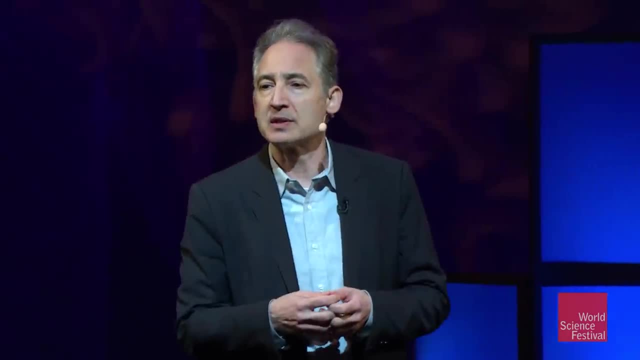 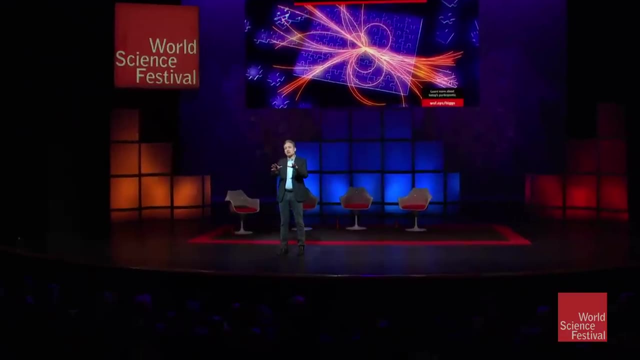 their resources in order to even be able to build the machines necessary to test these ideas, And that is going to be part of what will drive our conversation here today. But whereas Einstein's ideas and his confirmation was all about sort of looking up into the 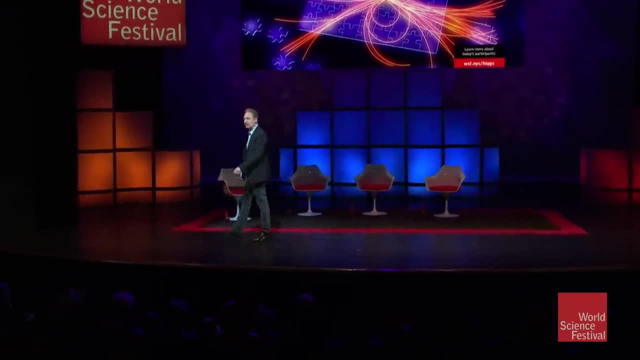 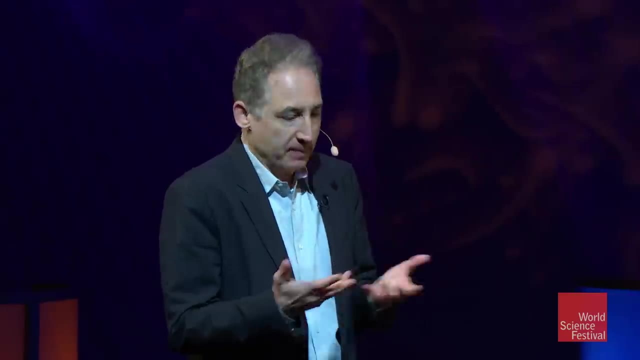 sky, thinking about gravity, thinking about big things. the focus here will be on the other end of the spectrum, For the most part thinking about gravity, For the most part thinking about gravity, about small things, particles, because we have, for you can really trace the. 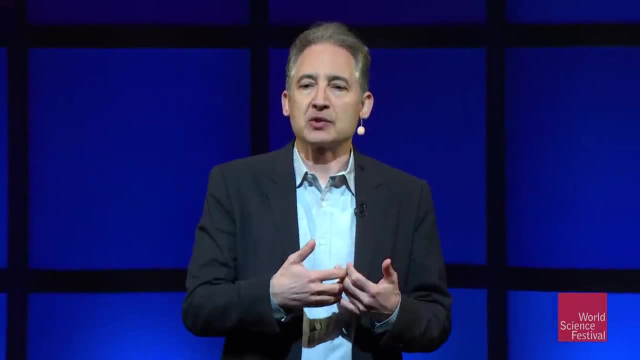 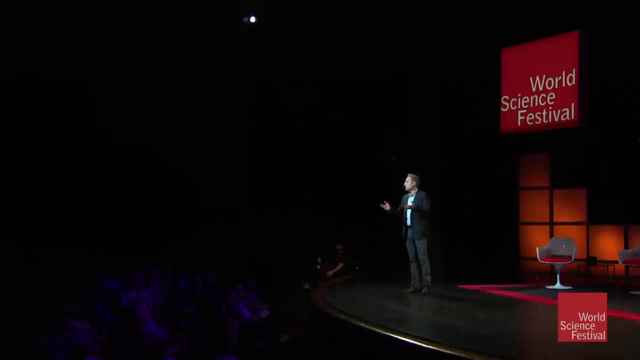 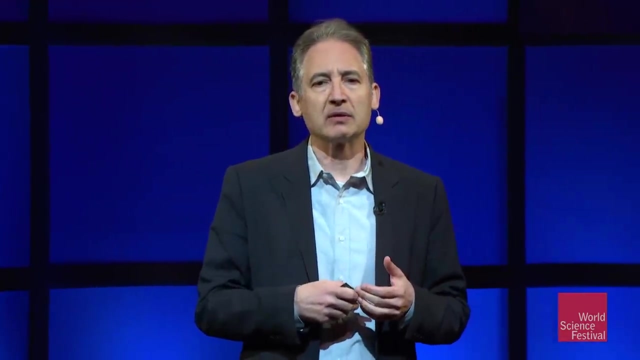 history back thousands of years, asked ourselves the question: what is stuff made of, what are the fundamental ingredients? and we've thought about this over the course really, of many, many centuries. but that program of trying to figure out the basic ingredients of matter really picked up in the middle of 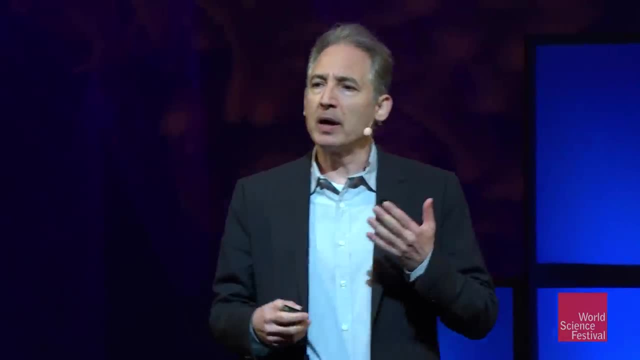 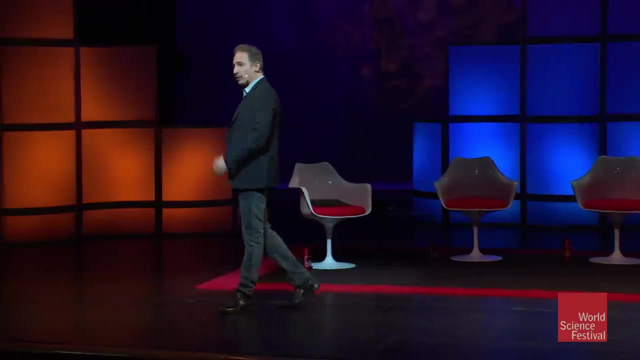 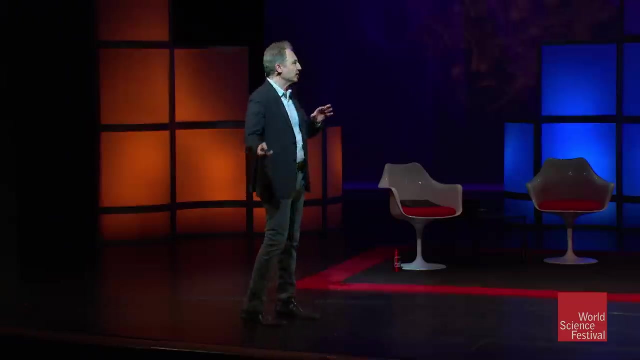 the 20th century, and it was a wonderful time where the theorists and the experimentalists really worked hand in glove, back and forth, playing off of each other, and Steven Weinberg, one of the great scientists of our era, summarized the excitement in a really wonderful ways. it was a time when graduate 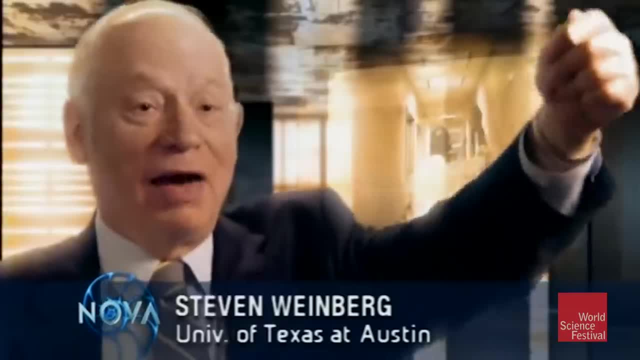 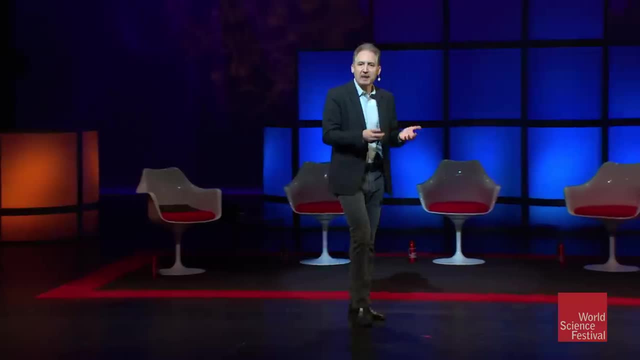 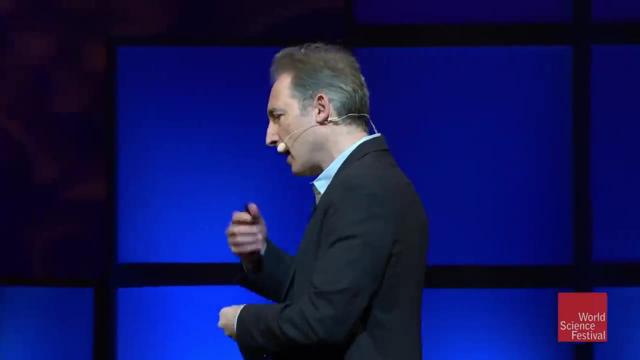 students would run through the halls of a physics building say they discovered another particle and it fit the theories. and it was also exciting back and forth between the mathematical, mathematical ideas that inspired the experimentalists to look for certain kinds of particles. They'd find the particles come back. The theorists would then update their equations with the 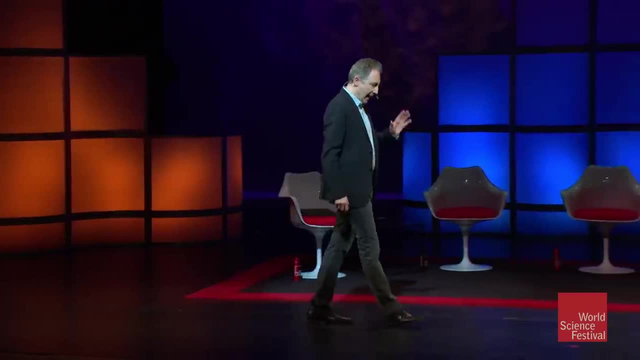 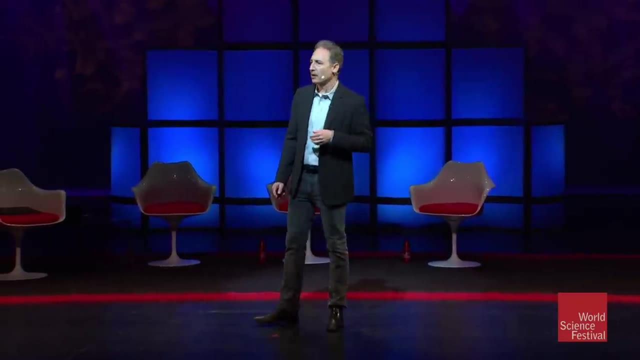 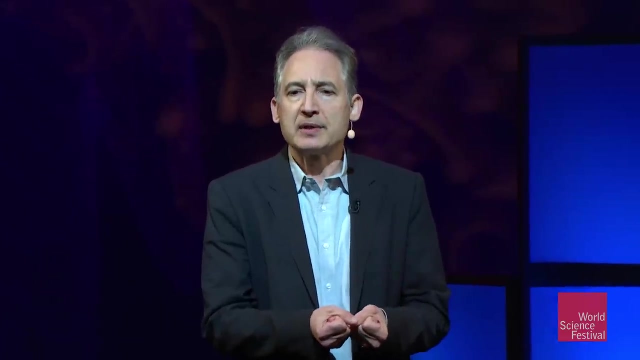 new insights, and back and forth it went, And as this unfolding occurred, there was one sticking point which is really going to be part of the focus of our conversation here today, which is there was a very basic question: Why is it that these particles that 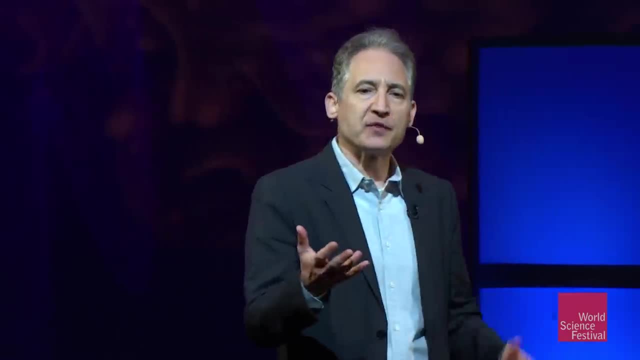 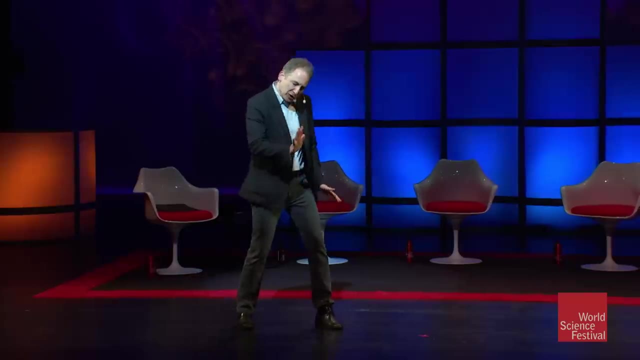 were being found, have heft, have mass. In essence, if you had one of these particles, fundamental particle, in front of you, it could be an electron, it could be a quark, whatever. As you push on it, where does its resistance to your push come from? Where does 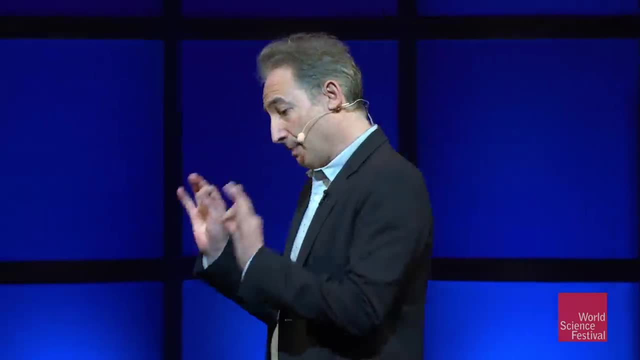 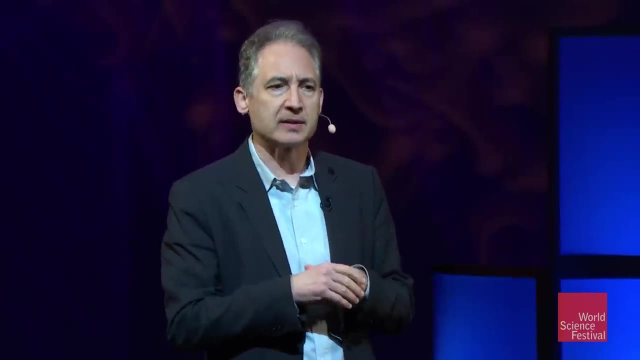 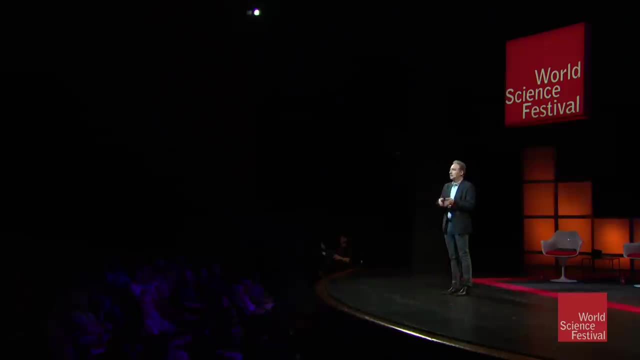 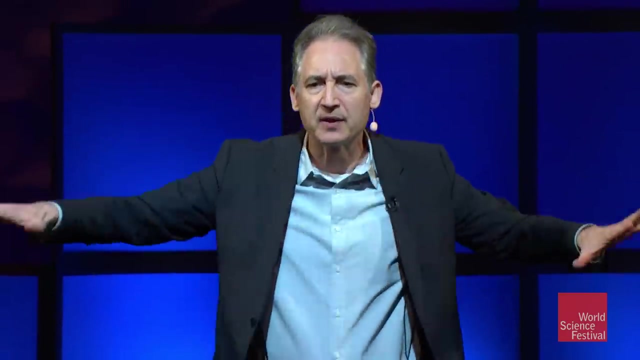 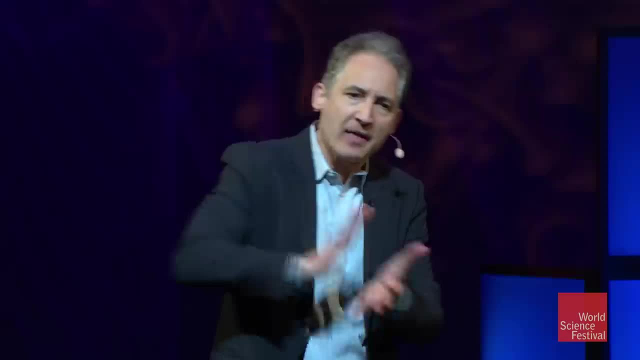 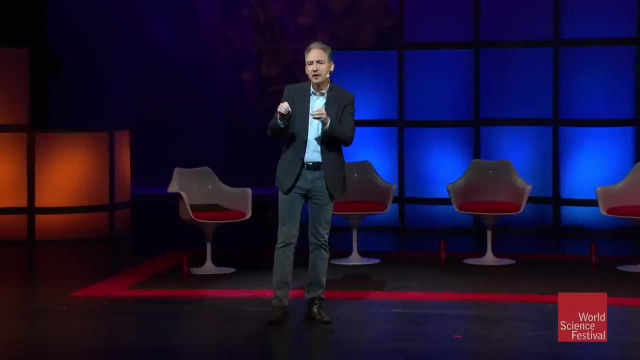 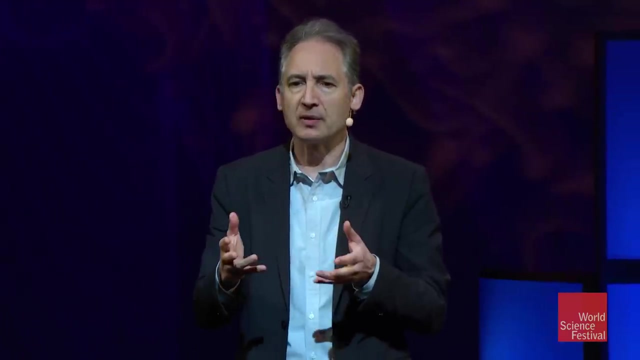 it came with the prediction that if you kind of banged on this molasses sufficiently in the right way, you could sort of have a little fleck that would come off, And that little piece of the molasses would be a particle called the Higgs particle or the Higgs boson. And on July 4th of 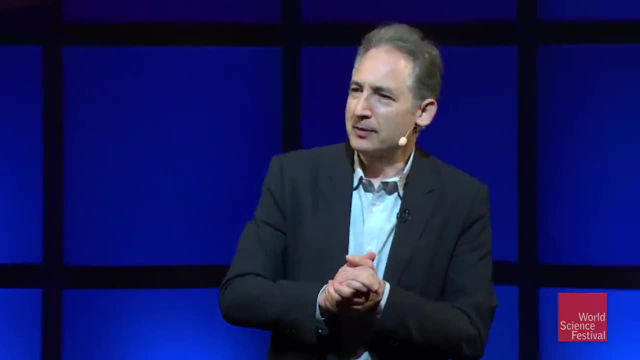 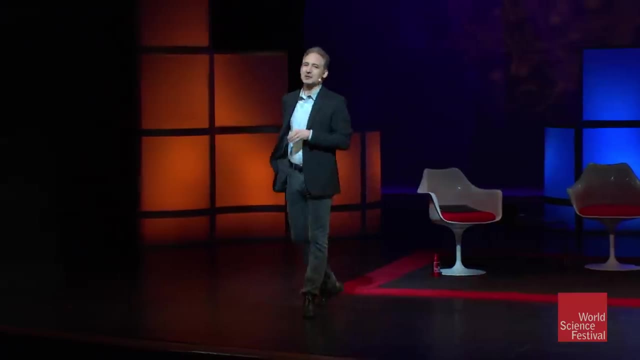 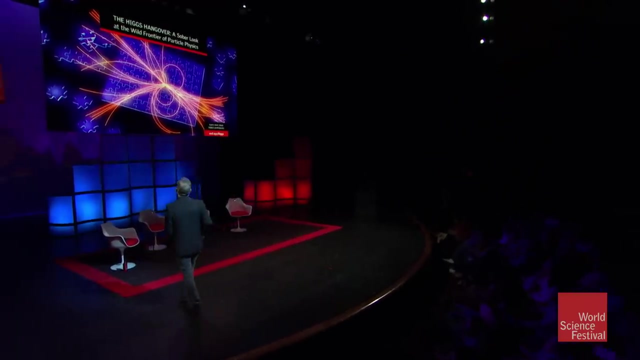 2012,. if you weren't out celebrating and doing whatever we Americans do on Independence Day, if you're actually paying attention to something some of us consider to be much more important, you might have seen the following press conference: If we combine the ZZ and gamma-gamma, 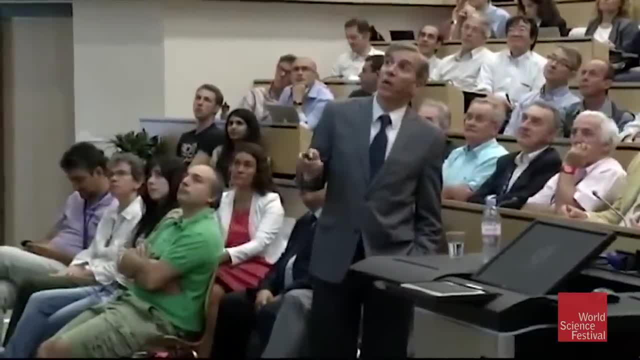 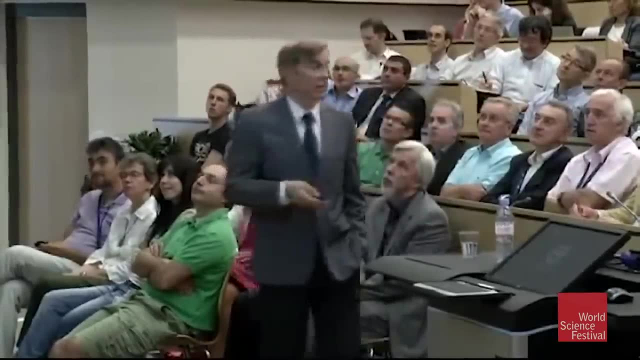 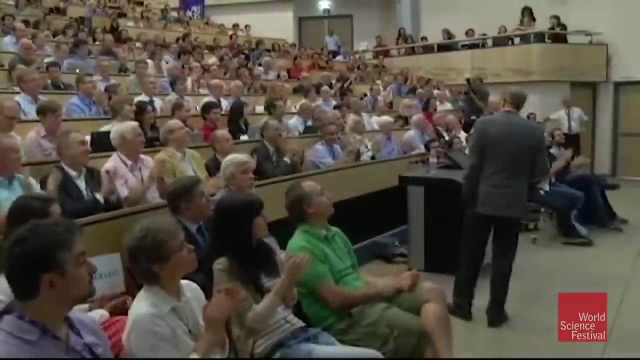 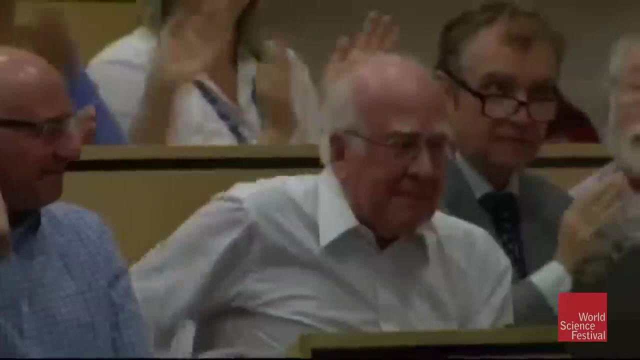 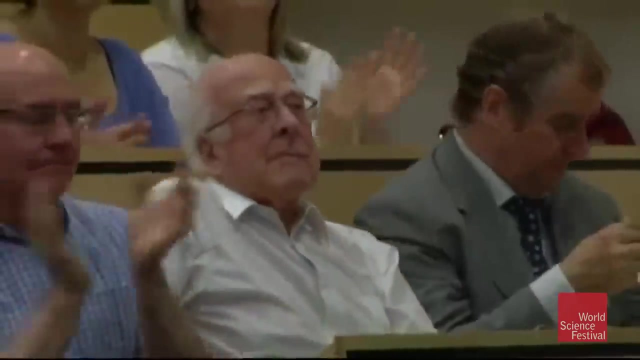 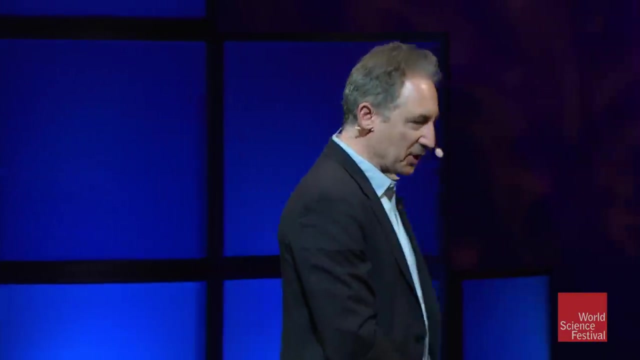 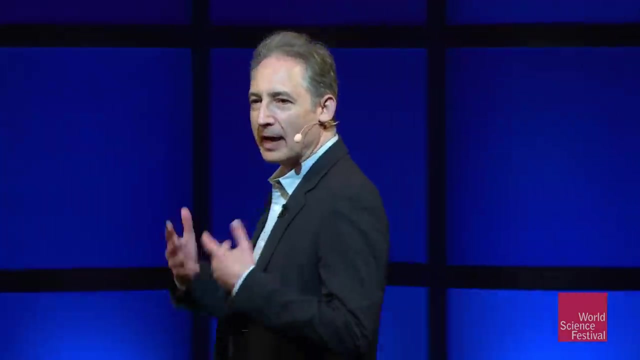 you might have seen the following press conference: This is what we get. They line up extremely well And in the region of 125 GV they combine to give us a combined significance of five standard deviations. So the emotional gentleman taking off his glasses, wiping his eyes, you might guess that was. 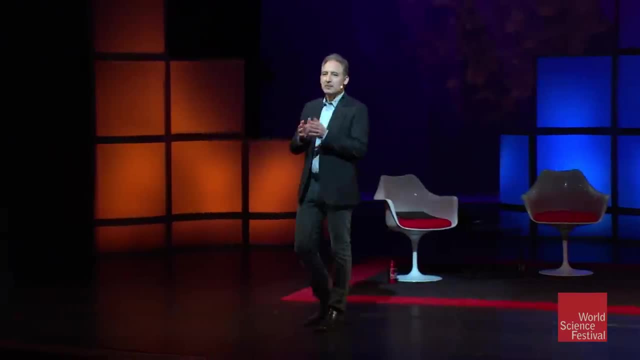 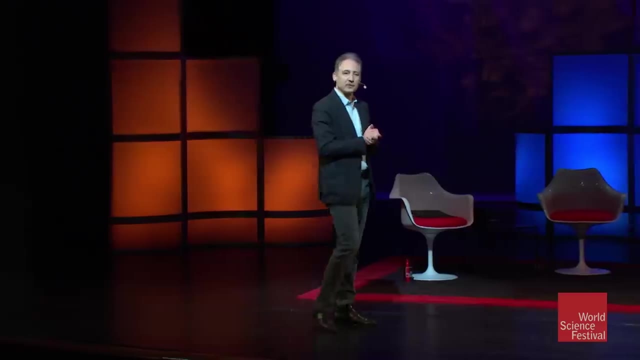 of course, Peter Higgs, the gentleman whose mathematics was put forward in the 1960s and about a half a century later was confirmed through the observation of this Higgs particle. And of course, this excitement. this excitement was the critical factor in Cecilia Higgs's humble mere. 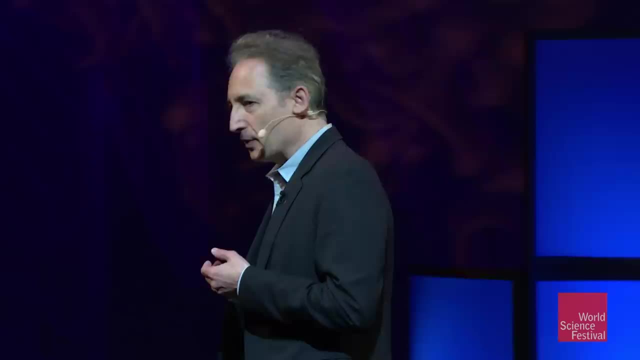 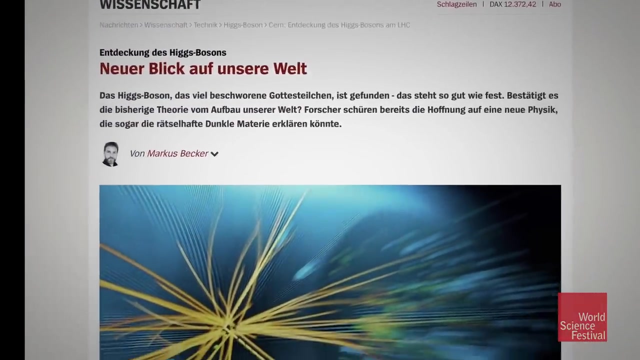 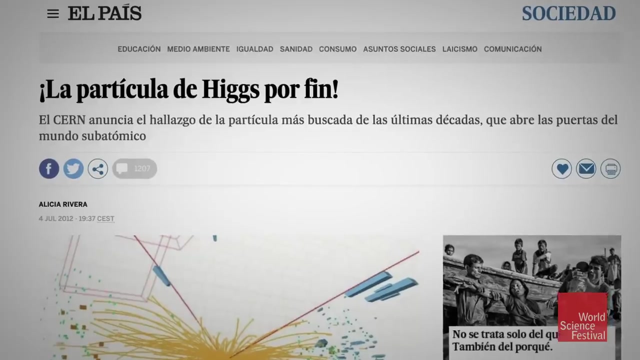 it was picked up by newspapers, television shows around the world, because this is again one of those iconic moments in the history of deep understanding. But, at the same time, the discovery of exactly what we expected to find based upon the mathematics, raised a certain kind of challenge. 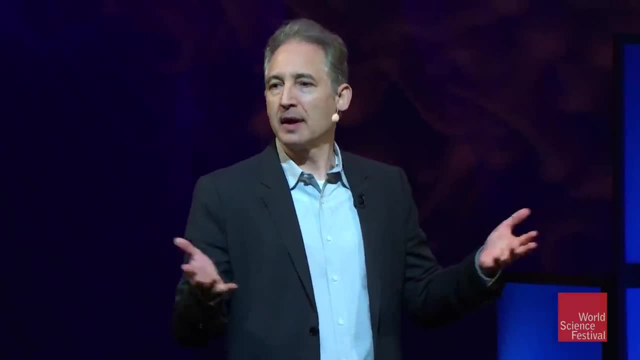 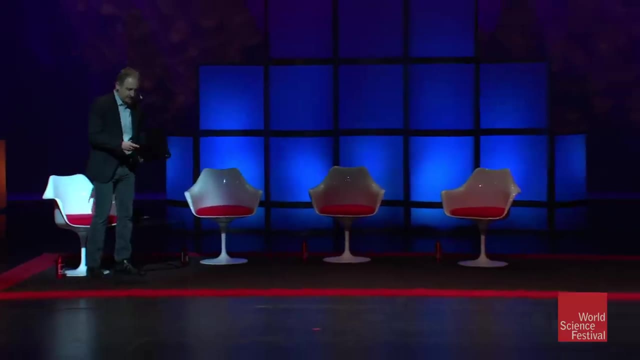 which is what's next And that's what we are going to have a discussion about here today, And we have some of the world's leading thinkers on these ideas of particle physics, so let me now bring them out to you. Our first participant this afternoon. 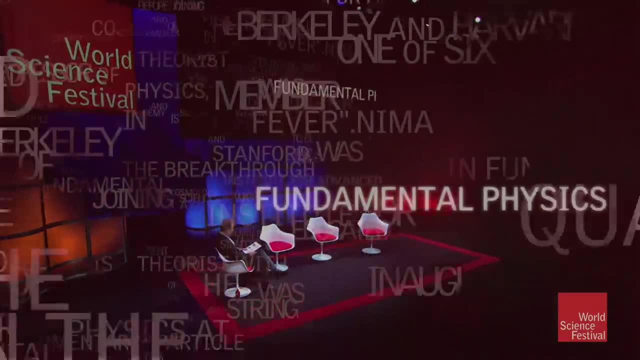 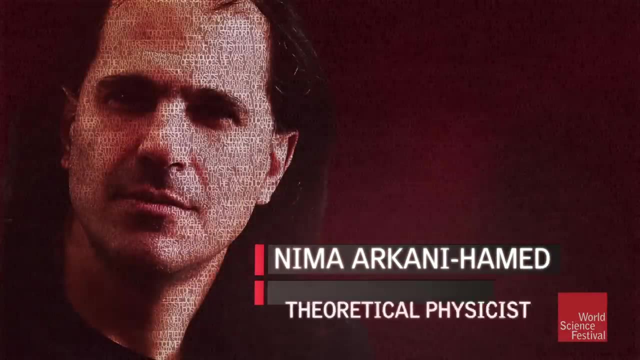 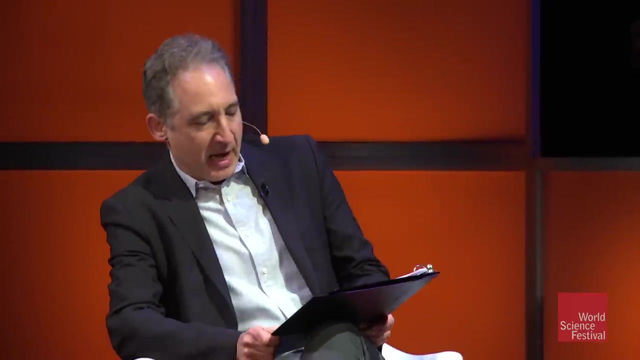 is a theorist at the Institute for Advanced Study. a member of the National Academy of Sciences, He was an inaugural recipient of the Breakthrough Prize in Fundamental Physics. Please welcome Nima Akrani-Hamed. Also joining us is an expert and experimental high-energy particle physicist. 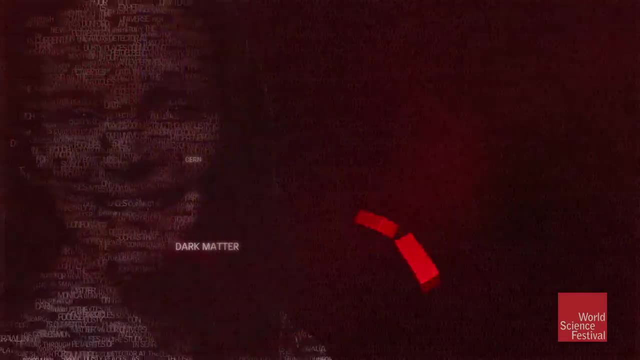 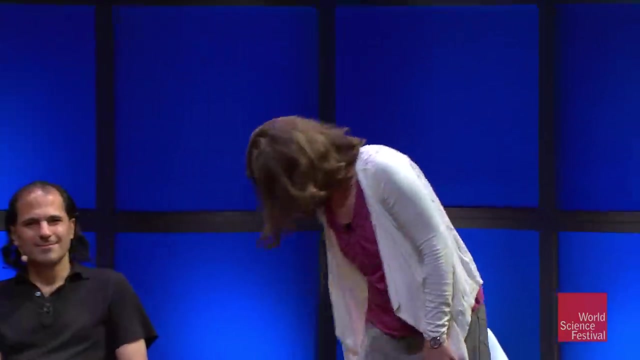 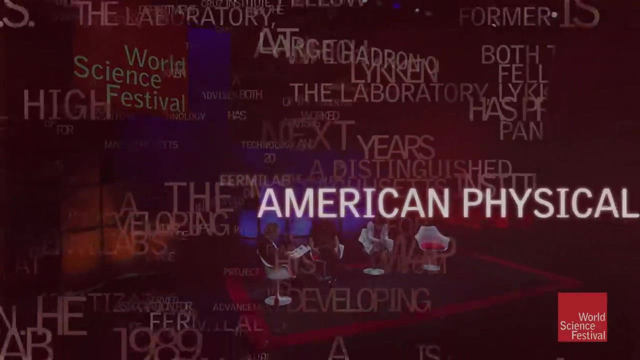 working on the ATLAS detector at the Large Hadron Collider at CERN. Please welcome Monica Dunford. All right. finally, please join me in welcoming the Deputy Director of Research at the Fermi National Accelerator Laboratory. He is a fellow of the American Physical Society. 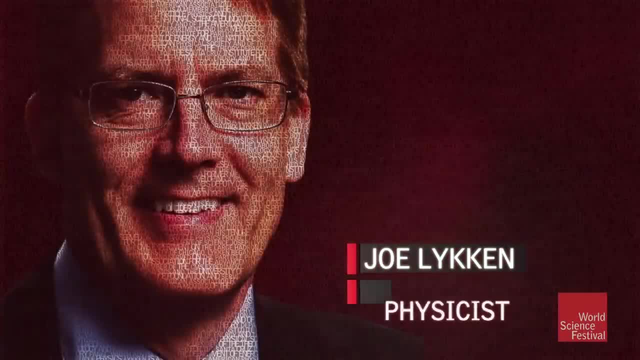 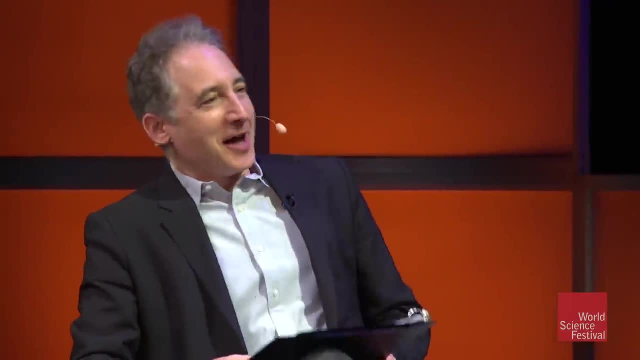 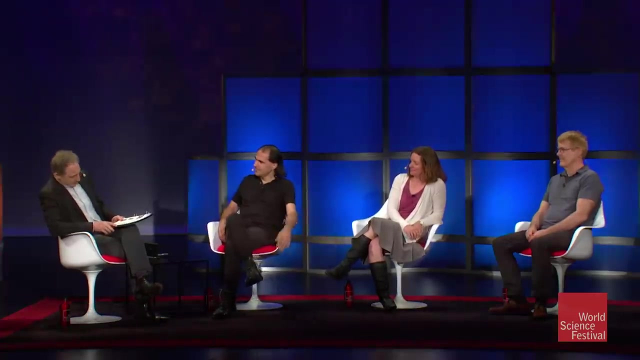 and the American Association for the Advancement of Science. Please welcome Joe Licken. I've known all you guys for many years, probably known Joe the longest of all. I think we probably go back 30 years. But whoever wrote my little notes here? 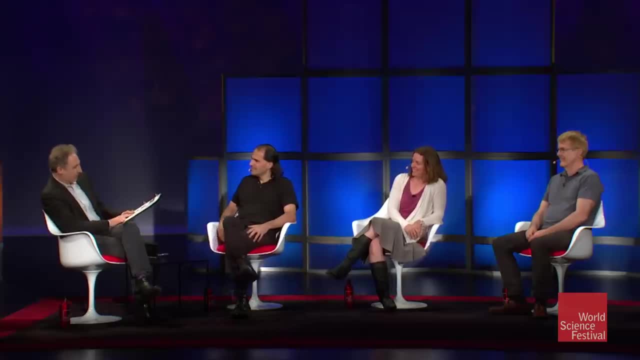 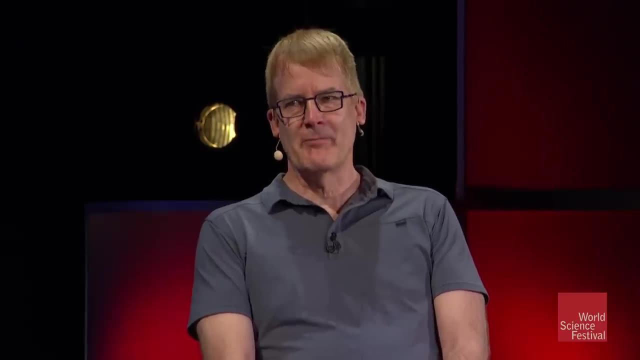 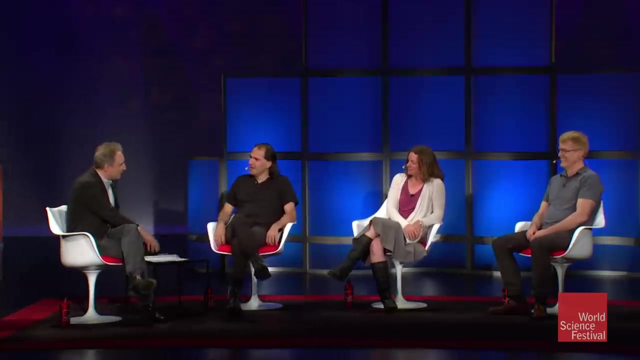 probably didn't know that fact, because they have told me that your name is pronounced Licken, just like finger lickin' good, So I think I would have gotten it anyway, but I appreciate that as well. So let's begin the discussion by just going way back. 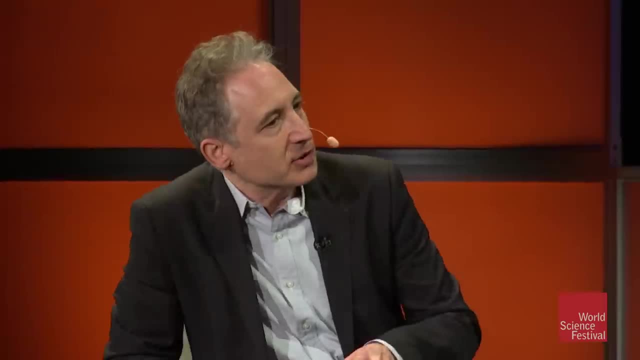 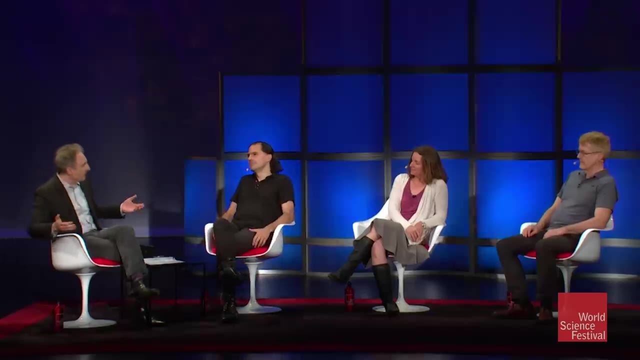 for a moment, way back to, you know, ancient Greece, when there were thinkers who began to ask the question. you know what is matter made of, What is the stuff around the world made of? And so we have this fellow right here. 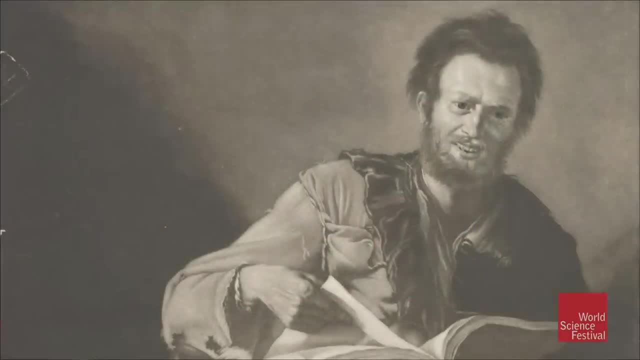 So, Nima, who is this and what role did he play in your mind? This is Mr Democritus. Apparently, I don't know how we know he looked like that, but anyway, But now Democritus is widely credited as being the person. 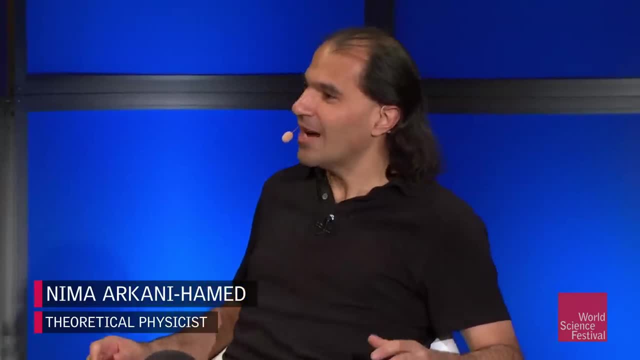 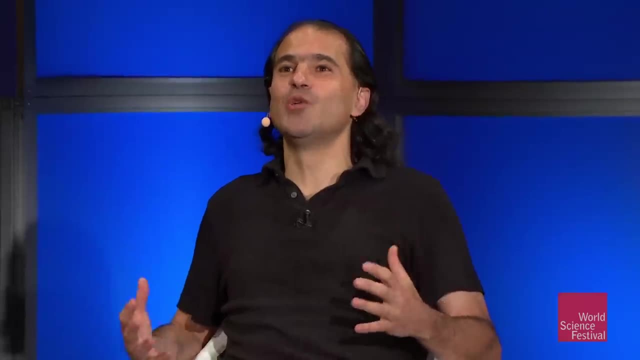 who suggested that the world is actually made up out of atoms, that matter is made out of some fundamentally smallest building blocks, And just tell us your view of that perspective. I think he's the single most over-credited individual in human history, Because there's absolutely no evidence. 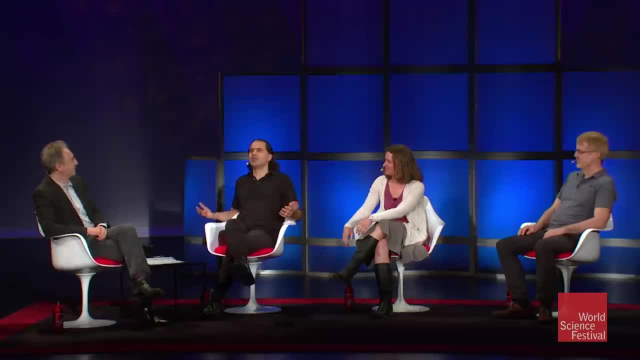 one way or the other, whether this idea was right. You know you're just sitting around in ancient Greece. hey, you think matter. you know you keep cutting it up. it goes all the way down forever. I don't know. 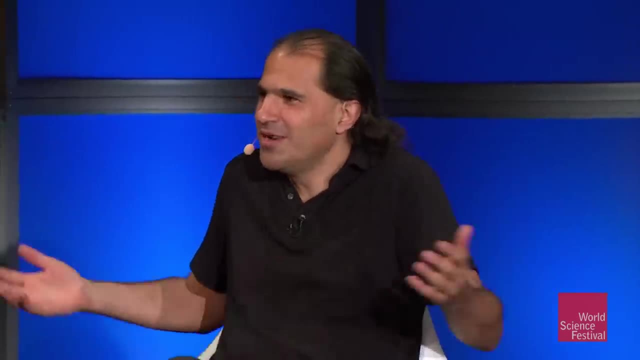 Yeah, I do. No, I don't. You know. there's absolutely no reason to believe either one. either way, The guy who said that it stops somewhere he's famous for 2,500 years. It's not fair. It's not fair. 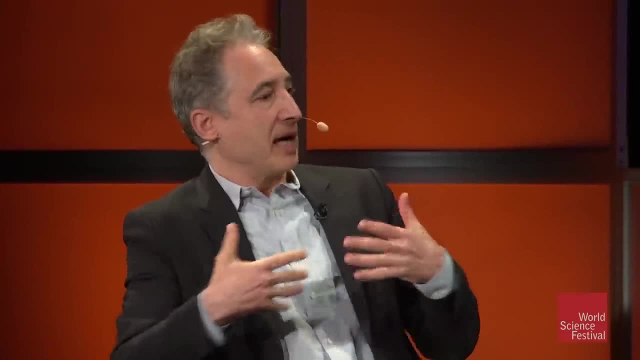 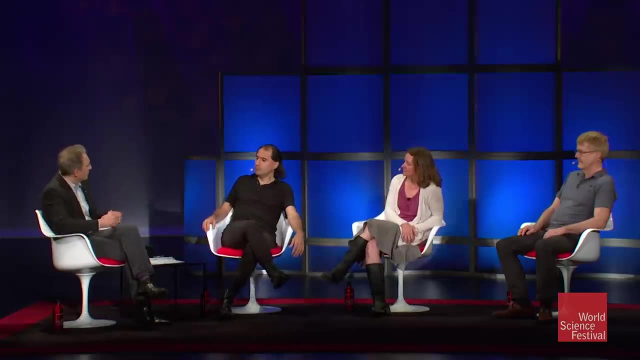 Let me ask you one thing, though. So we certainly tell our students- and I think it's a real truism- that asking the question is oftentimes as important as finding the answer, So perhaps, maybe it's worth crediting him with at least thinking about the possibility. 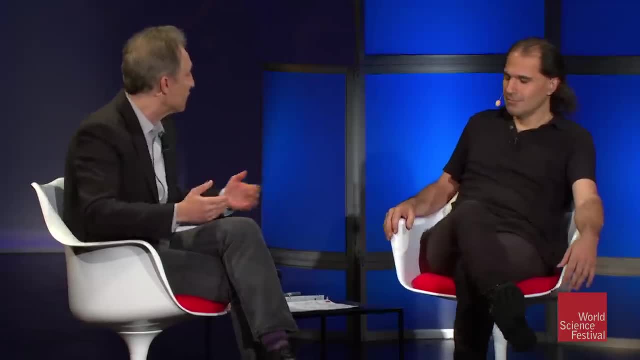 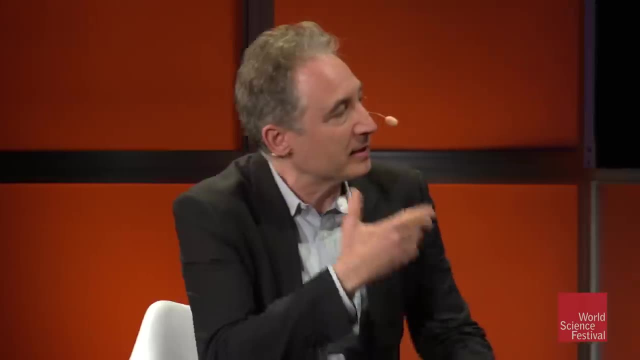 that this is a worthwhile question to investigate. I would agree with that. I would agree with that if what you said is true, but I'm not a historian of science, I don't know. actually Good, good, good. So the idea that he had, of course, 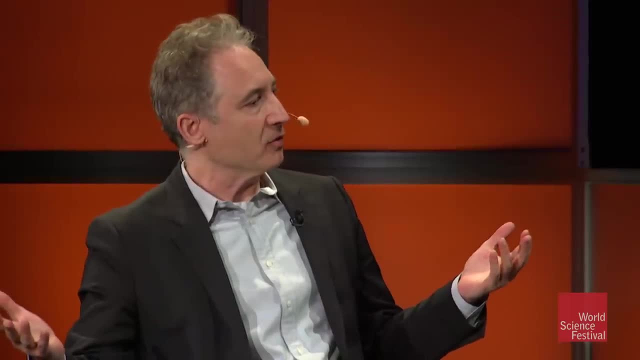 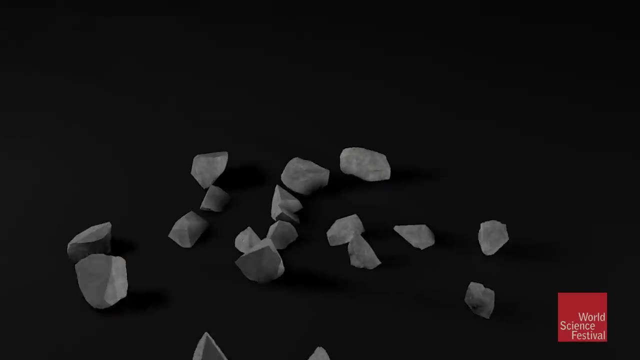 was presumably. you take a piece of matter and you start to sort of pound on it or cut it up in some. You know, we have an example here: It's a rock. And so what have we found in the past? you know, 2,000 years. 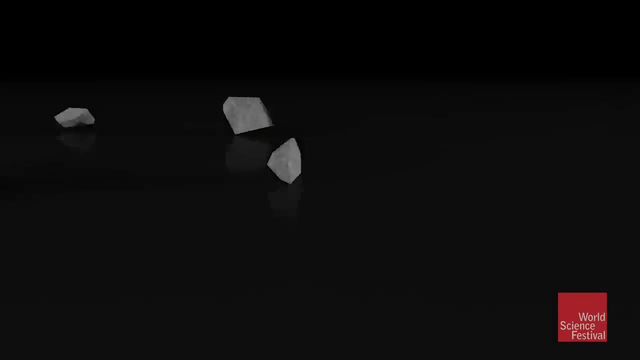 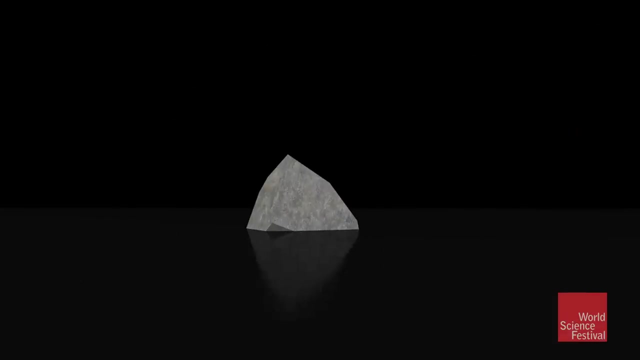 if we at least start the journey with Democritus. Yeah, so I think a little over 100 years ago, I mean in the mid-1800s, I guess, chemists, or back in the time when there was not such a distinction. 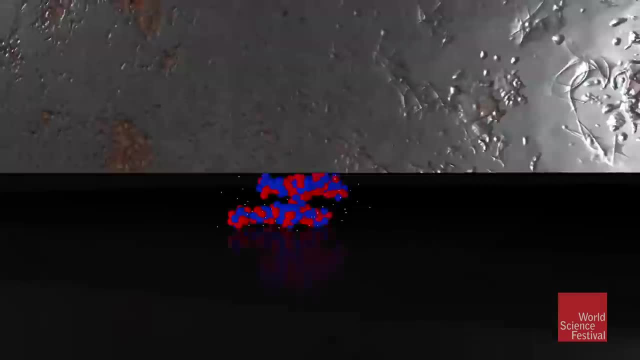 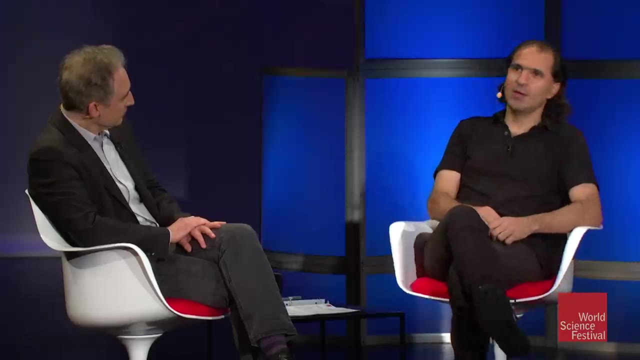 between the two, I mean the different physical sciences, but anyway, people started suspecting that there might be atoms, that ultimately different kinds of material were made out of different sort of building blocks. We have the system of the periodic table of elements. 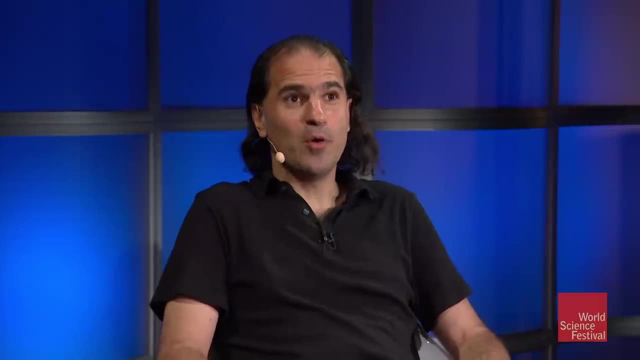 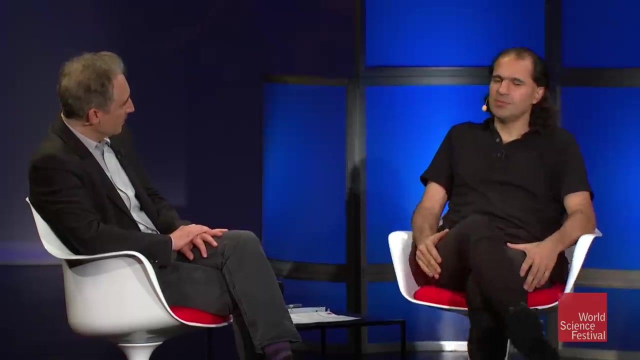 and so on, And already back then there were people who were skeptical that you were talking about these teeny, teeny, tiny things that no one can actually see. but there started to be more and more indirect evidence that atoms actually exist. Of course, today we see them in various ways directly, 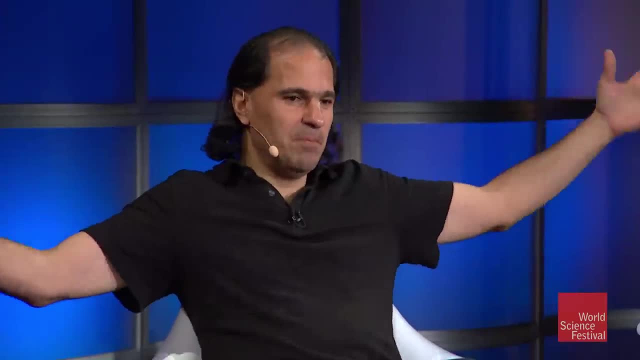 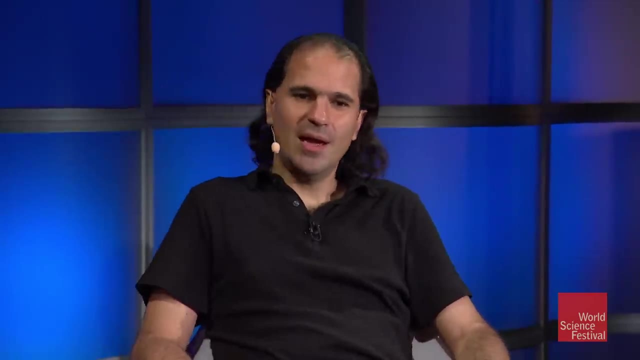 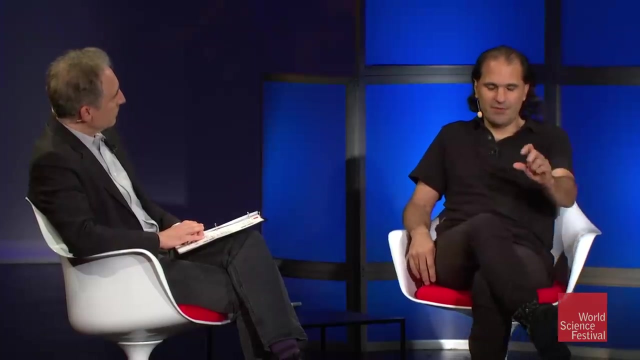 but that's where the sort of journey began that you know, these blocks of matter are made out of molecules or, in turn, collections of atoms. An atom is, maybe you know, a 100 millionth of a centimeter across, So it's very, very small. 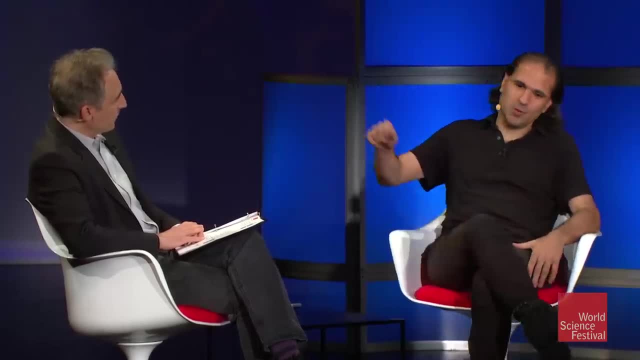 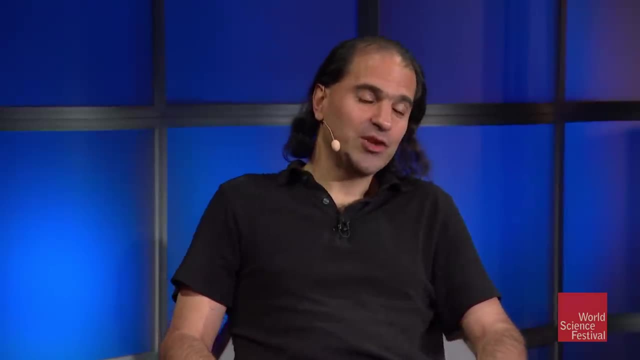 but then the atoms themselves were built out of other constituents. We have the electrons- probably all heard about in school- that were around the nucleus of the atom. The nucleus of the atom in turn is around a million times smaller than the size of the atom itself. 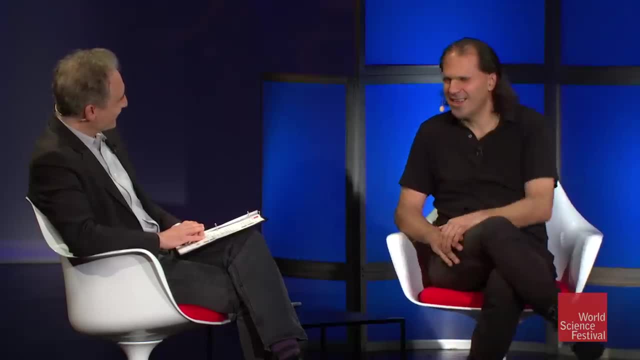 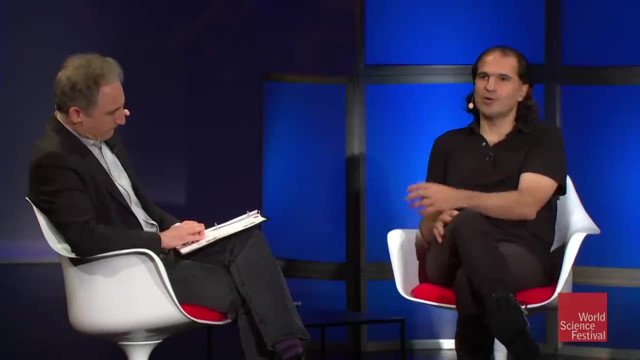 So these kind of pictures are not really to scale right. The nucleus is around a million times smaller than the atom itself. And then we go into the nucleus. we see that the nucleus is made out of particles like protons and neutrons. 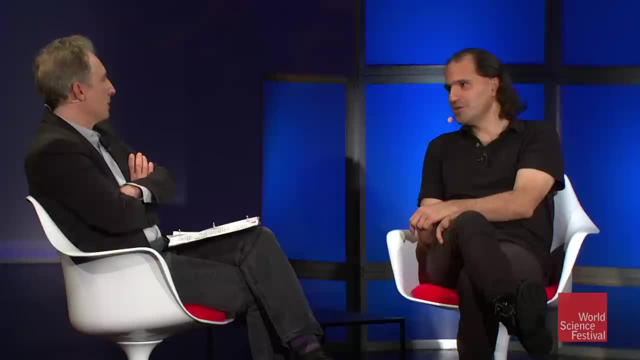 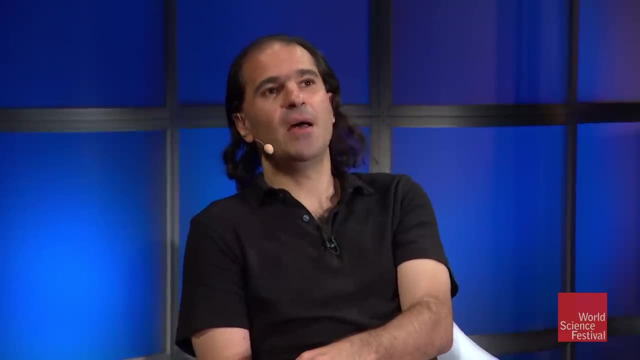 which are now around 10 to the minus 14 centimeters big And around 50, 60 years ago, we started peering inside gradually these apparently elementary objects- protons and neutrons- that turned out not to be elementary at all. 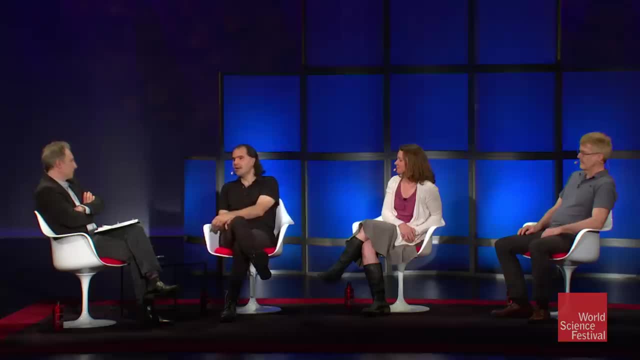 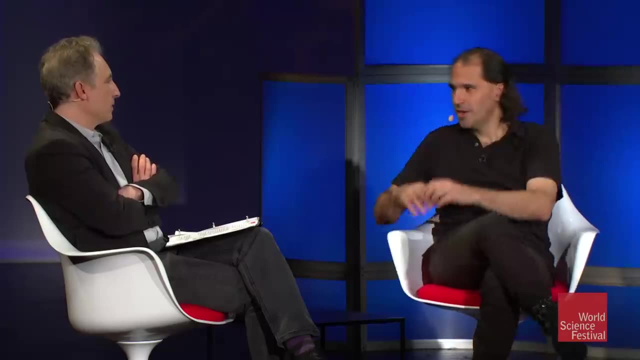 And built out of still more point-like constituents. So that's where the journey has been taking us, at least in this building blocks of matter perspective on what it is that we do, And hopefully we'll come back and talk about some other perspectives on what it is that we actually do. 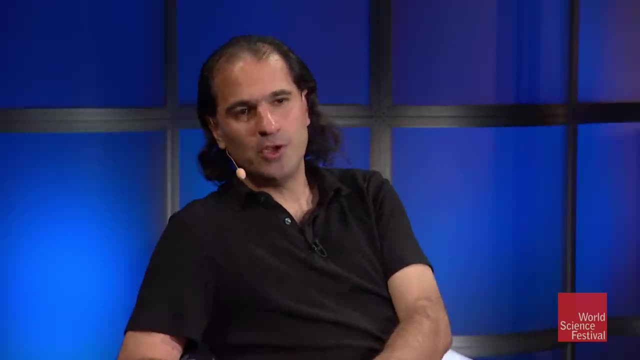 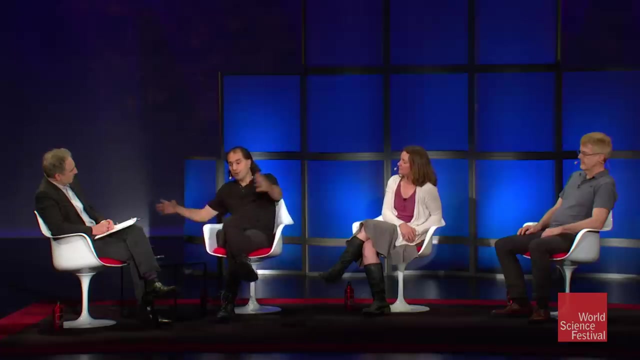 But anyway, in this very fundamental aspect of what we do, that's the journey that we've been on. We're now at a distance around what we're probing at the largest experiments in the world, like the largest accelerators in the world. 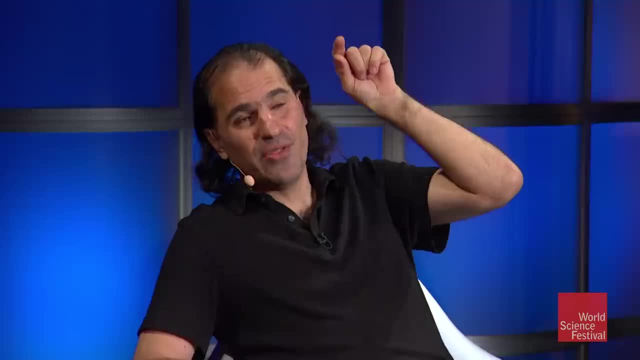 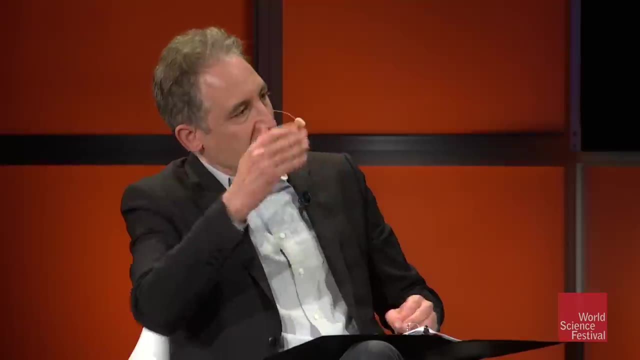 like the Large Hadron Collider, or distances around a thousand times smaller than that, a thousand times smaller than the nucleus of the atom, And there's a lot of drama that has unfolded there and that will be the focus of some of our conversation. 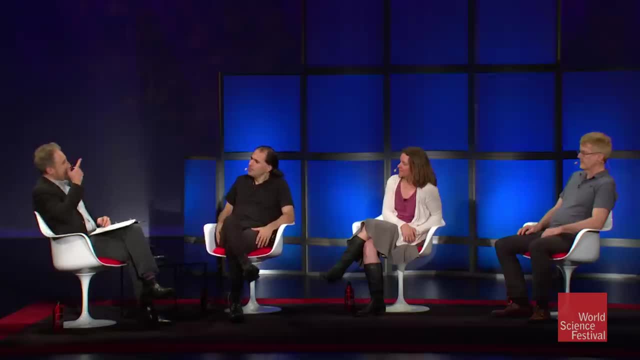 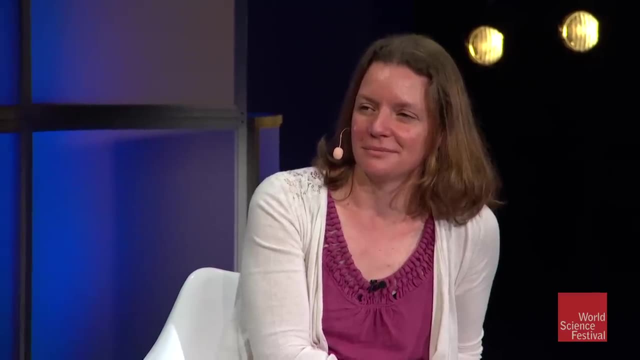 So let's talk a little bit about that. So, Monica, you know, when we show a picture, as we began there, with whatever, a sledgehammer smashing into rock, it suggests the most brutish way of figuring out what's inside of matter. 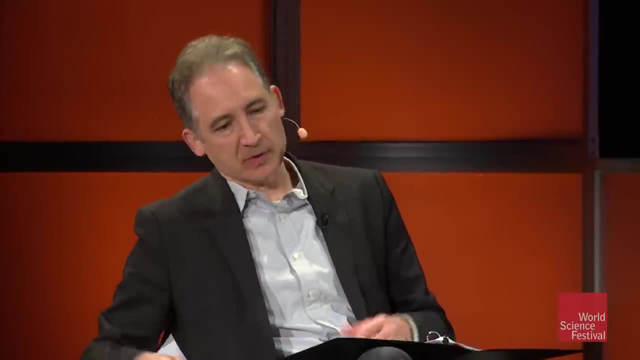 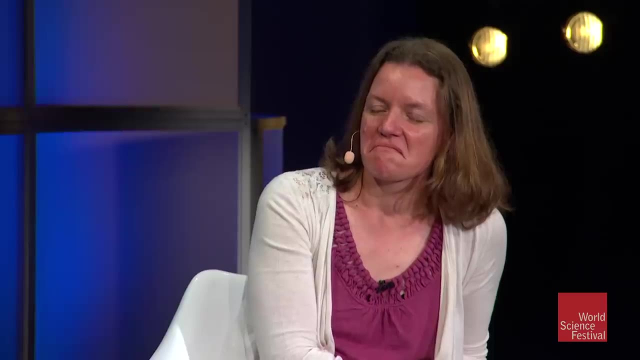 You just sort of smash it apart and see what the constituents think. It's like a five-year-old just smashing things together to see what's in there. Is that what we do At the Large Hadron Collider, Or would a more refined way be to make you say of? 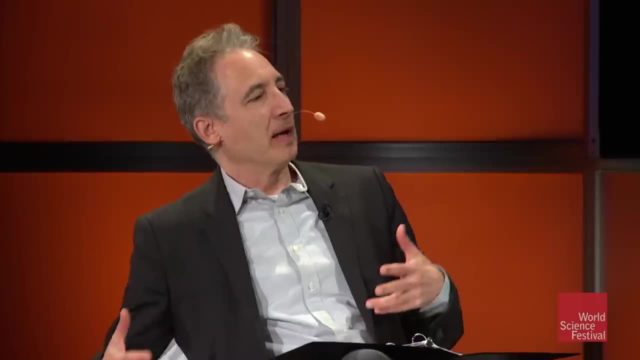 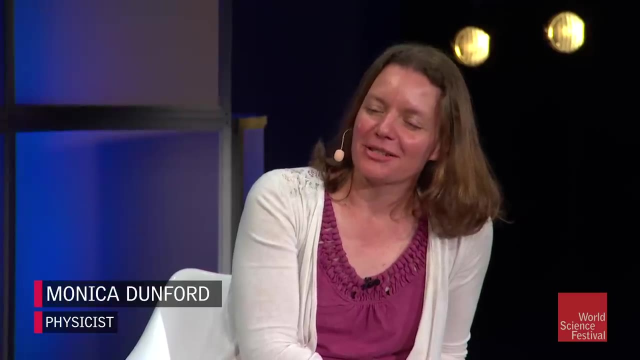 equals MC squared, sort of the most famous of all formula. So you know, are we using energy to create stuff or are we just sort of smashing things to bits? I think pretty much it's one and the same. I think it's just a question of whether or not. 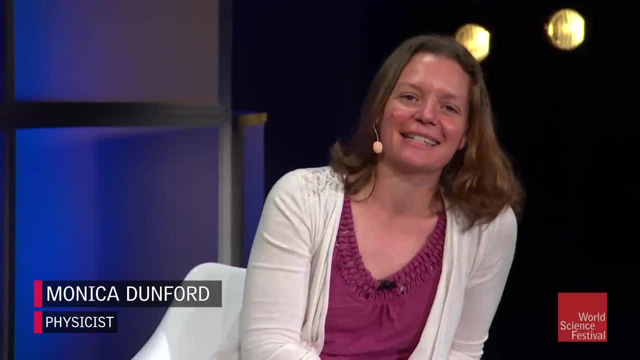 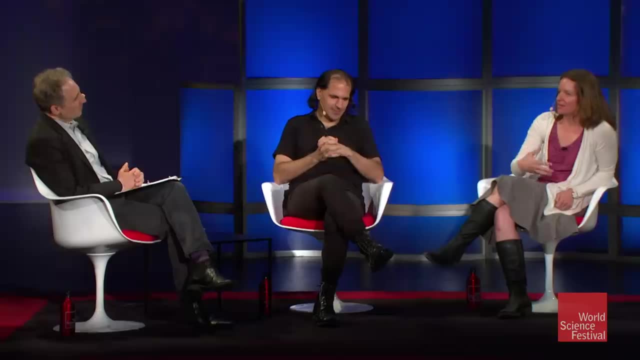 you want to speak elegantly or not. So yes, I mean, in essence, what we do is we take two things and we smash them together, And what we want out of that, of course, is a lot of energy, right? 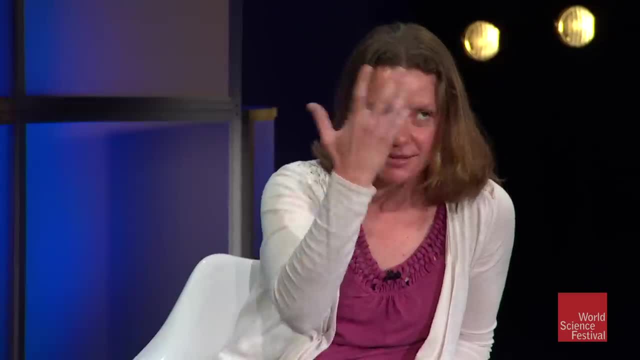 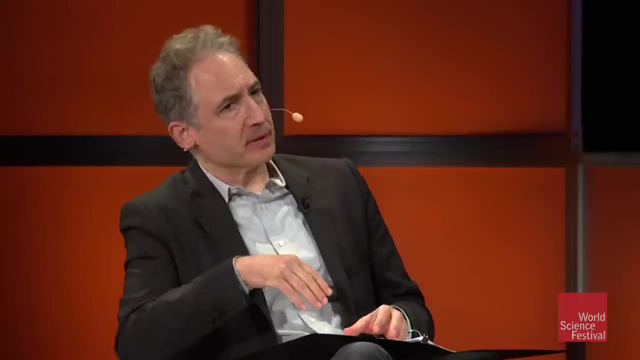 At any collision. you want a lot of energy And, as Einstein says, energy is equal to matter, and so, therefore, we can produce heavy things, and that's our goal. But a key part of that, and the point which I probably didn't say clearly, 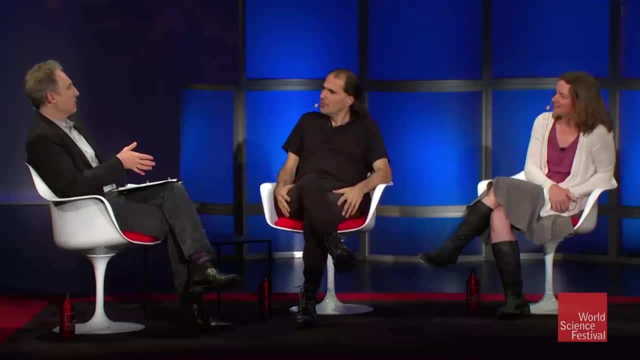 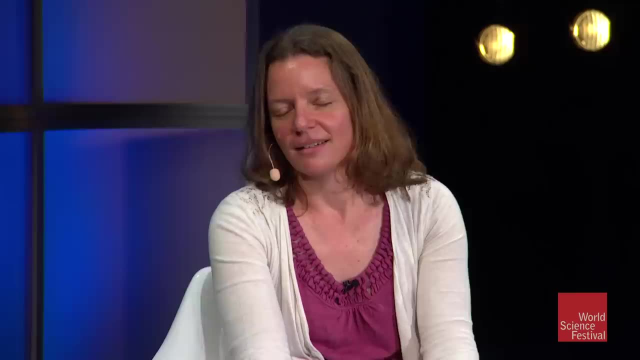 was. if you only are smashing things, you're only going to find the stuff that was literally there, whereas that's not quite what we do. No, that is absolutely not what we do. It's sort of like it would be more as if you took two. 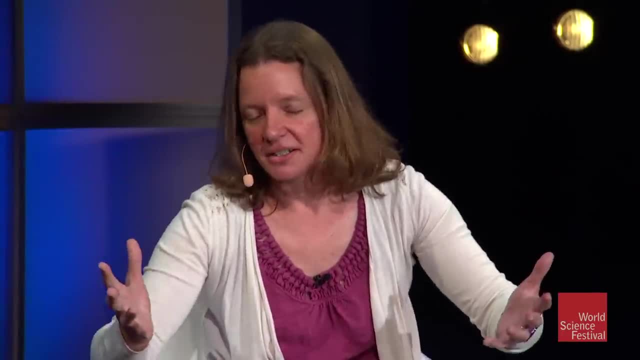 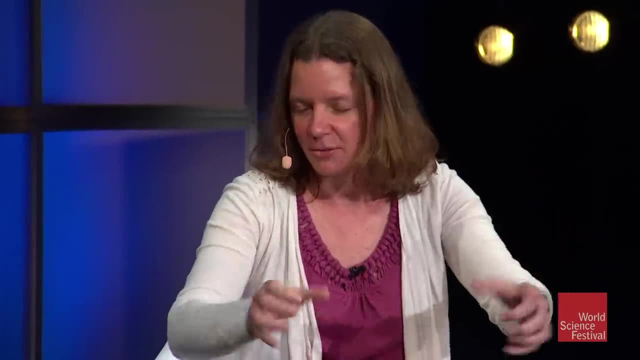 let's say, cheap coins, and you smashed them and you got yourself a Ferrari. right, That would be more the equivalent of what we're doing. I mean, you're really creating something new out of what you had, and what you had is now no longer. 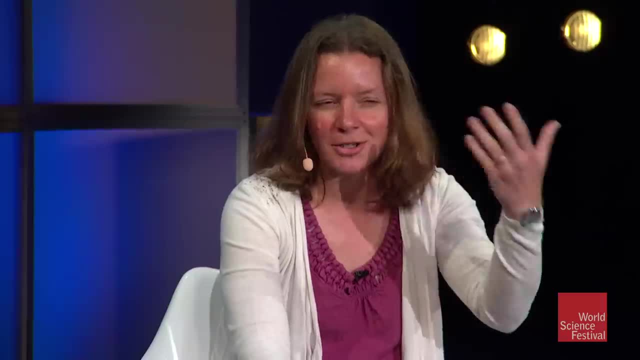 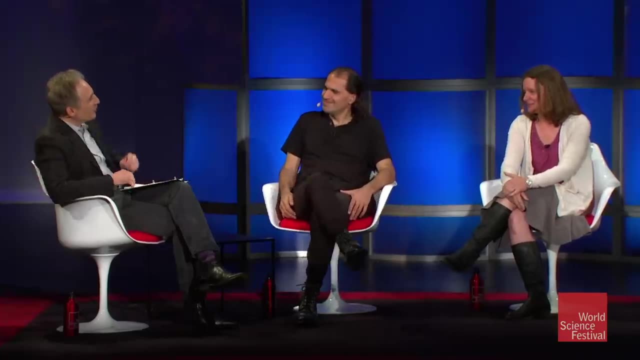 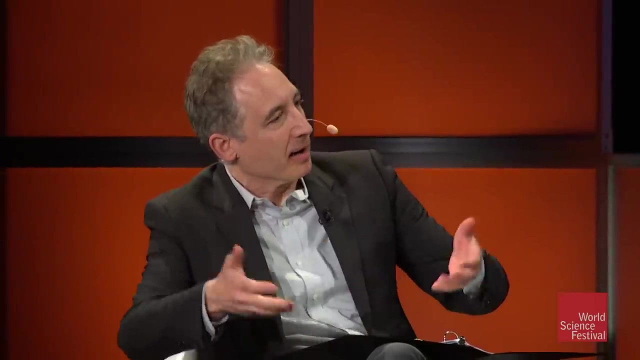 and you've got this elegant, hard-to-find status symbol that you're really looking for. So that is more along the lines of what we do. So, from that way of looking at things, energy is sort of the basic currency from which you can buy the status symbol. 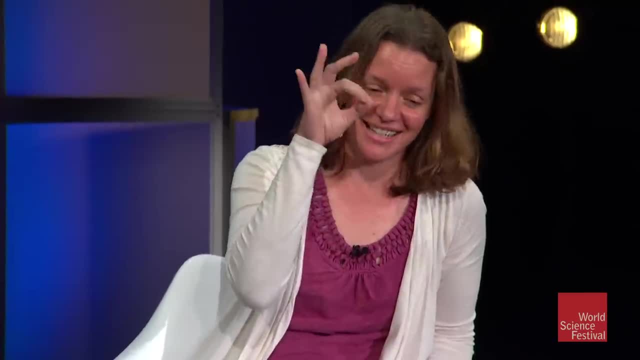 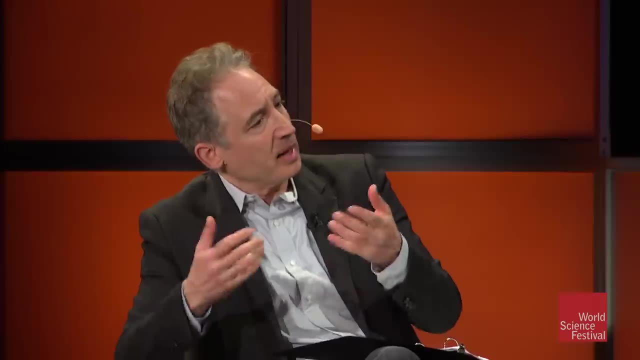 Exactly, Energy is money, Absolutely. Energy is money in our case, Right. So the more energy you have, the more options you have for the things that you can buy, or if we get off this metaphor, which perhaps is a good idea, 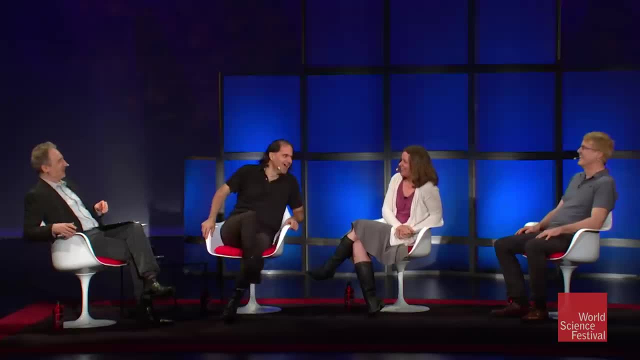 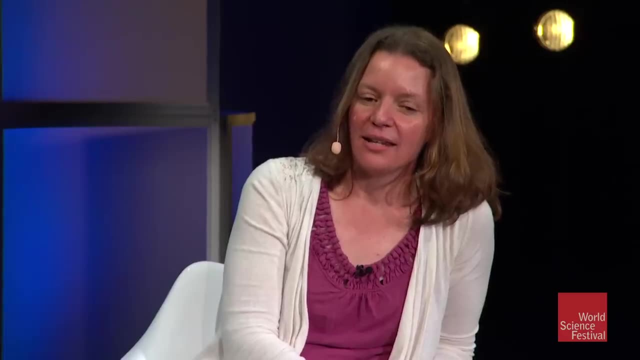 Yeah, that's done. I know Exactly. yeah, I didn't know that you were ever going. You know the greater the mass of the particles that you're able to create through these collisions. So the idea behind any sort of what we would call 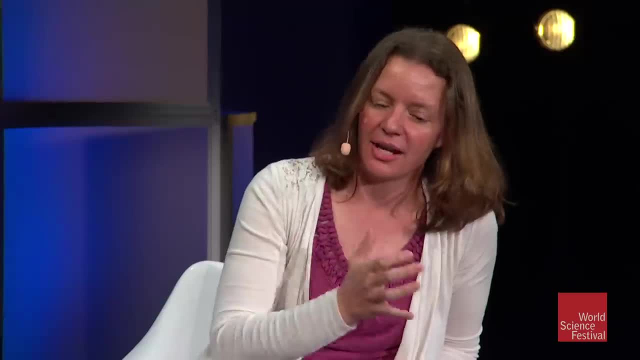 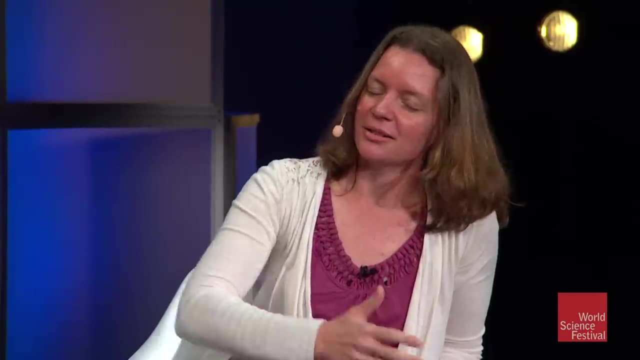 frontier collider is that it needs to be as energetic as you can buy. really literally, You want it big, you want it powerful, you want tons of particles, you want tons of energy, you want it all. So the most powerful collider of that sort, 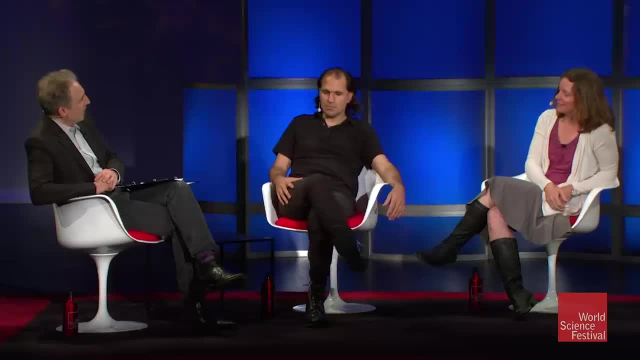 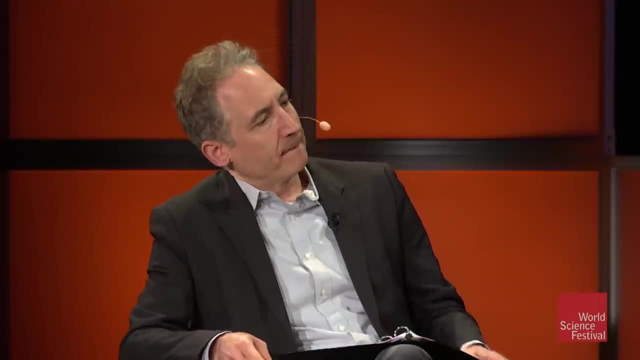 that we have today, I gather is where you work. It's the Large Hadron Collider, That's right. So give us some sense of what it can do and the energy that it has, and so on. So the Large Hadron Collider. 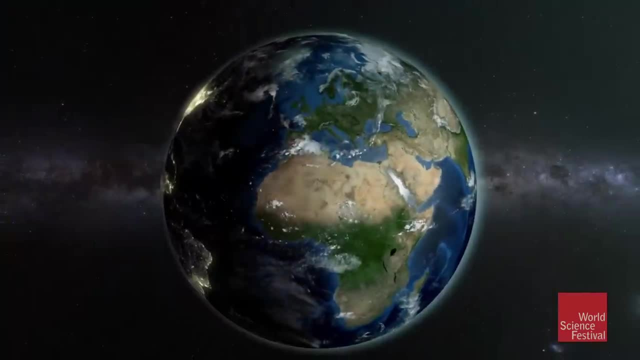 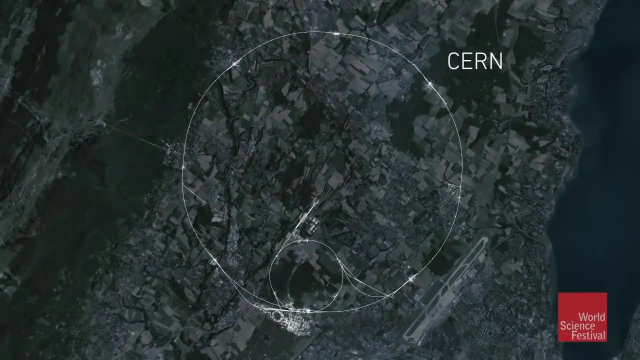 yeah, it's in a tunnel, it's about 27 kilometers. located near Geneva, Switzerland, in probably some of the most expensive real estate in the world, So probably in future colliders. well, you wouldn't have designs in Switzerland now? 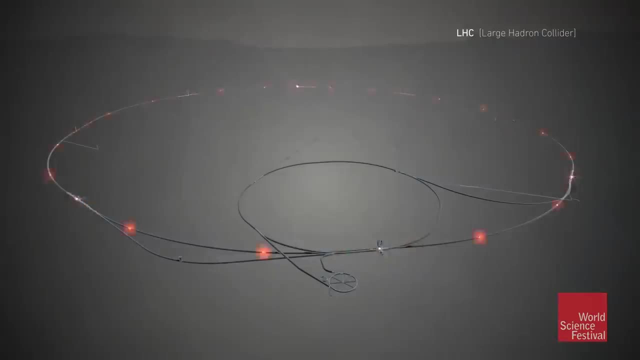 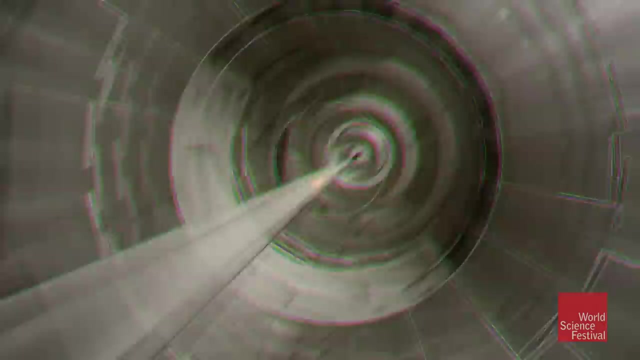 let's say, but it's where we have it. And the idea is, you've got two protons that are running around in this ring in opposite direction. They're being accelerated by superconducting magnets. They are, you know, getting to very, very high energies. 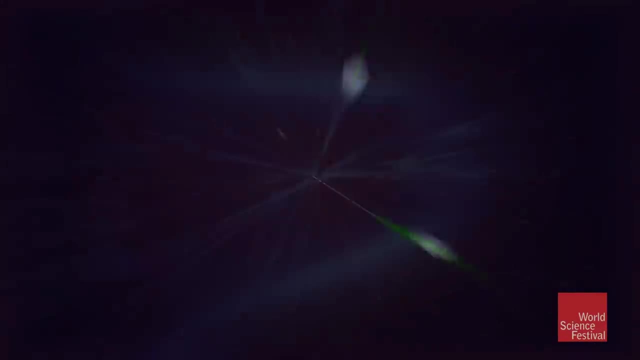 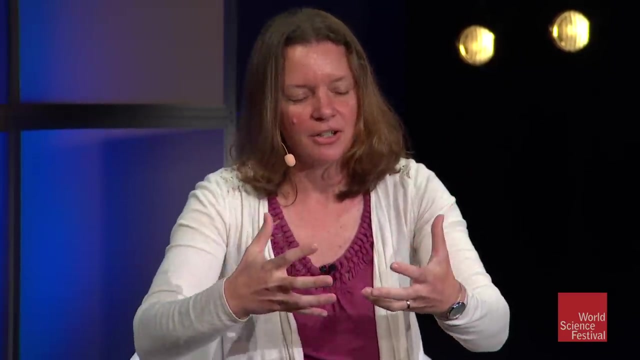 Energy is this currency here, so the higher the better. This one runs well at 13 TV, soon to be 14.. And then you collide them together. You have a tremendous amount of energy in that collision and you basically build this gigantic detector. 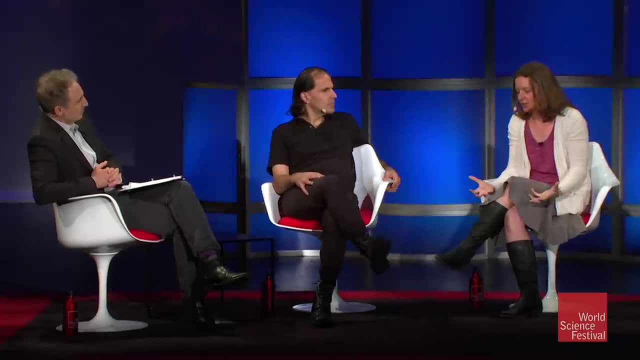 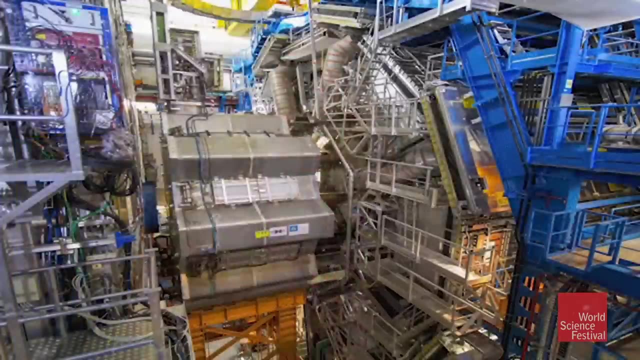 We have four such detectors. You build these gigantic detectors around that collision point. You know, the Atlas detector, which is a detector that I work on, is a five-story building, so it's humongous. And that basically takes a snapshot of the collision. 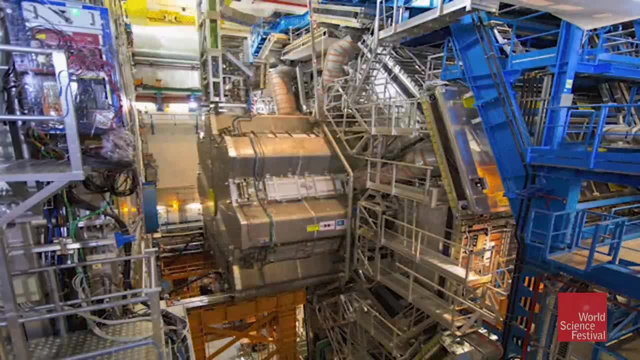 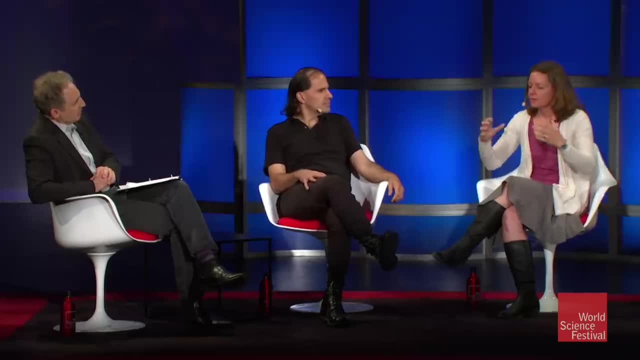 And the collision is messy. It's not like you know a couple of particles here or there, right? I mean it's like: So how many protons are in these bunches that are slamming? So in the protons you have many, many protons in the bunch. 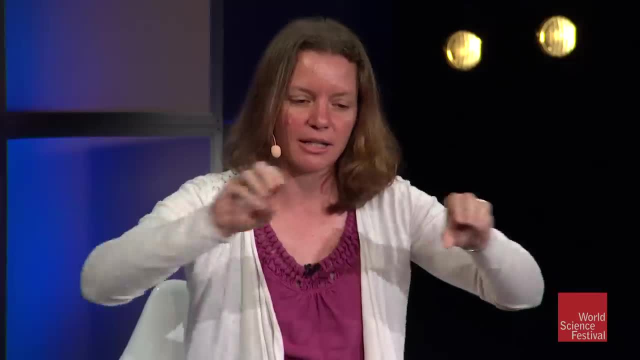 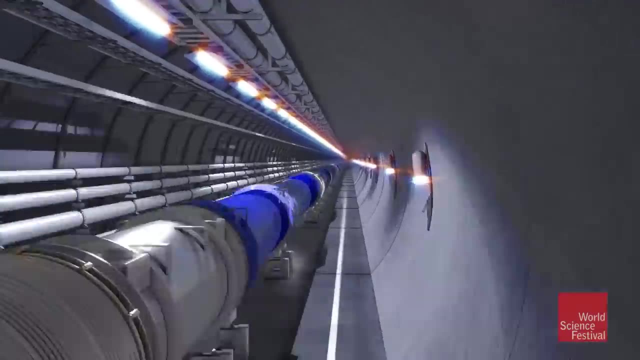 So the beam is not a continuous beam, as you might think. It's not like a stream of protons that are coming in. The beam is designed such that you have like little packets of protons- you know well, 10 to the 11th around. 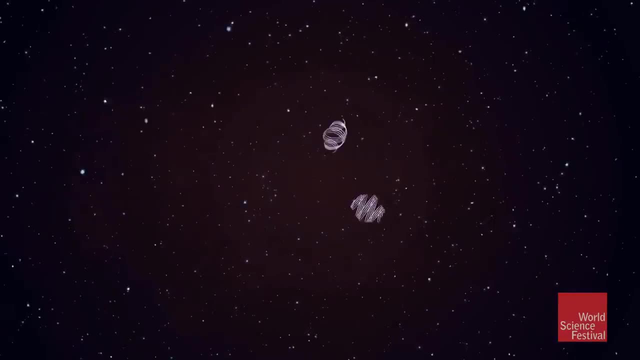 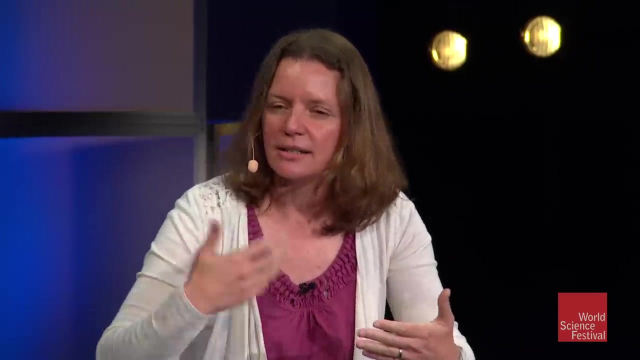 And you have these little packets of protons and they're kind of colliding every 25 nanoseconds, which means that it's like your camera, your detector's a camera and it's taking pictures every 25 nanoseconds, So 40 megahertz speed. 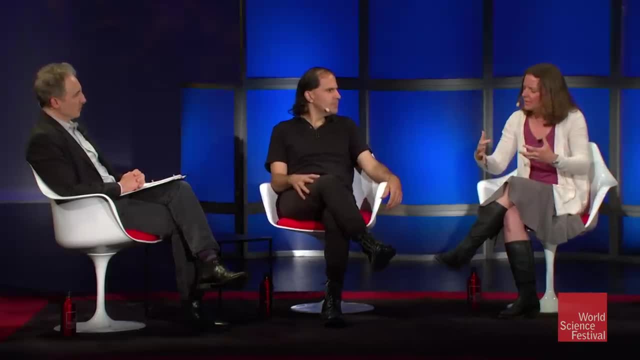 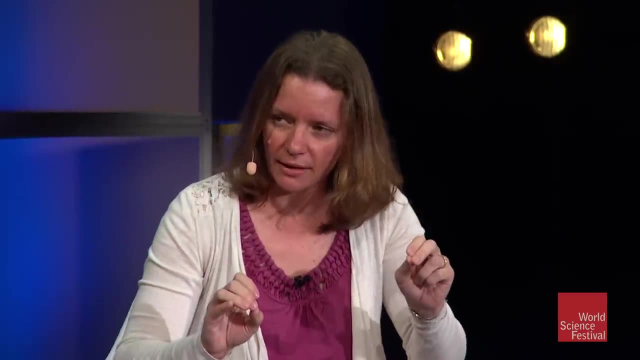 And these collisions are so big and they're happening so often that we actually cannot record all of the data and we have to make a very difficult decision quickly, within a microsecond, about whether or not this event is interesting or not. 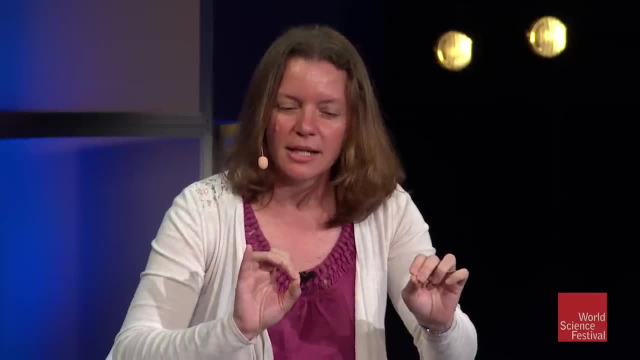 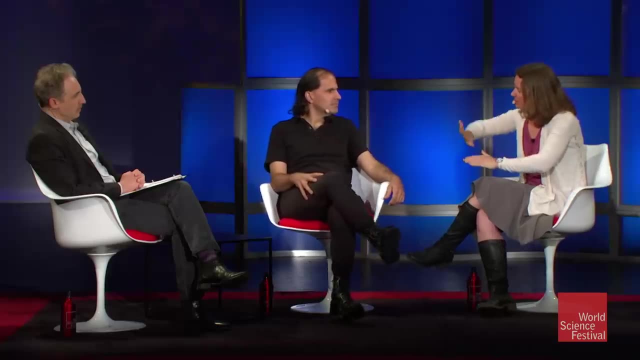 And this is a very challenging thing for us- experimentally, because, if you know, Nima comes to me a year from now and he says: oh, you know what? I think I saw a new signature. It would be something totally different. 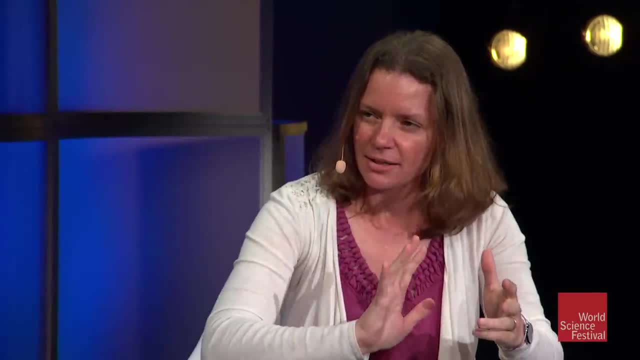 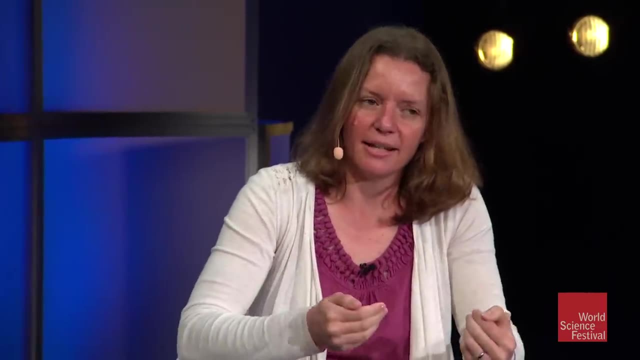 and it would have looked like this. And if my trigger system, that system that makes that decision, says, oh, I can look for that, or couldn't? the data's lost? I didn't record it, So I can't go back to the data and say 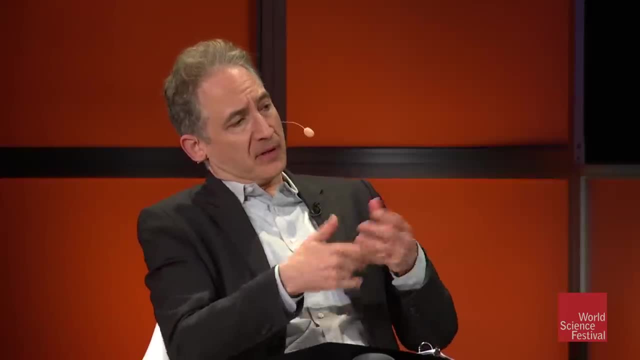 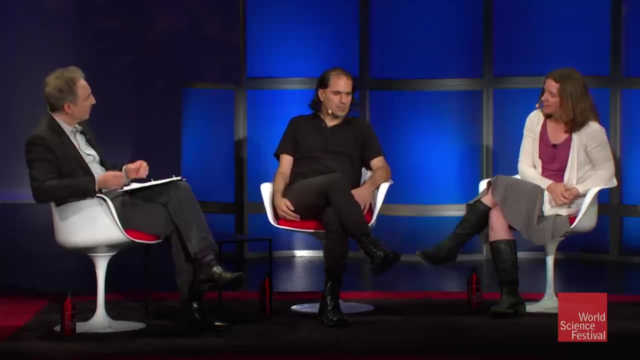 ah, I can look for that. So theory really guides the experimental approach. It's not as though you approach it as a blank slate and say let's slam these things together and just see what happens. Well, absolutely, And it's also a very difficult challenge experimentally. 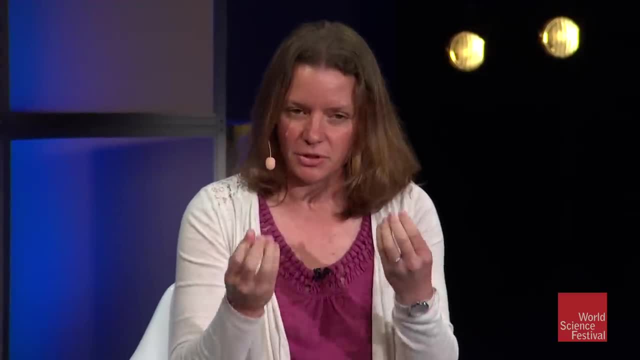 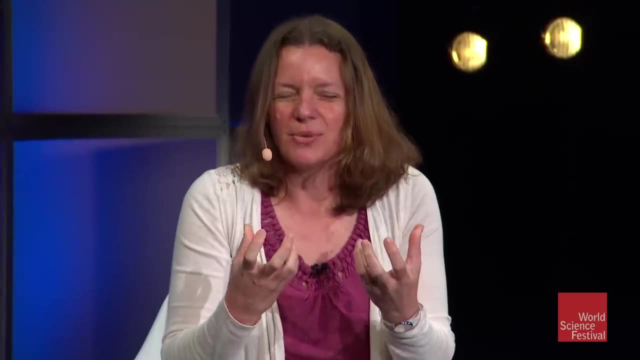 because in one hand, you need to be ready for everything. Your detector cannot record everything, So you can't take everything. We're ready for everything. However, you need to have made a decision, So you need to sort of have some sort of idea. 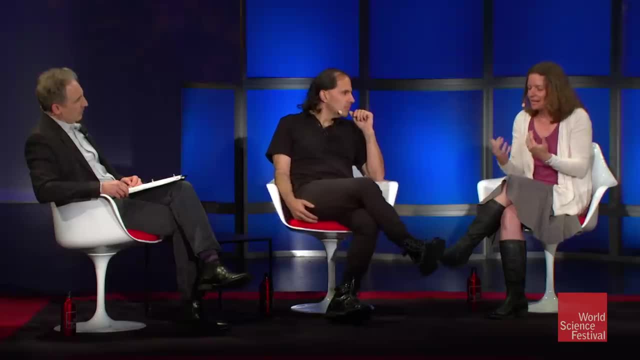 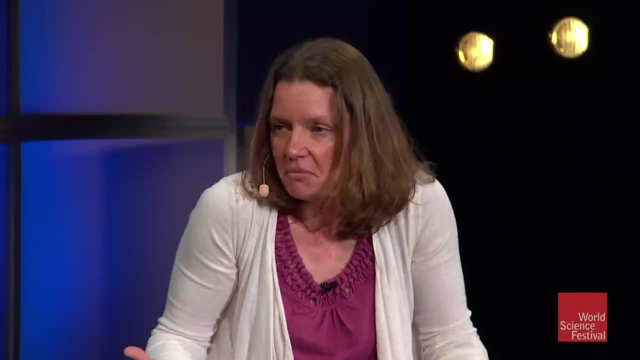 about what you're looking for And to get that idea of what we're looking for, then, yes, of course, we rely heavily on theory to tell us that, because otherwise You're at sea, We're at sea, We're absolutely at sea. 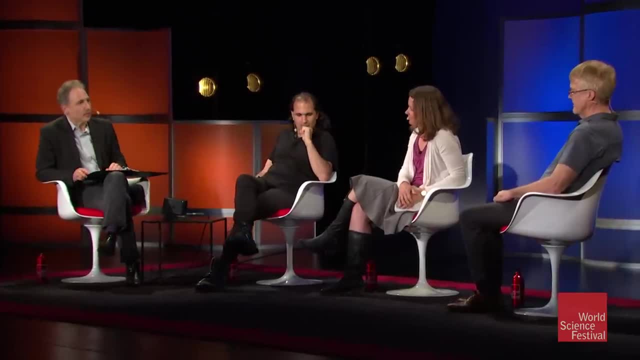 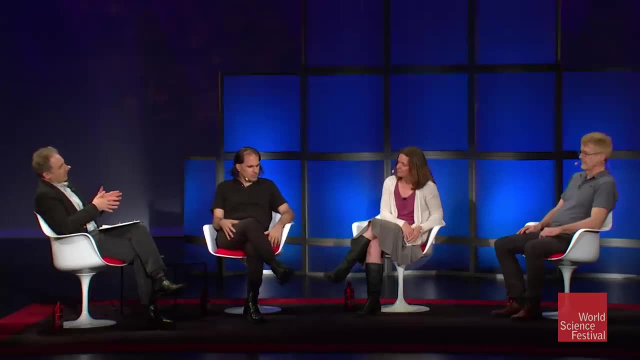 So, Joe, you of course also have spent your career working at a facility that undertakes these kinds of experiments as well- Fermilab- And, over the course of decades, both through collider experiments, but also through other kinds of experiments, 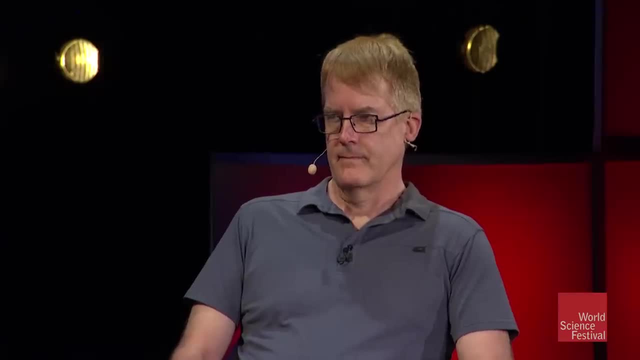 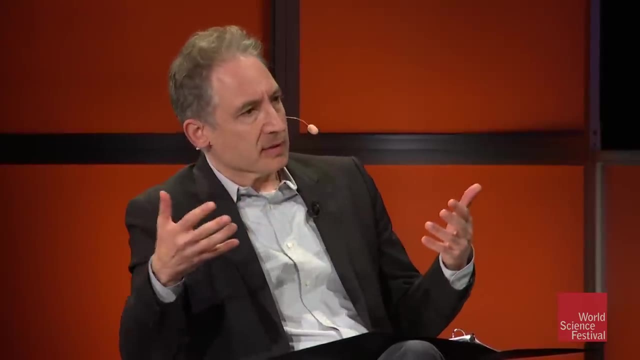 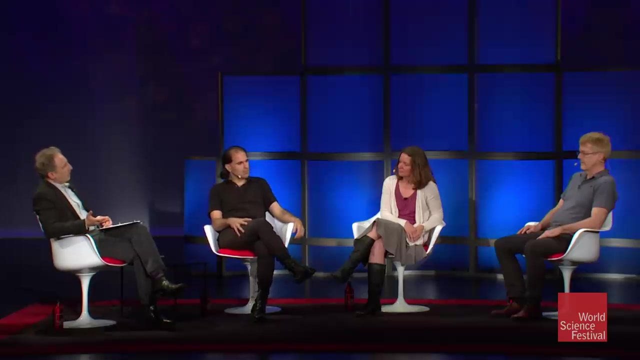 that we won't go into any detail. you know, cosmic ray experiments and other things of that sort. we have built up what we think may be the fundamental ingredients making up at least the stuff that we interact with in an everyday sense, And that's the standard model of particle physics. 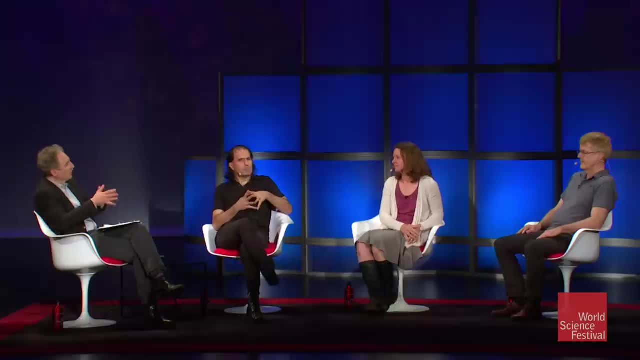 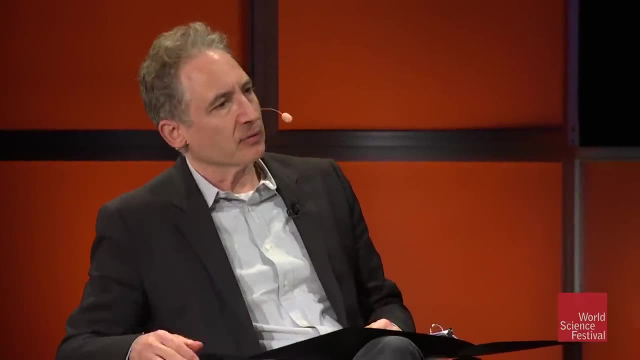 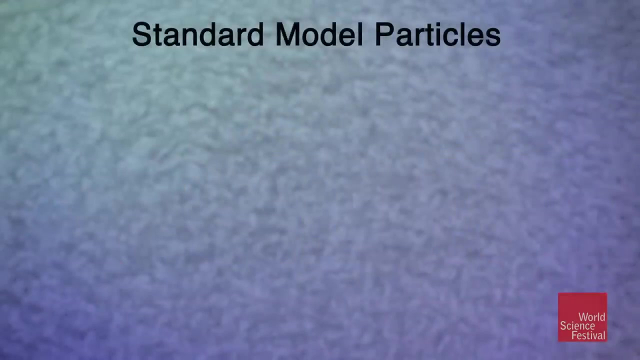 So I just wanted to go through the particles that were predicted and ultimately found, giving us our most complete understanding to date of what things are made of. So in the early days of looking for particles, maybe you can just sort of take us through some of these particles here. 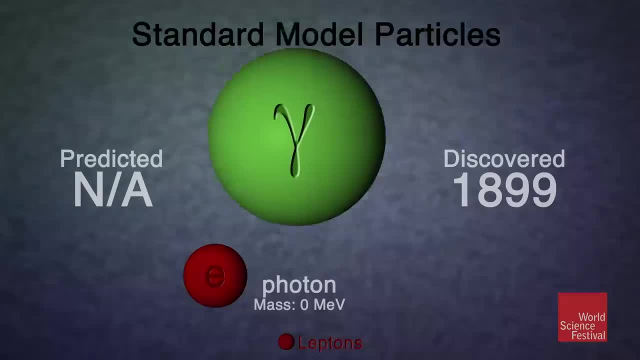 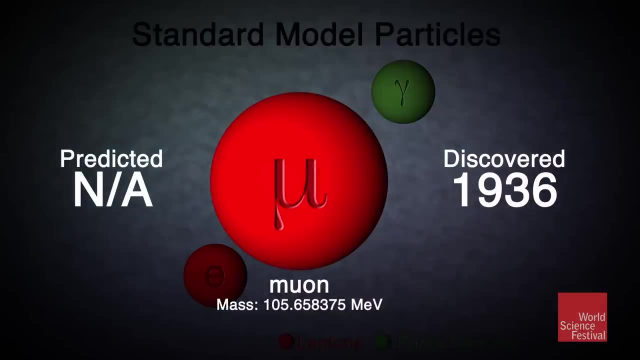 So that's a familiar one: electrons. Everybody knows electrons, Everybody knows photons. The muon was an example of a particle that wasn't predicted but was discovered, and we still don't know why they exist. but they are also fundamental particles similar to electrons. 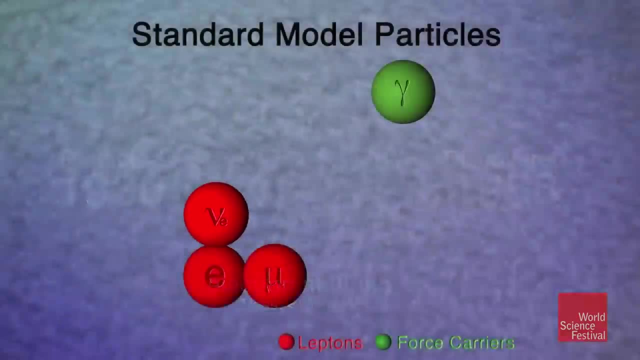 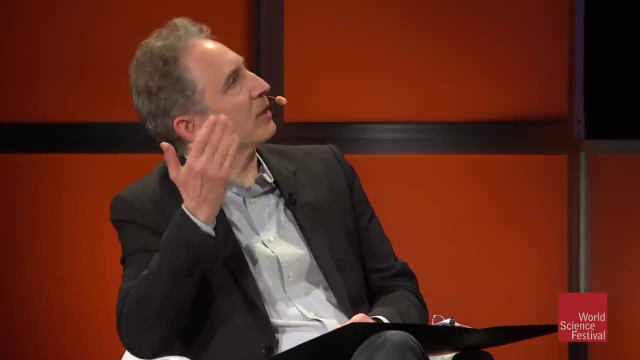 Neutrino is even stranger. We know they exist, but they're very different from the particles that you're made out of- and that's one of the things we're still trying to figure out. And they what? They have no electric charge. 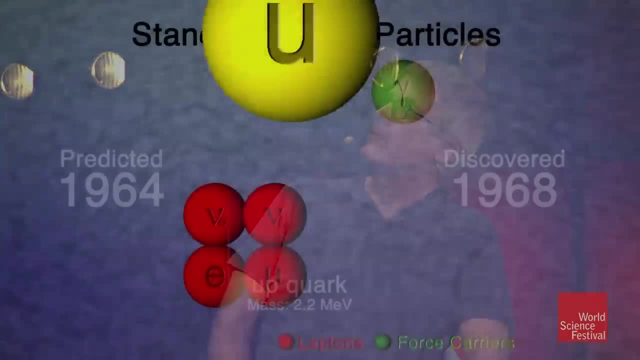 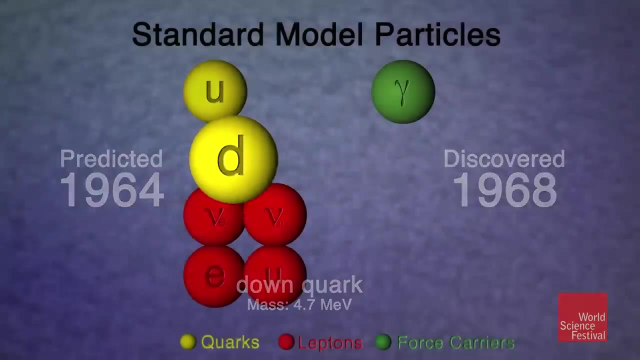 They don't have any electric charge, They're very difficult to detect and they're very different from other particles- Quarks. Murray Gell-Mann, who just recently passed away, invented the idea of quarks You are made out of actually. 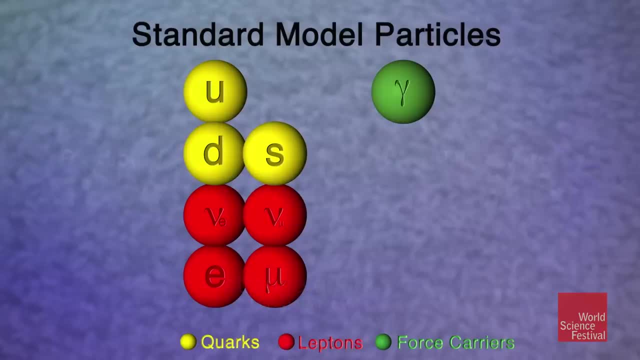 only three of these particles, the electron, and two of those quarks, the up and down U and D quarks. That's what all of I believe, that's what you're made out of, That's what all of you are made out of. But there are more quarks. The strange quark you see there was discovered later, and charm quarks, bottom quarks, top quarks- were discovered at my laboratory Fermilab. We're very proud of that. And what year was that? 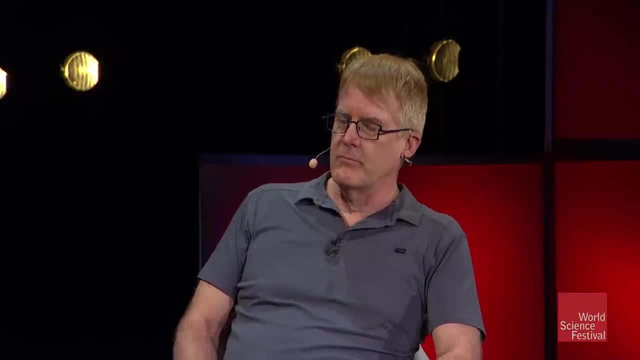 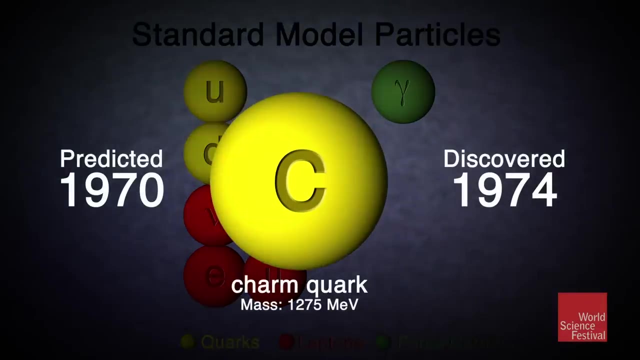 That was in 1997, with what was then the world's biggest particle collider, the Tevatron, before the LHC, And we don't know why there are so many of these elementary particles. There's way more than you need to make us. 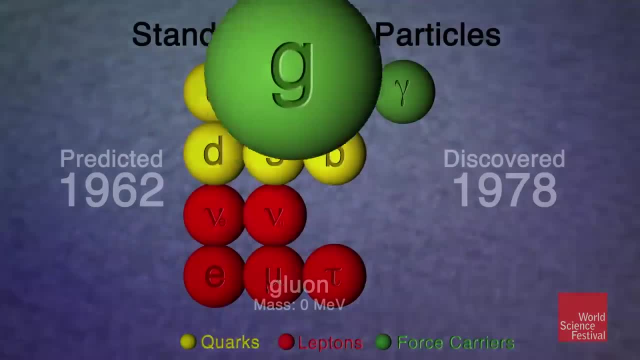 So that's one of the things that's still a big mystery and we don't know why they're so different from each other. We have some ideas for that, but it's part of the big mystery of this whole picture of the Standard Model. 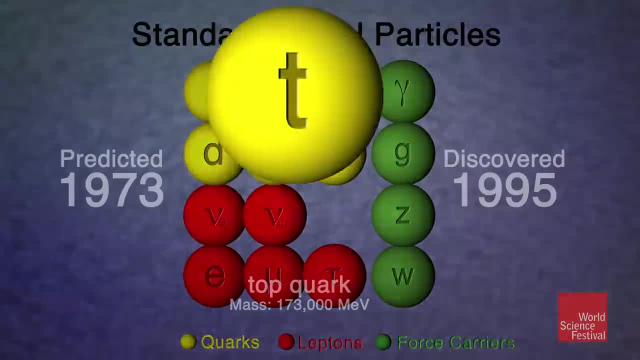 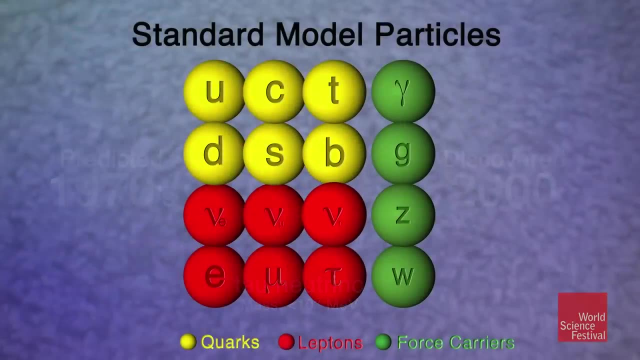 is. why is it so complicated, in some sense, and also why is it so simple? There are simple principles that hold it together. So we see here two collections of particles, if you will, The ones on the green on the far right-hand side. 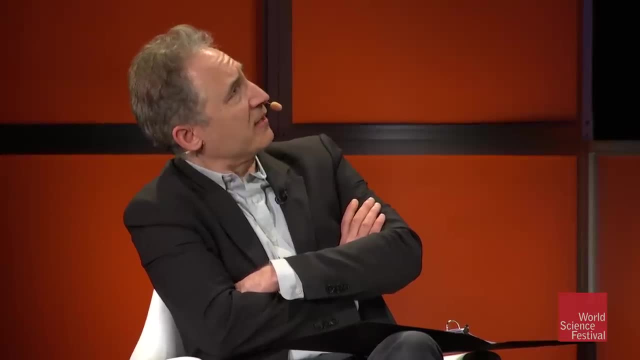 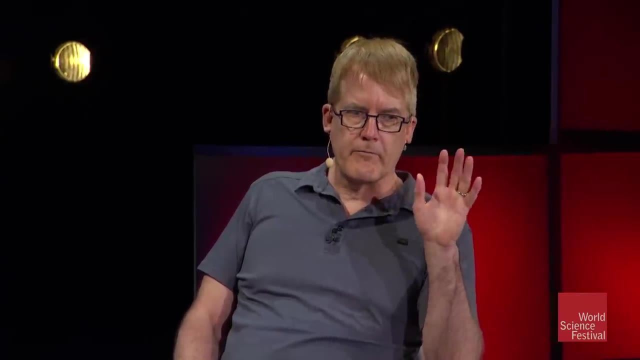 are distinct in a fundamental sense, In a fundamental way, from those on the left-hand side. Can you just draw that distinction for us? Yes, So the particles that you are made out of are called fermions, And so when we talk about matter, particles- 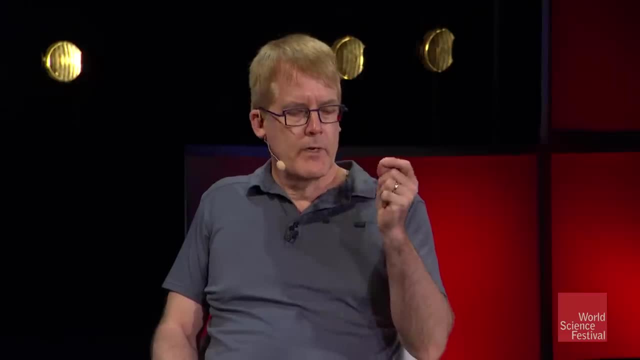 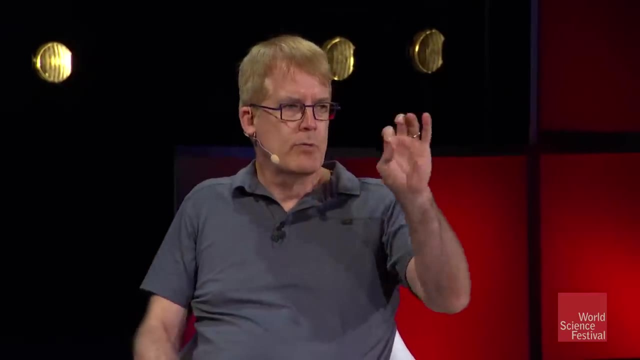 matter, particles are fermions And one of the ways of distinguishing them is that they carry a little unit of spin, which is not really spinning around like balls, because they're point-like particles, but they carry a little bit of spin-like angular momentum. 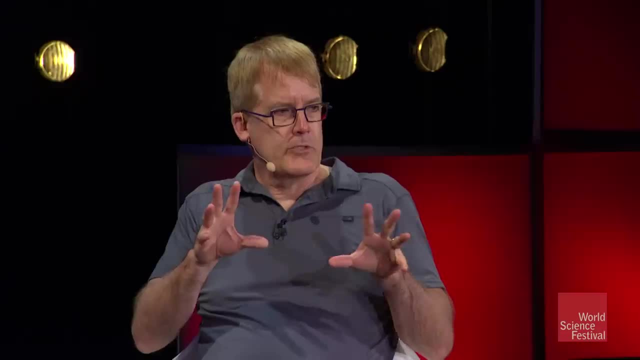 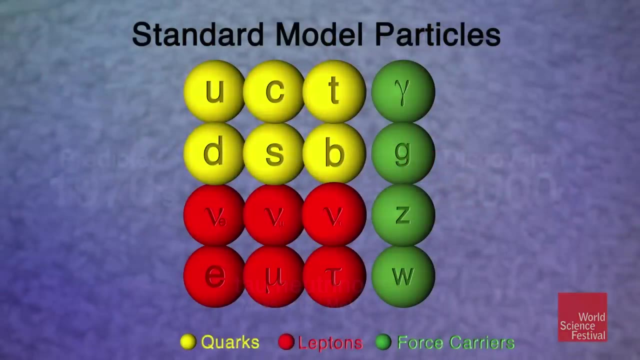 So you're made out of fermions. On the other hand, the forces that hold you together and hold the universe together are carried by these bosons, these green particles, of which the photon is the most obvious example for electromagnetism, But the gluon and the W and Z. 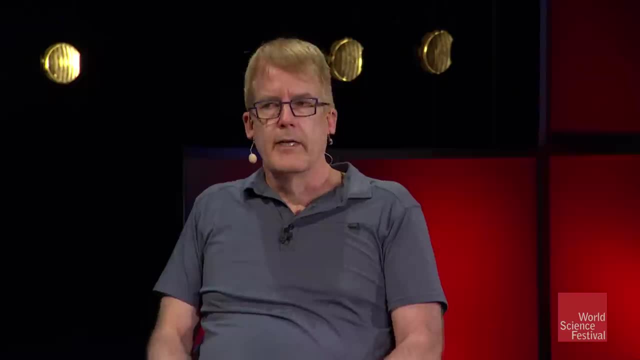 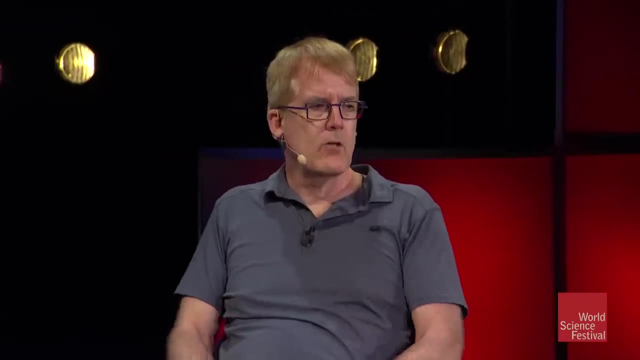 also carry fundamental forces of nature, And those are particles that have a different spin. They have a spin that's actually twice the unit of what fermions have, and they're called bosons, And they behave very differently. They behave like forces instead of behaving like matter. 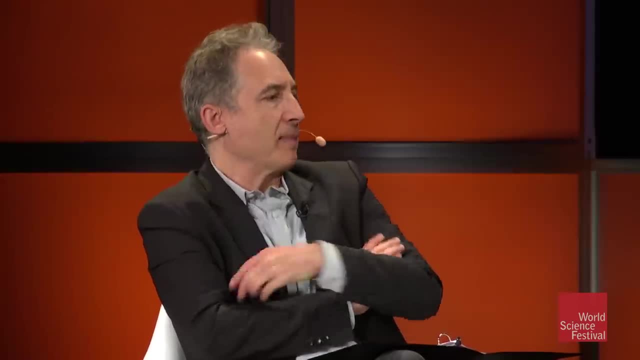 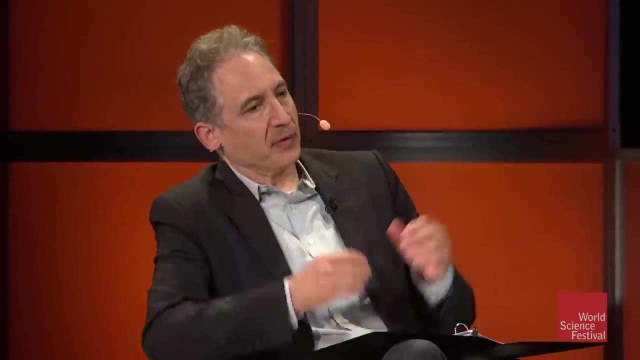 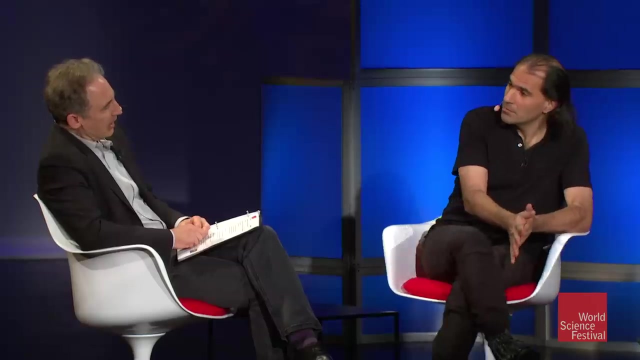 Now Nima. so when we actually begin to look at the mathematics behind this, one of the curious features that people recognize, even before the theory was fully in place, was that it was challenging to give mass to these particles And it's challenging to describe. 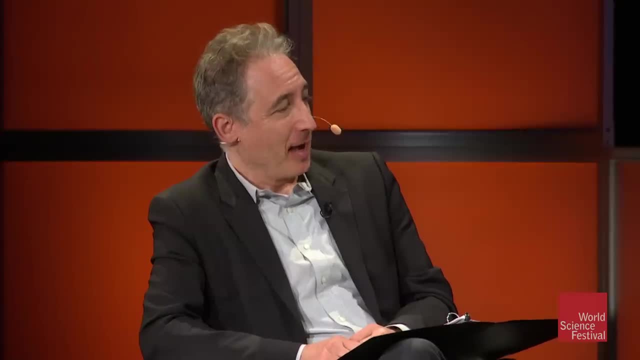 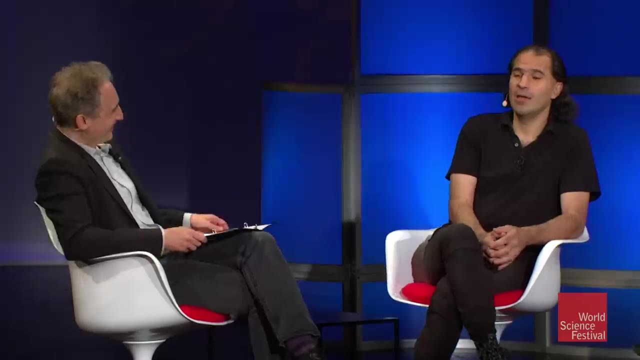 why it was difficult to give mass to these particles. I'm going to ask you to try to do it though. Oh, it's a piece of cake. Yeah good, It's actually a piece of cake, In fact, what we're about to talk about. 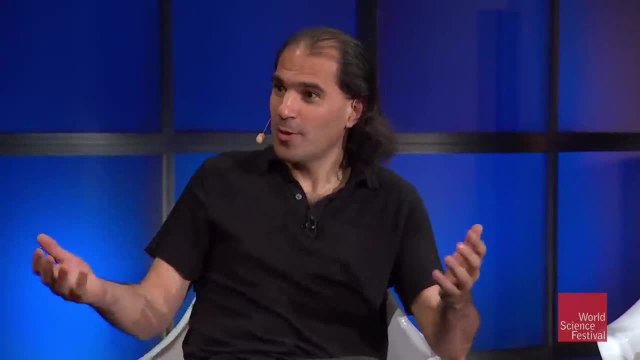 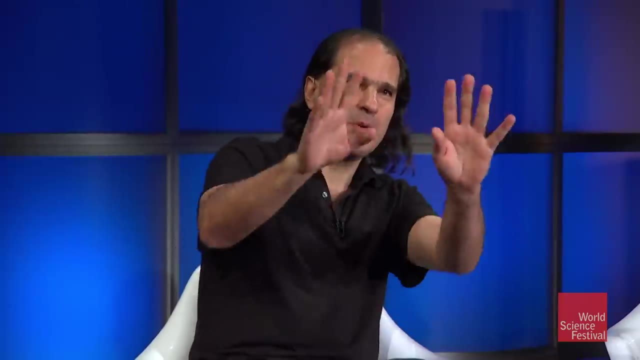 is a very large particle part of the conceptual drama of the 20th century in fundamental physics, and we're just going to have to count on our fingers a little bit. So maybe, before getting to it, I just want to make one just general comment. 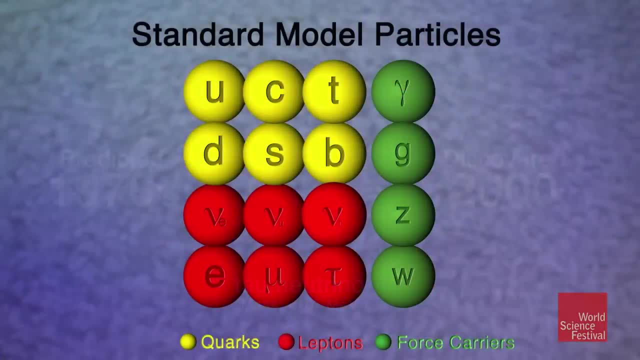 about this picture is that you might, and it's echoing something that has been said a couple of times already. On the one hand, it looks a little bit complicated. It's not the most complicated thing you could imagine, but there's many particles. 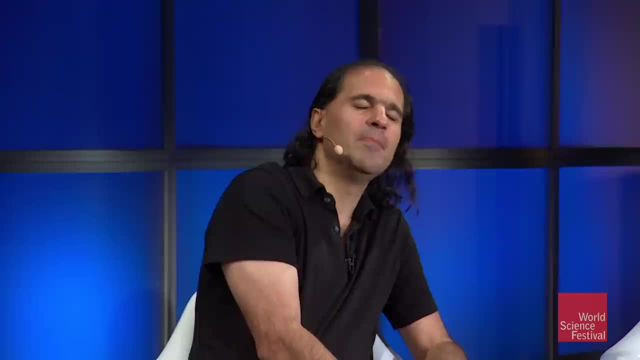 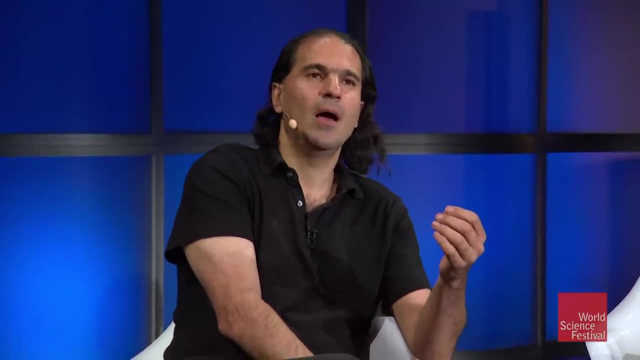 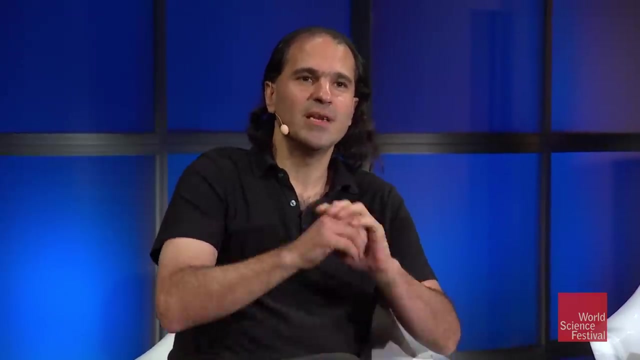 and it seems a little haphazard and random perhaps, But one of the aspects of our subject, I think the deepest aspect of our subject, is that all of these things are somehow completely governed and their properties, their broad properties, are almost entirely dictated. 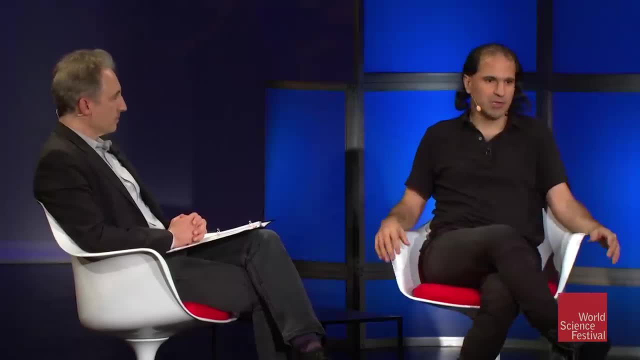 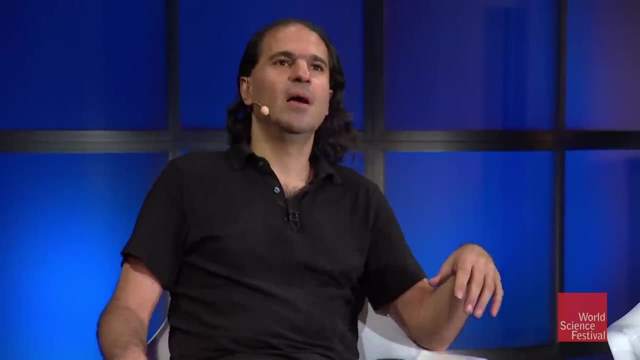 by big general principles, these two revolutionary principles that we learned in the early part of the 20th century, of the laws of relativity and of quantum mechanics. It turns out that these laws are almost incompatible with each other. It's not at all remotely obvious. 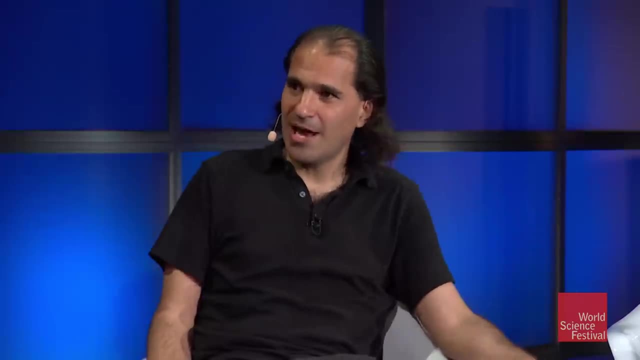 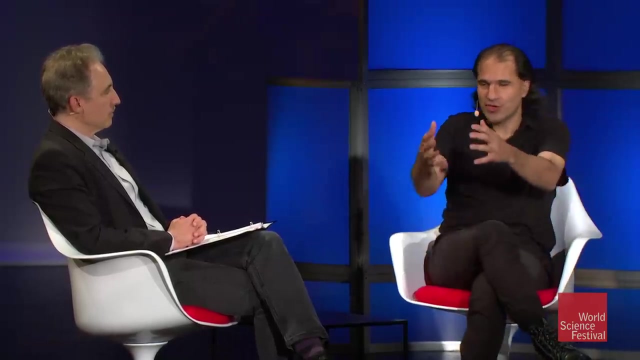 that you could come up even with toy universes that were compatible with the principles of quantum mechanics. but you just barely can. And if you hand sufficiently competent theoretical physicists these laws and lock them up in a room and refuse to let them look outside and just say: 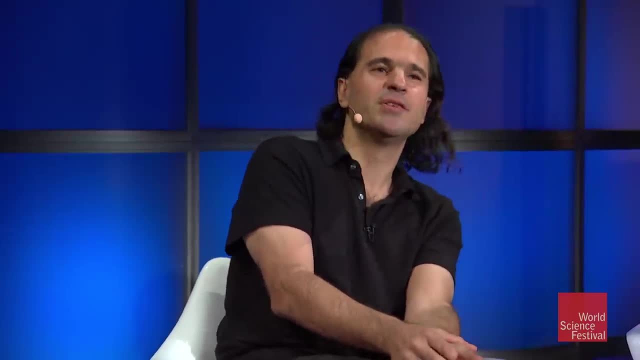 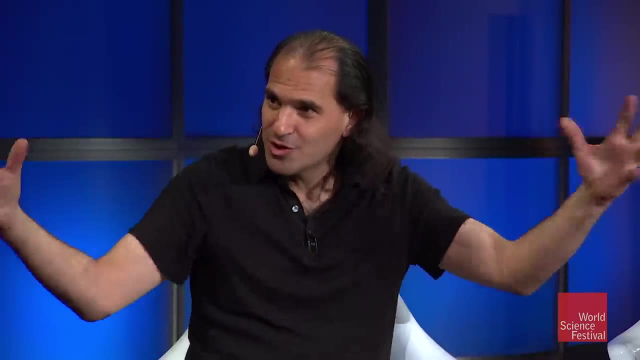 what could you come up with that's conceivably consistent with these principles, then this is the kind of thing that comes out, in a sense, out of pure thought, Once you put in, of course, these two big facts that we've observed experimentally. 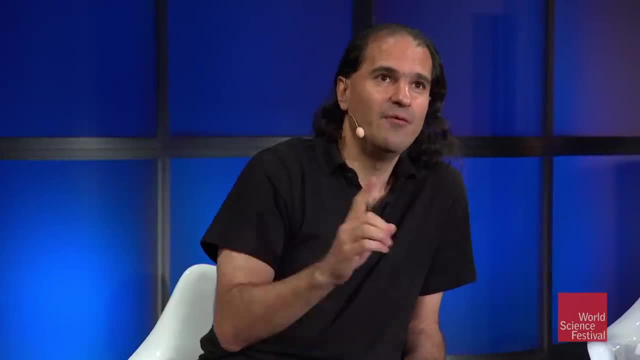 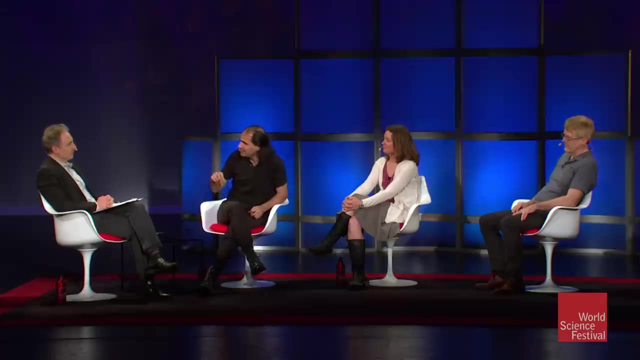 that relativity and quantum mechanics are both true, And a very big aspect of this, and a very big reason why it's so constrained, is exactly this business about the difference between being massive and being massless. So let me try to describe this. 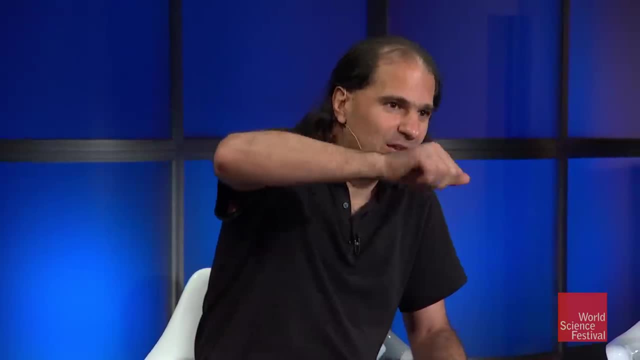 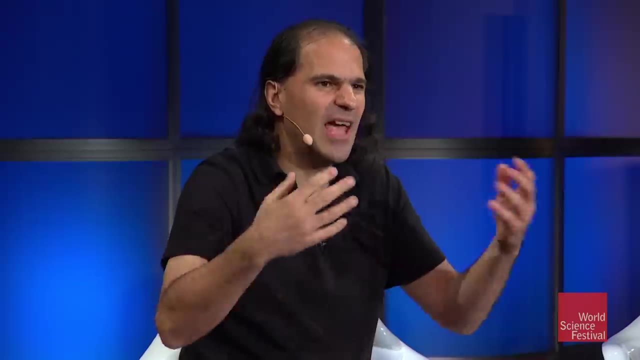 We just talked about the photon And, as Joe mentioned, one of the properties that the photon has is it has a little spin, If you're familiar from just thinking about light as a wave, sort of classically as an electromagnetic wave, sometimes we talk about it 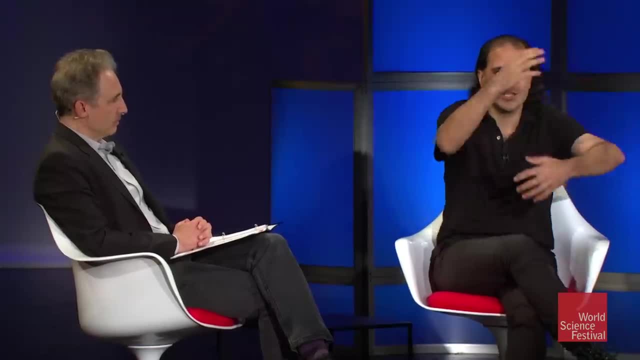 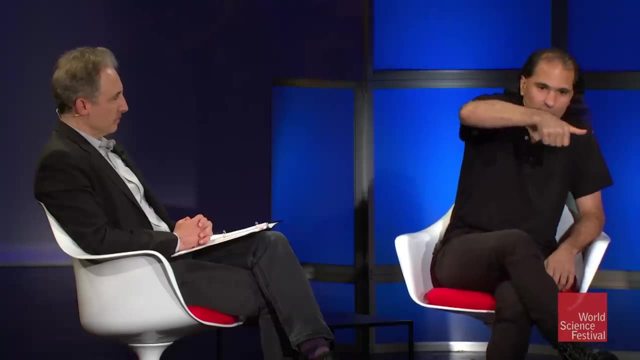 having polarization. It can spin around one way, It could spin around the other way. Well, what's really going on is the underlying photons that make up a light have a little spin, So they can spin either in the directions they're moving or opposite to the direction. 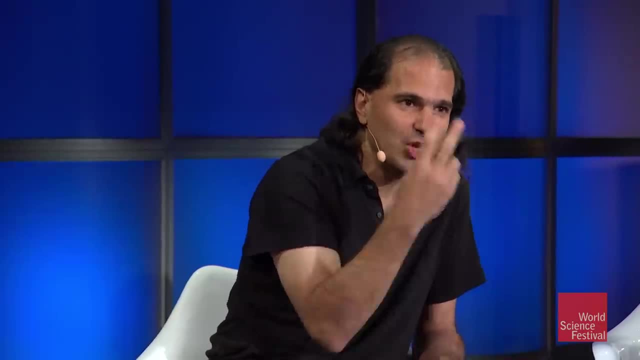 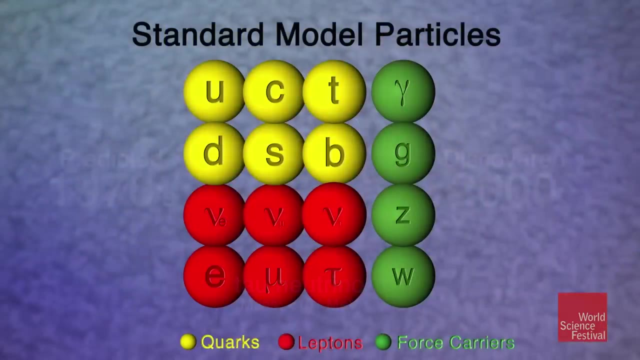 they're moving And this is a crucial fact- that they can spin in two directions. Now the other particles, like the W and Z particles, they are sort of massive cousins of the photon, But the mass is not a tiny correction. 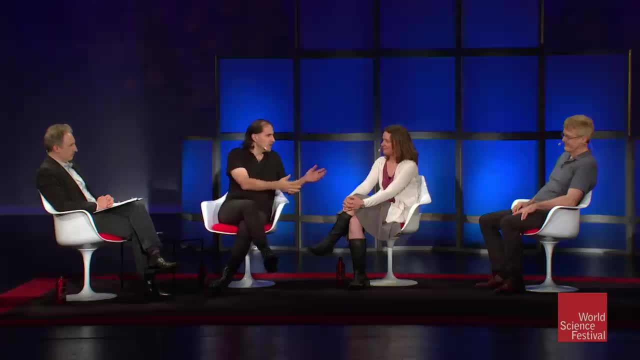 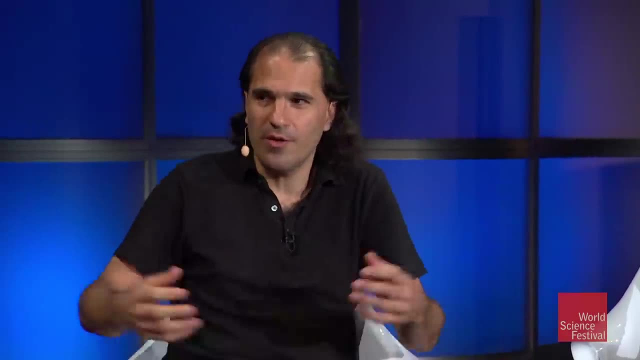 You see, if you're very naive, you would think, especially when we go to these huge accelerators, we smash particles into each other at incredibly high energies. Surely, when the energies are enormous, you can kind of ignore their mass so that the E? 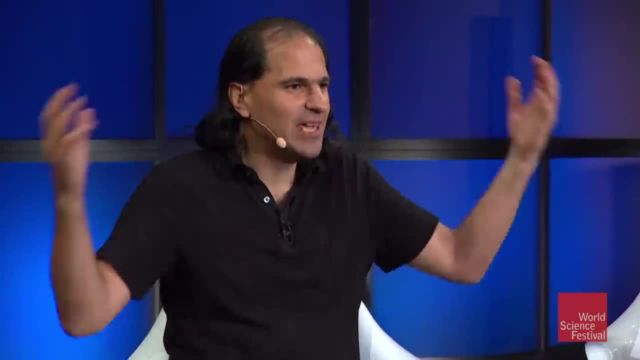 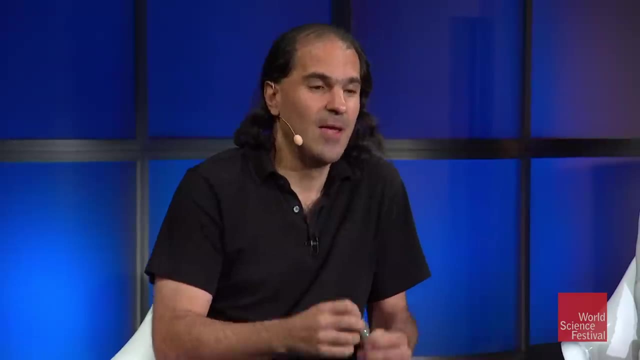 is so much bigger than the M so that you could really just basically ignore the mass, and you can at incredibly high energies. you can think of the mass as a little tiny perturbation and just talk about massless particles, But it's not true. 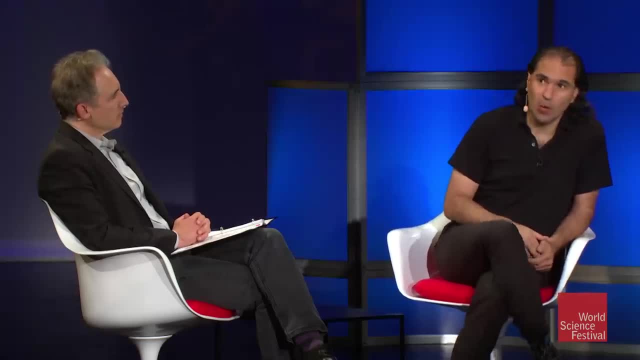 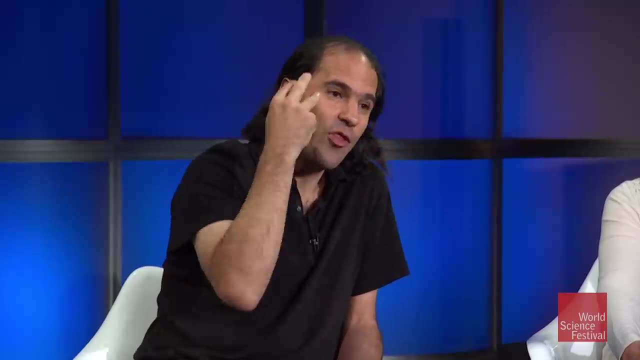 It's not true, because massive particles that have spin one, that have spin twice the spin of the electron- we say it's spin one, like the W and the Z- they have three ways that they can spin, While the photons have two. 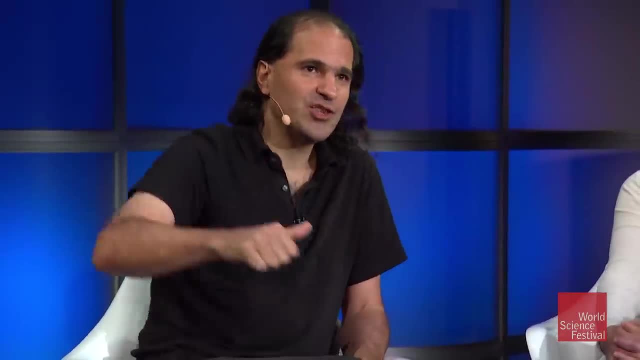 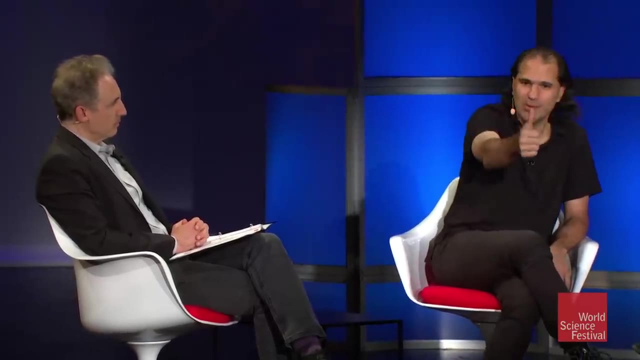 And what's this difference between this three and this two? It's no matter how quickly this W particle, let's say, is moving around, you can always catch up with it. You can always move and catch up with it. And let's say, it was spinning. 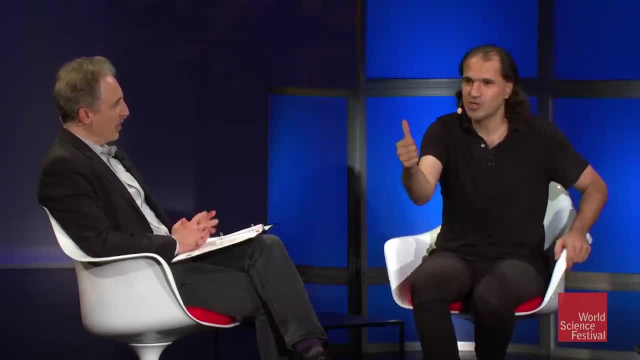 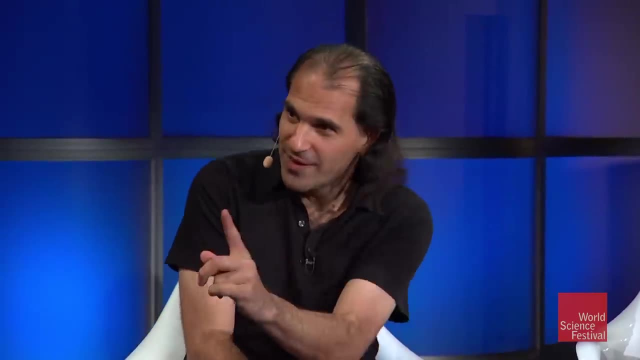 up this way. well, by tilting your head, you could see it spinning that way or the other way as well, And you could catch up with it, because massive is not going to be there. Exactly, That's right. That's the crucial point. 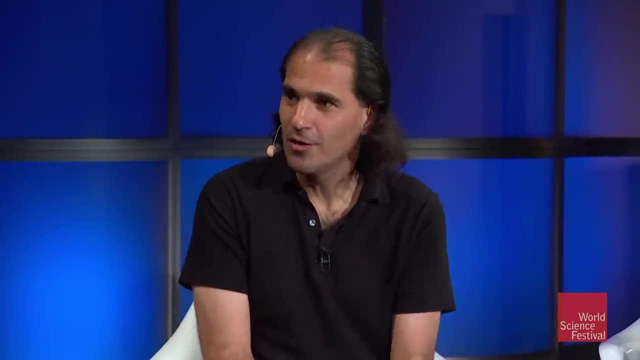 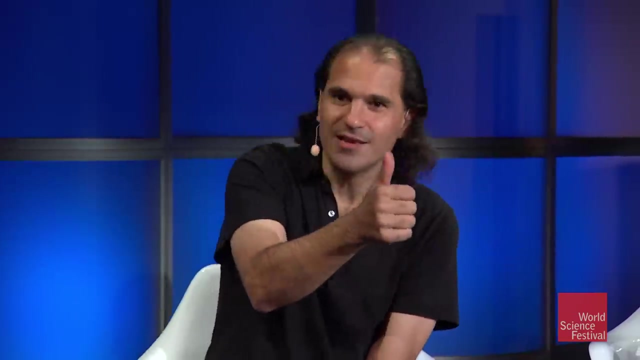 because it's massive, no matter how quickly it's moving. it's not moving at the speed of light, and so you can catch up with it at the speed of light. you cannot catch up with it, and therefore you can't play this game. 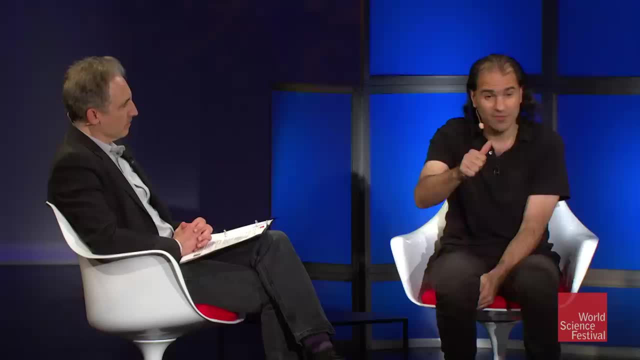 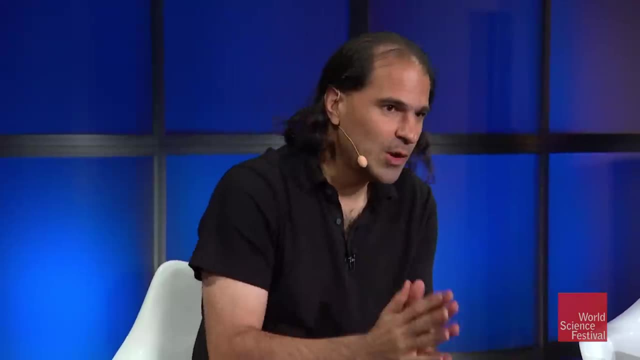 where you tilt your head and see it spin in every possible- in all of the three possible directions In fact. all you can do is conclude that it's either spinning in the direction that it's moving in or opposite to the direction that it's moving in. 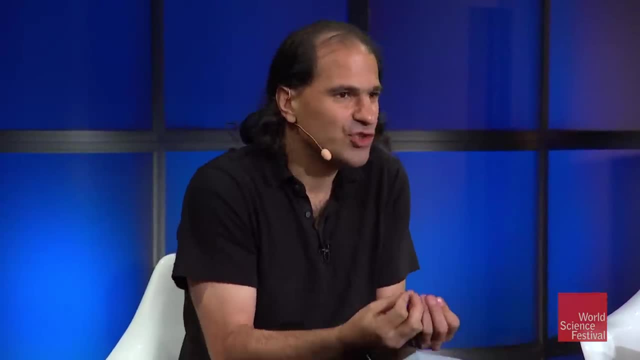 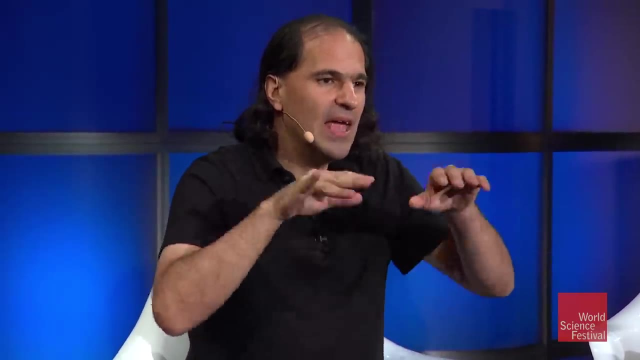 This two not equal to three business is really profound. It means that you can't think of mass as just a little correction to things that are massless already. And in fact, precisely because of this point if you attempt to describe the possible composition. 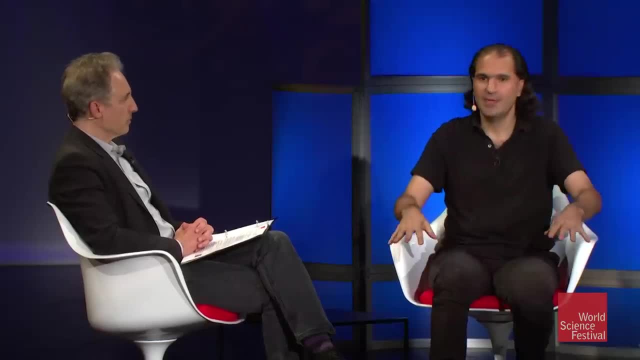 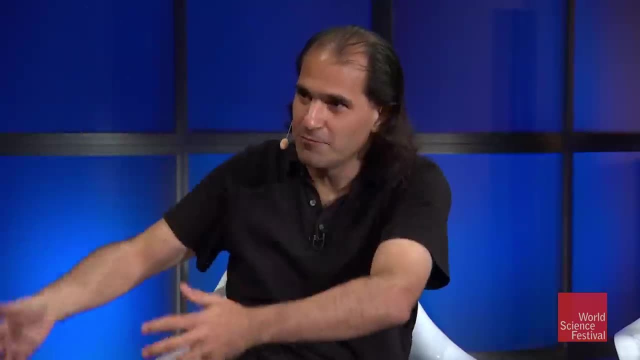 types and interactions of massless particles, then it's essentially a mathematical theorem. It follows from the again following from the general physical facts about the presence of both relativity and quantum mechanics, but the types and interactions of massless particles. that, you're allowed. 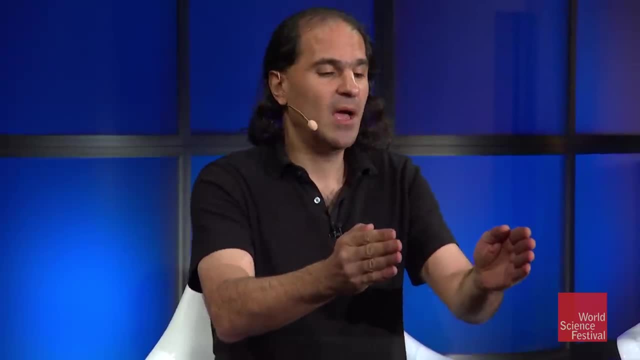 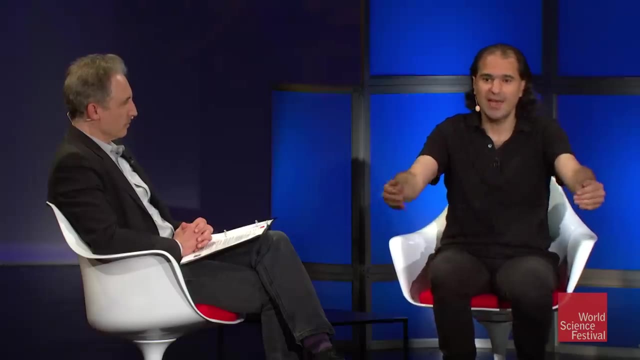 to have have to come in a miniscule variety. Okay, So the menu of particles that you're allowed to have that can interact in a way compatible with the principles following: The particles can have spin zero, one half. that's the unit. 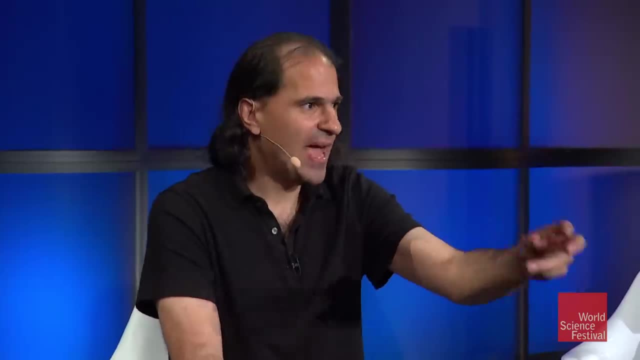 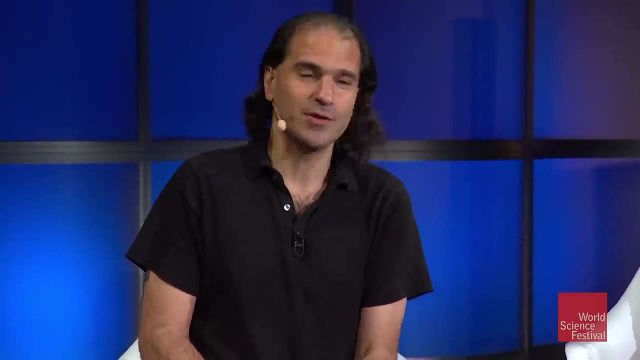 that the electron has. that's just a convention. So one, three halves and two, That's it. That's all you can have. Furthermore, there can only be one of those massless spin two particles. We're not gonna talk. 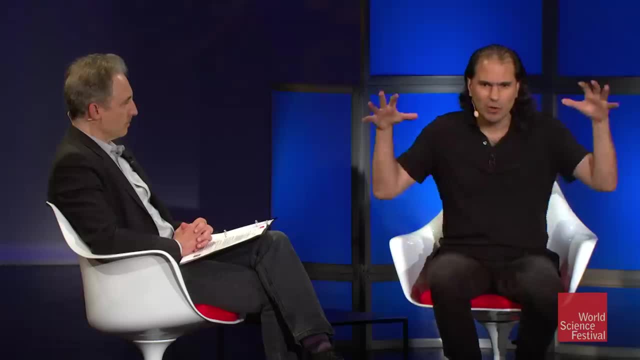 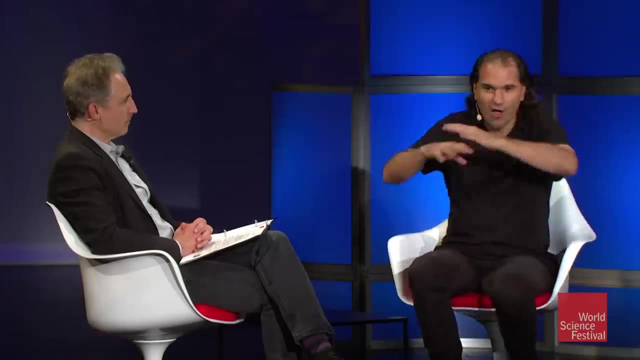 about it much today We can only have one of them, and if you study its properties that are sort of forced on you by relativity and quantum mechanics, you would find that it makes massive particles go around in orbits and so on. So if you're interested, 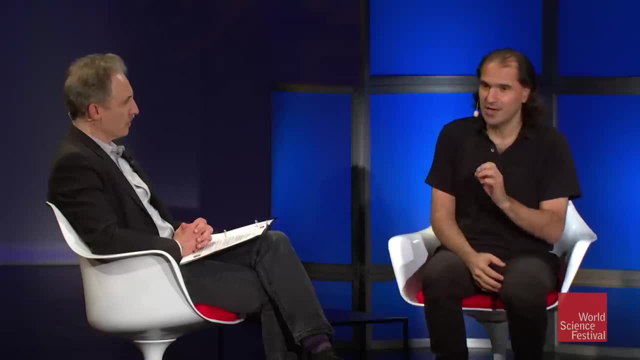 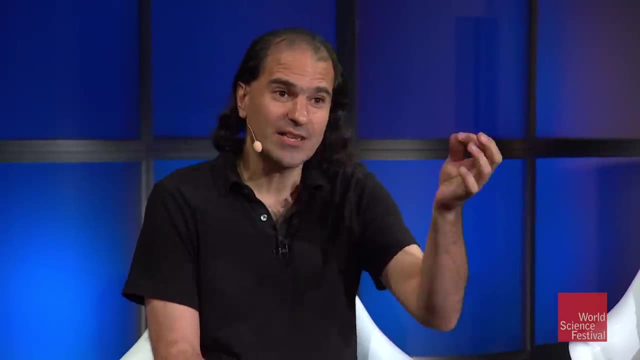 by these basic principles of Einstein's special theory of relativity and of quantum mechanics. then the spin zero particles: okay, you can have as many of them as you like. The spin a half, you can have as many as you like. The massless spin one particles. 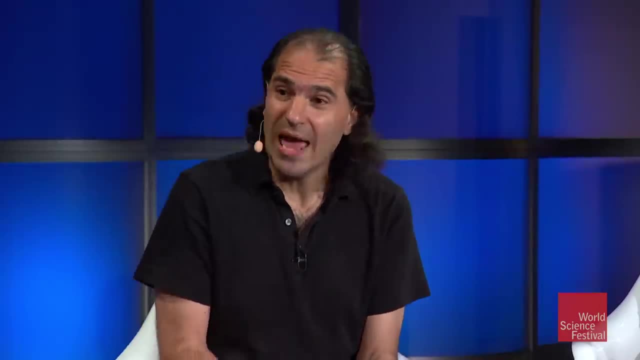 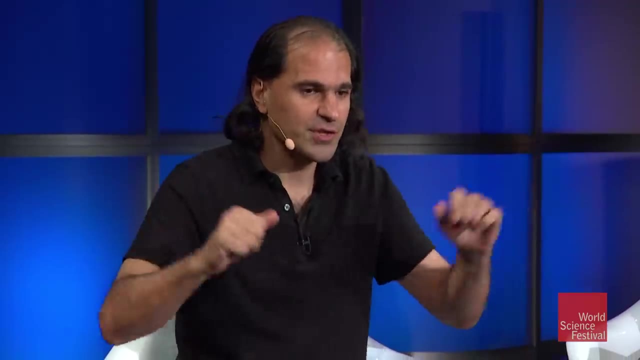 have to have very special properties and interact with each other in very special ways. You can have massless spin three, half particles. They have to be even more special, We might come to that later. and, as I said, the massless spin two. 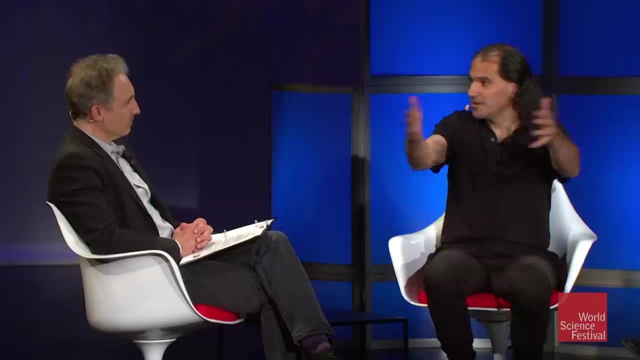 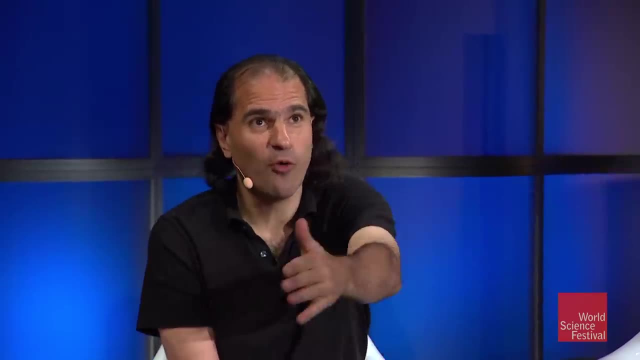 are associated with gravity. So that's it. There's this sort of tiny menu, and nature is making use of that menu, as far as we can tell. So we've seen of the set of possibilities before July 4th 2012,. 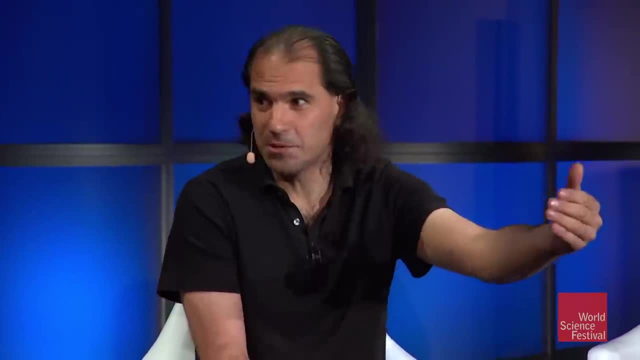 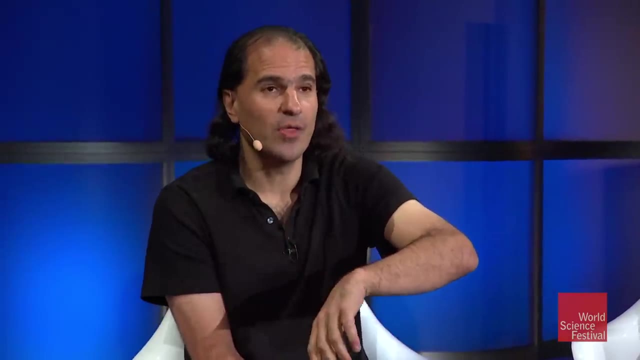 we had seen nature make use of some of these possibilities. It had used particles of spin, a half particles of spin one and, of course, the spin two associated with the gravity. One of the most exciting and important things about the Higgs is it's the first example. 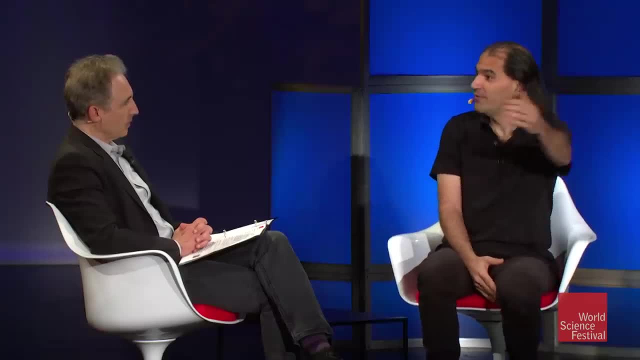 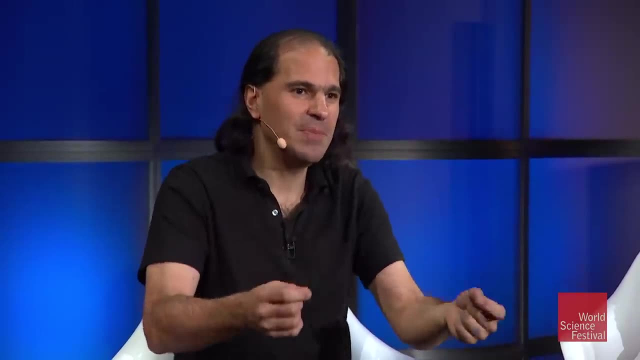 of an elementary particle that has no spin at all that we've ever seen. So that's been added to the, that's been added to the to the mix. But the reason why the Higgs had to be there is that something has to account. 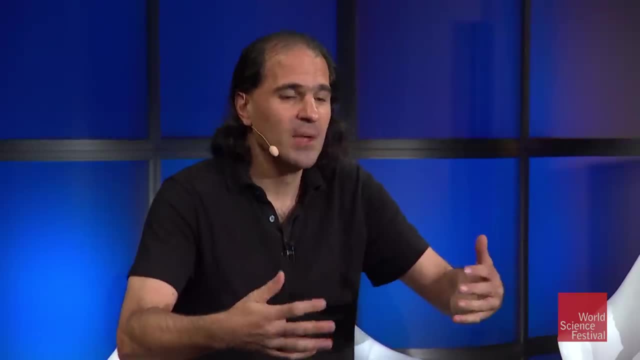 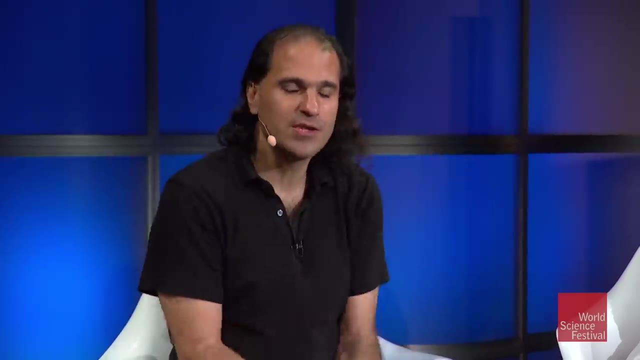 for this. two not equals to three business. Something has got to explain where mass comes from, not just, not merely to add this number, the actual mass of the particle, but to account for this extra stuff, this extra spin ways, that the extra ways. 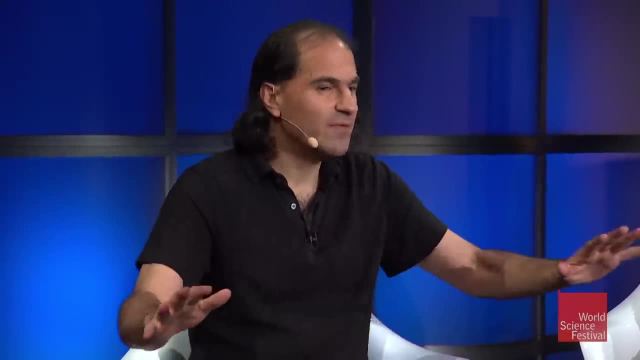 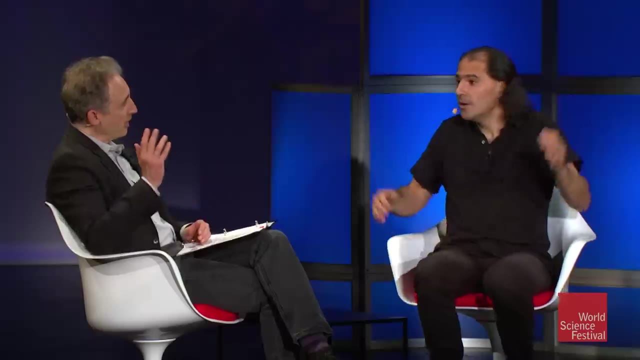 that things can spin when you give spinning particles a mass- And that's the entire story of the Higgs- is to account for the origin of these extra degrees of freedom. Now, that's quite a piece of cake, Yeah Right, Well, but it is all. 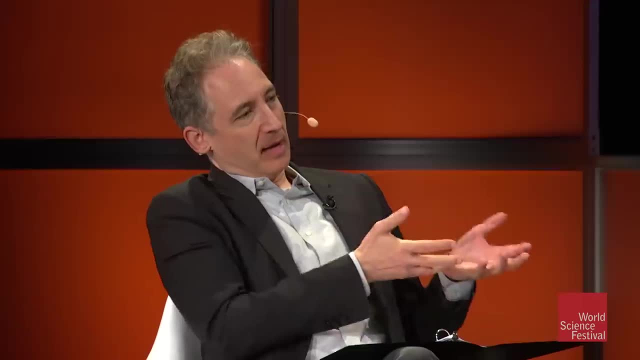 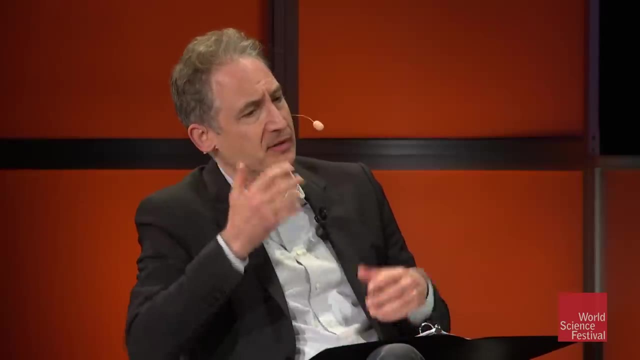 just about counting. It really is all just about this. two not equals to a three business. So with that as a preamble to the motivation that you had to have something fundamentally new added to the story, Monica, can you take us back to the 1960s? 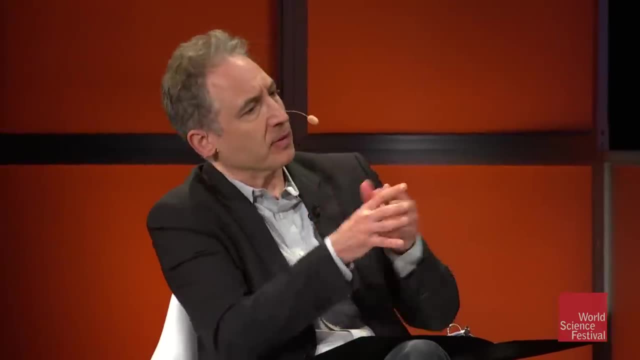 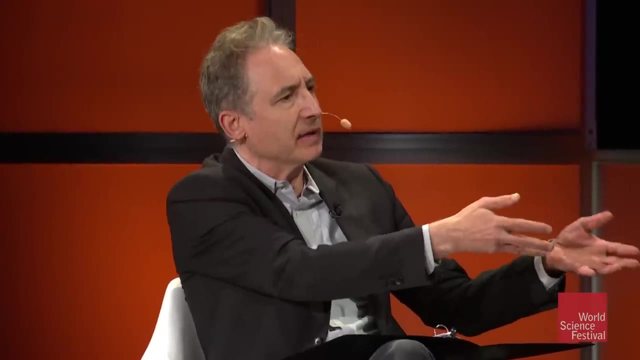 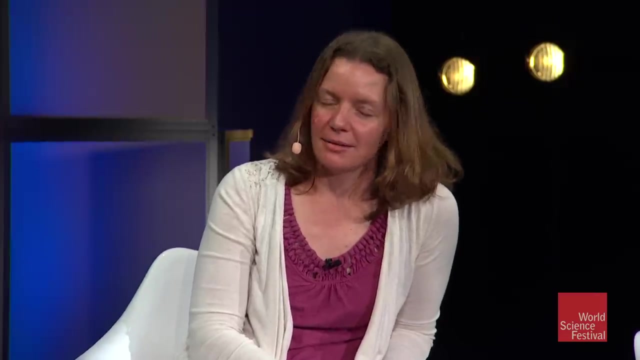 when Peter Higgs and others who shared the Nobel Prize with him as well, and what was the approach that Peter Higgs took to add this crucial, profound new ingredient that would fix up the two not equal to three puzzle that Neiman articulated Well, so Peter Higgs, 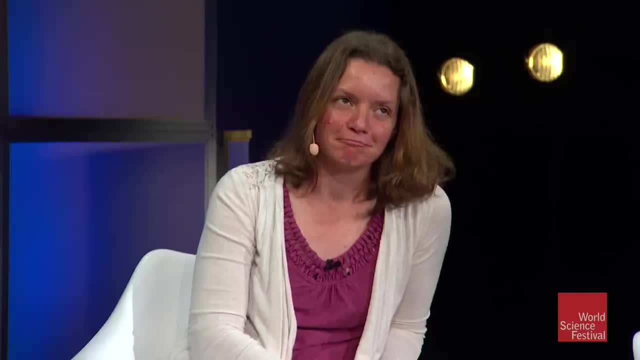 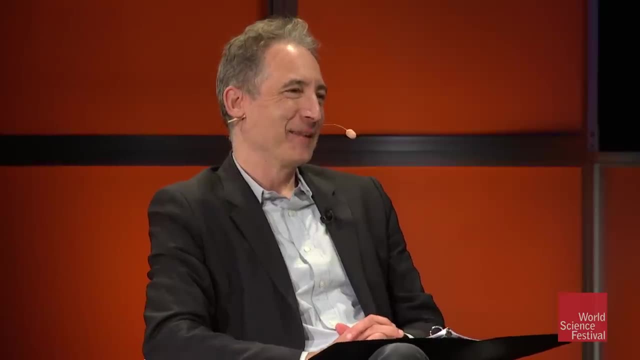 postulated the Higgs particle, And well, I wasn't there in the 60s so I can't really tell you a whole lot about exactly what was going on when that was, but it was a pretty revolutionary idea, You know. 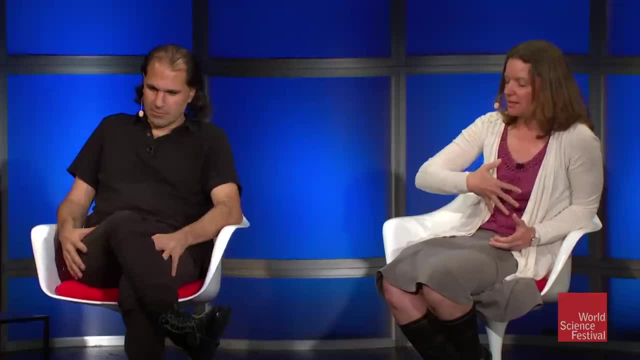 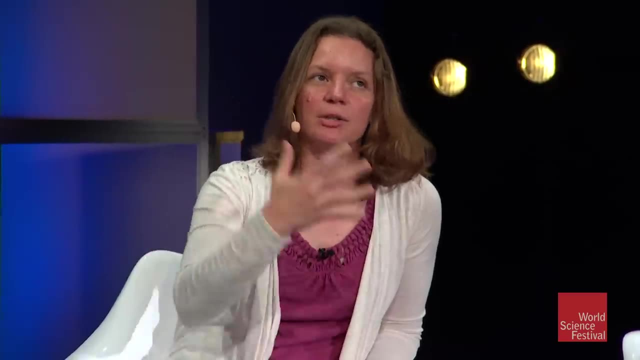 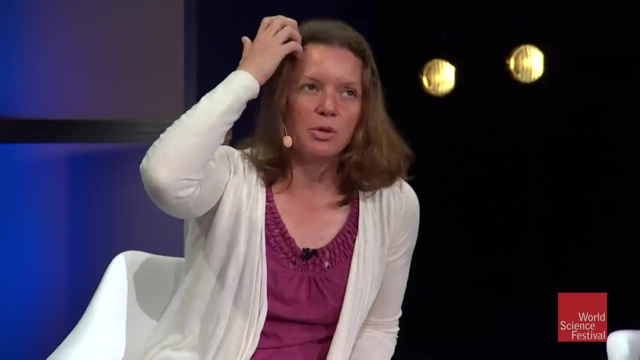 you had suddenly in the 60s this huge explosion of particles right Suddenly. I mean, the 60s was this period where it was like every week- essentially new particles were being discovered, and not maybe elementary particles like quarks and muons, but more like 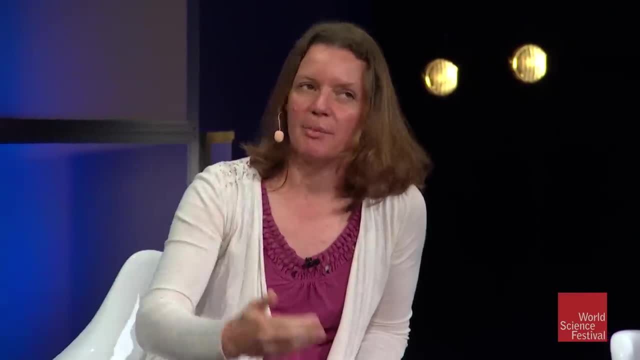 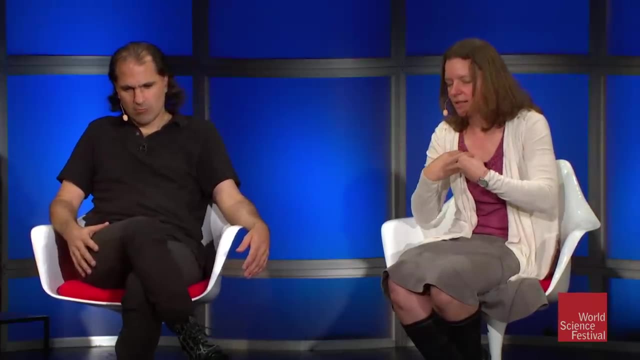 we were seeing mesons which are combinations of two, quarks or hadrons which are combinations of three, and you know every week, and so suddenly our kind of picture came up to a whole fleet of particles that didn't really seem to fit into anything. 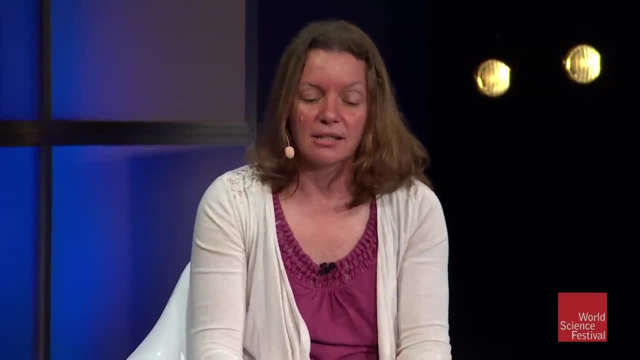 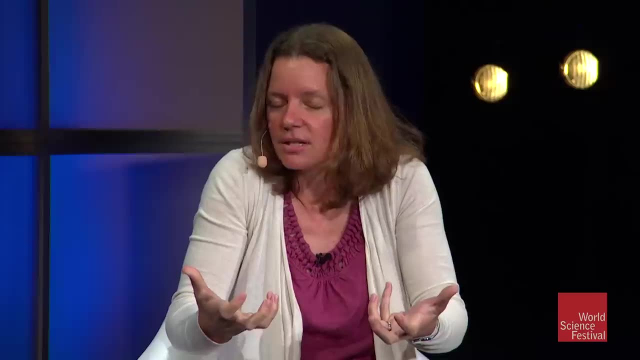 We didn't really need them Why. Why do we have, why, suddenly, all of these extra particles? And certainly you know how do they all fit together. You know what's the bigger picture. And then also, as you said, 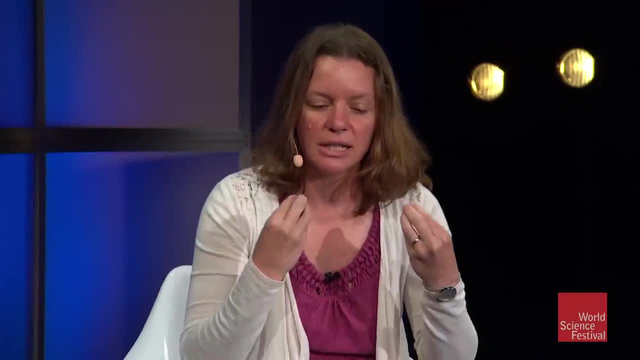 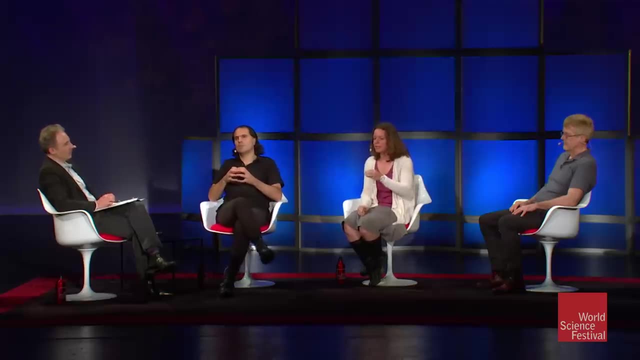 what gives them mass. And so Higgs was, you know part of that which was sort of to say, well, you know what's the mass of this particle, And that it could be something that we could then discover and detect. 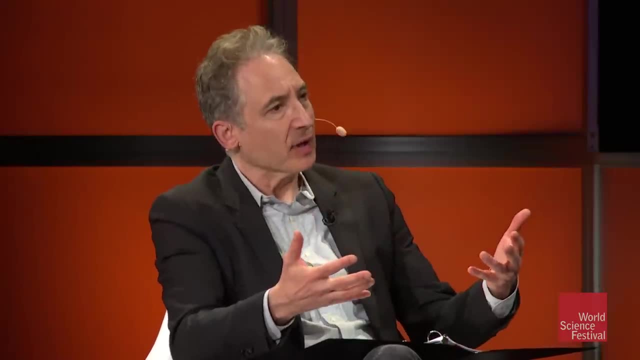 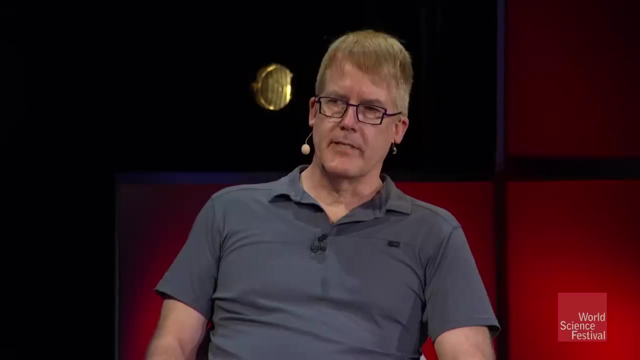 So, Joe, tell us about. so the Higgs particle is a key part of the story. Tell us also about the Higgs field, which ultimately is a key part of getting a sense of how particles acquire mass in this new idea. So you had mentioned. 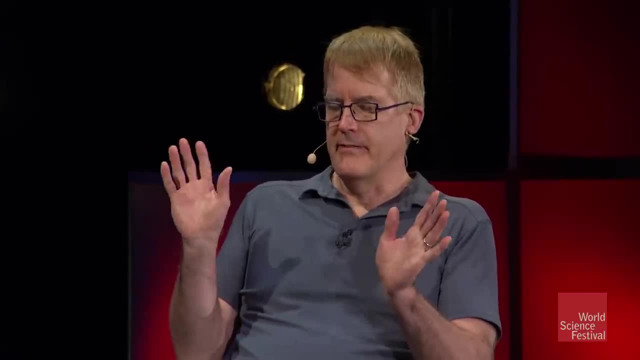 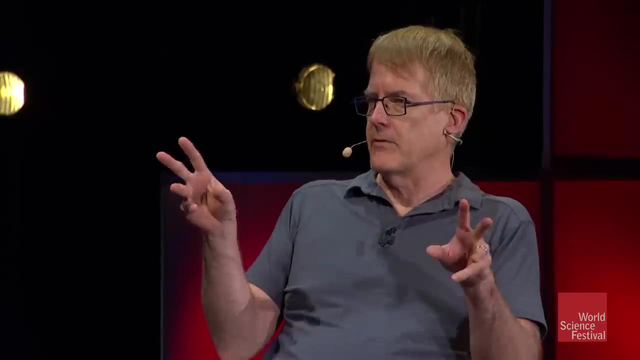 this phrase, cosmic molasses- which I think is as good a way of picturing it as anything else, but it's really a daring idea, right? So you have a cosmic molasses whose effect is to give the particles that we're made out of and other particles mass. 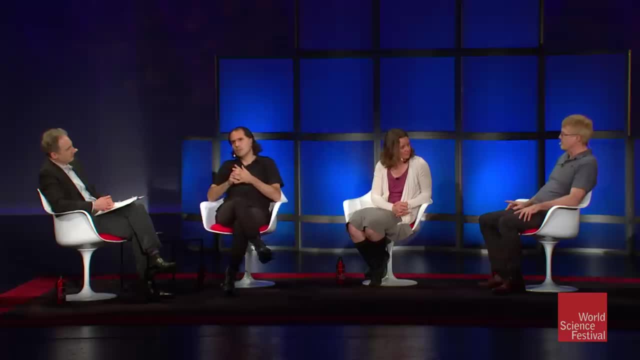 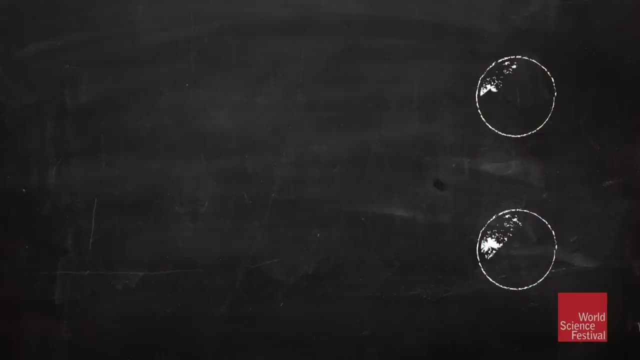 So that's a really daring idea and in fact, Higgs' original paper on this was rejected for publication. It was considered a little bit, a little too wild. I mean what we're seeing right here. in fact, we can probably play this again. 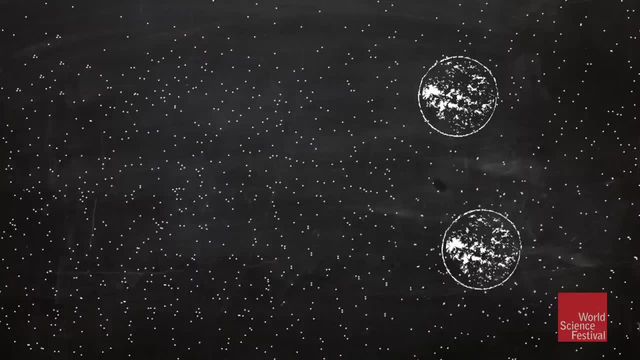 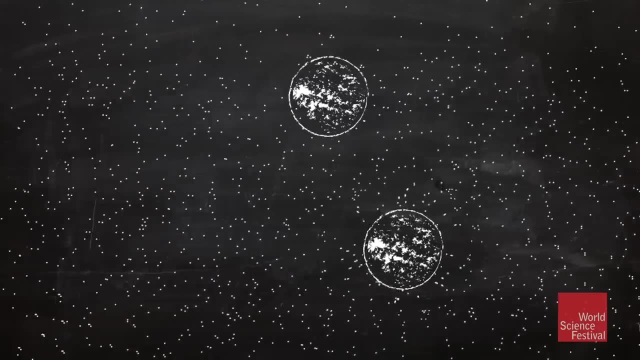 so these are the dots here are meant to be the molasses that you're referring to, and then one of these particles is meant to be masses, like the photon, I guess. and the bottom one is, if you're an electron and you're moving through the molasses, you'd like to move at the speed of light like a photon, and the only thing that stops you is the fact that there is a Higgs field everywhere and you can't avoid it. On the other hand, for the photon, the photon is not interacting. 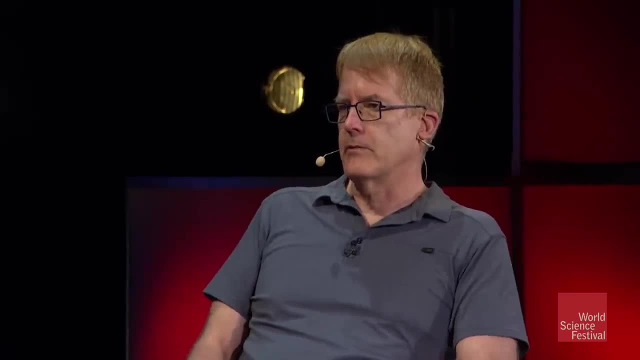 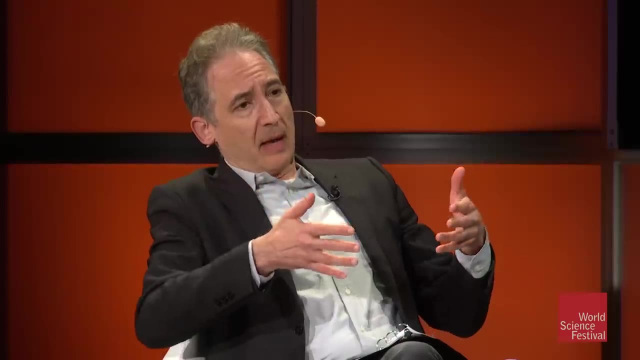 at least directly with the Higgs field, and so it just zips through the speed of light, and that's the difference between those particles. So for this crazy sounding idea to be true, we'd have to accept that empty space is not empty, and it's not. 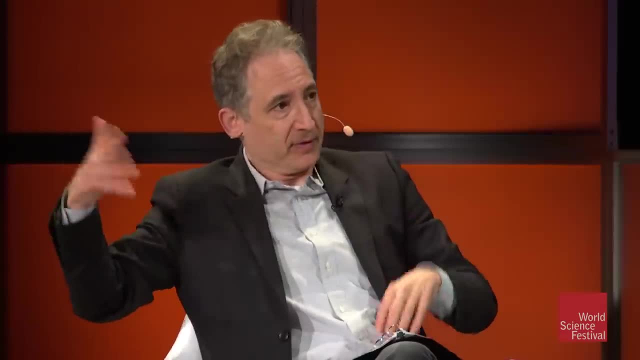 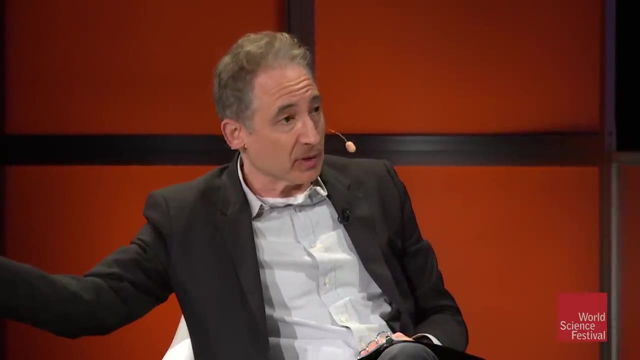 even a quantum mechanical notion of fluctuating fields that people may have heard of. This is just. there's actually a something there permeating all of space. Obviously it's invisible because we don't see it. It's tasteless, right Like when I move my hand. 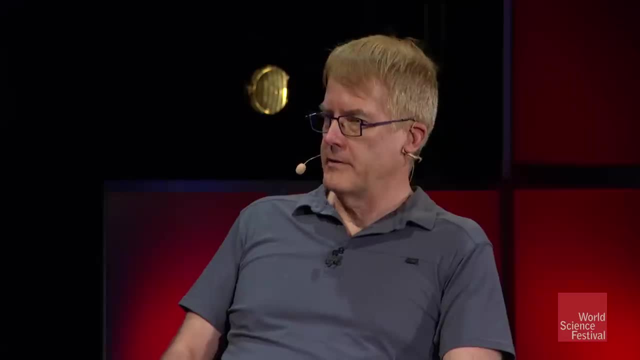 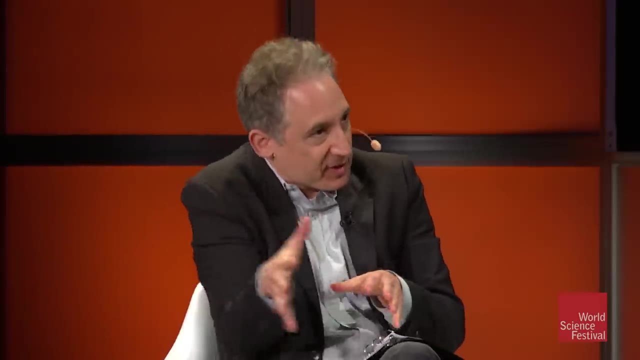 am I touching it? in some sense You are interacting with it all the time, Because part of the resistance I feel as I try to move my hand would be the electrons and the quarks, in some sense moving against this. molasses, Yeah, He puts forward. 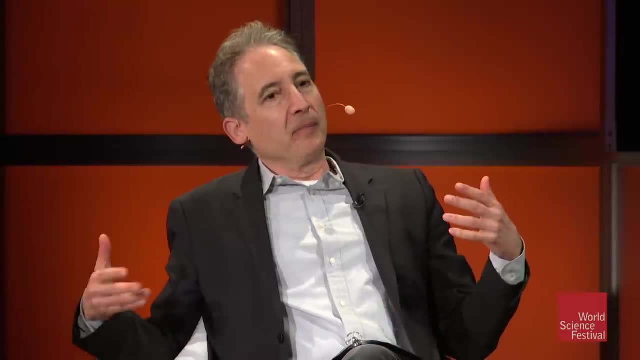 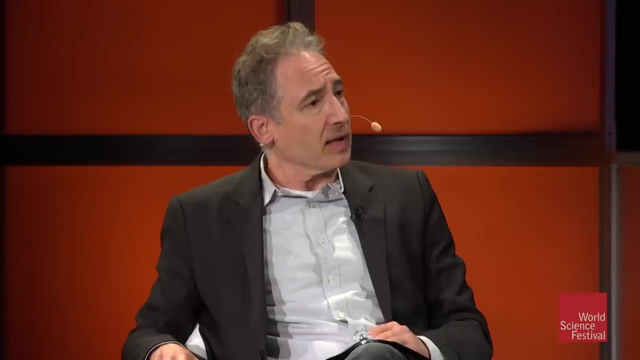 this paper and it gets, as you say, rejected. Yes, Now, many of us, if we have a paper rejected, we kind of back off. This is not what Higgs did, right, He actually went around and lectured on this and proselytized. 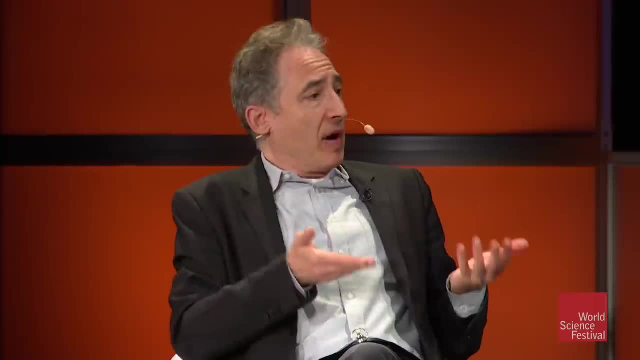 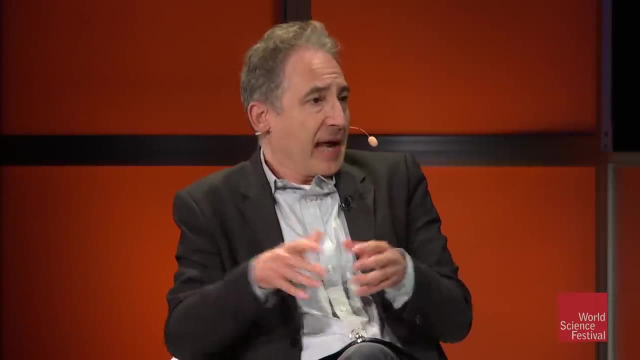 and discussed this and ultimately- I've said it before, but when I was a graduate student and first learned about these ideas, the class that I took, the professor taught it with such certainty that I had no idea that the Higgs was a hypothetical idea. There was a time. 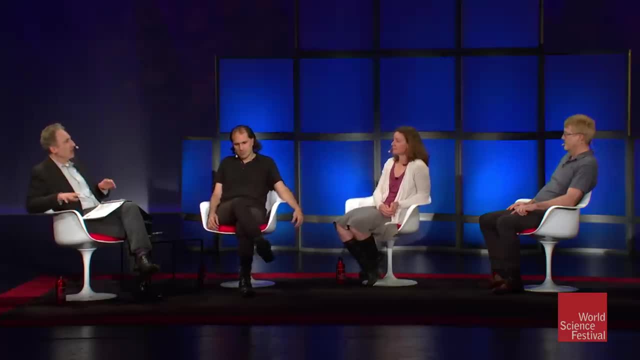 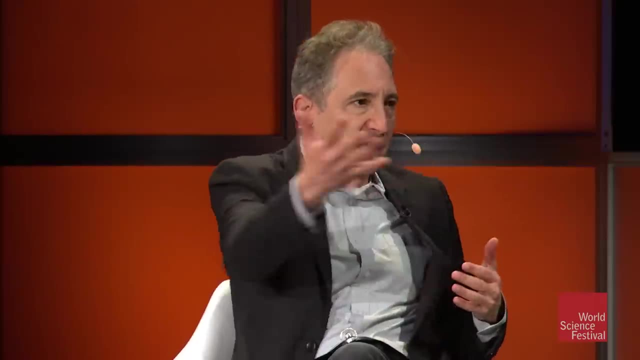 in our community by probably the mid 80s, early 90s. it was almost a foregone conclusion that this crazy mathematical idea from the 60s, which had now somehow permeated the consciousness of particle theorists around the world, that it was. it was right. 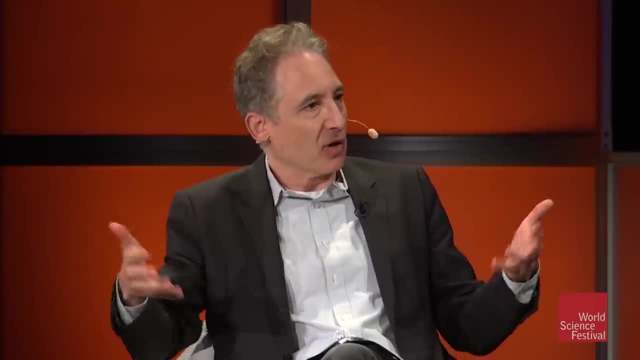 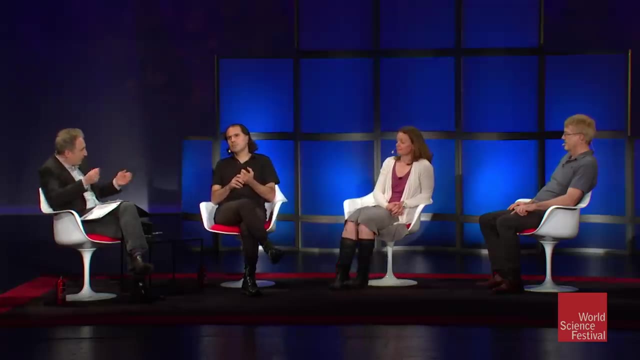 But still, you gotta, you gotta try to confirm it. So we start to look for it through these kinds of collisions. So, Monica, I guess you were there when the Higgs was actually happening. So what was it like and what exactly were you looking for? 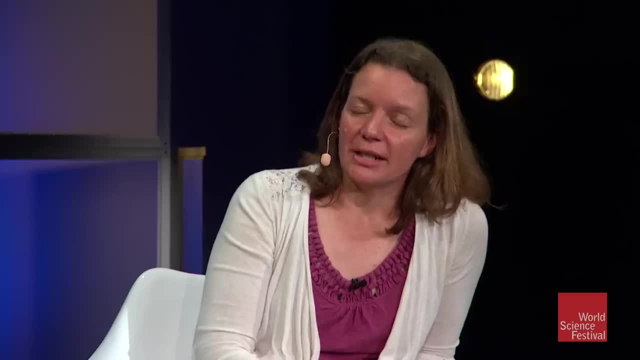 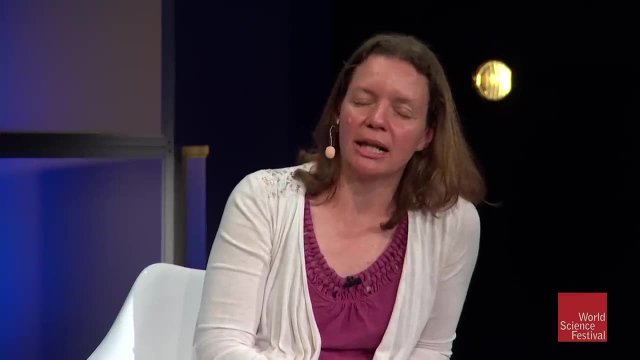 in those collisions. Well, in the beginning it was very intense. I mean, at first, when we first turned on the accelerator, we weren't really thinking about the Higgs. right then We were thinking about: my god, please let it work. You know, I mean 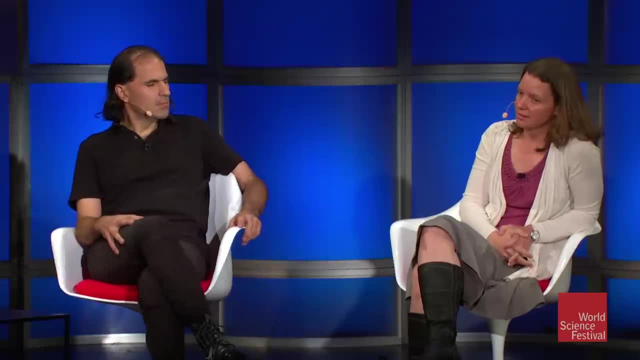 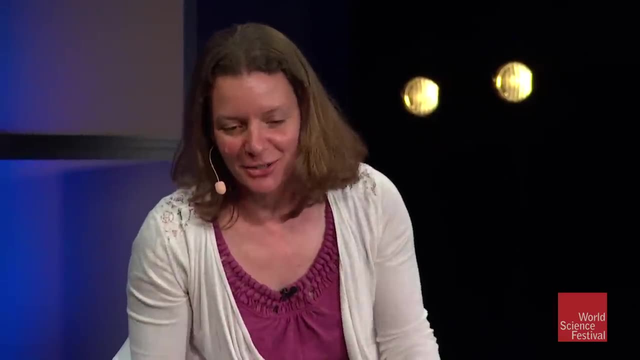 it was 15 years to build this detector. You're working on collaborations that are, you know, 3,000 people the days leading up to it. So in the beginning you were more concerned with the technical challenge and the Higgs was sort of a far off dream. 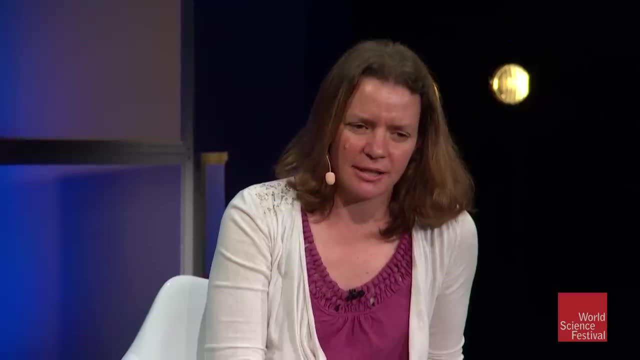 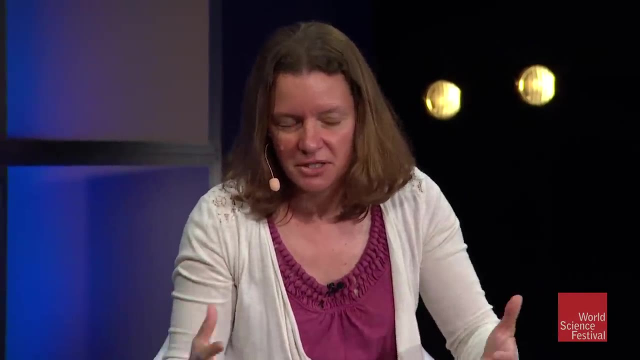 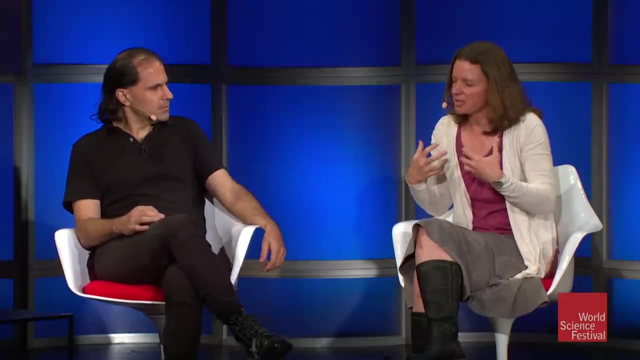 and we certainly, at that time when we first turned on the accelerator, and also, you know, just collecting up the data. you know, we, you've got a brand new detector. it's five stories tall. it involves, you know, millions of electronics channels that all need to be understood. 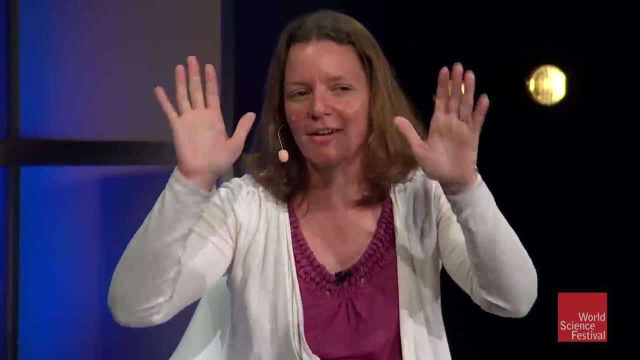 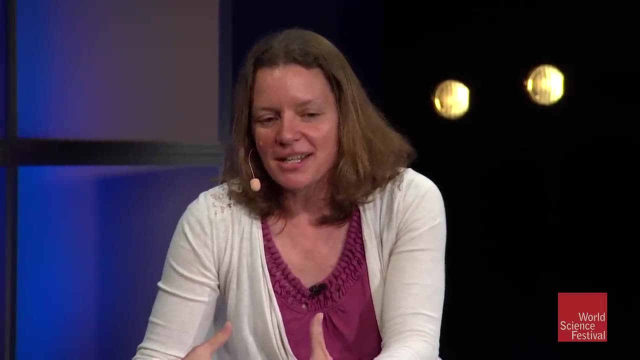 and calibrated. you know, give me, give me five years. you know I've got to discover, I've got to figure out this detector, we've got to collect enough data and I think for us, we were really amazed, maybe very happy with ourselves, at how fast the discovery. 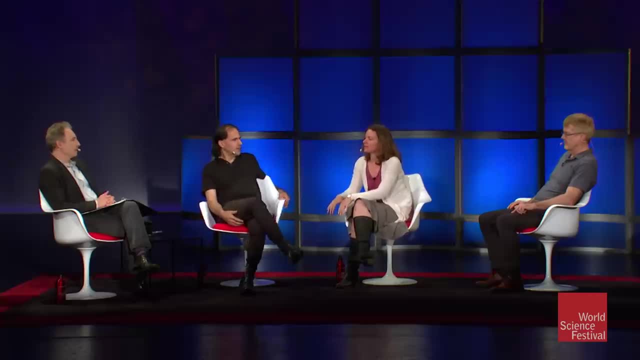 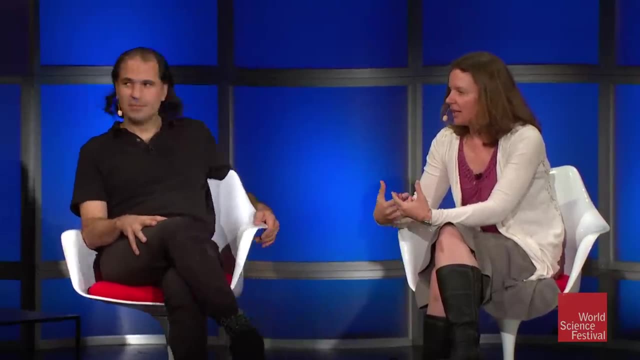 was made. actually, I mean, we were not. no one was predicting that we would have discovered the Higgs in 2012.. The Higgs ended up in a particularly nice spot. It did. it was it was there for. because of its mass, it has many. 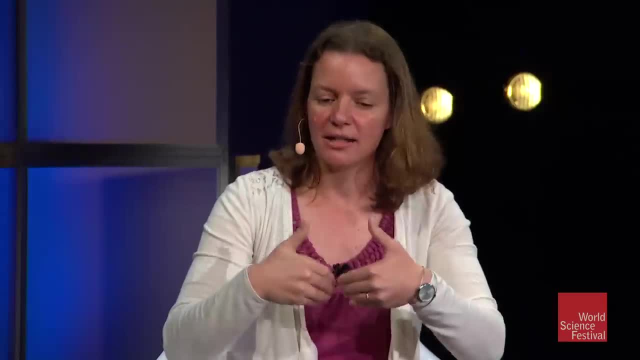 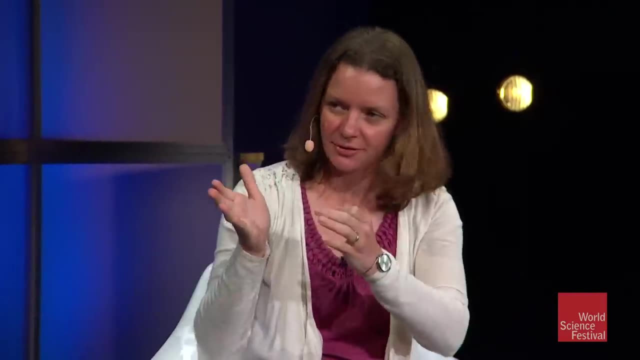 it has the maximal possible ways in which it can decay the Higgs. So how do you find it? So you smash these protons together. what happens? Smash these protons together, you get a lot of energy and in that energy you produce your Ferrari, which is your Higgs. 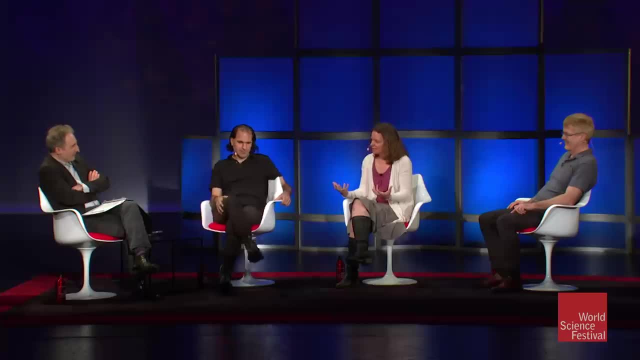 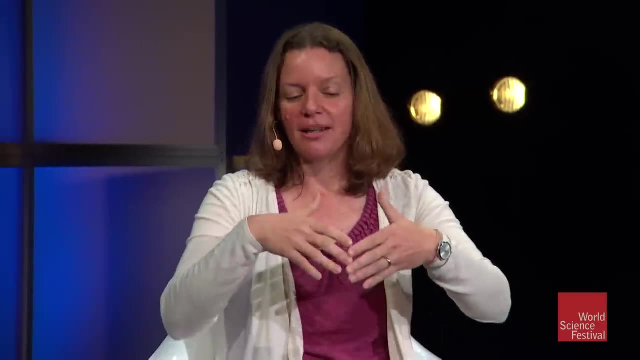 Yep, The Higgs then decays, It falls apart. It falls apart, Not exactly a Ferrari, Yeah well, Meh, You know. So the Higgs, the Higgs falls apart and you know to, it prefers to couple to mass, which means that it prefers to fall apart to the heaviest things. 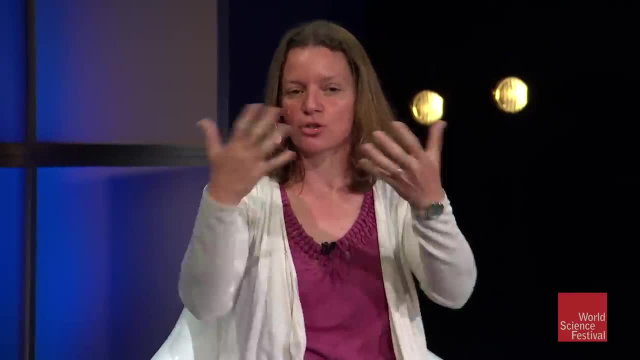 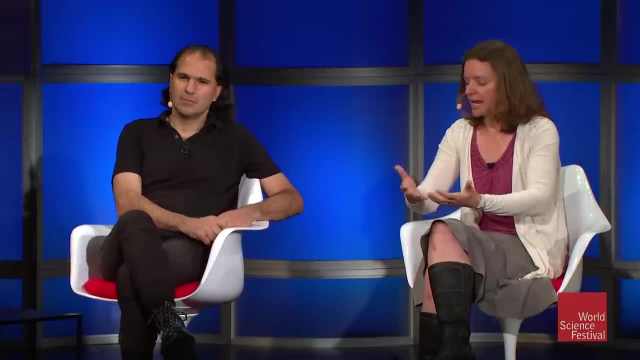 that it can Yep. So depending on the Higgs mass, if the Higgs is extremely massive, then it will prefer to fall apart to two top quarks. If it's at 125, which is where it's at- 125 times the mass of the proton, Exactly. 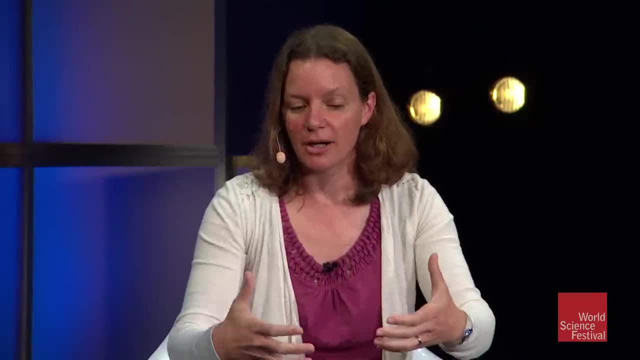 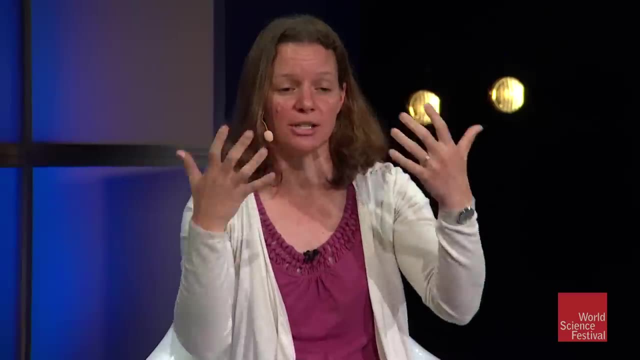 125 times the mass of the proton, then it falls apart. then it can fall apart in a whole bunch of things, which is, in essence, an experimental dream. Right, Because it means that it can fall apart to Z bosons and you can look for for the decay. 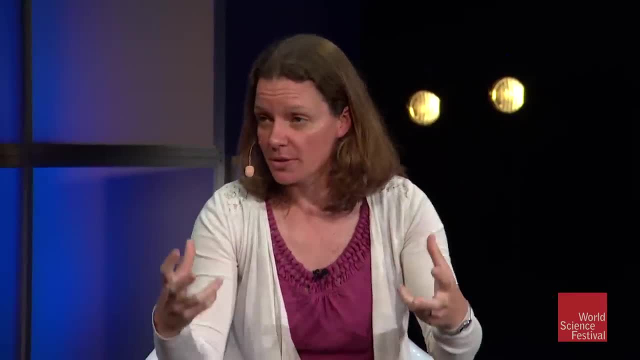 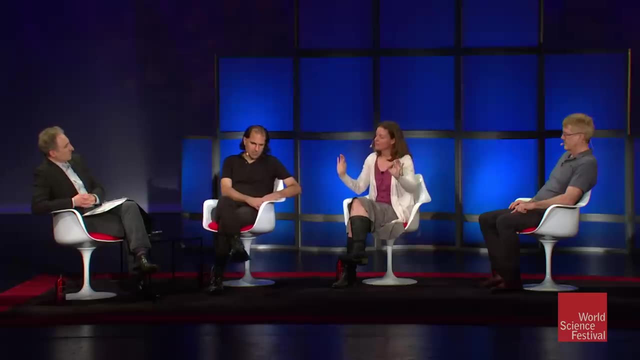 of the two Z's. It can fall apart to two photons, It can fall apart to two W bosons, and so you have a variety of different ways that, experimentally, you can test, and that, for us, was really key because it allowed us to be able to. 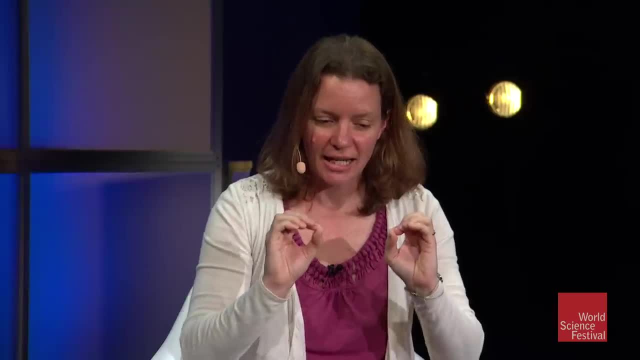 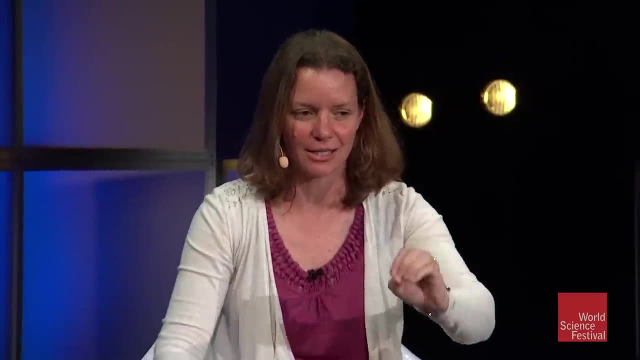 to say, okay, I looked into. I looked at the decay of the Higgs to two Z's. I see exactly where it should be. I looked at the decay of Higgs to two W's. I see exactly where it should be, because, from an experimental perspective, we never actually. 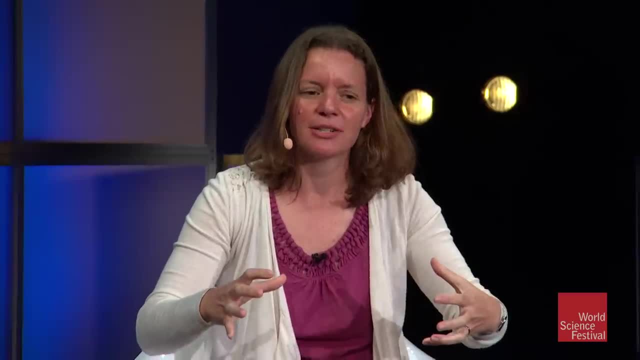 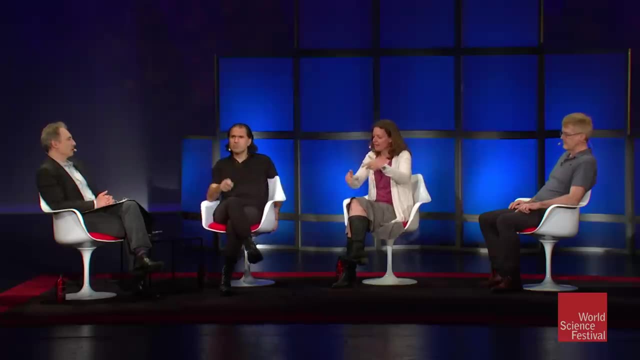 measured the Higgs Right. We never measured the Higgs, so all we knew at that time was we had measured something new, whether or not it was the actual Higgs boson. we then had to compare the rate of decay to two Z's. the rate of decay. 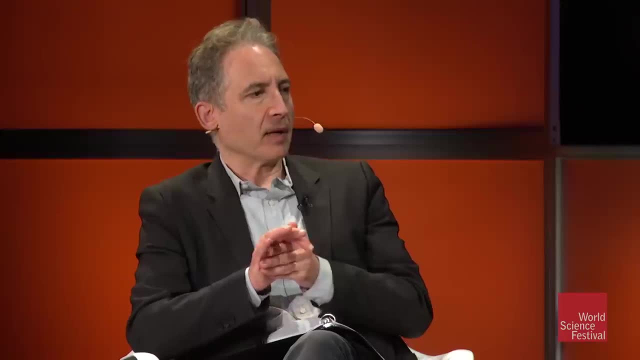 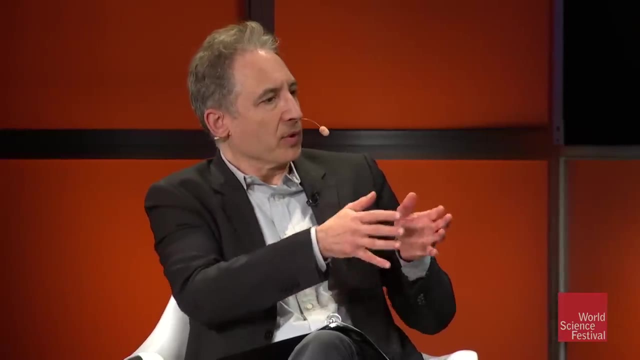 to two W's, of which the theory, once you know its mass is predicted, Makes a statement about it. Yeah, exactly. So if you, if there's an announcement on like July 4th, you're pretty certain that you had it. is it months before? is it six months before? 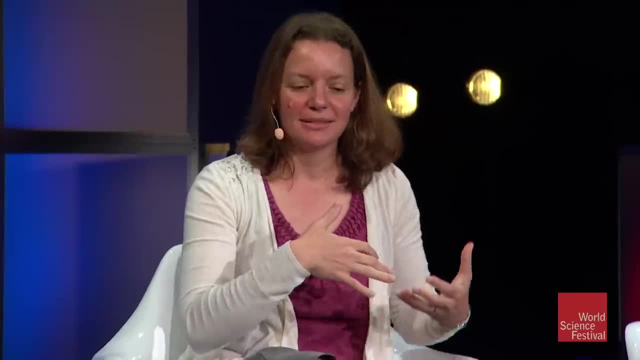 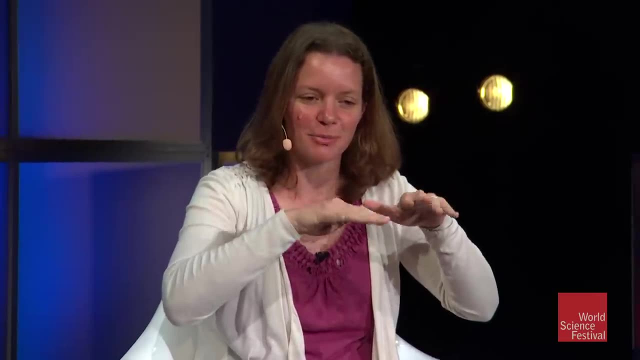 or the day before. I mean you, I mean statistics- is such that you know we were collecting data and if you, if you see some sort of statistical signal, you should expect that as more and more data. you know the size of the, the size of your, you know. 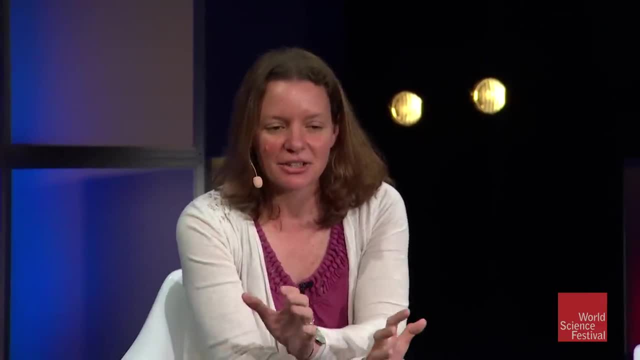 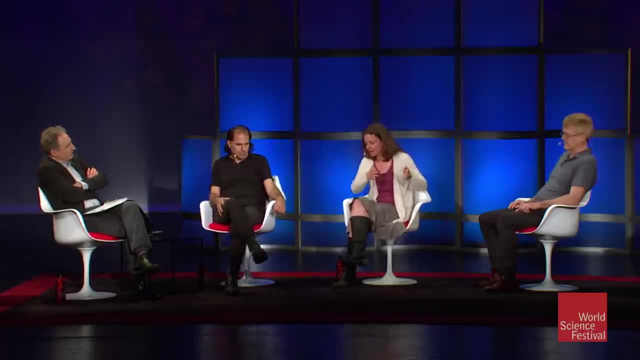 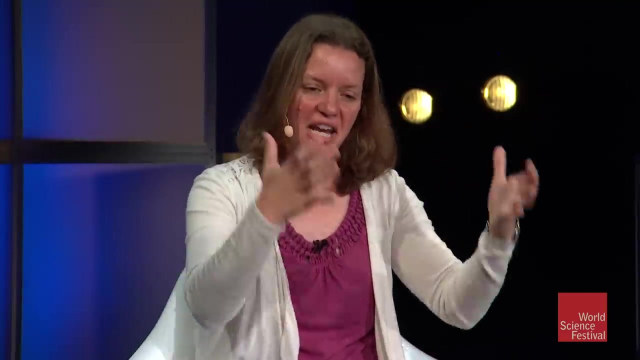 Higgs peak, let's say, starts growing and growing and growing, Yep, But that's not actually usually how we analyze data. we usually get it when we're talking continuously over the day. you know, we have to calibrate our detector and we we tend to data, just kind of. 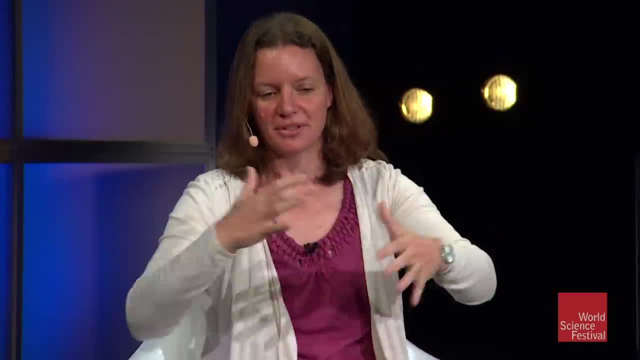 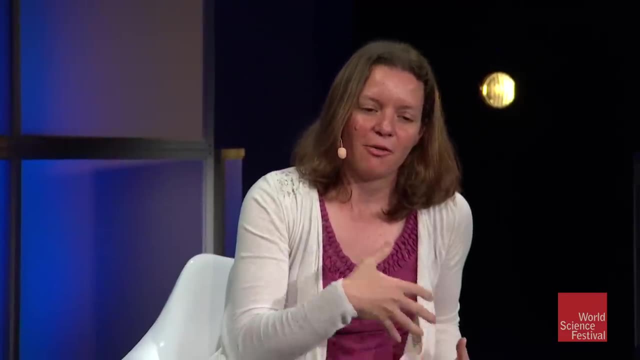 comes to us in chunks, we'll do this calibration. try to understand it. okay, that's chunk A, we'll do this calibration. that's kind of chunk B. so we're kind of looking at it kind of in chunks at a time and because a false discovery is. 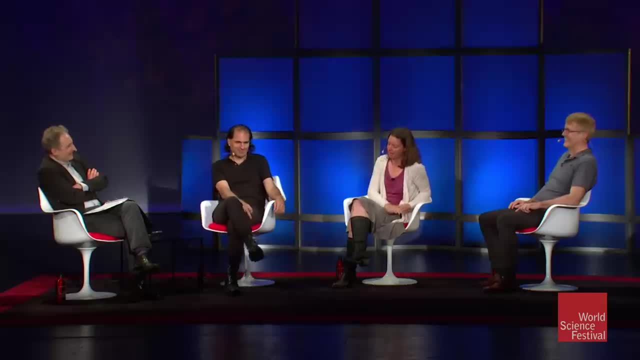 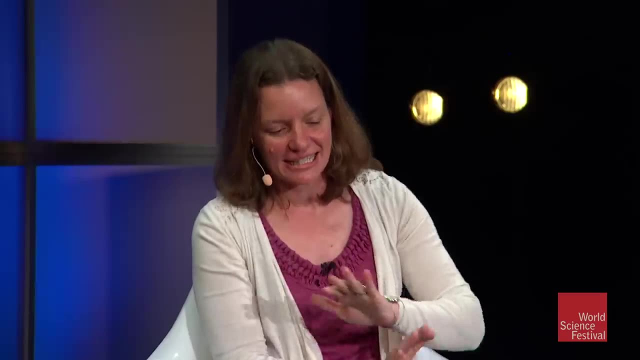 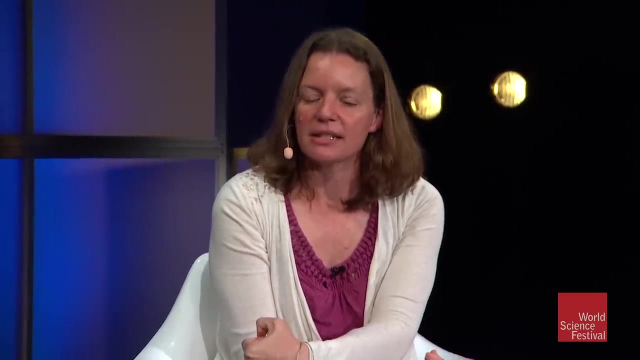 worse than death. let's- let's put it that way- death. people won't keep making fun of you forever. yeah, I know so. a false discovery is: yeah, right, yeah, so you're going to do anything that you can, anything. what we, we oftentimes do, is we. 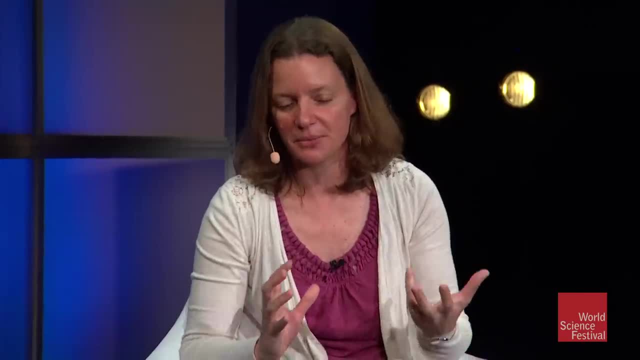 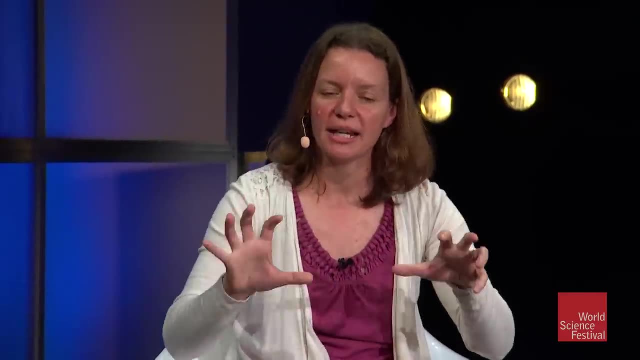 we blind the data from ourselves, right, so we will. we will do the entire analysis chain where we have and we can do blinding in a variety of different. there's several strategies, but what it means is either we- we make sure that everything is correct, our calibrations- 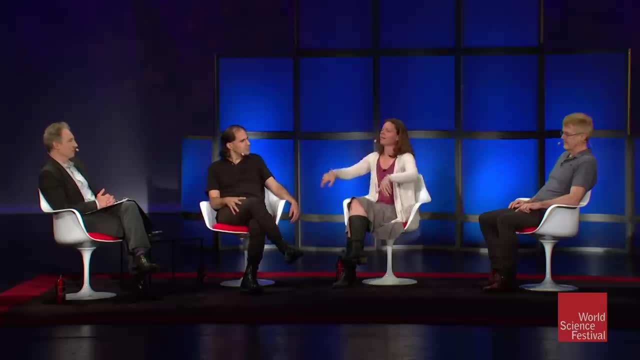 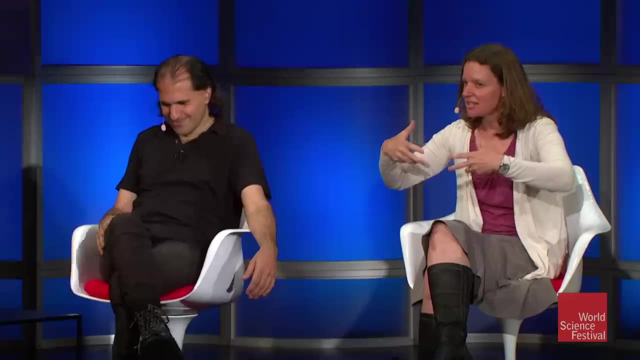 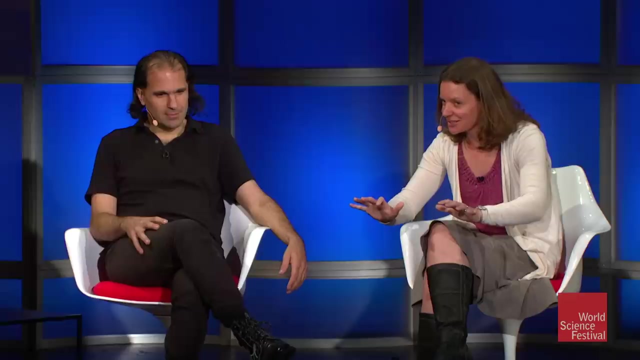 our analysis, selection, so forth and so on. and then we unblind. and it's extremely stressful that moment when you get the. you get it's a collaboration of 3,000 people. and then they agree to unblind and you, you know someone hits the. you got a computer program. 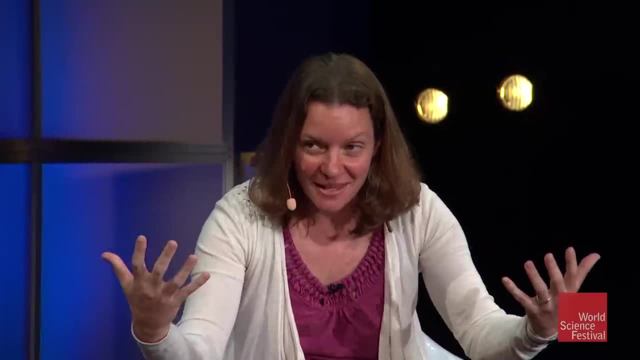 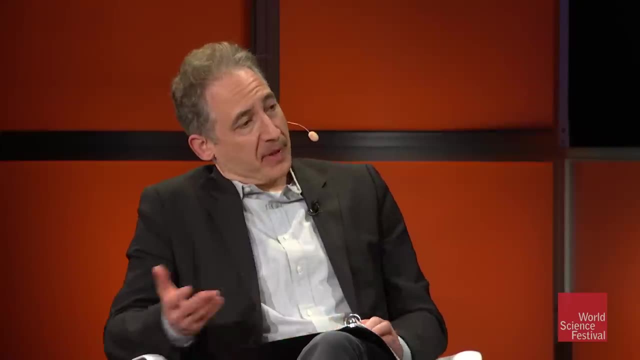 someone starts it, you know you're watching the data being processed. watching it being processed, you get the plots, is it there? is it not semi instantaneous that we- but that's sort of an amazing moment, and now that you have the Higgs and we can now turn, 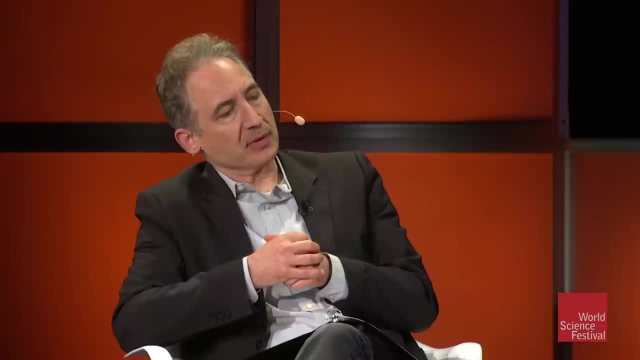 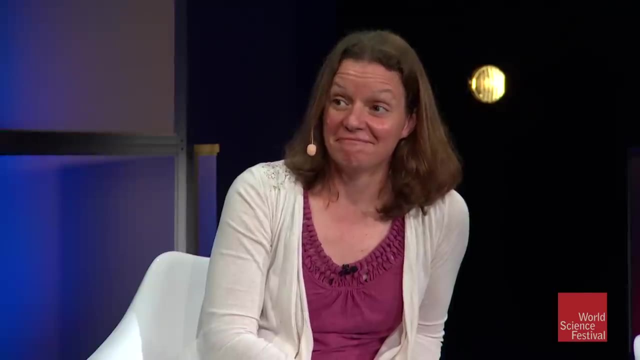 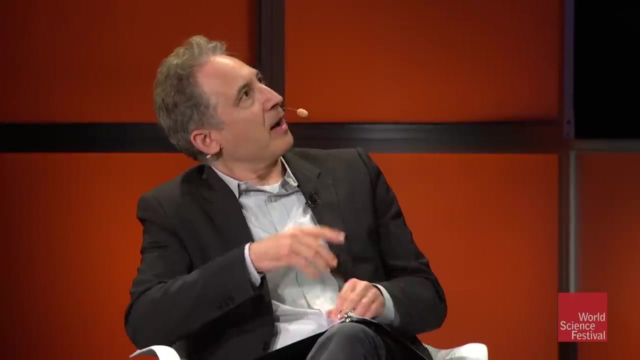 to the question of like going beyond this major discovery. you were actually at the World Science Festival about I think it was 10 years ago, having a conversation prior to the discovery of the Higgs, and I thought I'd just show you a little little clip from that. 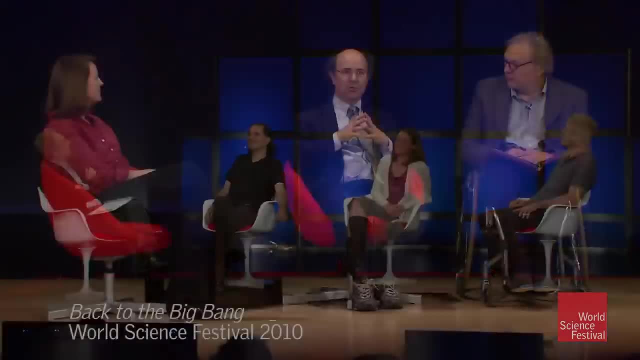 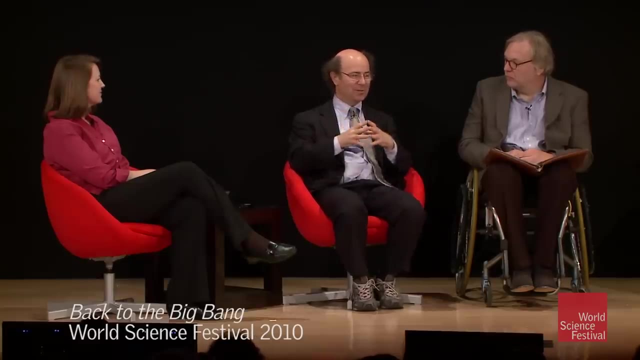 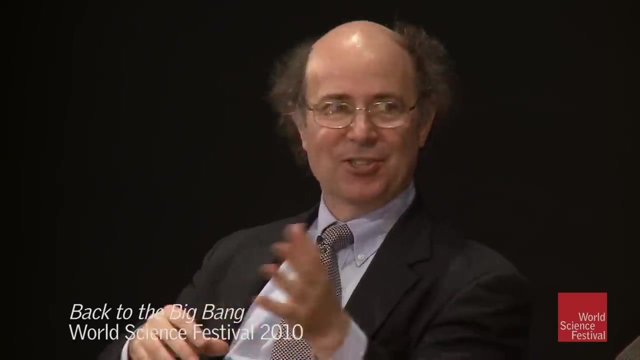 if you don't mind, so can you just run that that little? the worst scenario as far as I'm concerned would be that the LHC sort of completes the standard model and doesn't do anything more, so in the standard model as it stands. we need this cosmic molasses. 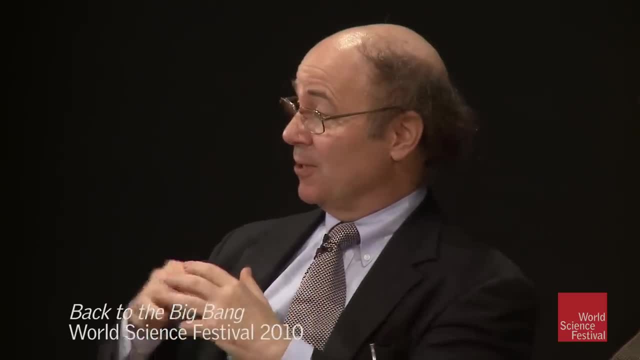 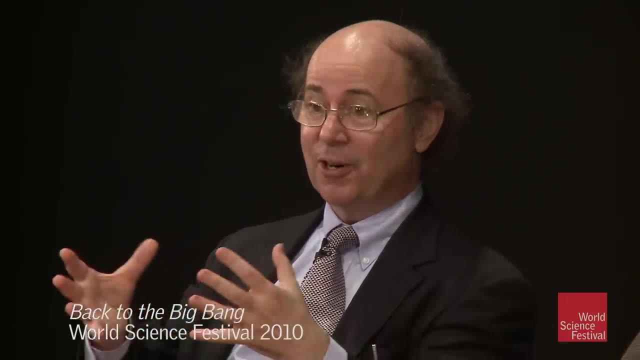 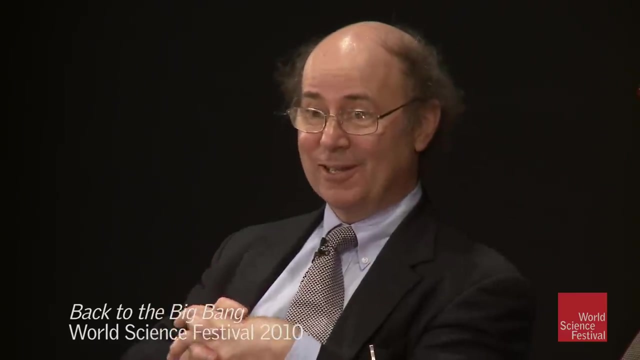 that was mentioned. we don't know what it's made out of. the simplest idea is that it's made out of one new particle, this so-called Higgs particle, and that could be true. and then you've you've accounted for the missing ingredient of the standard model. 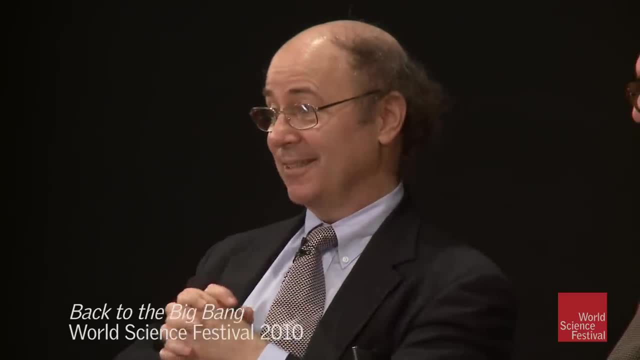 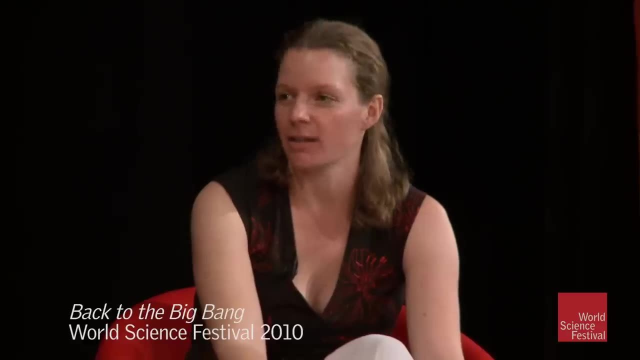 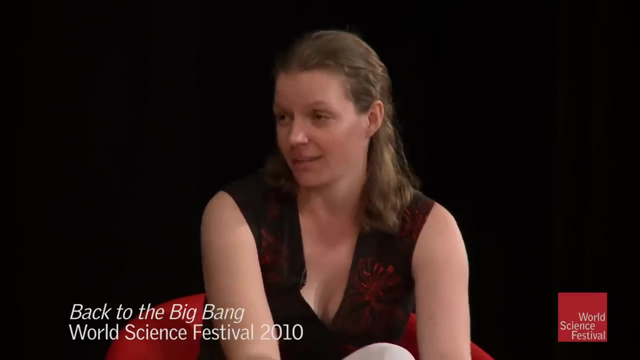 and that would be it, and that would be horrifying, Monica. well, I think there's there's pretty much two scenarios where I would end up at McDonald's, and that is that if we discover the Higgs, and the Higgs only, which is Frank's worst case scenario. 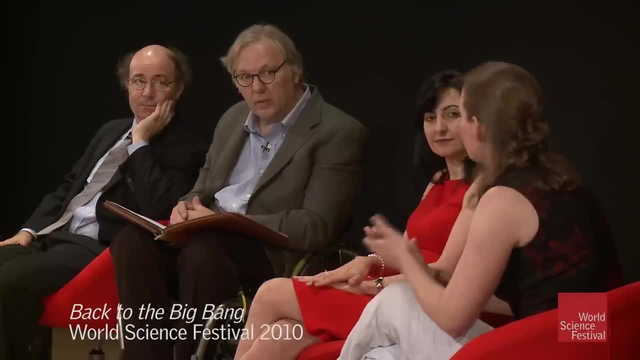 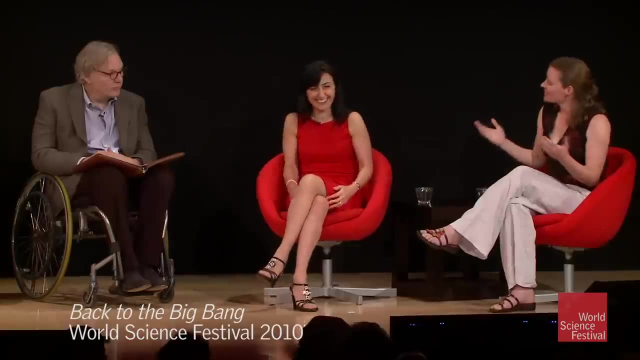 and also mine so far. every collider experiment we have is really: we have predicted this and we measure it. the standard model predicts this and we've measured it, the standard model, and so success is our curse. yeah, yeah, success is our curse, exactly. and so I think from 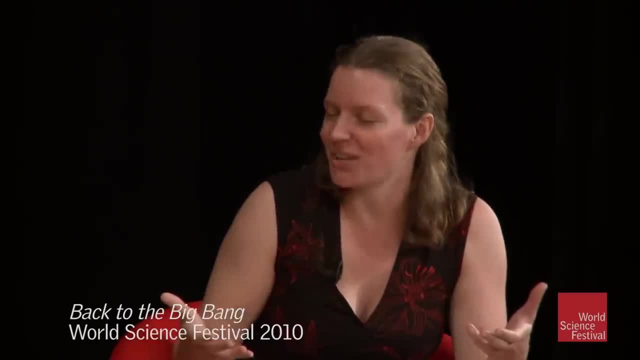 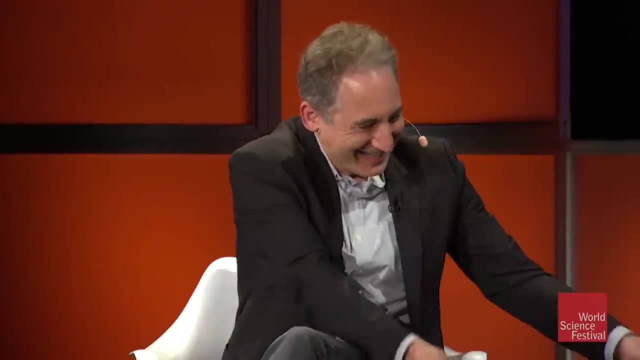 the experimental perspective. we're really sick of the standard model. so to just to just continue to measure the standard model, which would be a Higgs and Higgs only scenario, would be frustrating. so so you said I so at the beginning, I guess I'm gonna have to go. 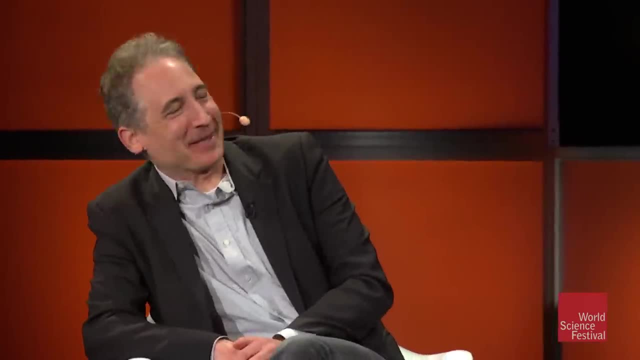 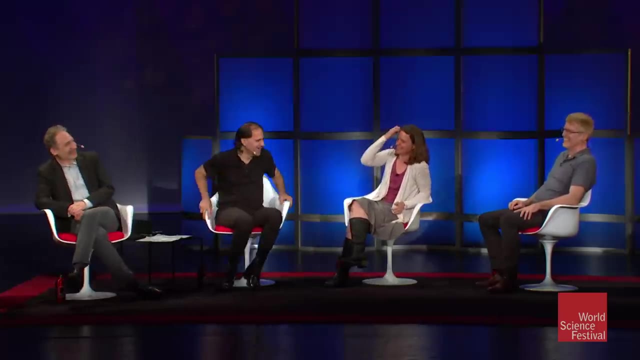 to start working at McDonald's. that's right. so at the beginning of the clip you said at McDonald's, you're not at McDonald's, I'm not at McDonald's. so I'm assuming that in the second part of our discussion, yeah, exactly so. so let's. 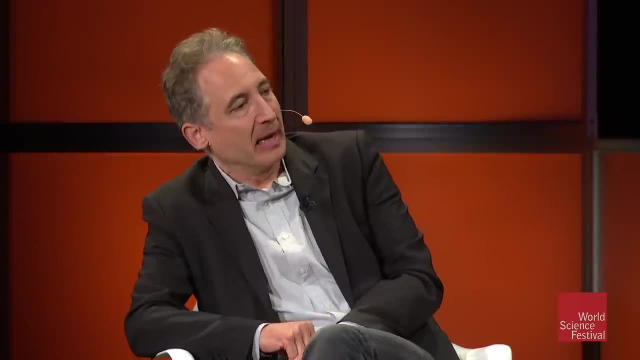 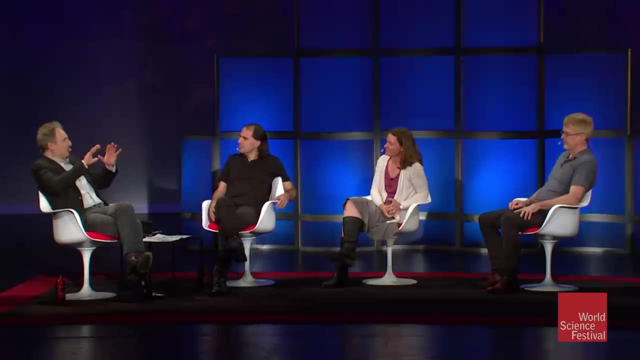 let's think about how we go beyond and how we've tried to go beyond these ideas and and to sort of start that discussion. you know, Nima, you pointed out that the standard model has a sense of both simplicity and complexity, sort of, depending on how you look at it. 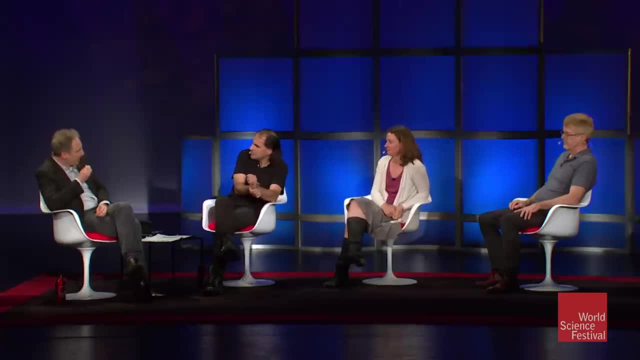 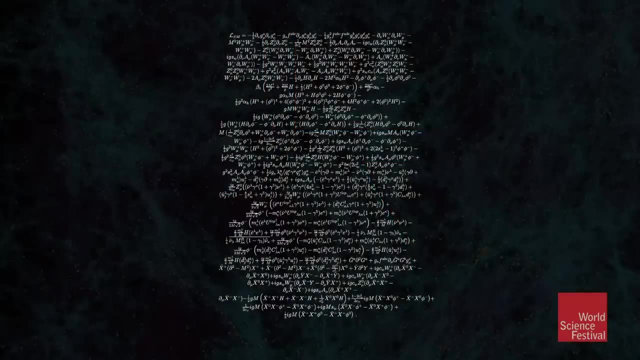 and we were looking at it just graphically, with the particles and the equations underlying the standard model of particle physics, and you just like write them all out. this is what the equation looks like, yeah, which certainly has a sense of complexity associated with it. it's sort of hard to imagine. 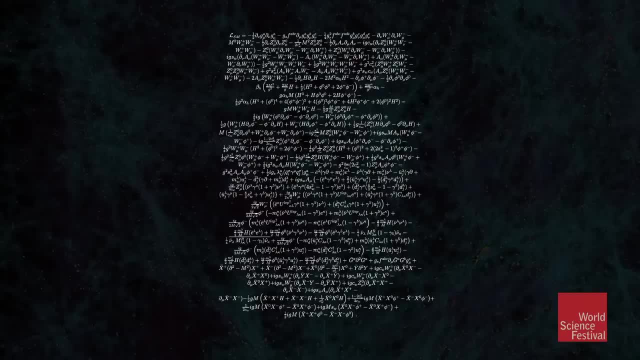 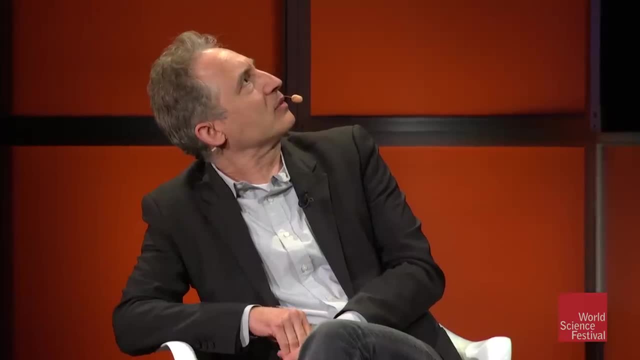 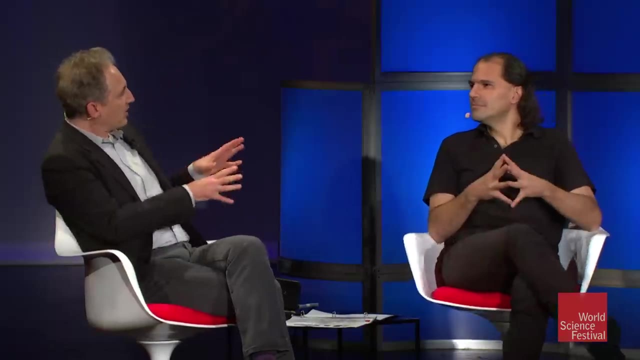 that you know. after you know a certain number of days and nights, the Lord simply said: let there be the standard model Lagrangian, you know. so now you know, I think that you know, that you know. you can also say: I mean, this is misleading, because this is the most. 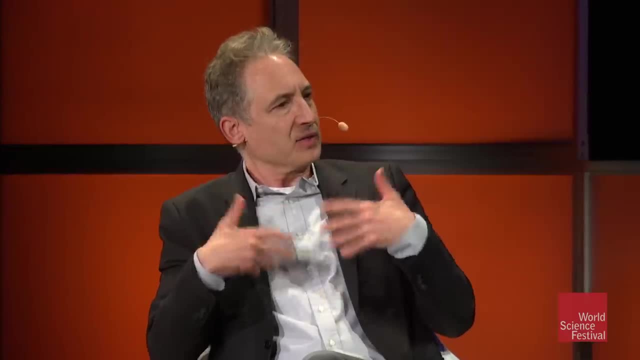 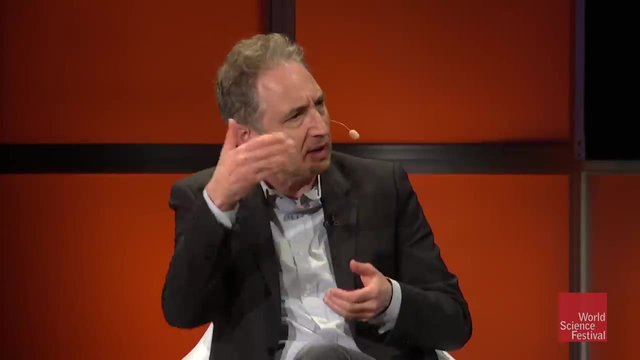 naive way of writing out the equations, and what we have found over the course of many decades is that symmetry is sort of an important way of being able to repackage our understanding in a way that really simplifies and allows us to shine a light going forward. 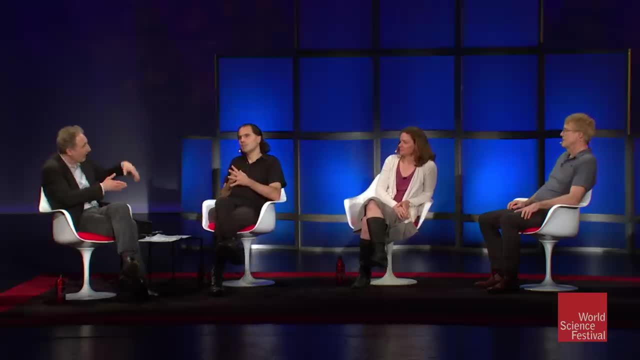 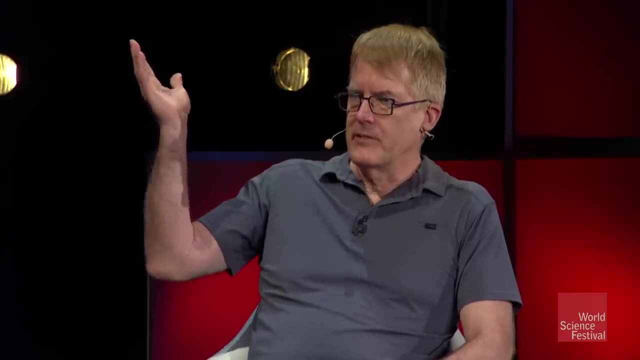 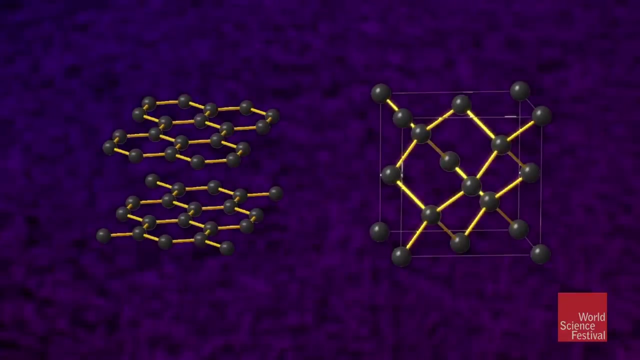 so, Joe, can you say a little bit about symmetry? sure, and and and how? for instance, it helps us to understand this better if snowflakes have interesting symmetries. a diamond is a good example of symmetry in physics. you know what's the difference between the diamond? 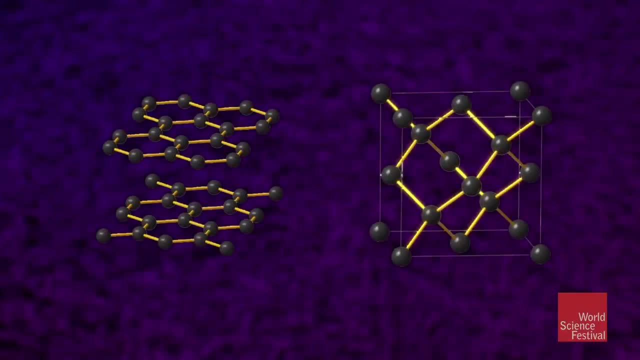 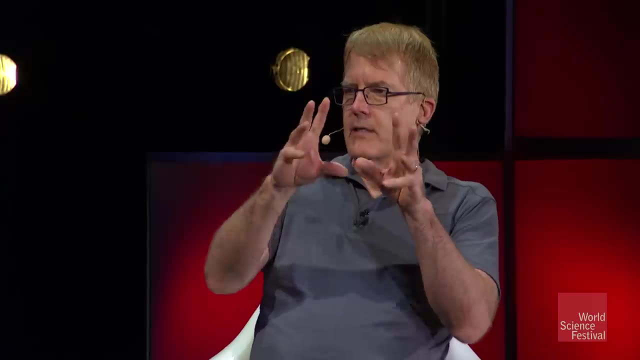 and the graphite and the pencil. they're both made out of carbon, but the difference is that diamond is in a beautiful crystal lattice- symmetry, and that's what gives diamonds its special properties and so symmetry in the physics world. it controls the physics properties of the things that you're talking about. 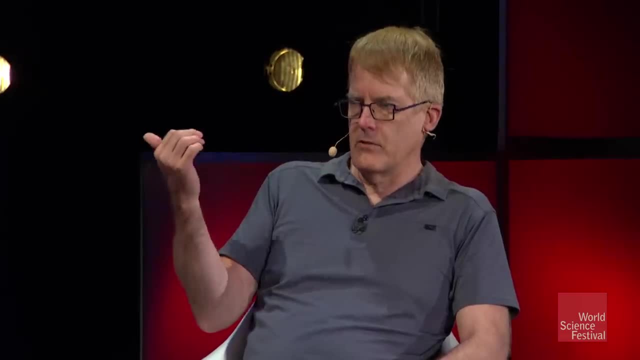 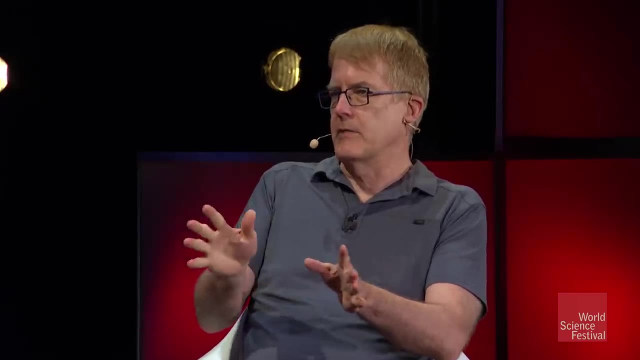 so this happens in the subatomic world as well, and we're actually talking about principles that control how the standard model works and actually make it much simpler than it could otherwise have been, and that's why those complicated equations can actually be expressed almost in words, in terms of a few 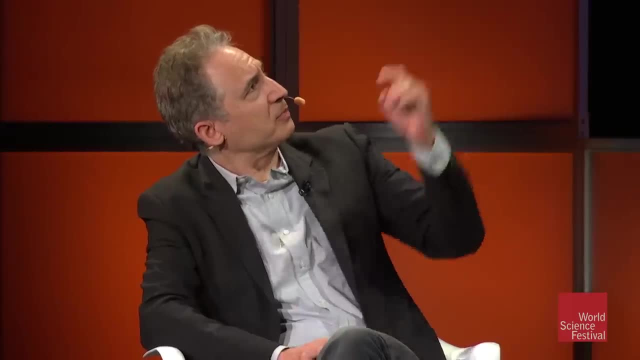 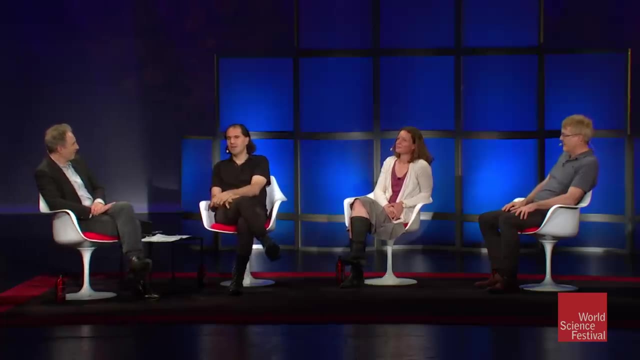 symmetry principles. in fact, you can even use that symmetry to put those equations on a coffee, exactly as has been done, and I think it's worth. it's worth really stressing that these it's kind of an unusual sort of symmetry that we're talking. there's some important differences. 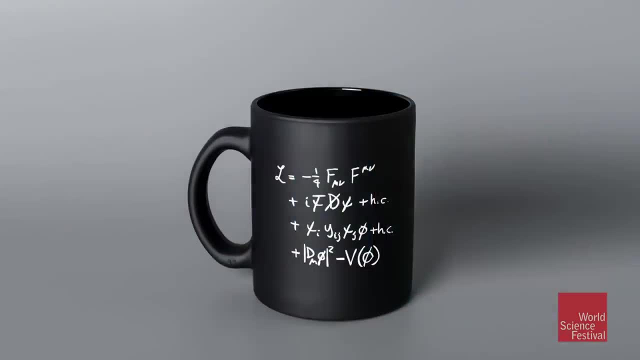 in terms of how we get into it. but but this very simplicity and the fact that there's a certain kind of symmetry that is useful for theorists to describe this, physics has everything to do with this. two not equal to three business. it has absolutely everything to do. 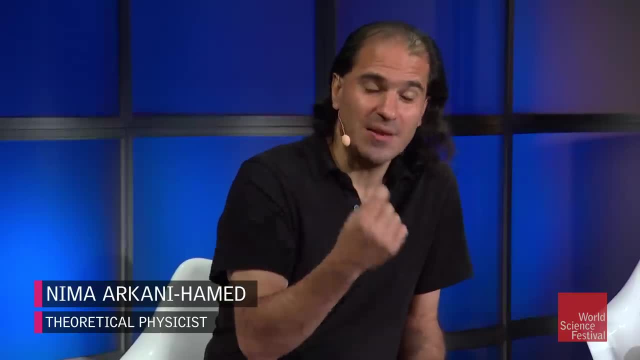 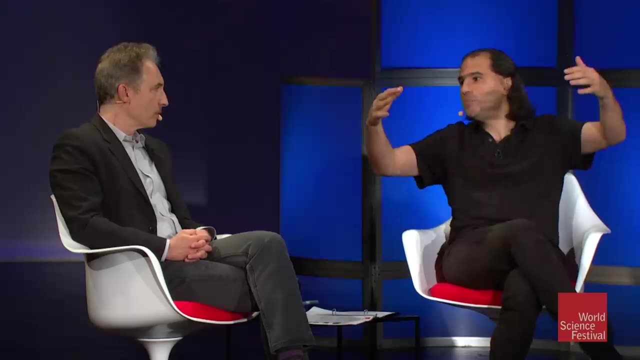 with the fact that we're only allowed this tiny menu of elementary particles when they're massless, and that mass is a big is a big perturbation. so trying to describe massless particles, which we think we should be doing in some approximation, is going to force. 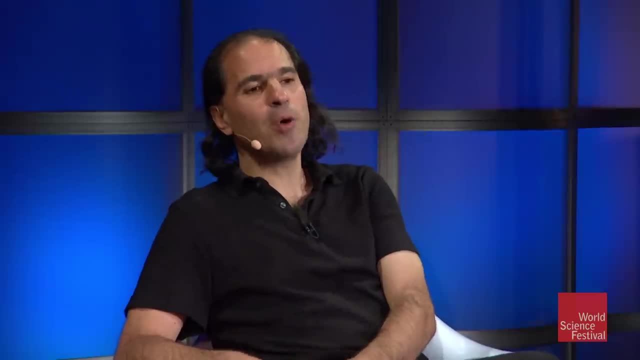 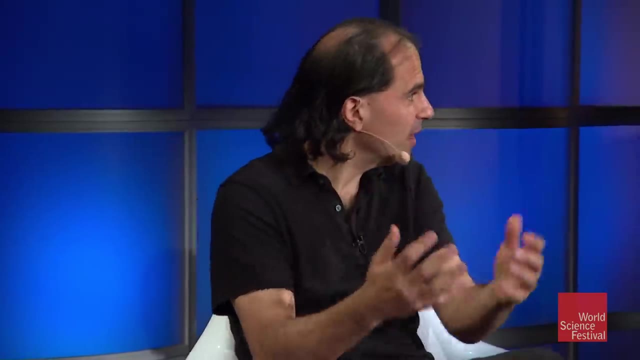 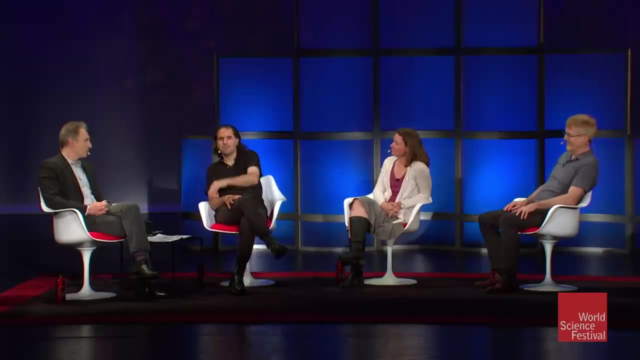 you to these incredibly simple, compact looking formulas. and these formulas are really directly reflecting the underlying principles of space, time and quantum mechanics that govern everything. so so it's, there's- there's not very there's no real veil between these, these remarkable simple formulas and these grand 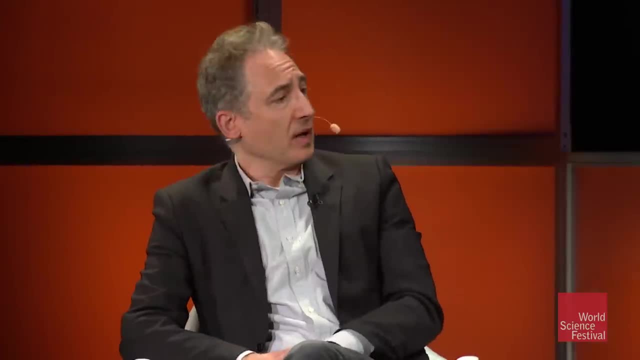 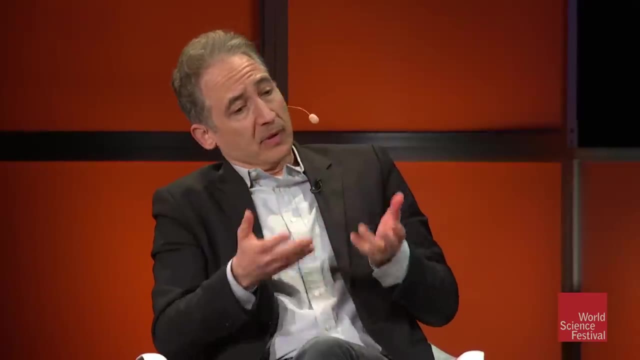 underlying principles of 20th century physics and to draw the connection to Higgs and others who were working along the same lines in the 60s, and I think that's one way of describing what they found was a powerful way of including mass in a manner. 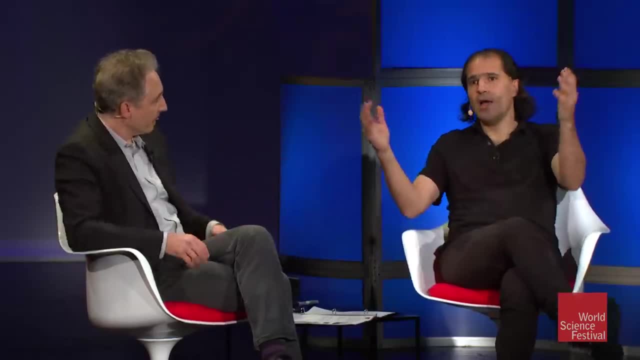 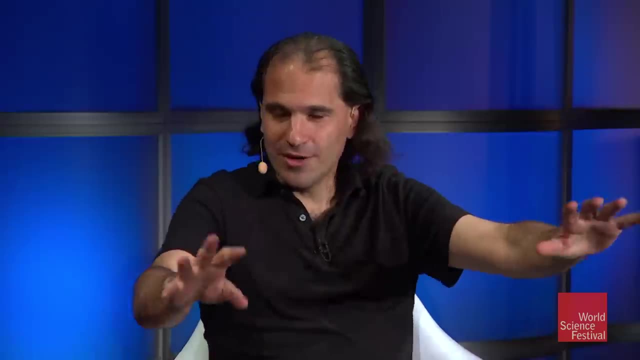 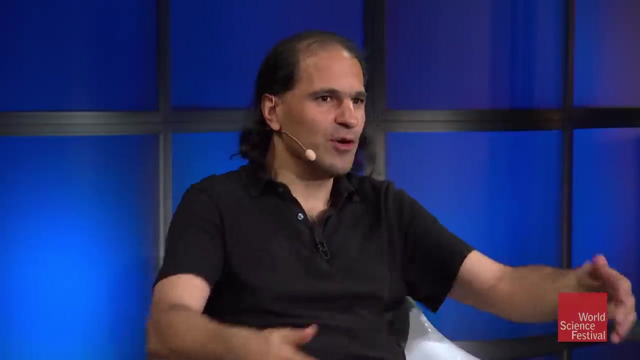 that didn't spoil the beautiful underlying symmetry. in fact I would say that I mean this molasses analogy is. it's probably the sort of best metaphorical analogy that one can use. it raises various questions that probably occur to you if you're a kid in the audience. 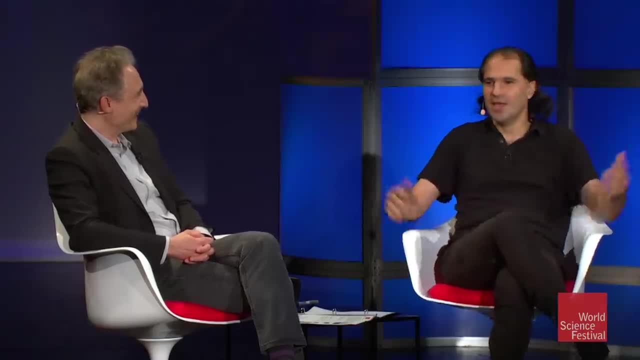 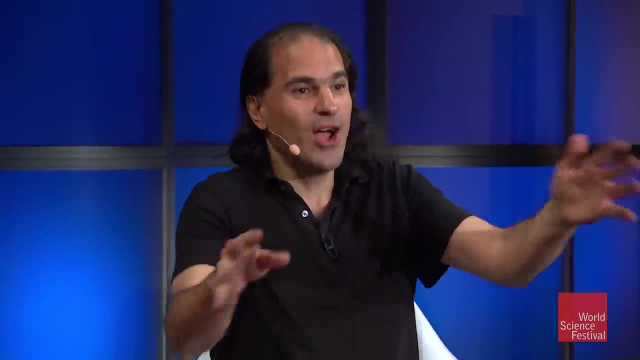 you know, is this like the ether all over again, Dom? you know, didn't you not have the ether? You had the ether 100 years ago and it's gone now. All we can say is that this is something, but it's not like the ether. 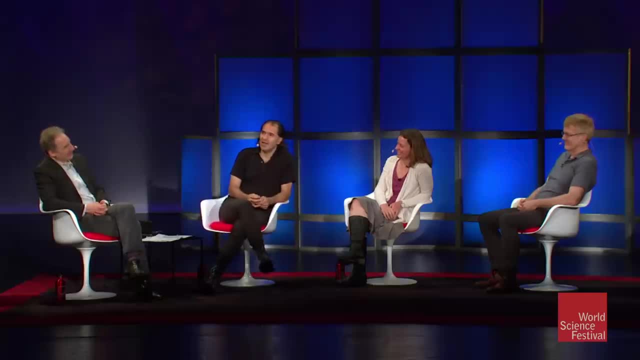 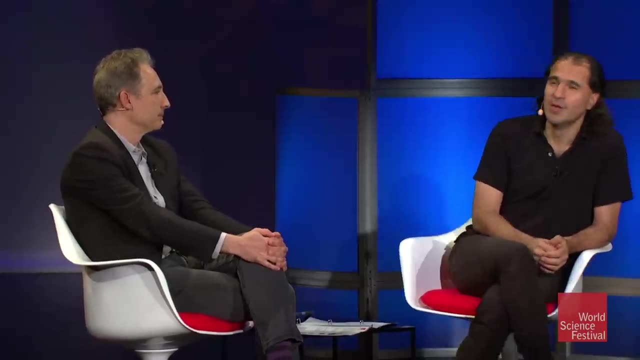 It sounds like ether but it's not like the ether. But I suspect the most fundamental way of saying what the Higgs is about, the way that you know people will still be talking about in 200 or 300 years, after maybe robots have come up with better metaphors and analogies. 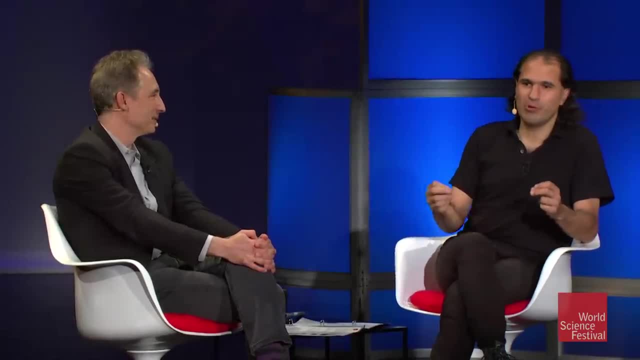 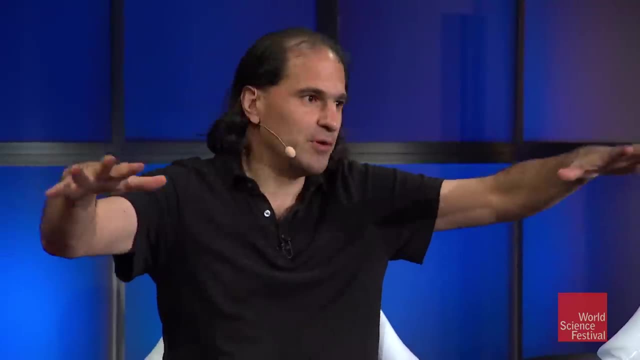 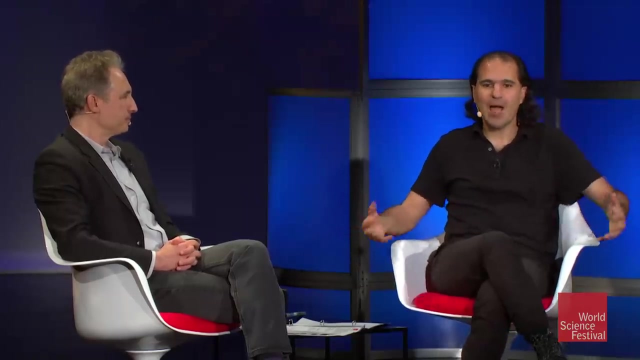 is that it's sort of precisely what Brian just said. The world of massless particles is completely prescribed and sort of fixed by general principles of space-time and quantum mechanics. The world around us appears to have massive particles in it, And so you have to somehow take the stuff that you see. 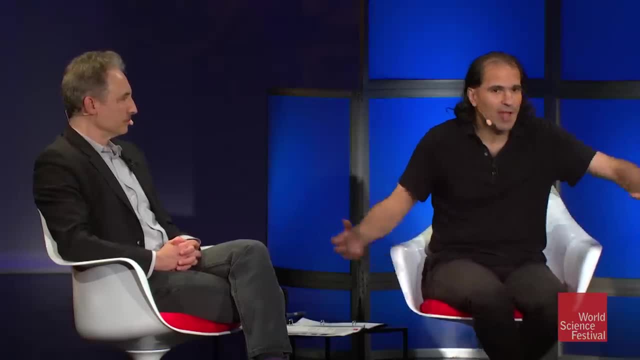 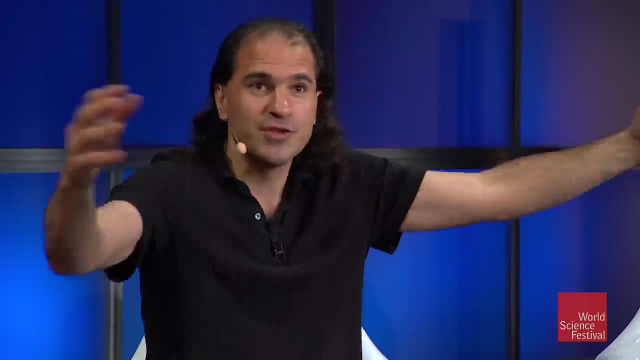 that's slow and massive and low energies and as you collide them at higher and higher energies, be able to continuously interpolate to a world with massless elementary particles smashing into each other at very high energies. And if you just finish this countermeasure, 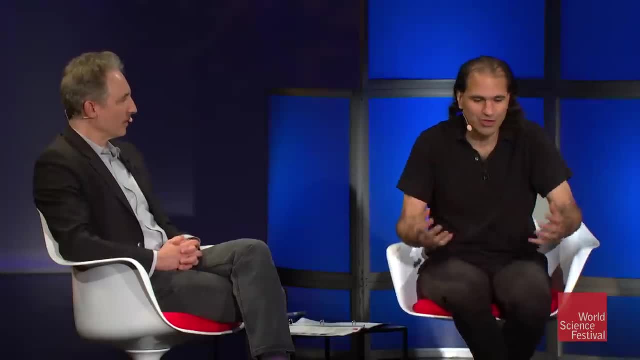 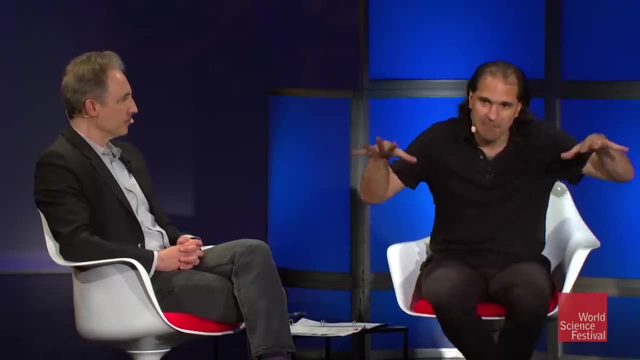 something that we talked about and you went through it in a little bit more detail, you would find that you just can't do it with the elementary particles that we knew of before the Higgs. You just had to have something else in order to be able to take massive low-energy particles. 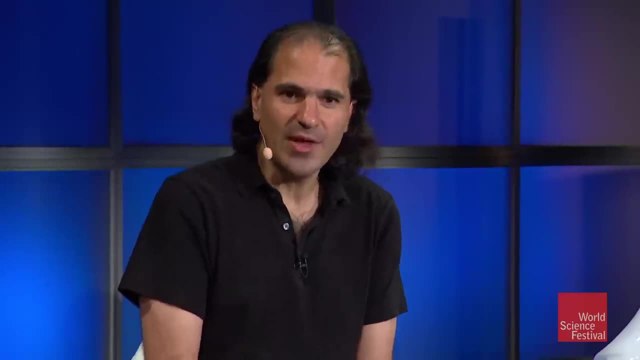 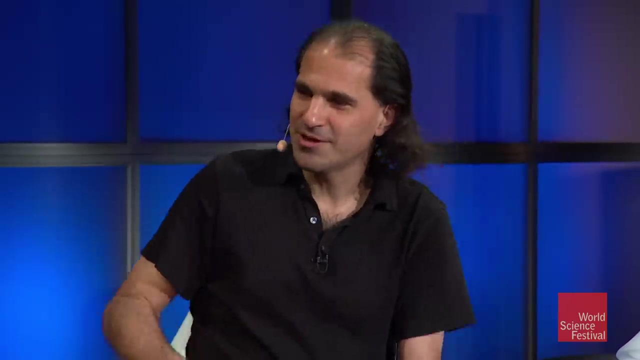 and interpolate them to massless high-energy ones. The incredible thing- and this is part of the sort of cognitive dissonance and the real irony about the Higgs You just described it, for example, as something people knew ought to be there for 50 years. 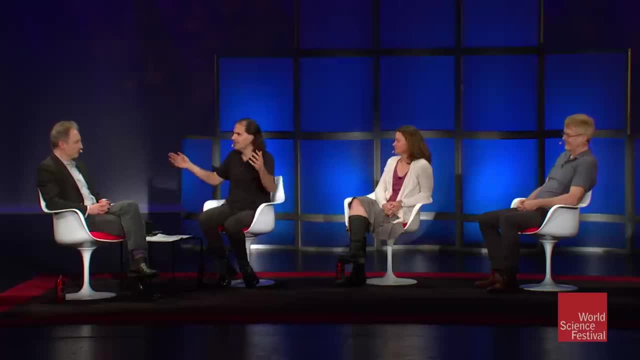 So that's like it's very amazing that people predicted it, but it's sort of boring that it's the thing that we expected all along, But it's in fact something. it's actually quite shocking. We'll come to it later in the discussion. 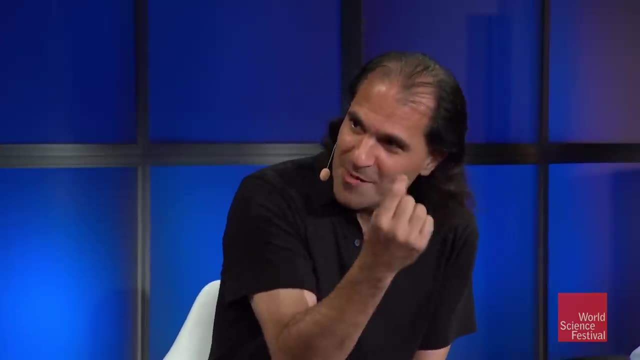 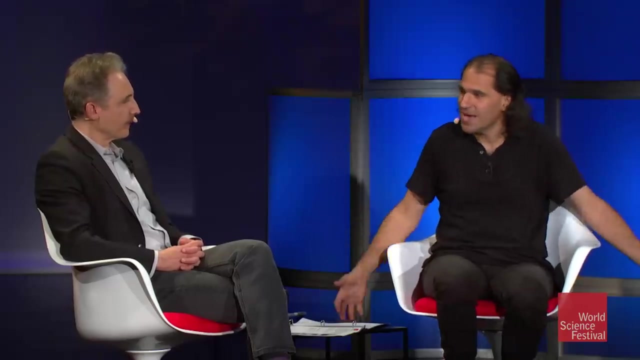 It's quite shocking that all it took was one stinking little elementary particle. Just one extra thing was needed to allow us to be able to interpolate smoothly and continuously between this world of massive particles at low energies and this very sharply prescribed world of massless particles at very high energies. 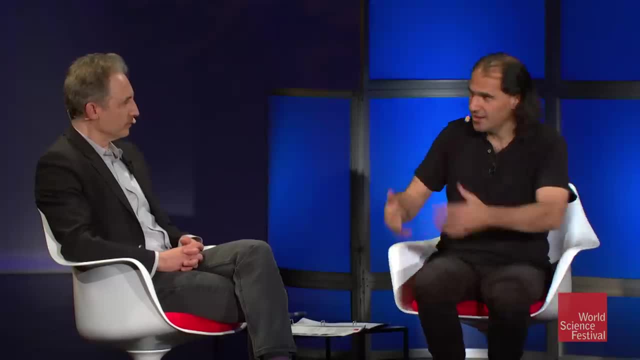 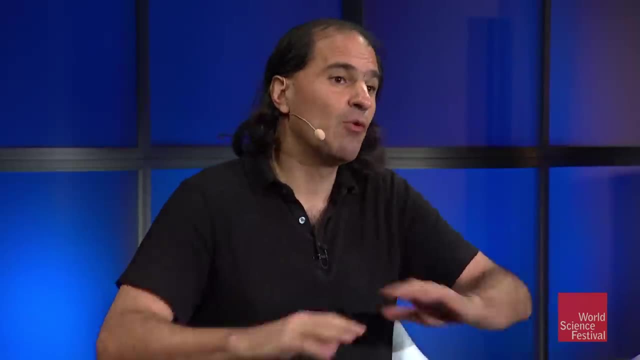 And it's shocking that it was so simple. That's the irony about the Higgs that we'll come to. It's that nowhere else in physics when this rough type of phenomenon happened did anything remotely as simple as the Higgs happen. 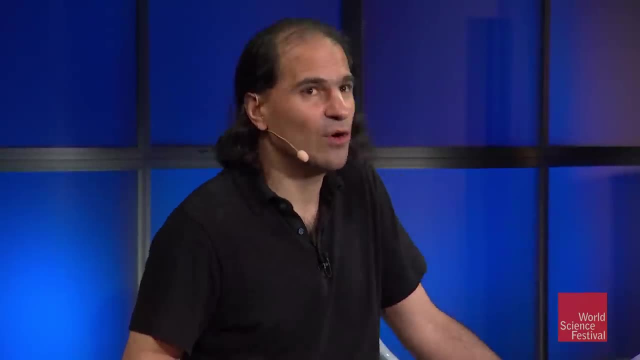 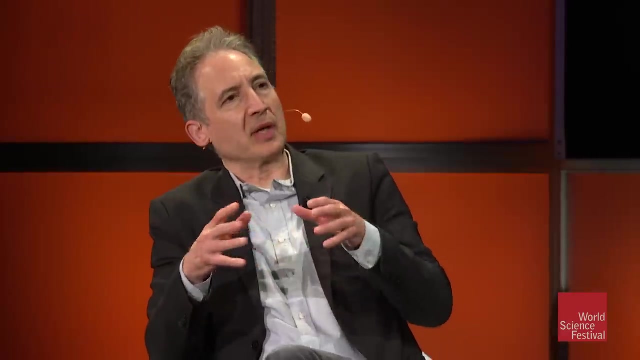 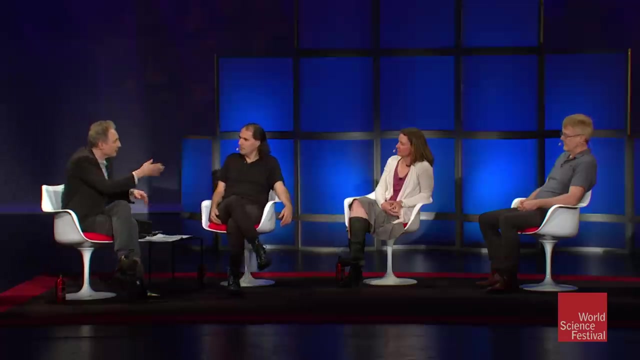 And it's a feature of the and a mysterious feature of our world that the simplest possible answer ended up being right. So, along those lines, as we've tried to push our understanding of the world further using this idea of symmetry, particles that, in some sense, are the different tips of the snowflake, 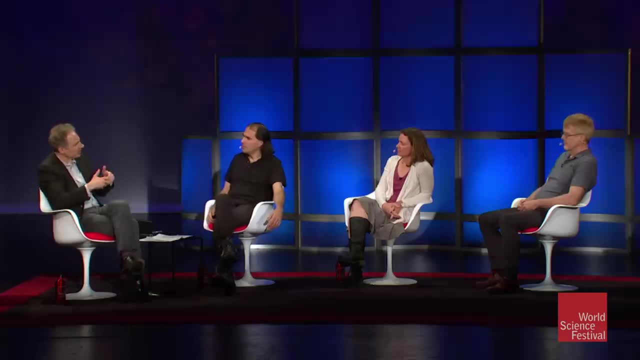 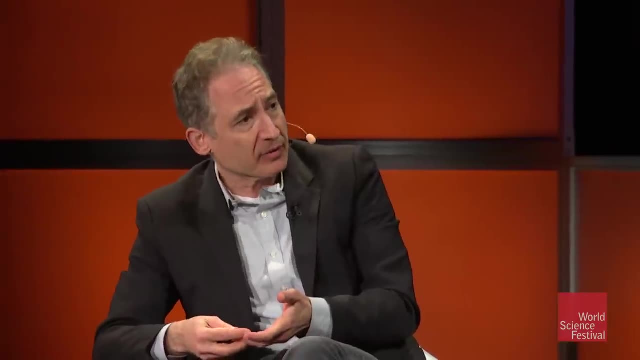 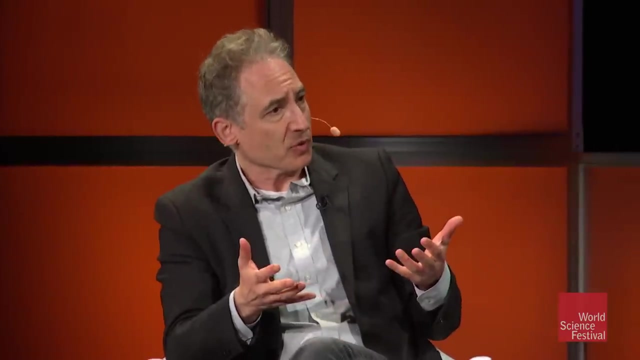 to use Joe's metaphor, that can kind of be rotated into each other in some sort of abstract sense. We have come upon other symmetries, mostly from mathematical studies, not really from observations of the world, And the most prominent among those is supersymmetry. 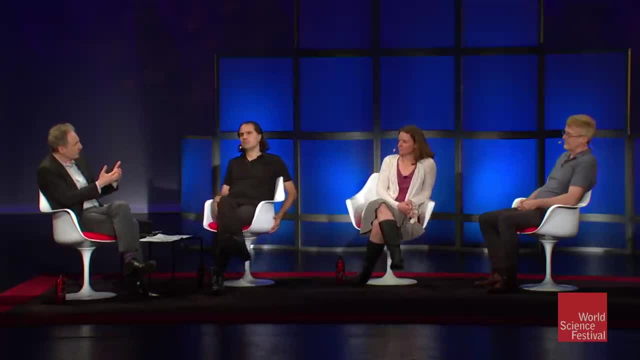 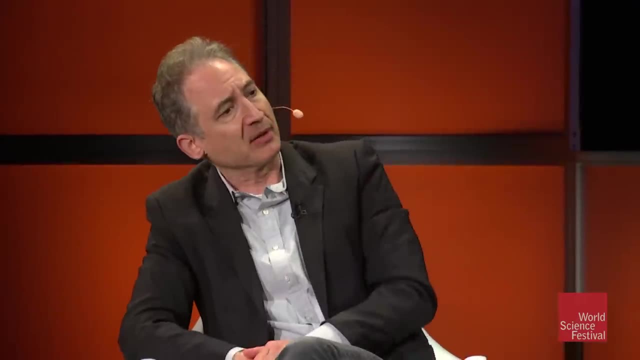 So can you tell us a bit about supersymmetry and what it implies for what we should find out there in the real world if nature abides by this particular symmetry? So supersymmetry is actually an idea that relates, not the tips of the snowflake. 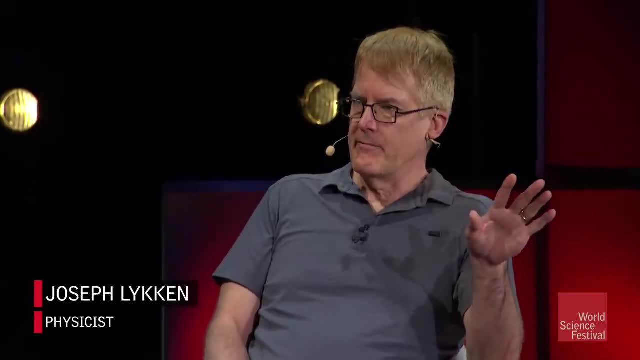 but it actually relates the kinds of particles that we said we were going to find out about- And we said we were going to find out about, We were made out of these fermions of matter particles, to the bosons, like the particles that carry forces. 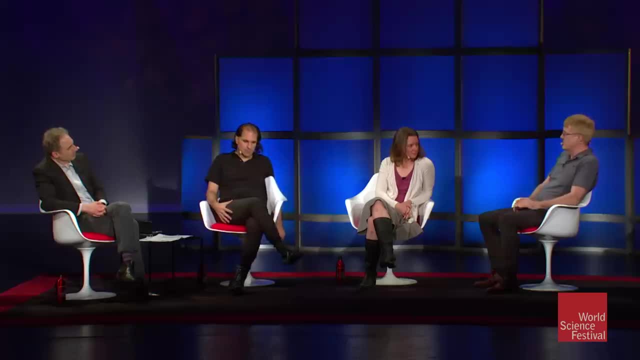 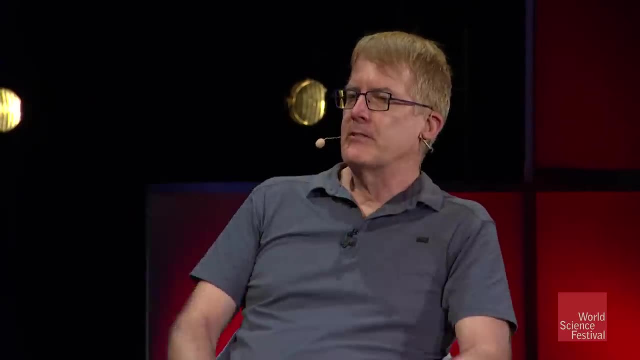 So that sounds like a very profound relationship, and it is a very profound relationship. It was first noticed by a bunch of physicists in the 1970s and immediately got the whole community that we belong to excited, because it sounds like it's a theoretical breakthrough. 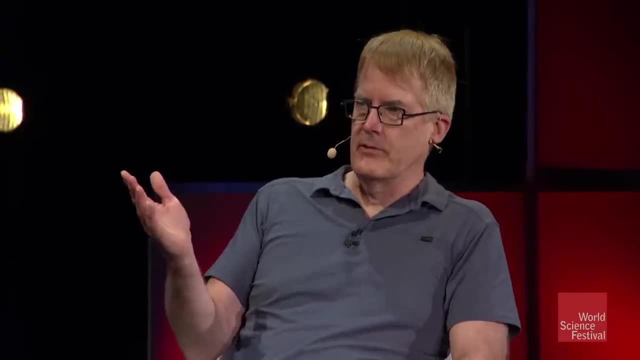 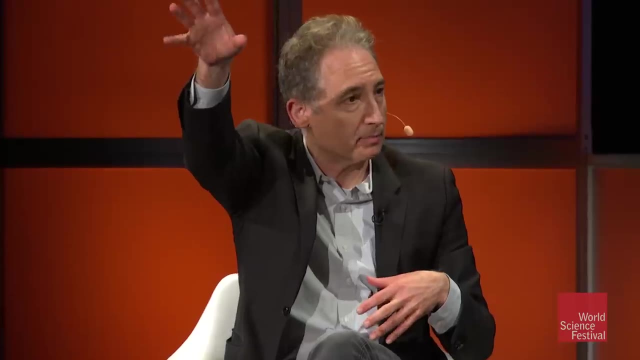 It also makes predictions. It predicts a bunch of new particles. Now, the way you framed it, let me just say the way you framed it was- it takes the particles that make us up and it relates us to them. The particles say, that make up light like the photon. 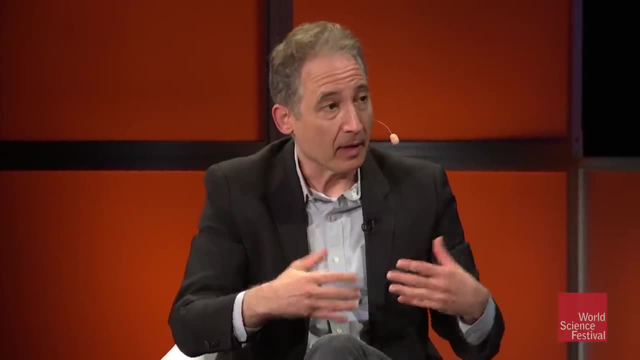 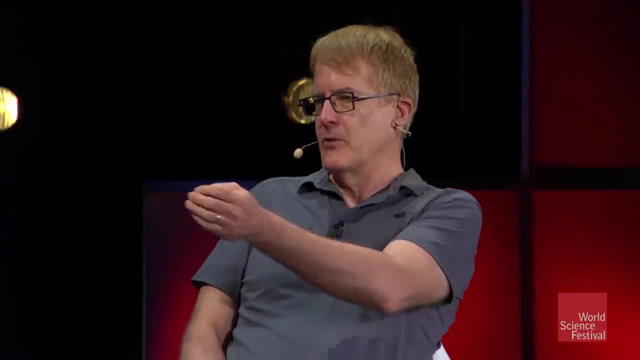 Yeah, That sounds very economical. Yes, It's not quite as economical as you might have thought because, for example, the electrons you have in your body are related to a boson in supersymmetry, but it's not the photon and it's not any of the other bosons you showed on your chart. 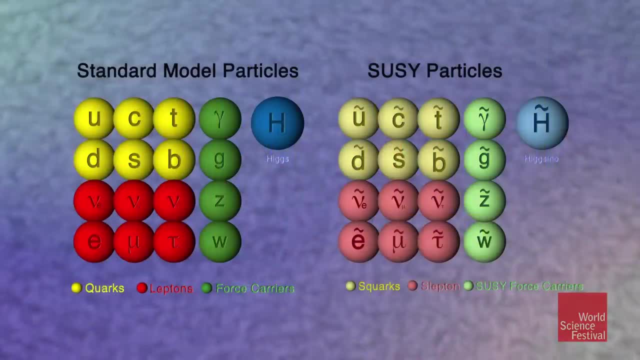 It would be a new particle. We call it the selectron. In fact, I think you see it up That hasn't been discovered yet. Yeah, So in that sense it doesn't sound economical because it's postulating a whole bunch of new particles. 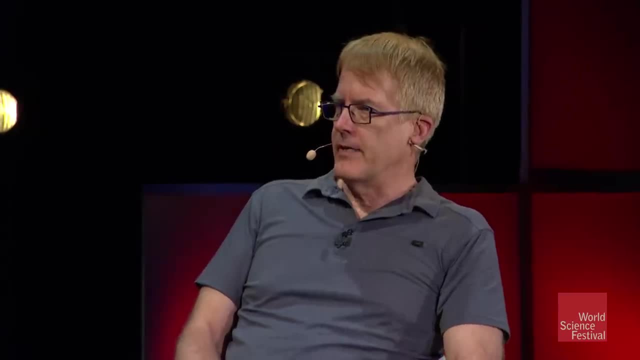 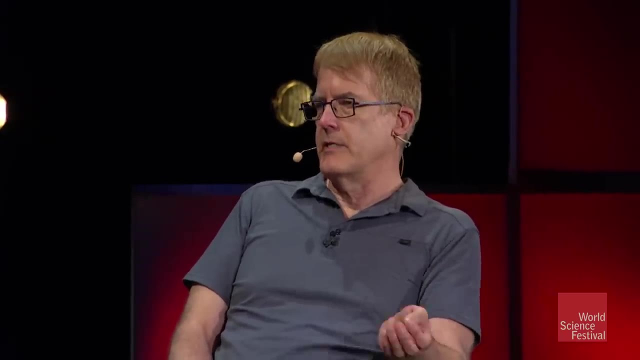 that nobody had seen. On the other hand, there's a historical analogy for why this might be reasonable, which goes back to what Nima was talking about was the early days of quantum mechanics, when we were trying to understand how quantum mechanics can be made compatible with relativity. 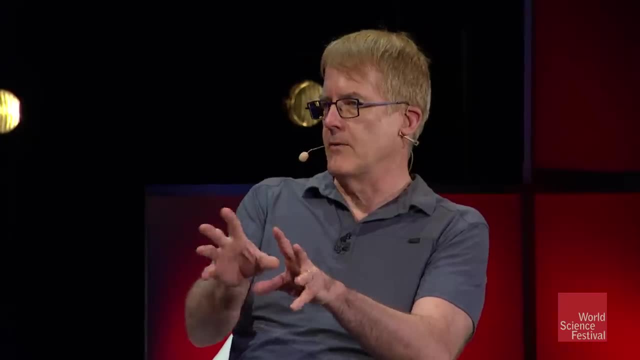 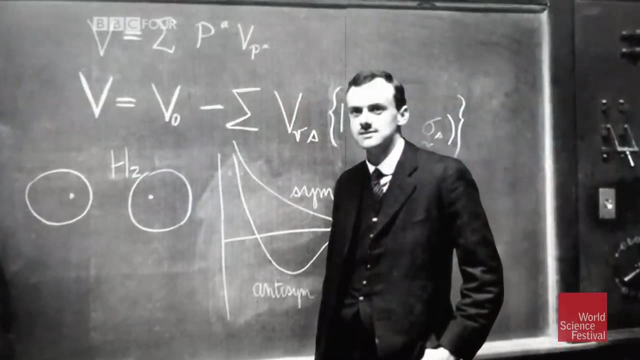 And, as Nima said, that is a very, very difficult mathematical understanding, which was Part of it, was first put together by Paul Dirac, one of the great giants of our field, and he found in making that work just in the mathematical basis. 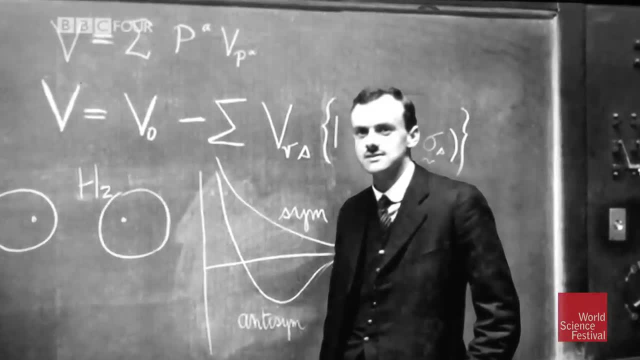 that that particular particle predicted also a bunch of new particles, what we now call antimatter antiparticles, which also seems pretty out there, And in fact Dirac. it took him a long time to convince himself that this even was reasonable. 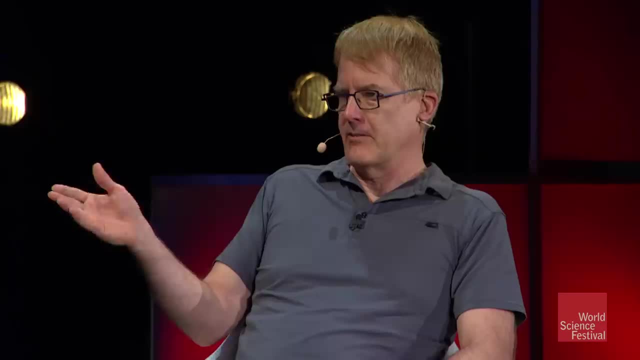 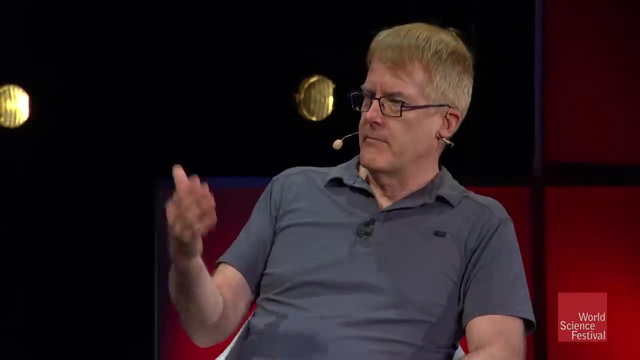 But he was right And in fact he was super lucky, because the first antiparticles discovered about a year after his prediction came out. We now know that antiparticles exist, We can make them and they're part of our standard model. 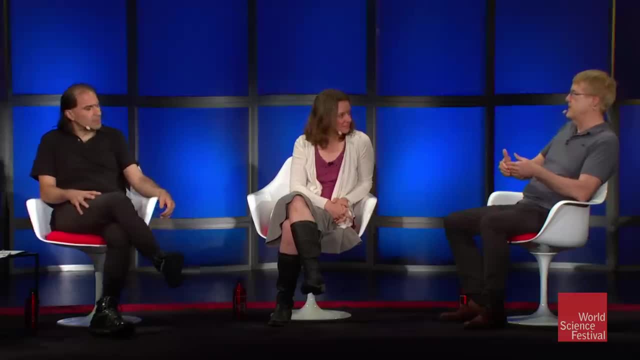 So in some sense, supersymmetry is, if you like, the next phase of that. It's saying, yes, there's antiparticles, and then there should also be these superpartner particles, and you just have to go out and find them. 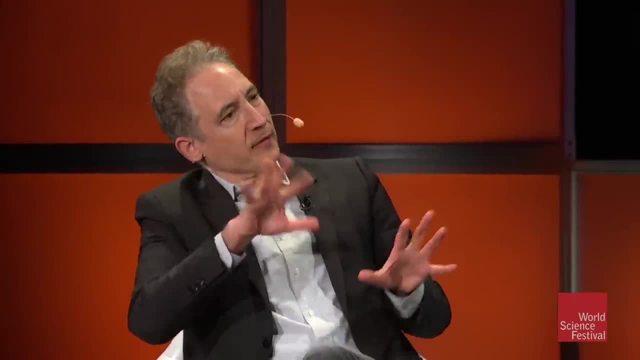 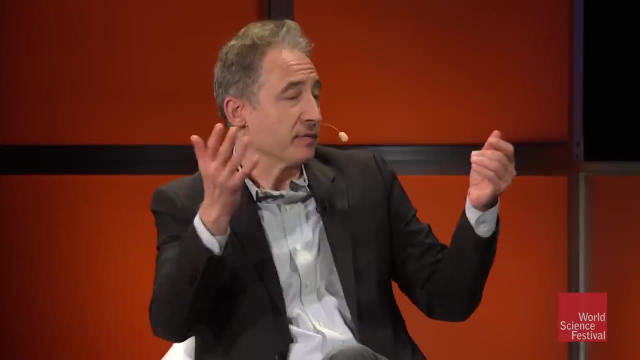 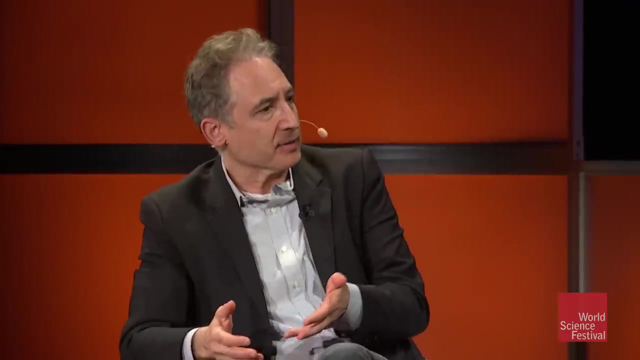 So let me just make sure we have the full playing field. So the idea, then, is we see a pattern playing itself out over the course of the last hundred, if not more, years, where you invoke some notion of symmetry embodied in mathematics and make some statement about the world. 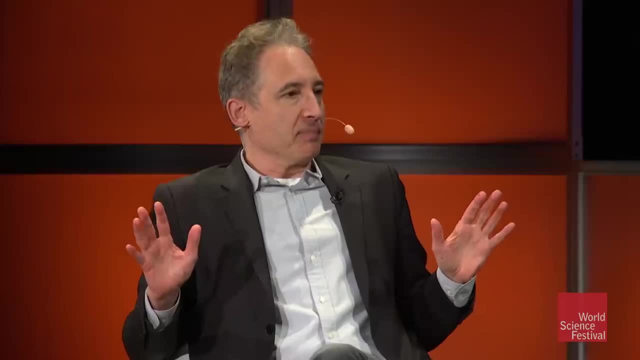 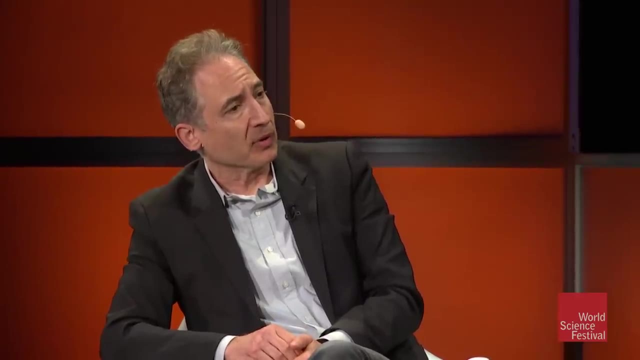 You resist it at first because it's something you haven't yet seen, but then you go out and you look for and you happen to find it. In fact, there's a beautiful quote- I think it's Steven Weinberg- where he said: 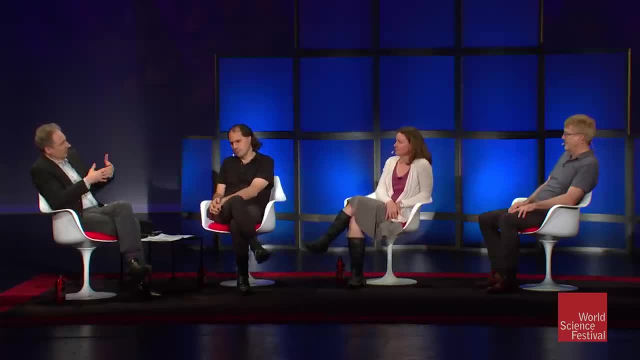 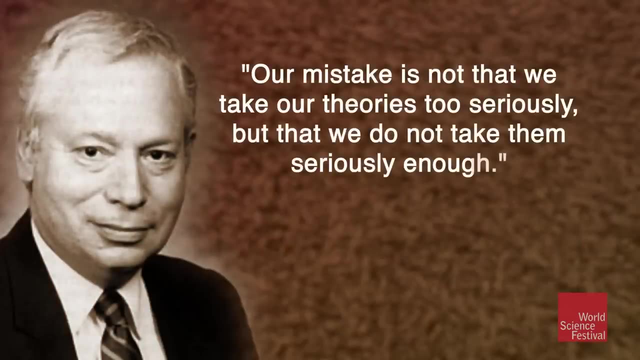 the problem with us theorists is that, not that we don't take our equations seriously enough, it's not that we take them too seriously, we don't take them seriously enough. Yeah, good, we have it right here, And so, if you sort of take this to heart, 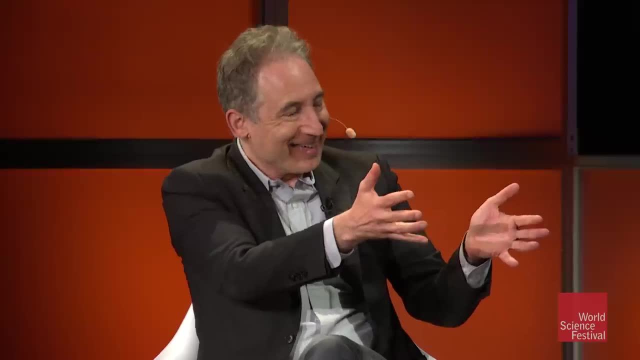 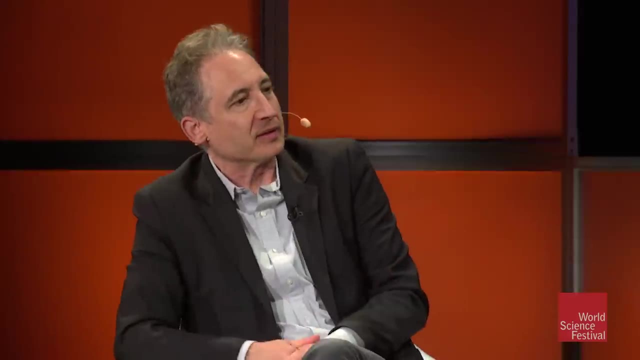 it does suggest that if there's this beautiful new symmetry that, as you say, seems to in some sense be the final symmetry that you could ever invoke, because it puts sort of everything together, there's a strong mathematical motivation to look for all those particles that this symmetry implies. 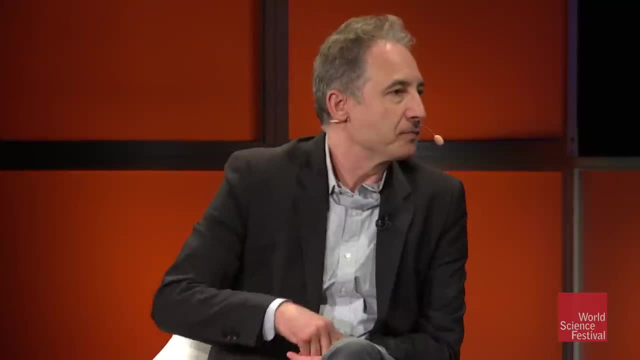 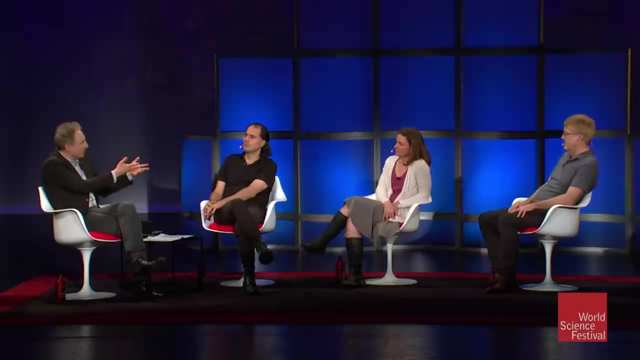 But that I mean. how do you then make the argument to governments and to funding agencies? right, Because this is not a small undertaking, right? I mean? this is part of the motivation for the Large Hadron Collider, as well as with the Higgs. 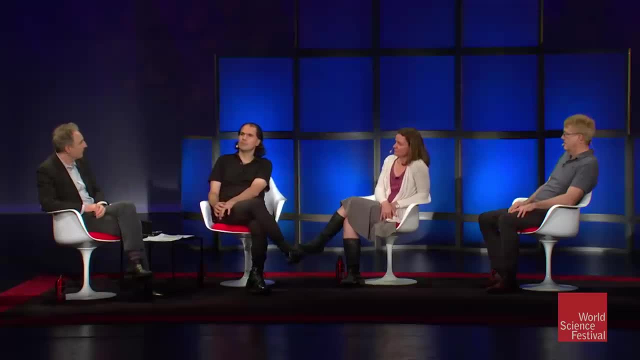 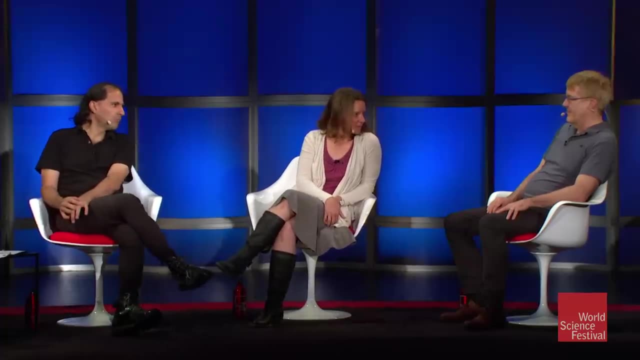 How much did that machine cost? Oh, what was the cost of the LHC In the end? I mean, it's hard to do. you remember what's the final number of the LHC? It's, you know, it's billions of dollars. 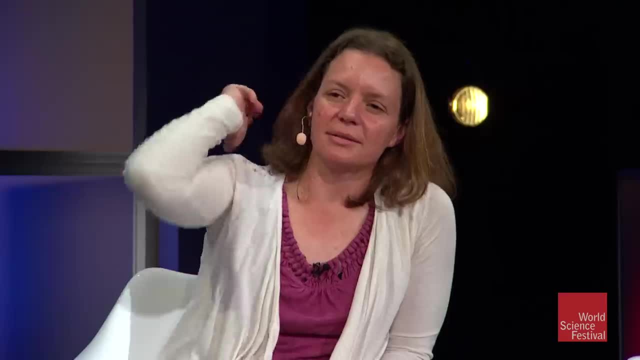 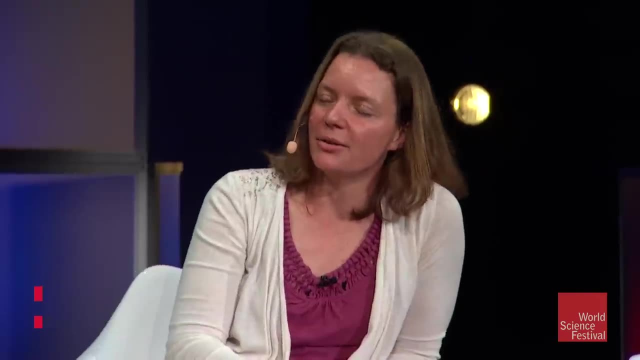 Yeah, it's under 10 billion or so dollars. Yeah, but it's a hard number to quantify, I mean, because in that number you have, you know, like my salary and Joe's salary, you know, Sure, of course it's a very small fraction. 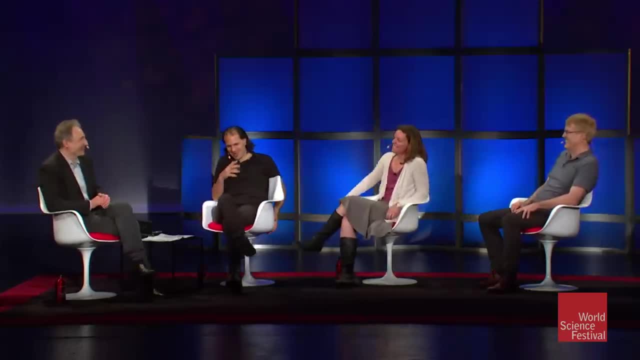 Yeah, which is a very small fraction. Now we're up to 12 billion, right? Yeah, exactly, yeah, So, but you know, yeah, it was, but you know, I think that the time that the LHC was built, 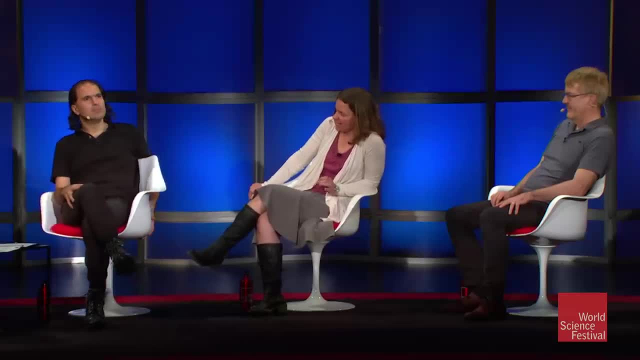 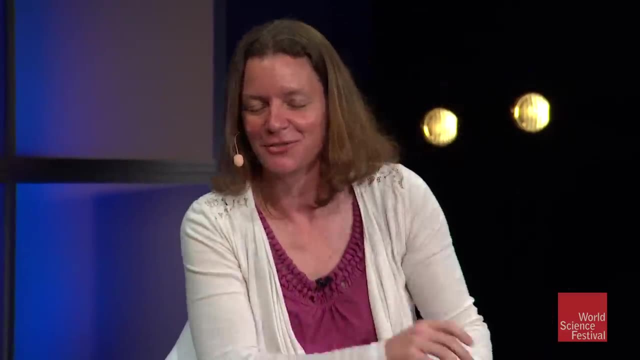 was, was a very unique time in particle physics and it's exactly like it's a unique time like we're at right now. So there's a great symmetry between, you know, the start of the LHC and the start of 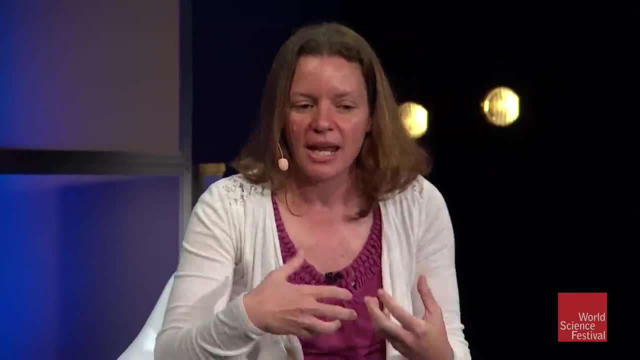 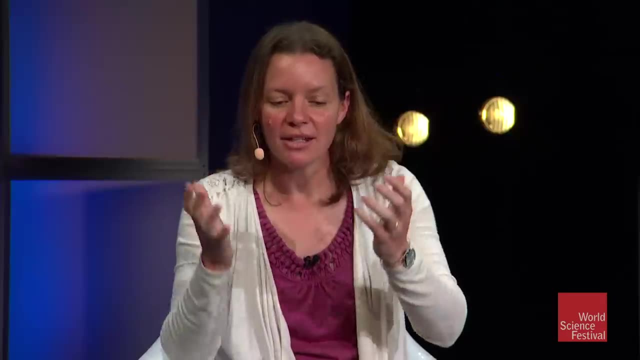 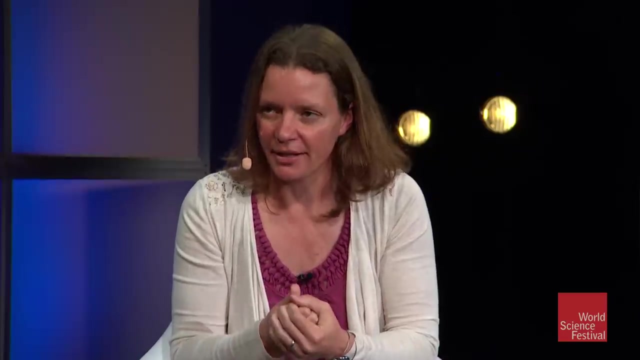 what's going to happen next, Which was, you know, we had a tremendous amount of of- well, evidence is the wrong word, but we had a tremendous amount of of consensus that there was going that we would discover something at this energy. 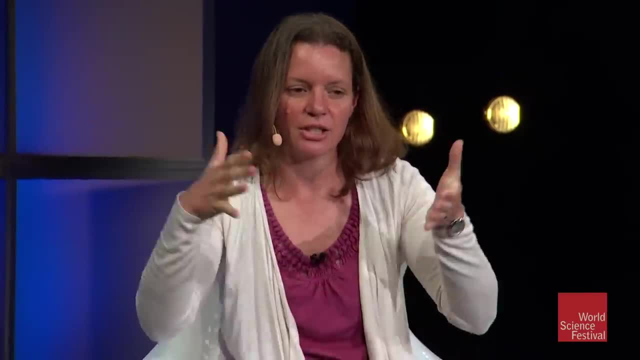 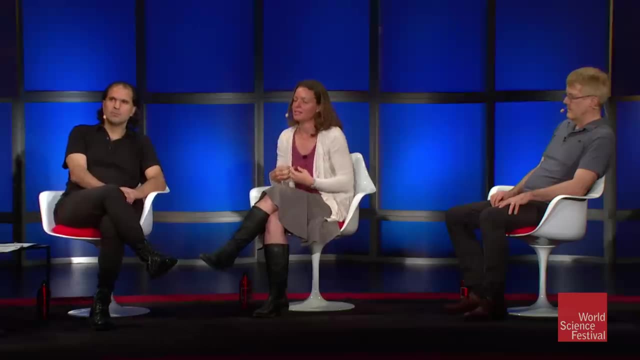 This energy is very unique to the standard model. So the energy at which the LHC can probe, let's say the energy of particles that the LHC has has enough to produce is, is a very key energy to the theory itself. 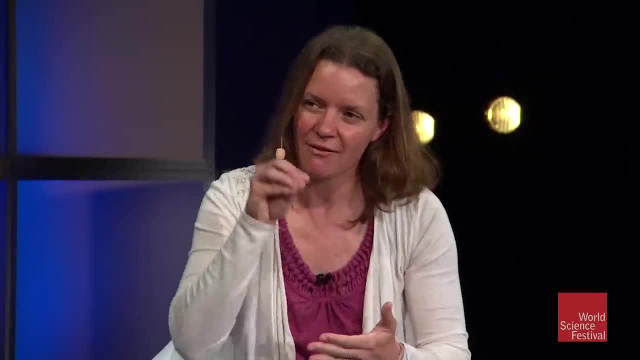 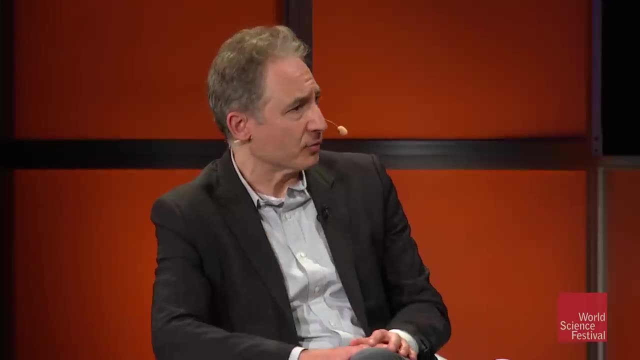 And so if you expected supersymmetry to appear, you would have expected it to appear at the LHC energies, And did you? did you expect it to? in fact, I'd like to ask all three of you, because there's a lot of rewriting, I find. 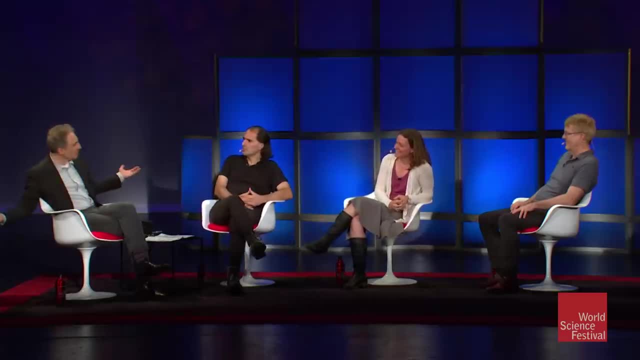 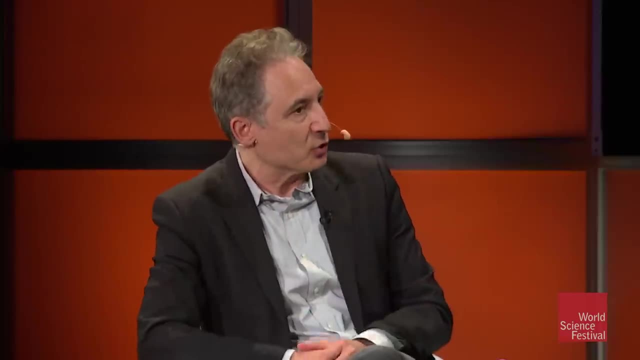 of history. post facto that happens, And we're just a small group of friends intimate gathering here. I mean, how many of you really would have argued and thought that supersymmetry, those other particles that we saw briefly on the right-hand side of the screen? 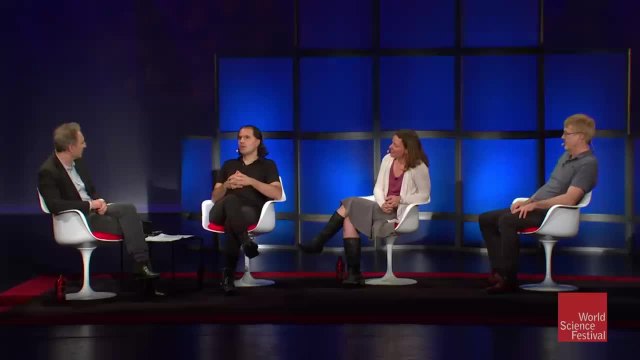 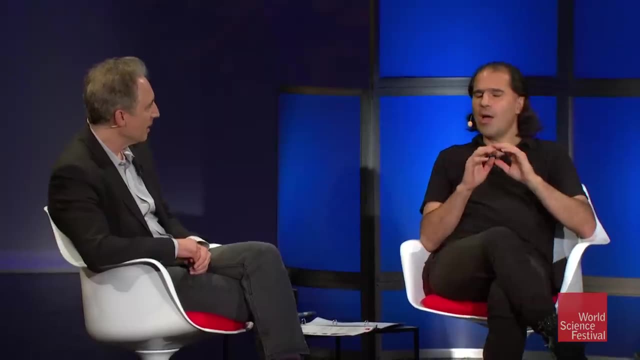 would be found by now at the Large Hadron Collider Nima. I mean, did you? Well, I, I think um, And I'm looking for a yes or no here just so I can like. Well, actually, I, I um. 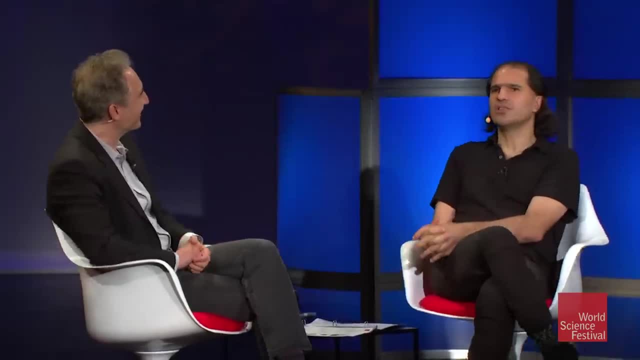 I would have said already: No, it's actually. but it's actually a very interesting question because there is a whole, it's not because it's not just about supersymmetry, There is an entire. it's presumably something we'll. 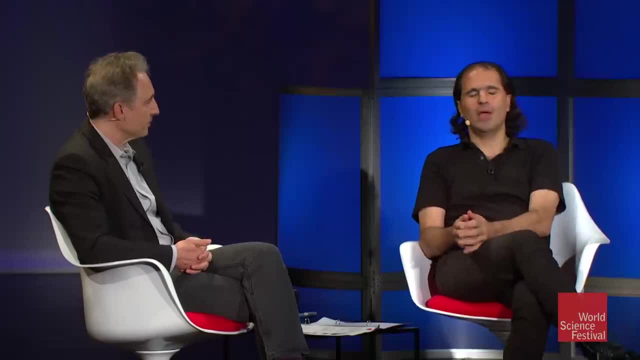 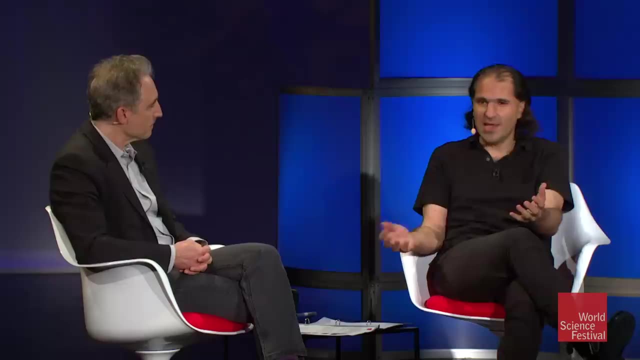 we'll come to in a second. there's a sort of whole paradigm that goes around um the existence of the Higgs particle and how strange it is, how, how bizarre it would be to have the Higgs as a lonely beast accompanied by anything else. 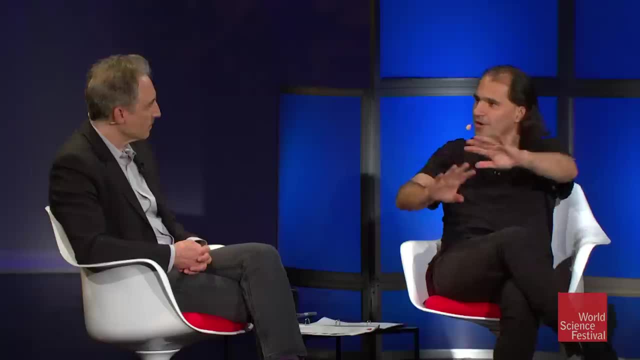 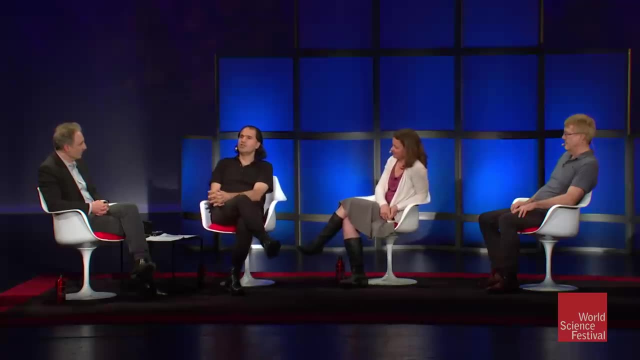 That's something, uh, even when we've seen roughly this kind of phenomenon elsewhere in physics before, we've never seen something like that for very good theoretical reasons that perhaps we'll, we'll come to. So there's a whole sort of paradigm. 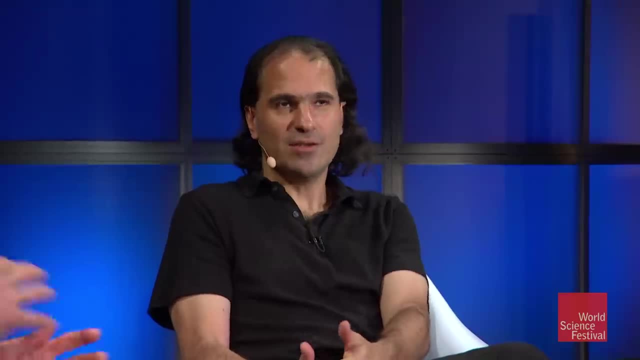 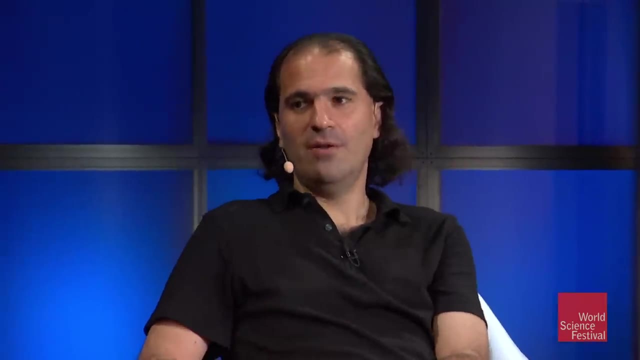 built around, um, uh, uh, what it would take to see something like the Higgs particle. Yeah, And it's that whole paradigm supersymmetry being the sort of best developed version of of uh and most concrete and uh. 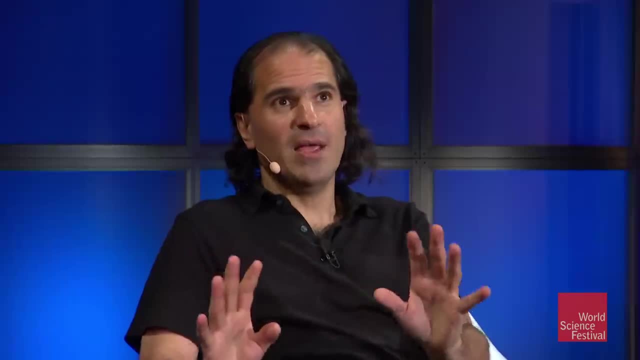 and and and well put together version of that paradigm And, by the way, it's not broadly the idea of supersymmetry, I mean the the uh, uh. as it's been said a couple of times, supersymmetry is just. 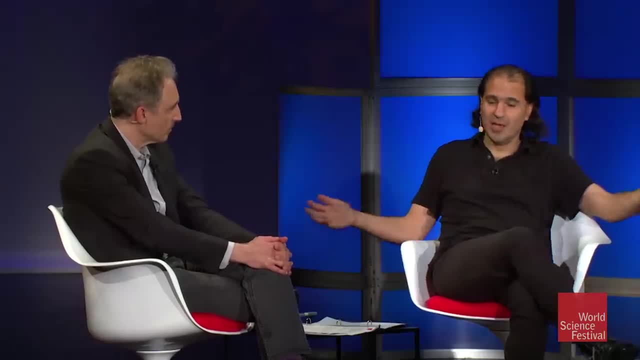 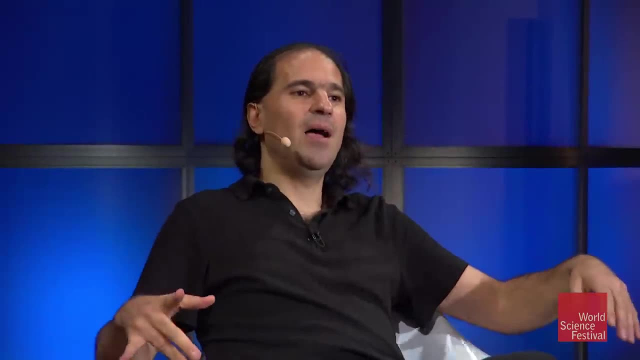 the very last thing nature can do, compatible with its grand principles, that we have not yet seen it do. Yeah And uh, uh, but this is at the level of massless particles, right? Um, uh. however, there is mass in nature. 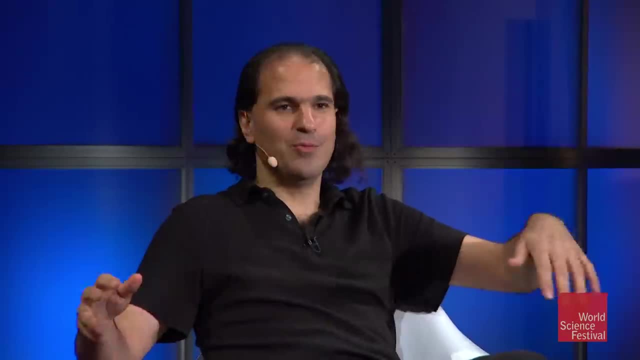 And so so we have to go to high enough energies, where where we we see all the relevant particles, in order to be able to see the asymmetry. Um, from that point of view, supersymmetry could show up, you know, anywhere. 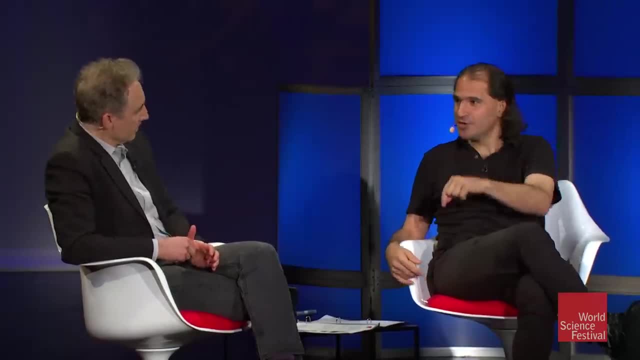 and still be relevant for nature. But there's a specific problem associated with the Higgs particle, which we'll we'll talk about more. In fact, we can do it right now if you want. Yeah, Well, yeah, So I think, um, uh, the uh. 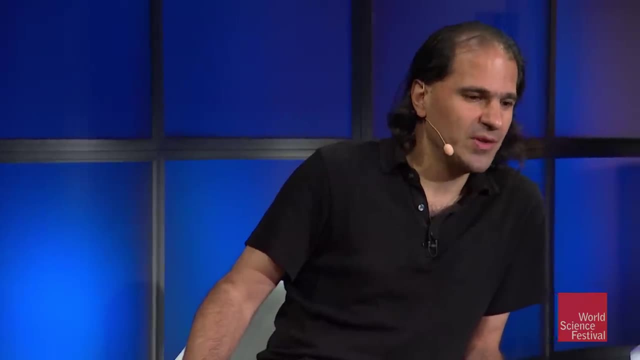 all the drama about, about the Higgs has to do with this, uh, with this, uh, with this, uh. basic fact: For all the other elementary particles, there's a difference between them being massless and then being massive. 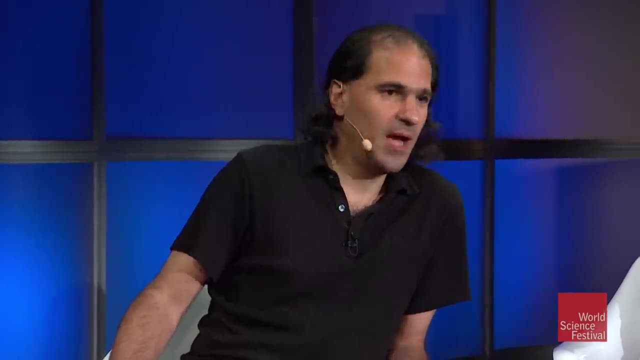 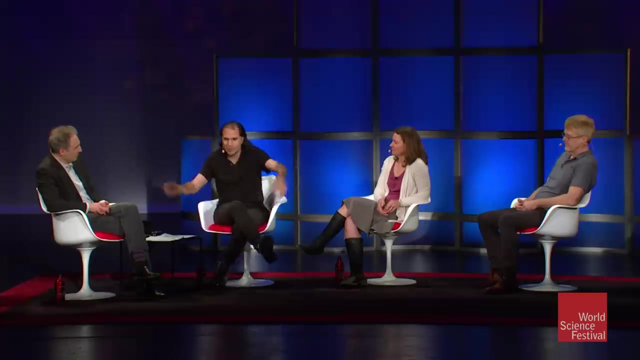 So, for example, if you ask the question: why is the photon massless? Um, uh, in this kind of uh, in this uh analogy, you imagine that, uh, that that space is filled with these violent quantum. 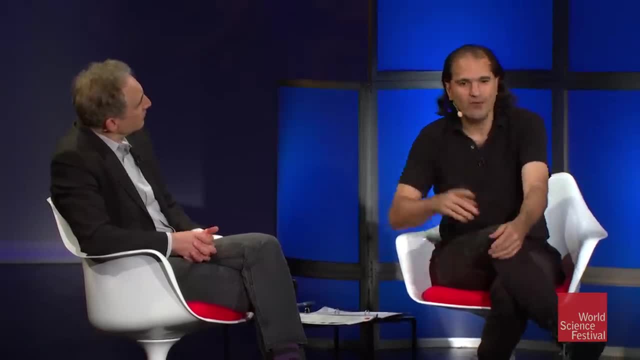 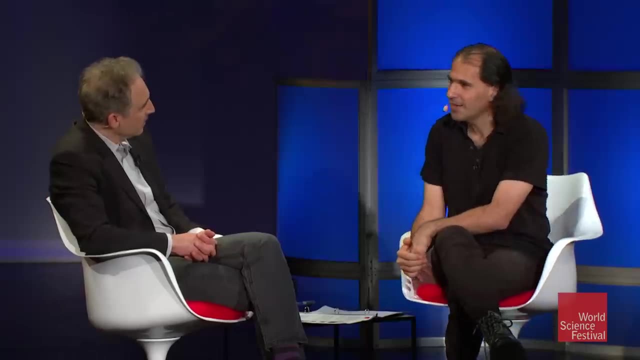 mechanical fluctuations that are, that are going on everywhere While the photon is zipping through this, uh, this kind of medium? why isn't it banging into all this crap all the time and uh, and picking up some inertia, just like the kind of? 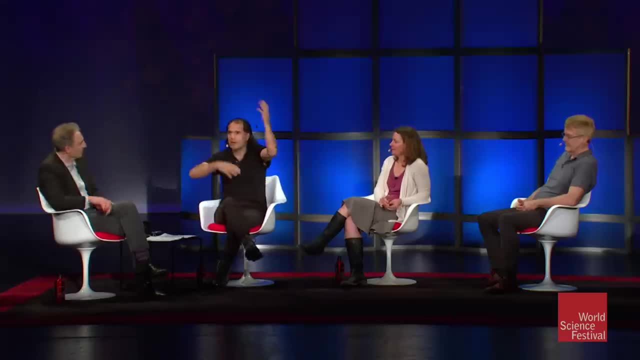 molasses. picture that we- uh, This is just quantum mechanical uncertainty. This is just quantum mechanical uncertainty going on all over the place. right, You know there are, and those quantum mechanical fluctuations get more and more violent as you go to shorter. 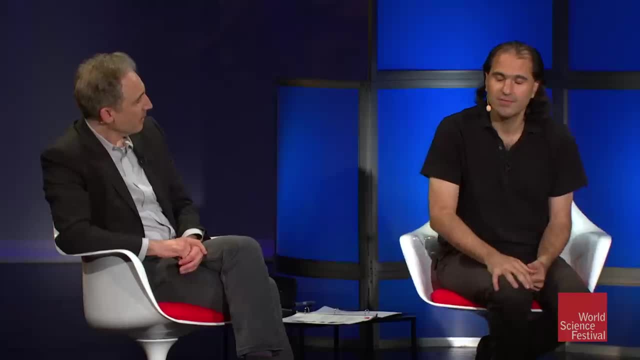 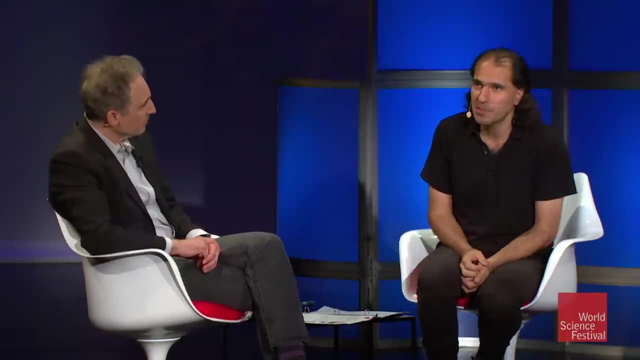 and shorter distances, Higher and higher energy. Higher and higher energy is because of the uh Heisenberg's uncertainty principle. So why does the photon, sort of impervious to this, go zipping through, uh, through through space? 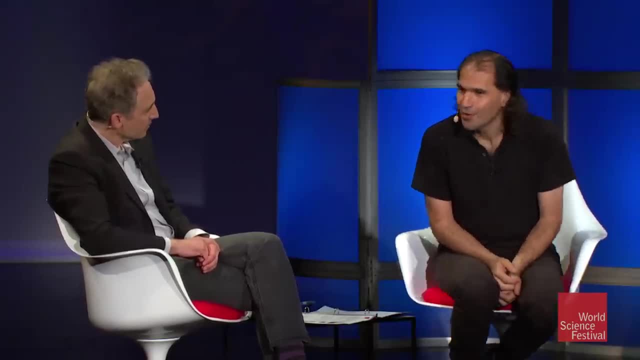 at the speed of light. And the reason is that two is not equal to three. Okay, Because if the photon did have a mass, if it somehow picked up a mass, with all these interactions, that's not. uh, you can't be a little. 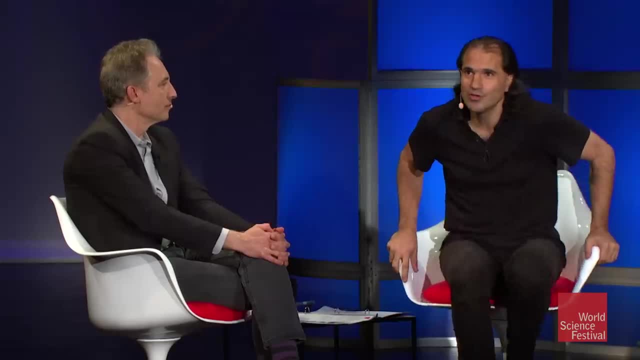 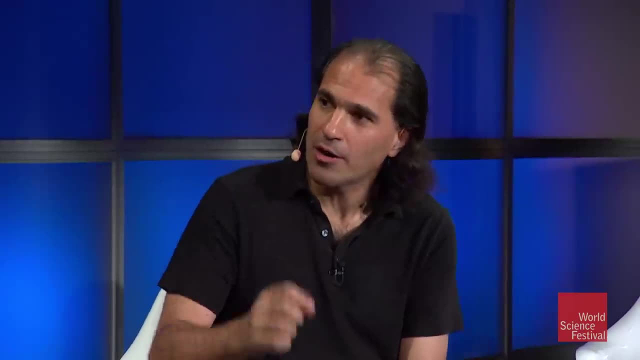 bit massive. It's like being a little bit pregnant. It's not possible, right? Those, those extra, the, the, the extra way that it can spin, has got to come from somewhere. Uh, and that's the deep reason why particles. 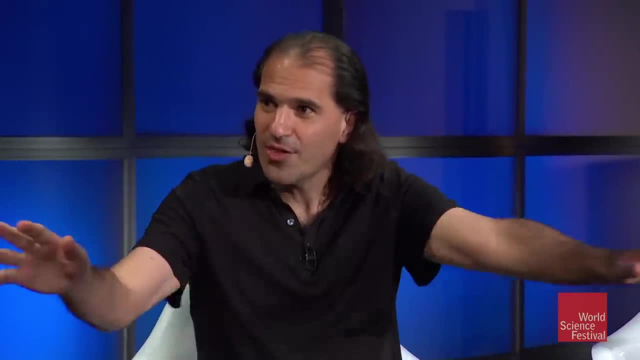 that have uh spin, like the photon, the graviton, the electron, everything else. there's a good understanding for why they could be massless in some approximation, and then you've got to do something to them to make them massive. 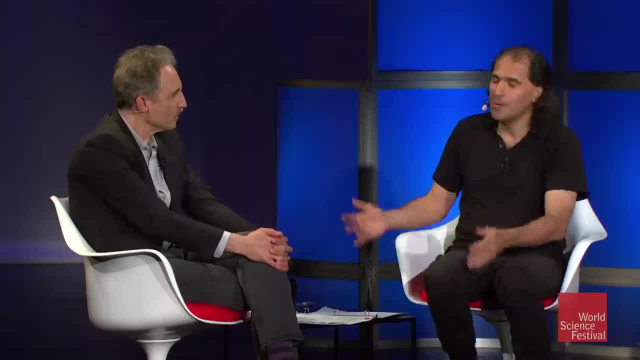 Sure, Okay, And- and that's something that has everything to do with the Higgs- Well, that's the huge irony: is that the thing that solves the, that gives us the understanding for why all the other things can be consistently massive. 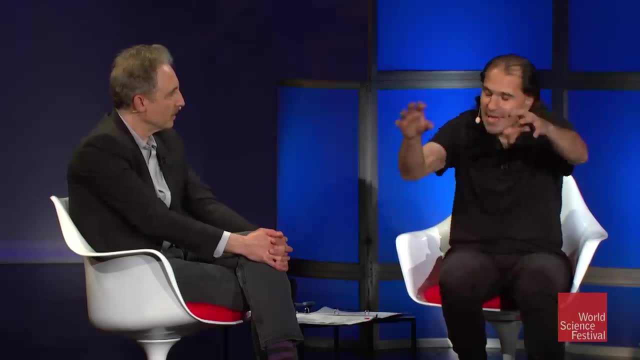 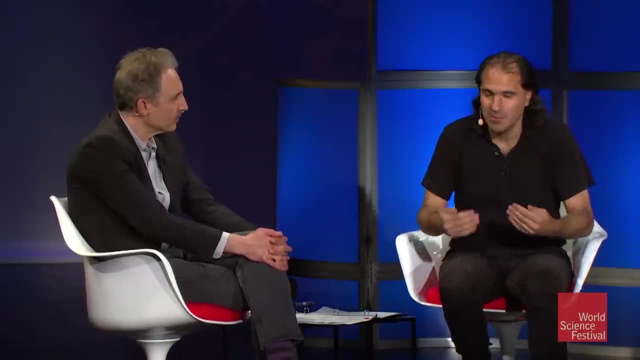 and there's a good reason why the mass of all the elementary particles is pegged to the scale associated with the Higgs. we don't understand why the Higgs itself has the has can, uh, uh, has a mass or what could be. 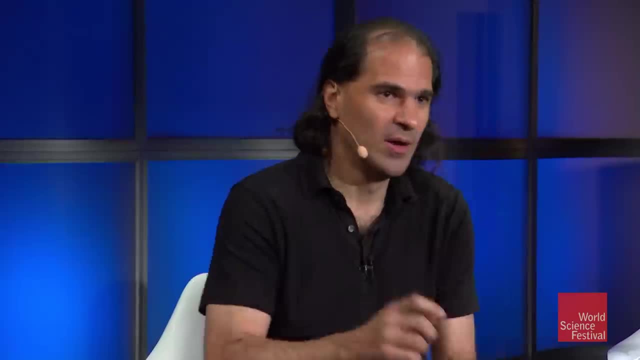 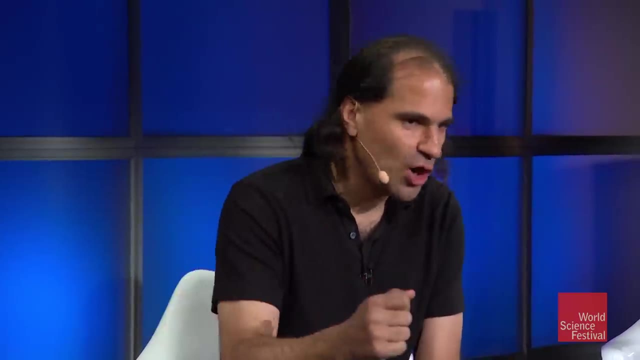 massless in some approximation, because the Higgs has no has spin zero. That's. that's the strange thing about it. It's the simplest elementary particle we've ever seen. It has no spin, no charge, no kind of properties of any sort. 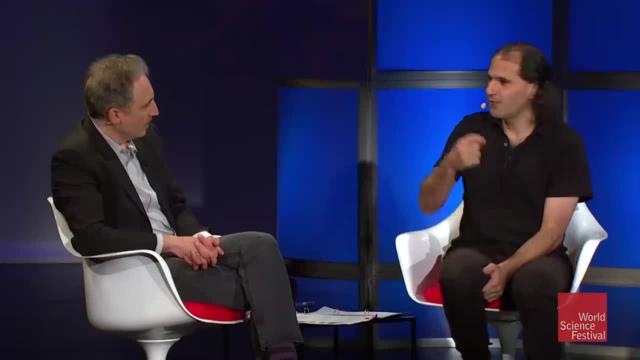 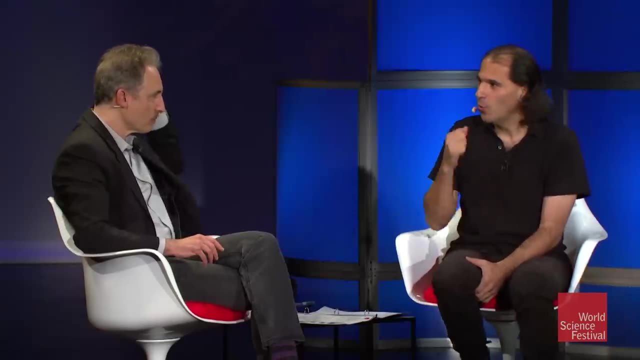 other than having a mass and the. the difficulty is that, unlike photons, for which massless guy has spin, has two degrees of freedom, massive has three, the Higgs has spin zero and one is equal to one. There's no difference between the. 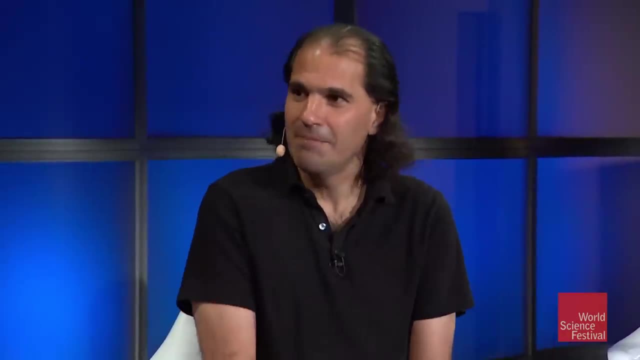 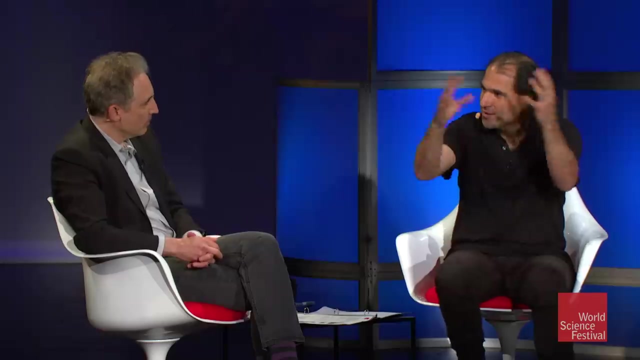 uh the the number of ways, namely none that a massless or a massive uh Higgs particle uh can have, And therefore the Higgs is zipping through. this uh complicated, uh um. 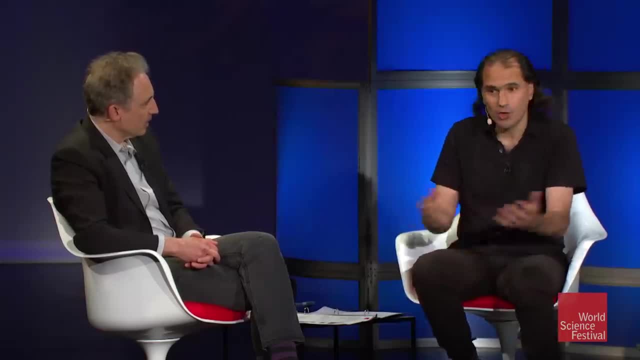 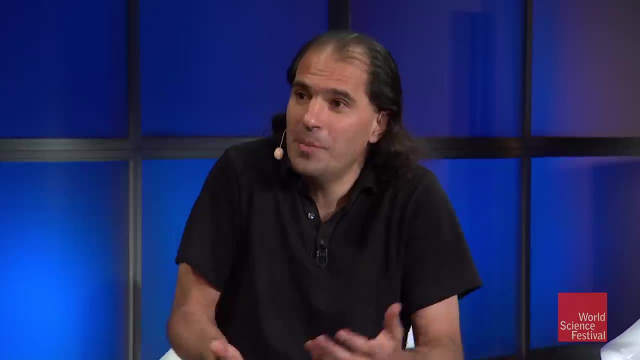 uh, quantum mechanical vacuum. There's absolutely no reason why its interactions with all this virtual crap, um, couldn't give it, uh, a huge inertia? And in fact, if you do a simple back-of-the-envelope estimate for where the Higgs 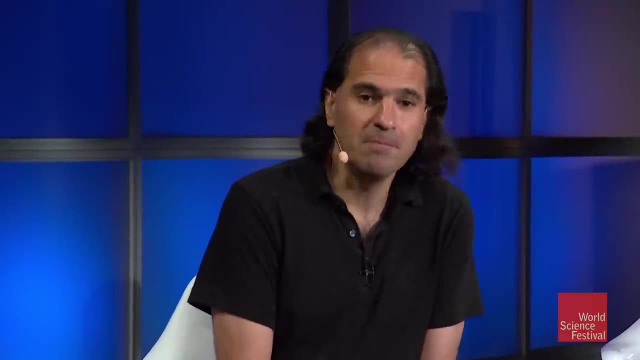 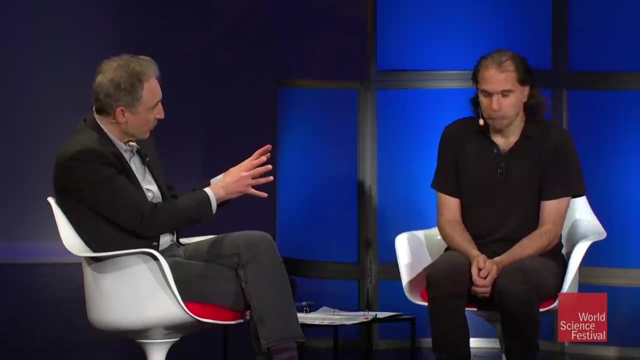 should end up, it would be orders and orders and orders of magnitude, um uh, more massive than than naively, than than uh, than than we've actually seen it to be. So you need some explanation for why. 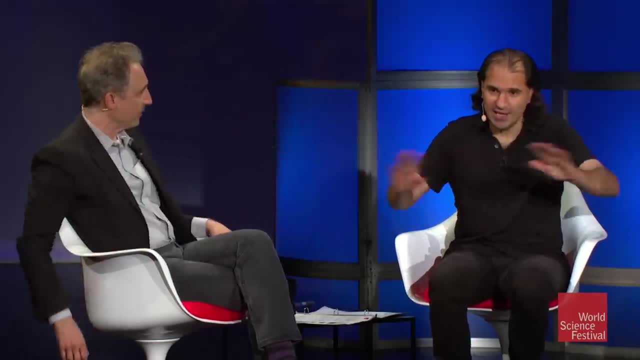 the Higgs didn't pick up a lot of mass going through all this fluctuating stuff And and and- and it's really important to stress this point- It's not inconsistent for it not to do so. We can perfectly do it. 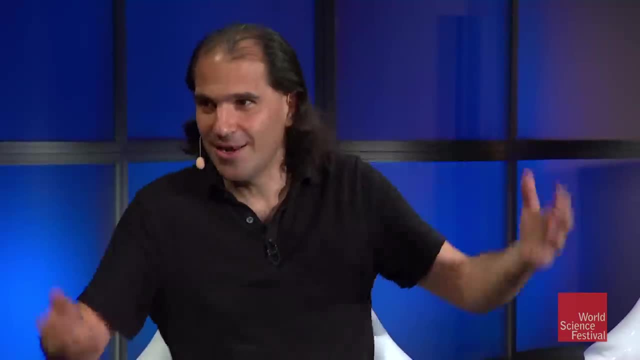 In fact we've we've done it right. Higgs did it before ever having thought about any of these things. But when you think about it more deeply, you would not expect the Higgs to be right, And in fact, 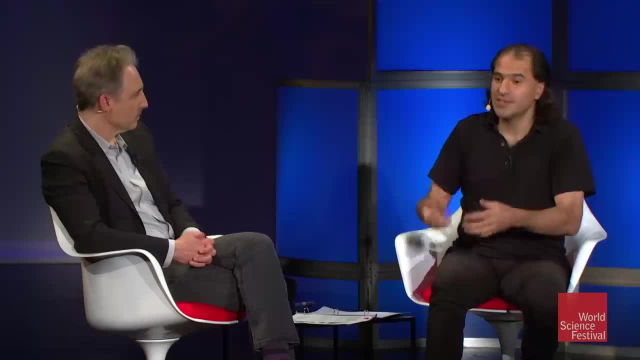 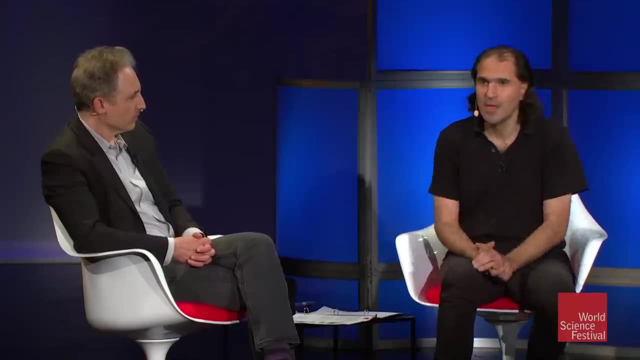 nowhere else in physics where a similar phenomenon have shown up. has something like the Higgs ever been seen or ever been been been? uh, something as simple as the Higgs been the correct explanation. Um, so if there's a mechanism, 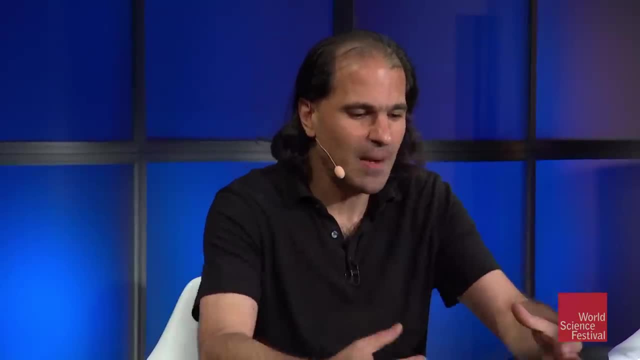 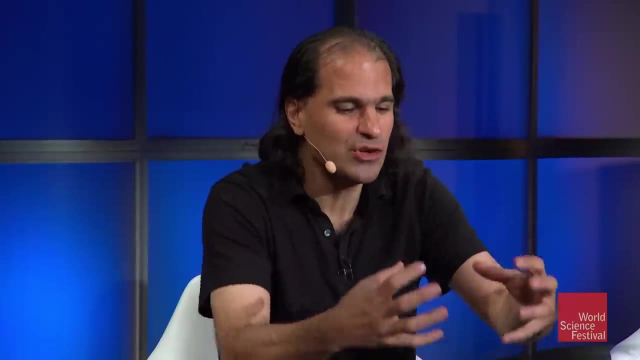 if there's a reason that we can, we can understand. uh, that shows up right around. uh, as has happened for 400 years in the history of physics. where you to to find some explanation for a phenomenon that that takes place? 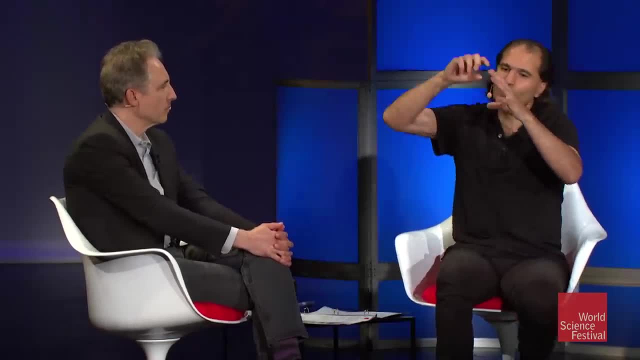 in some at some scale- You don't have to look at what's going on. you know 500 million times smaller than that scale. Yeah, That's a that has to show up sort of right around the scale of of the. 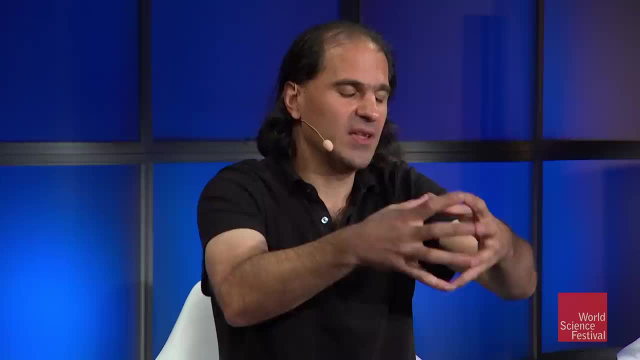 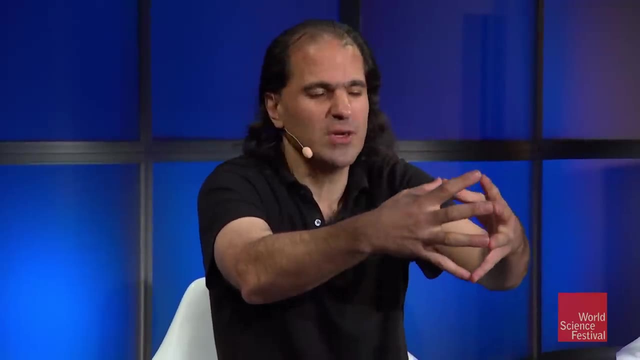 of the mystery itself, If that mystery, if the, if the origin of the mass of the Higgs was explainable in that way, that which has been the trajectory we've we've been on for centuries- essentially the reductionist paradigm. 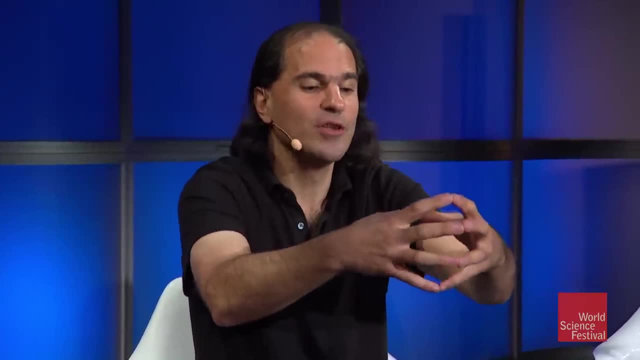 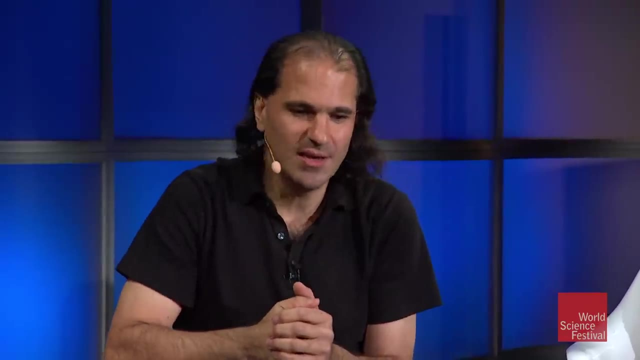 if the reductionist paradigm, uh, that we've been on for centuries holds the way it has before, then we would have expected to see something come along with the Higgs. It's like, uh, I, I've used this, uh. 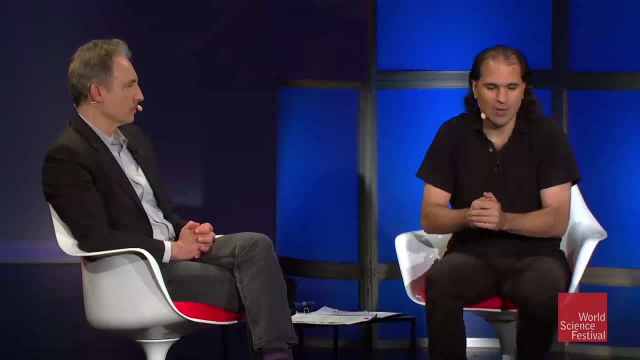 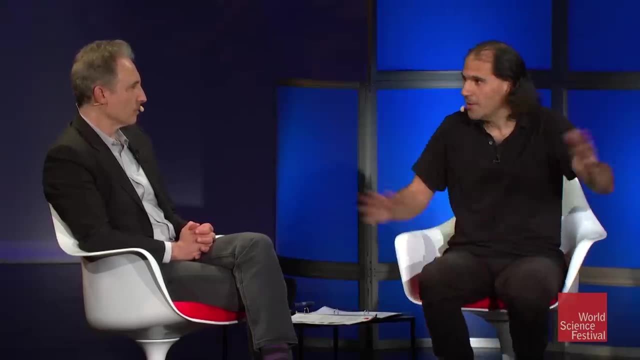 analogy. many people use this analogy. the sort of difficulty is like walking into a room and seeing and seeing a pencil standing on its tip and it's not inconsistent. It's perfectly allowed for a pencil to stand on its tip and it's okay. 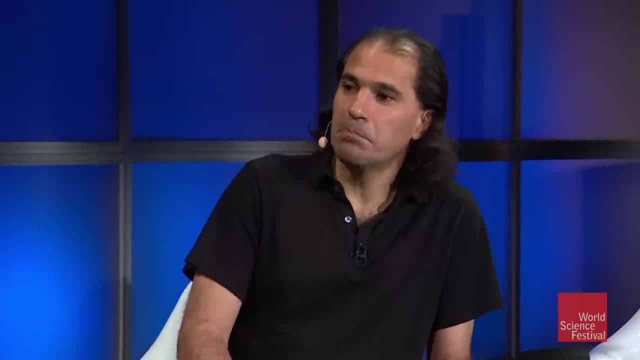 Um, it's not violating the laws of physics, but if you saw it, you would probably try to find an explanation. right, Maybe it's hanging from a string. right, There's a string hanging from the ceiling. Maybe you look. 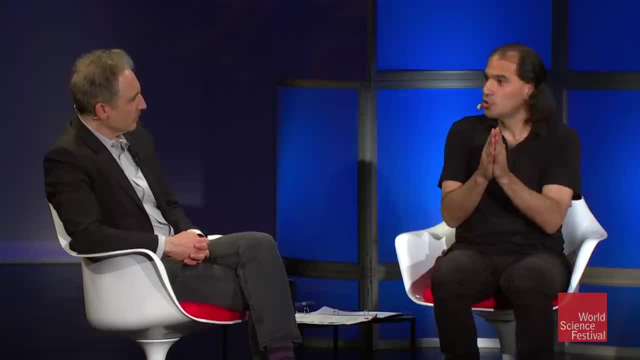 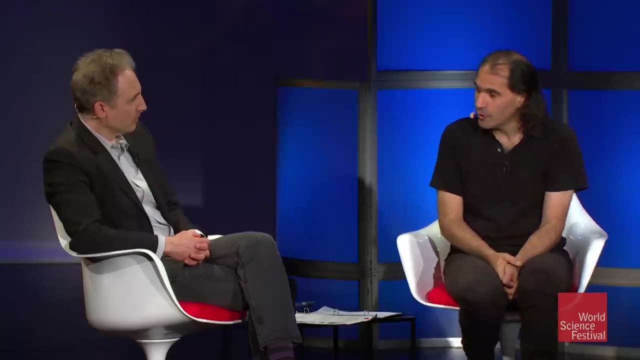 there's a little hand holding it up. right, You need to find some mechanism to to explain it, And it's that mechanism. It it? uh? supersymmetry and the other ideas that people have talked about for for decades. 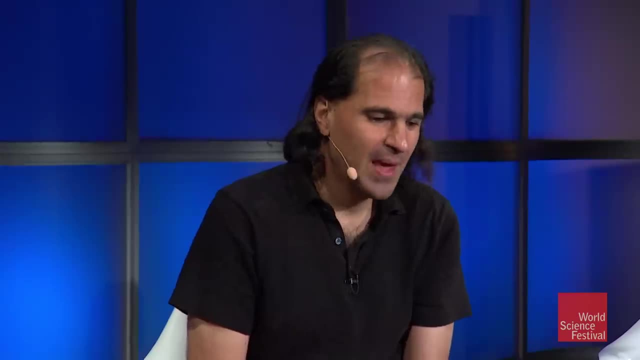 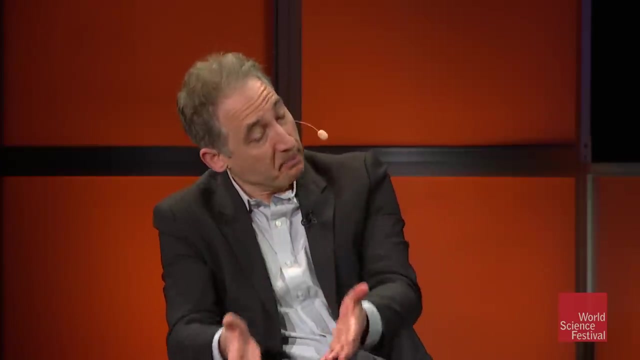 were trying to look for a hand, uh, So just to give a quick summary. so the idea is: supersymmetry provides an approach that, at least on paper, allows the mass of the Higgs to stay relatively small, like 10 or 100 times. 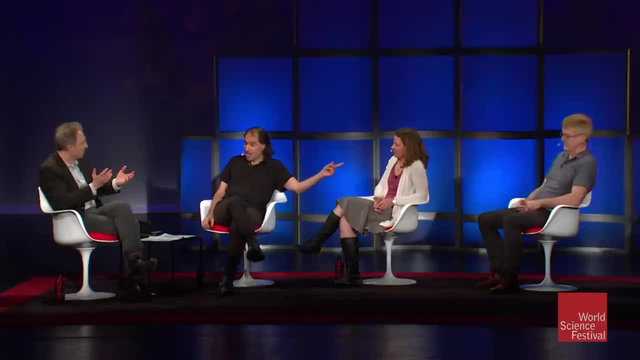 the mass of the proton, but not billions and trillions of times the mass of the proton, And in fact it's very much related to what to to, to how we were just talking about. uh, what, what supersymmetry. 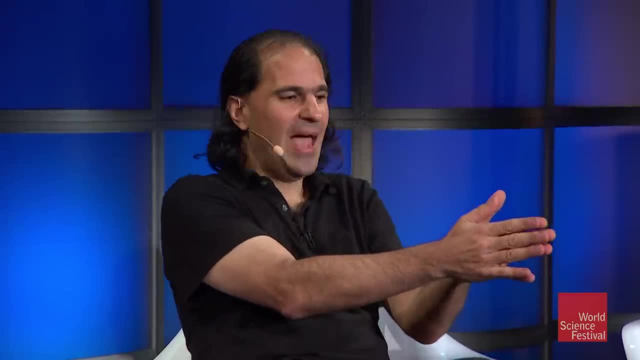 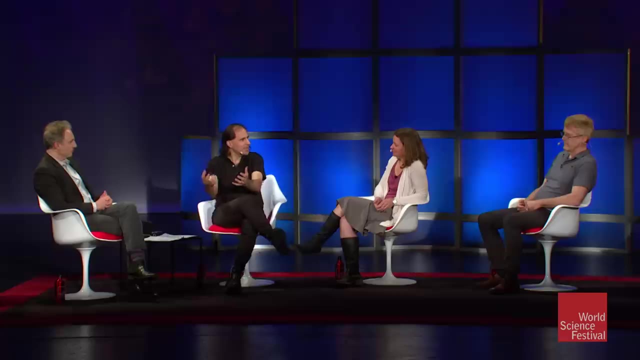 is about. You see, supersymmetry relates particles of different spin, And uh, and, and. if the particles have a spin- we have- we have no difficulty understanding their mass. That's just what we alluded to. So by relating something, 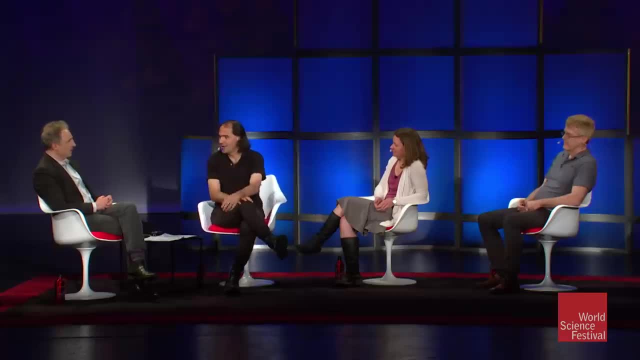 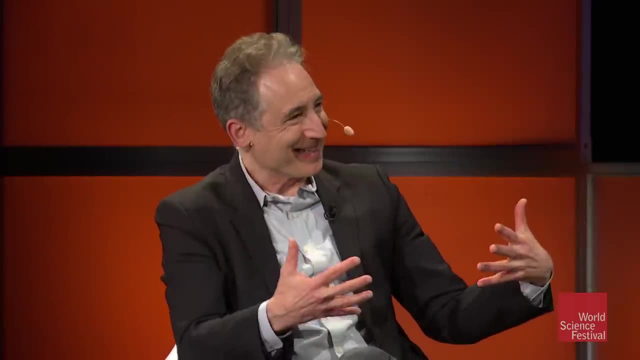 that has no spin, to something that does. we get to inherit the the clean understanding we have. So all of this gives some confidence, even if you're not willing to say it directly. but it gives some confidence that we thought that supersymmetry. 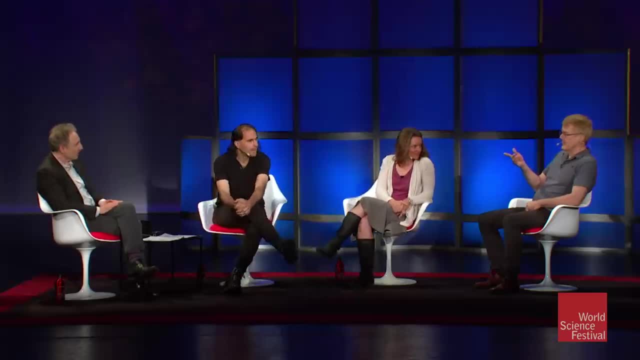 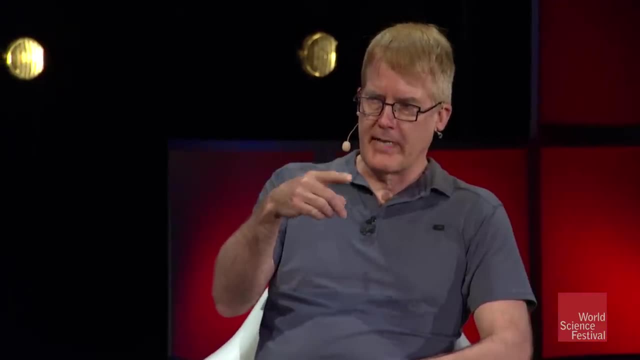 was going to be found. I mean, Joe, did you? I mean just to show how frustrating this is, at least in the simplest version of using supersymmetry to do this job, you can actually do a calculation that says the Higgs boson. 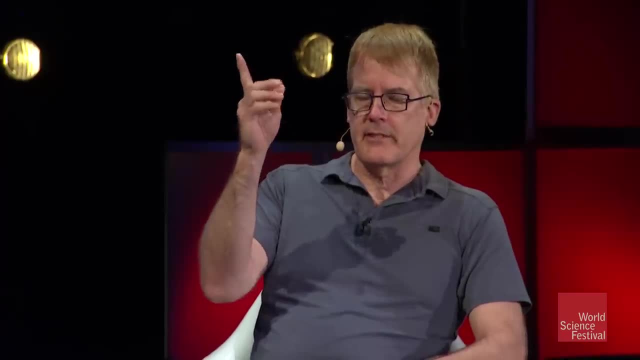 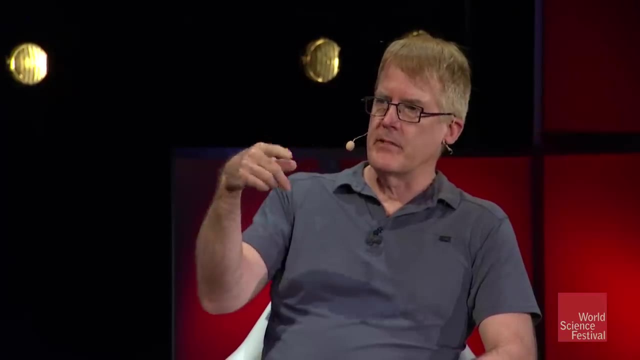 can't be heavier than a certain amount, And that amount was. this calculation was actually done by my colleague, Marcella Carino, who you saw in the clip there, And that the answer was 130 in these units that we've been using. 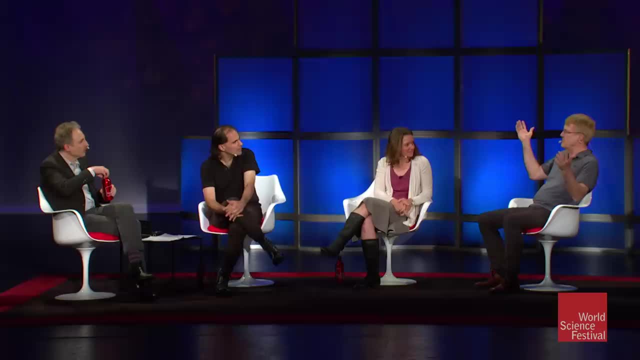 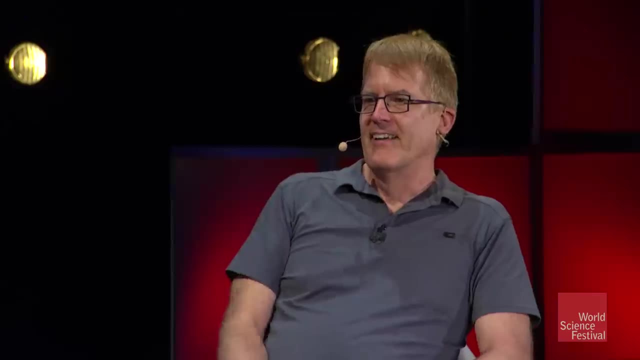 So when we found the Higgs at 125 in those units, it's like, okay, the supersymmetry must be right, It's right around the corner, right, But it's been a really big corner so far. So as we've turned, 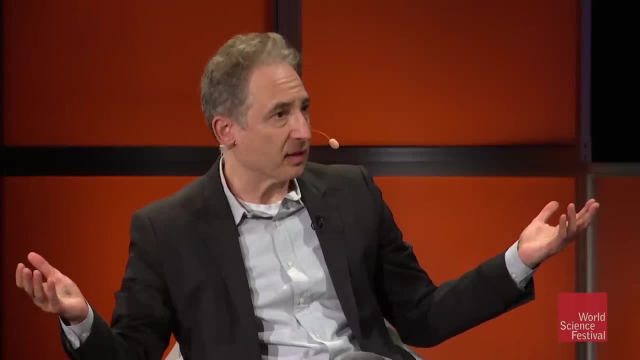 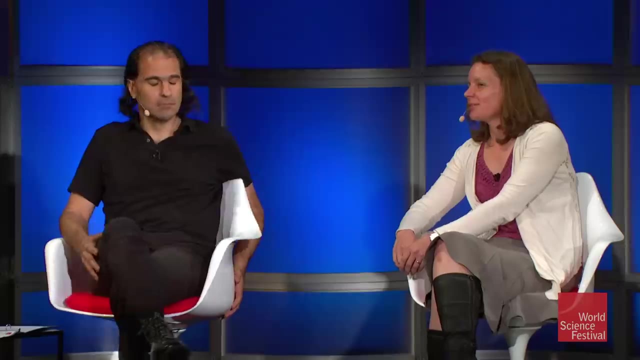 the corner. we have found. what have we found? Nothing, We found nothing. I mean certainly from the experimental community. it was a pretty heavy romance with supersymmetry, Let's be honest, because I mean from the experimental. 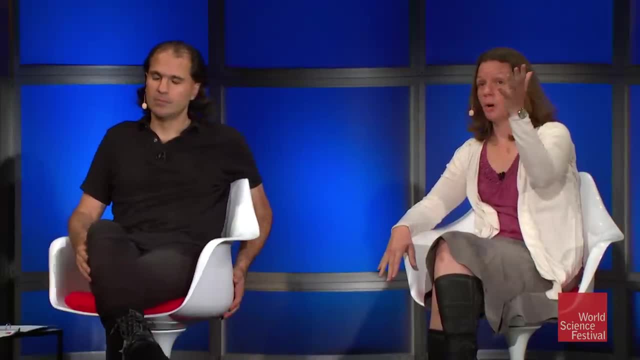 perspective. it was the experimentalist dream. I mean it was going to be one new particle for every particle that we already have. right, I mean I remember when I showed up at the LHC and I was just a very young postdoc. 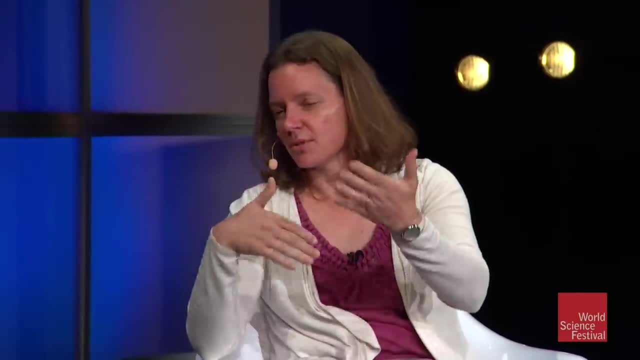 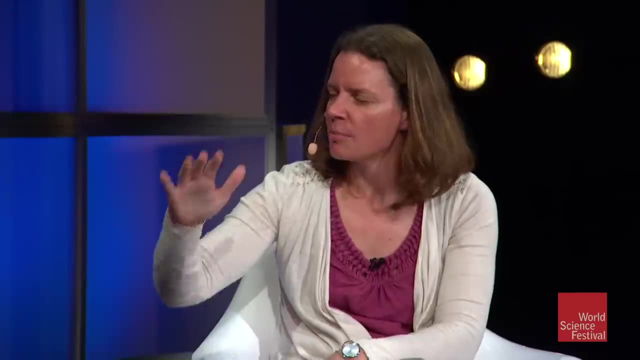 at that time and I was working on the trigger system. so the system that you know helps us keep events versus rejecting them. And I remember, you know senior physicists coming up to me and saying, like you know, you've got to be. 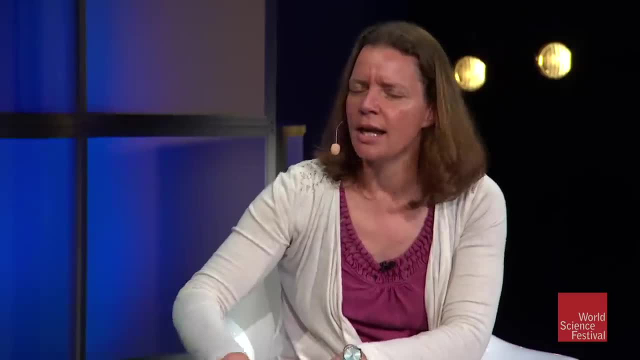 really careful. Supersymmetry is going to overload the trigger And I remember thinking to myself like I'm happy with that problem, You know, like I'm okay with that. But that was kind of the feeling, was that? 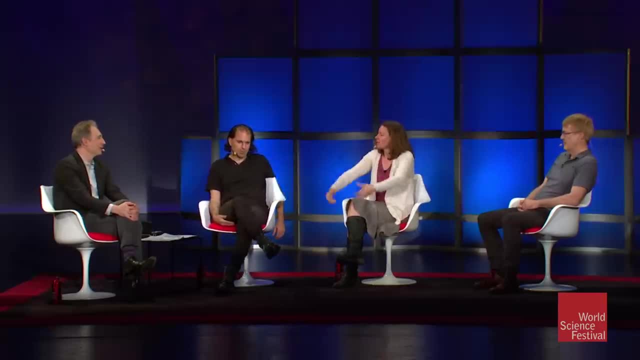 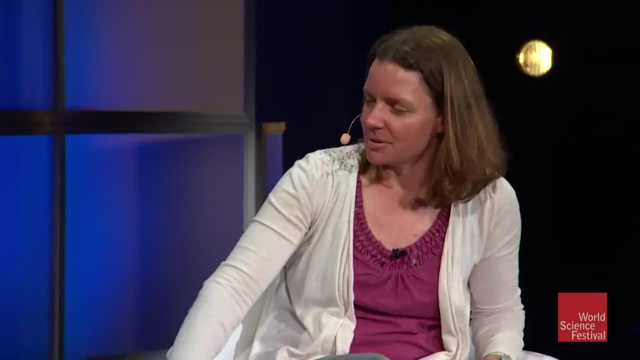 you know that this age of discovery was going to be this age of discovery again And I think that we, you know, I agree with you that I think many people, you know, there were many problems with supersymmetry, you know. 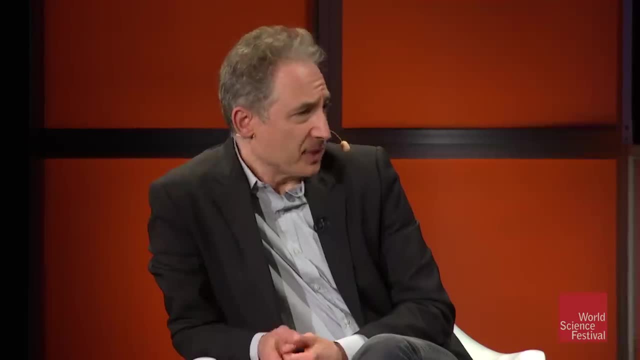 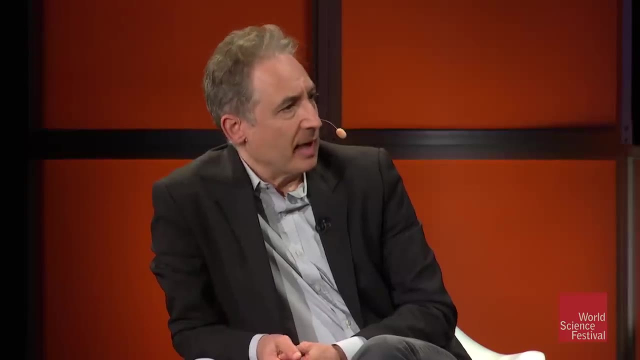 but we didn't want to hear it at the time. But even it's not just experimentalists, of course. I mean, I haven't done a calculation of it, but a significant fraction of every single paper I have ever written has supersymmetry. 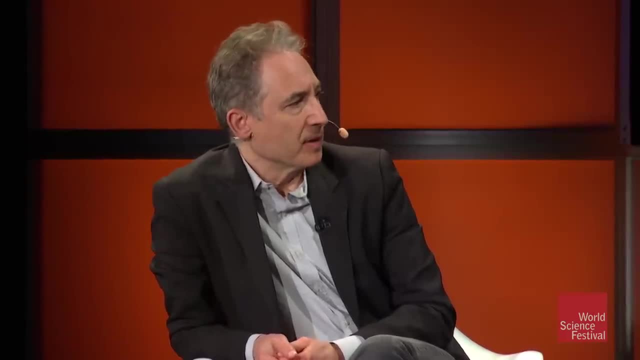 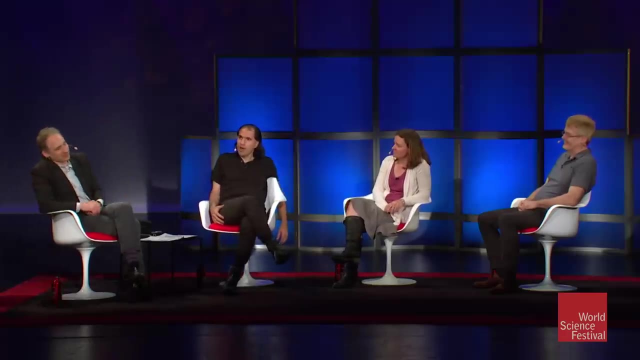 at its core The assumption that these ideas, Because it's a super deep theoretical idea, It's a very deep theoretical, mathematical idea which has driven even mathematical discovery, not even just discoveries or non-discoveries in physics. But the bottom line is: 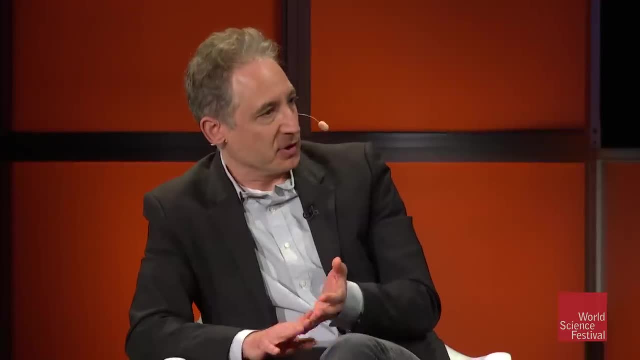 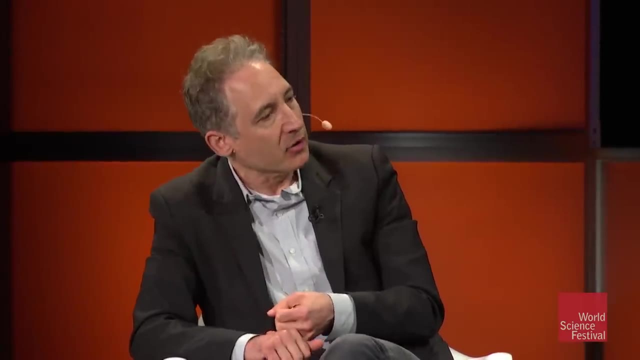 here we are sitting in 2019.. We built this massive machine in Geneva. It found the one thing that we were really certain about- the Higgs particle- and it has not found the other particles that we thought would come along for the party. 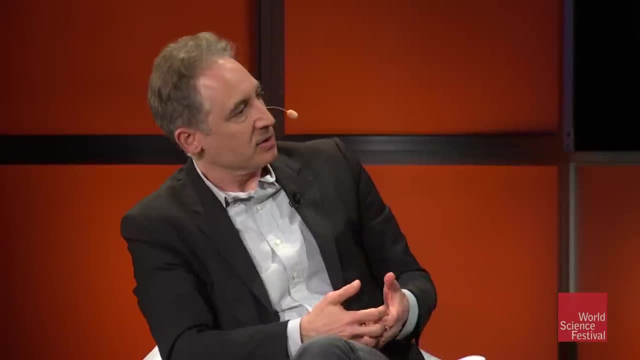 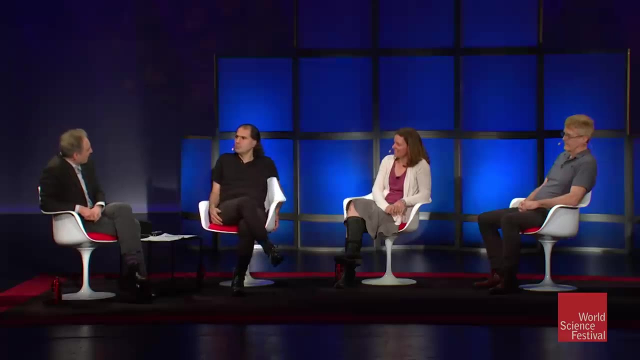 because they're so, as you've articulated, directly related to the Higgs as well as directly related to this DNA. So it's a very deep idea of symmetry. So the question is: what do we do from here? And we can continue. 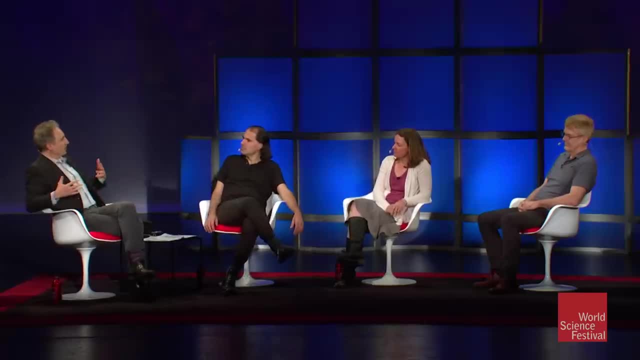 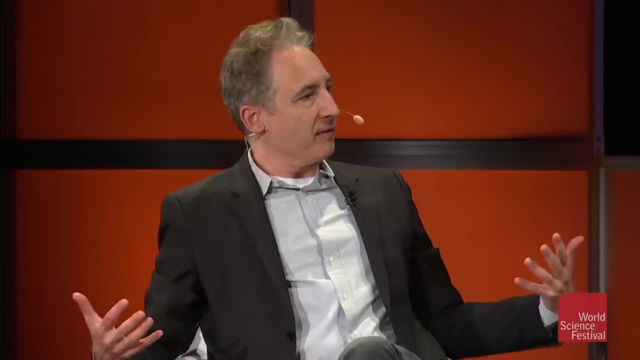 to follow our mathematics, as we will do, but at the end of the day, we're going to need data And we have to convince people to build new machines. So can you give us a sense of where we are on the frontier? 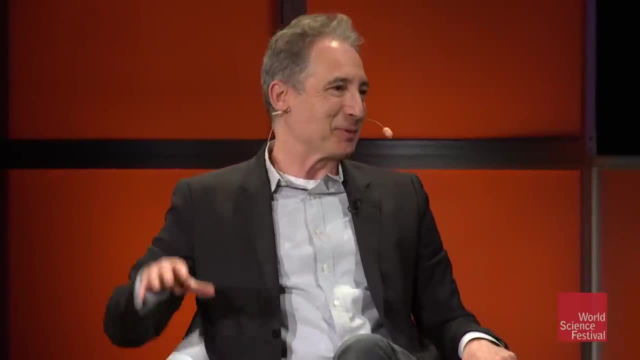 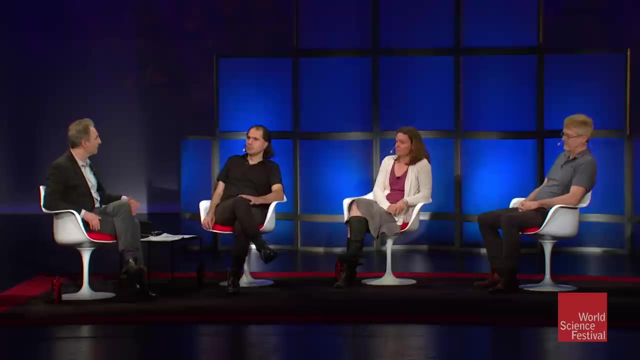 of building new machines that will have higher energy, be able to probe yet other domains, and perhaps maybe these supersymmetric particles are there, they're just heavier. So what's going on in that space? So there is, let's say. 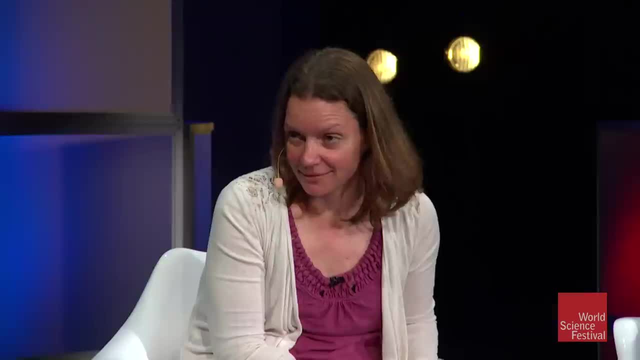 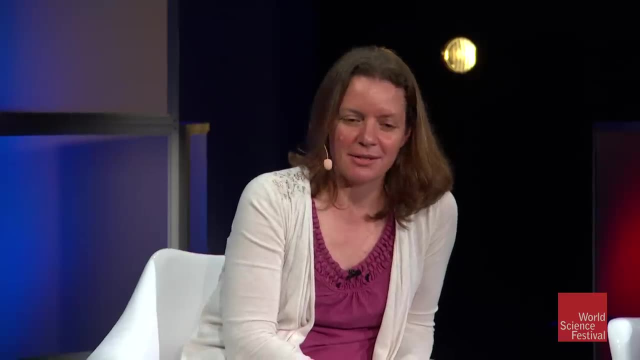 a roadmap right now, but I think there's no money yet. let's say in part of this: And there's two projects that let's say: if money was not a question, what would we do in particle physics? Well, we would build. two things. We'd build two new accelerators, one of which would be a linear collider. Japan has expressed a lot of interest in building such a collider and hosting such a collider. let's say: And this would be where you, instead of colliding, 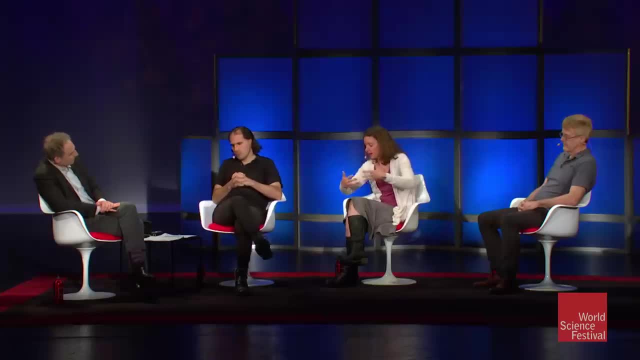 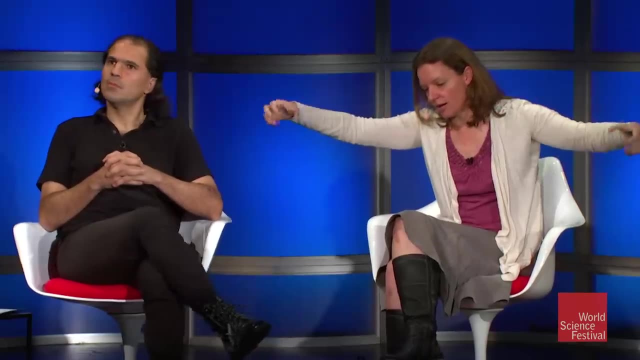 electrons and protons, you would be colliding- I'm sorry, instead of colliding protons, you'd be colliding electrons and positrons. It's a linear machine, so you've got to, it's extremely long and you basically collide them. 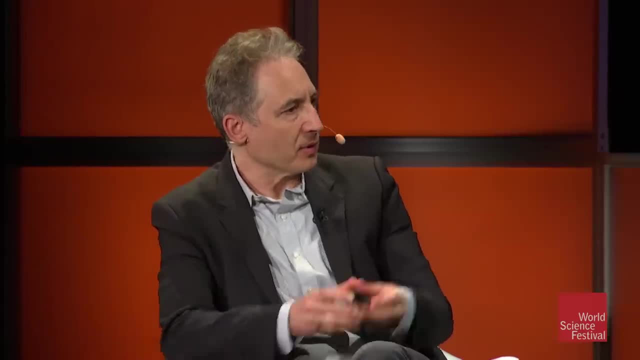 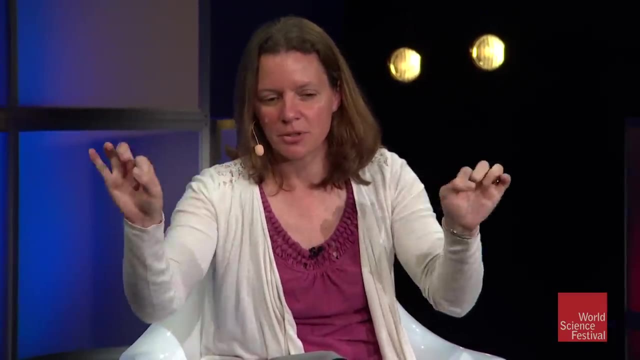 into each other, And why is it a good idea to do those particles as opposed to protons? So the advantage to electrons is that they're point-like and therefore they're just clean. The problem is when you take two protons and you smash them together. 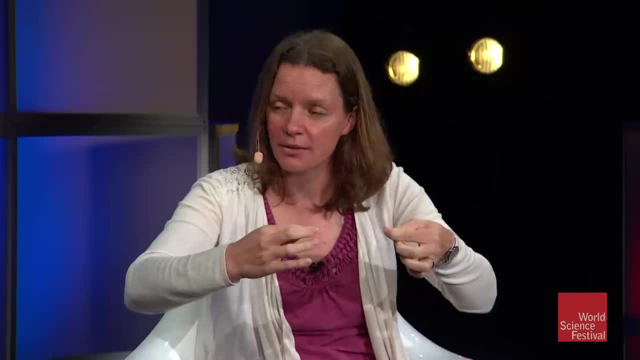 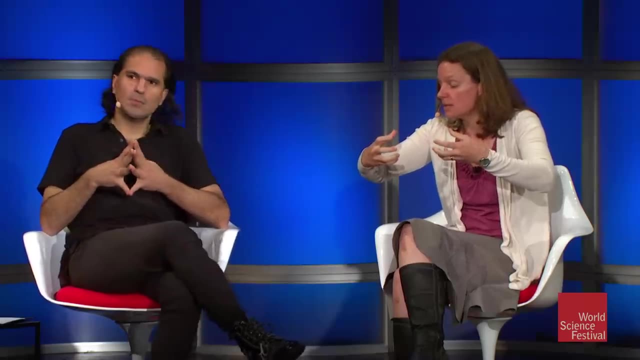 what you're doing actually is you're smashing two quarks from inside those protons, But the actual how much energy those quarks have inside the proton is very difficult to model. And then on top of that you've got the rest of the proton. 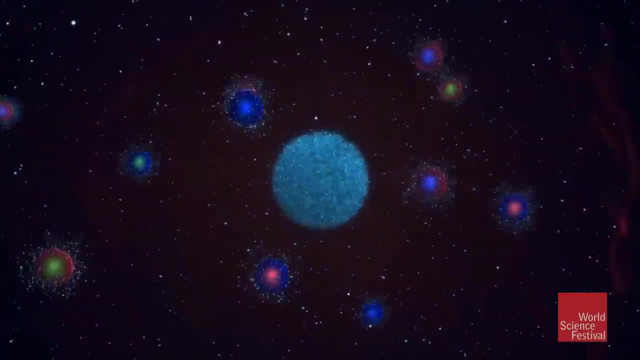 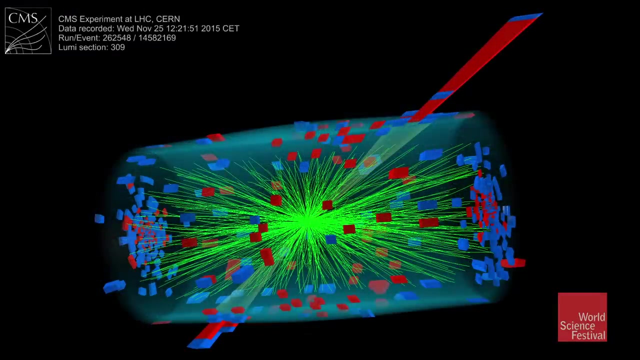 that breaks up and it just leaves a huge amount of mess. If you look at pictures- I think we have some pictures of what a collision looks like, for example in one of the detectors- you'll see there's just huge amounts of particles. 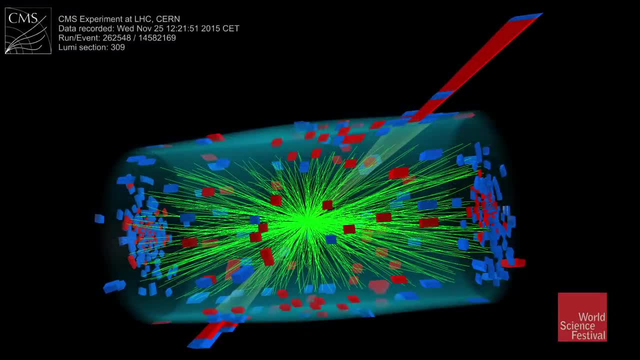 coming out Like we see here, Like what you see here. So here, in this event, you actually only have two particles that you're actually interested in. This would be kind of what you kind of see with these big red-blue clusters of energy. 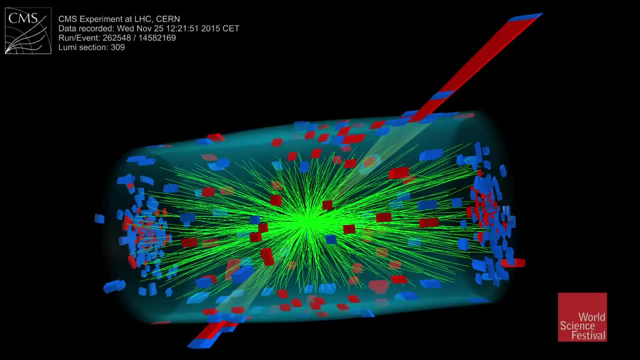 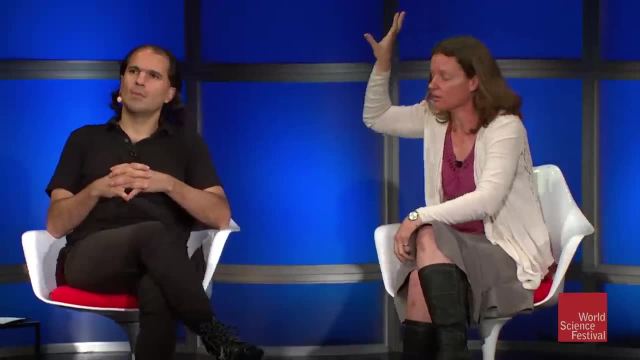 Those would be the two particles that you're interested in, And these are tracks, And these are all. the green is all tracks of particles and so forth and so on, And most of this is just crap from the rest. That's a technical term. 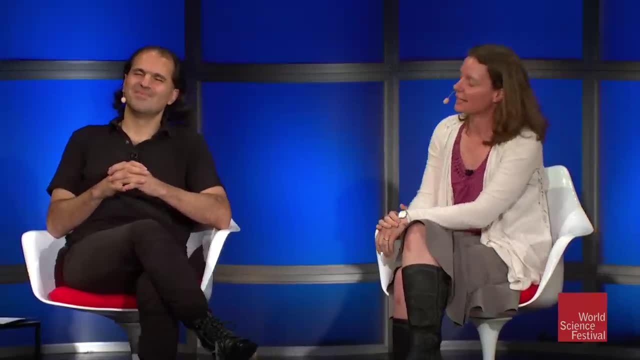 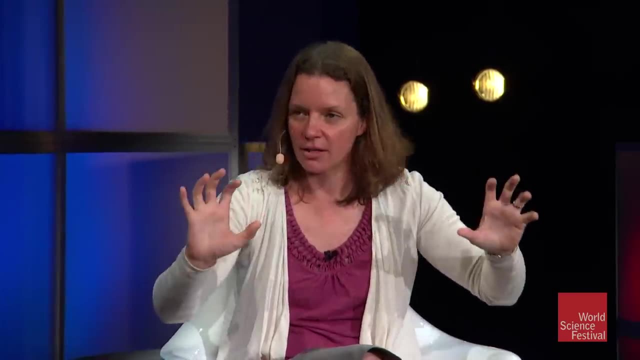 Yeah, that's actually, that is the technical. We use that a lot in publications. Yeah, good, Yeah. So you know, that's just the crap that comes, And in an electron positron collision, everything's clean. 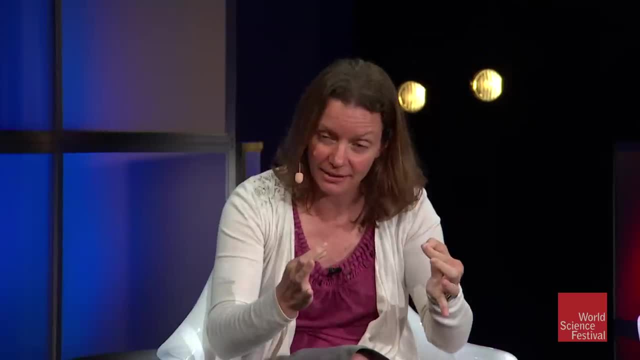 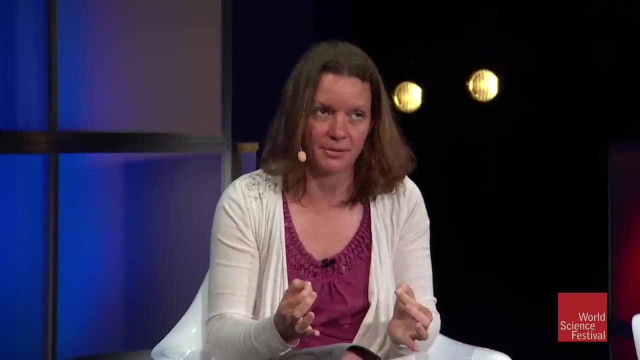 You don't have this breakup of the and you know exactly what the electron is, What the energy is. So, from a precision measurement perspective, it's superior, Right, Absolutely superior. However, if you want to really go high energies. 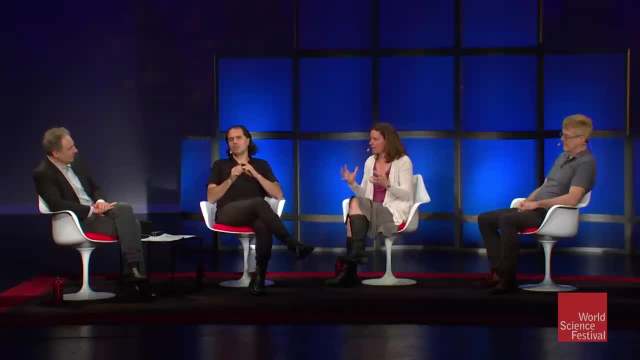 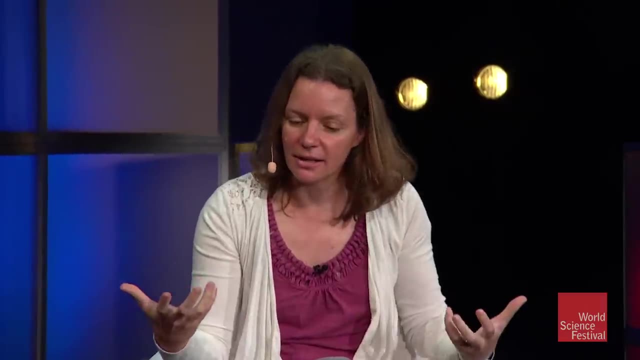 then you've got to go protons. Protons are what gives you your power in terms of the energy aspect, And so, in addition to a linear collider in the ideal world is what we would have. So we'd have an ideal, a linear collider. 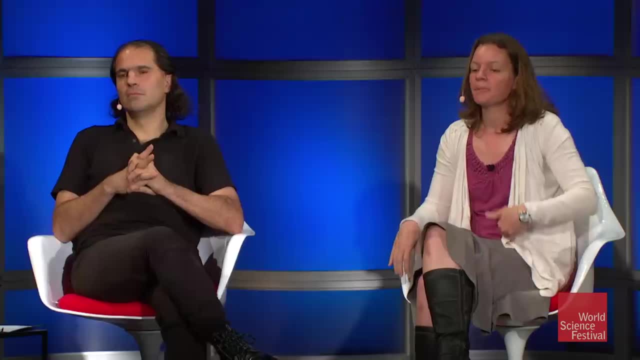 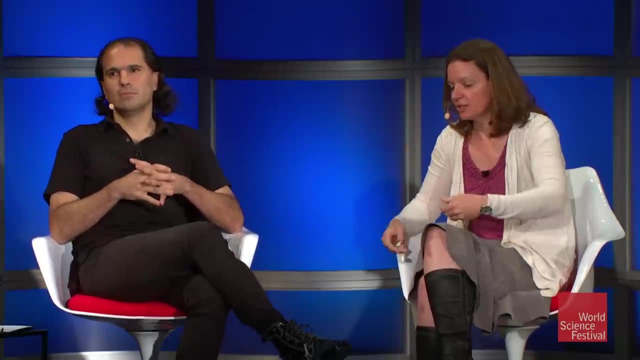 to really measure top and Higgs extremely precisely, And then, in the ideal world, you would have another hadron collider, which was, you know the well, the next generation, the FCC, Future Circular Collider, or there's also. 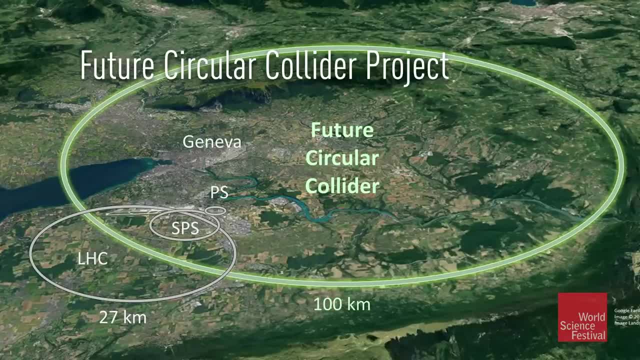 And where might that be? And that would be at CERN. This is a picture of what it looks like. It's actually very it would be a hundred kilometer ring. So the LHC just pointed out it's clear up there. 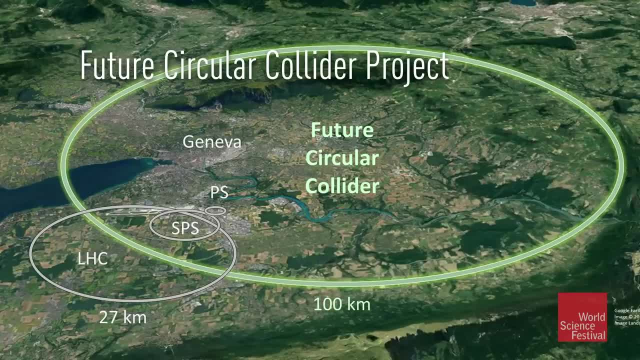 but just pointed out. Yeah, the LHC is a smaller ring here, And what's actually interesting about the circular collider is that God apparently put mountain ranges exactly perfectly, such that you could build such a tunnel. it would have to go underneath Lake Geneva. 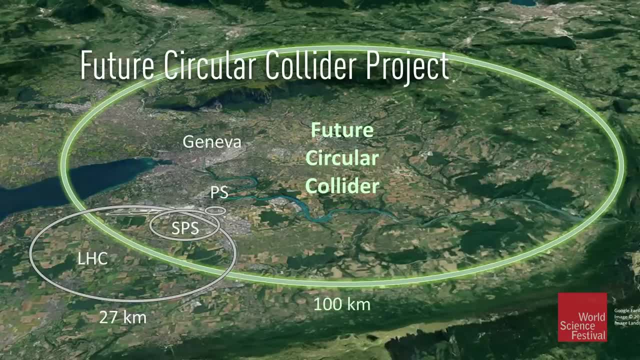 and it would just pass right through there. It would pass right before the Alps, pass right before the Seleve coming back, So it's just perfect. Going under the lake is actually not a problem. Everyone always asks about going underneath the lake. 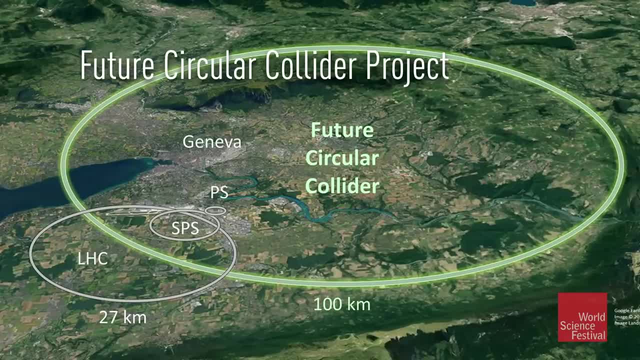 But you know the thing about a lake, because I always worry that there's going to be a leak. you know, the thing about a lake is that there's never a leak in the lake, because if there was, you wouldn't have a lake. 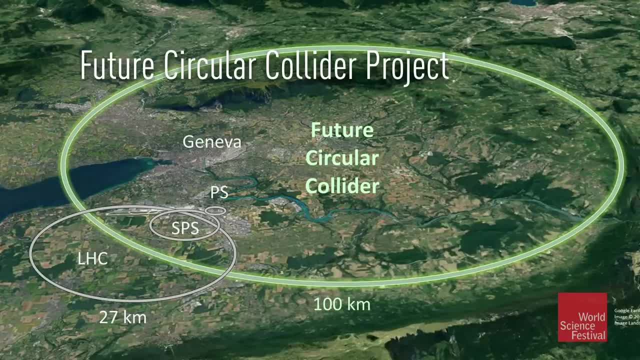 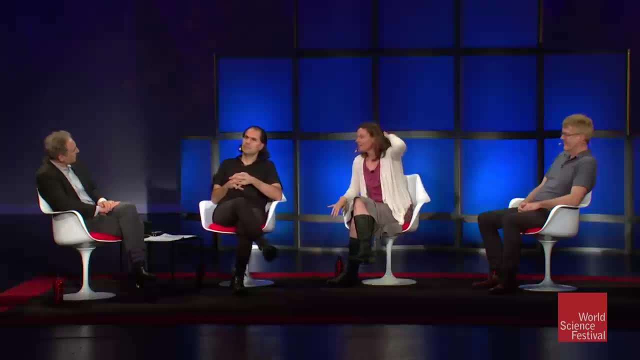 So going underneath, Going underneath the lake, is no problem, but it is a problem in the sense that you do have mountains, and mountains lead to a lot of water drain. What would the energy scale of that machine be? So this would be gosh. 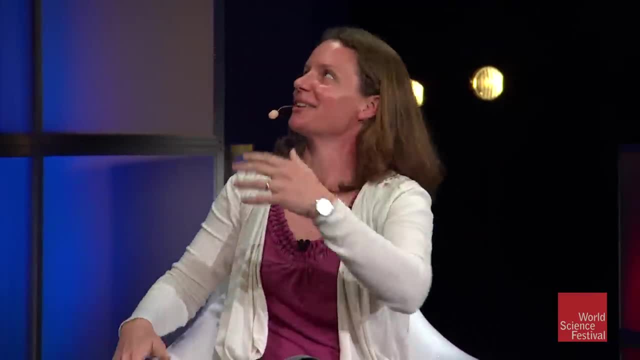 it's 100.. 100 TeV. I suddenly threw a blank there. I saw the 100 kilometers and I thought yeah, it's a 100 TeV machine. So it's roughly not quite, but maybe eight times. Eight times what we have now. The LHC here was 14, and then you had the Temetron, which was lower, And so this would be your real discovery machine right, which would be: you go out to 100 TeV and you would. 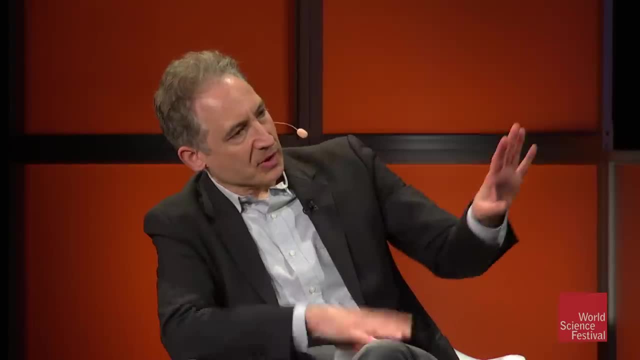 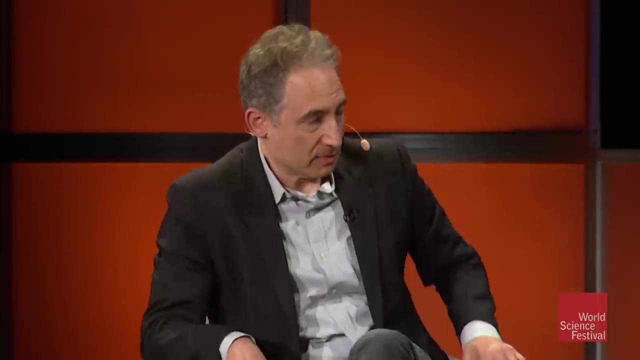 you know, again, it would be proton, proton. But, Joe, let me ask you a question, Just so we have the information, I'll put those numbers up there. So Nima was describing how the energy scale that the Higgs was at. 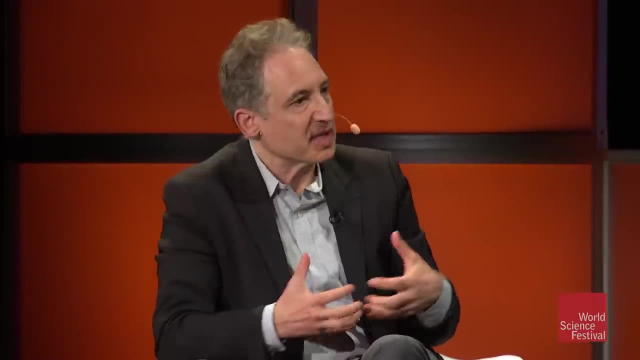 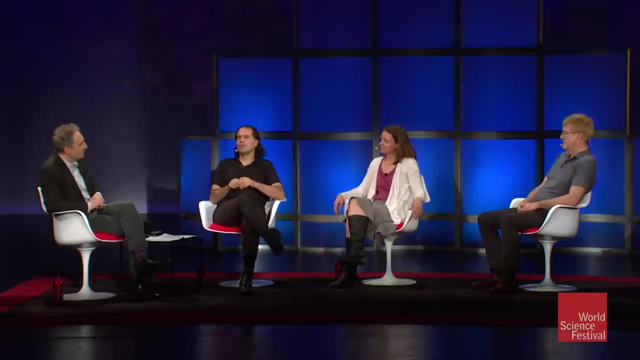 and supersymmetry and its most conventional formulation. it all seemed to come together. It was all happening at the right energy scale. Now, when we go, say, from 14,000 times, you know the mass of the or you know. 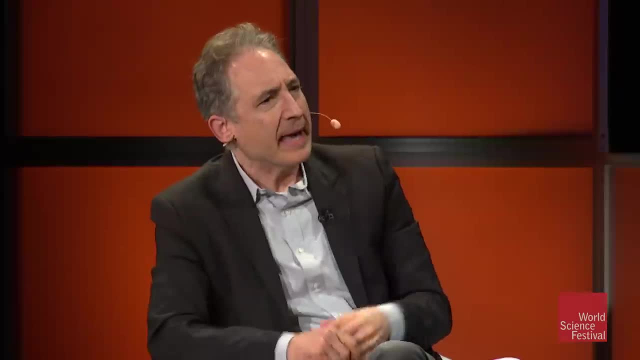 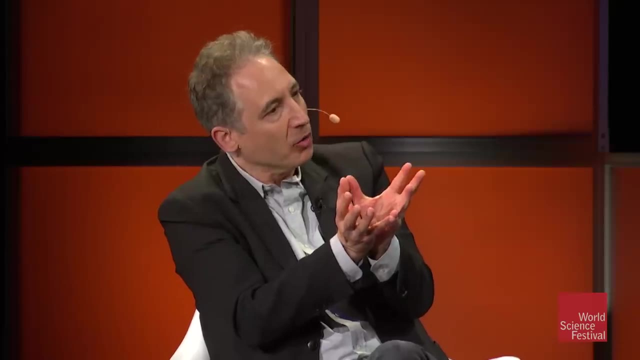 14 TeV to 100 TeV, a factor of eight in there. is there theoretical motivation that that particular slice of energy space is going to really hold something new? or are we just simply saying let's go bigger because we haven't found anything yet? Well, of course it's a combination of those things, because there's never a guarantee that any particular collider is going to discover anything. We didn't know that the LHC would discover anything, So you're always making a gamble. But there is motivation. 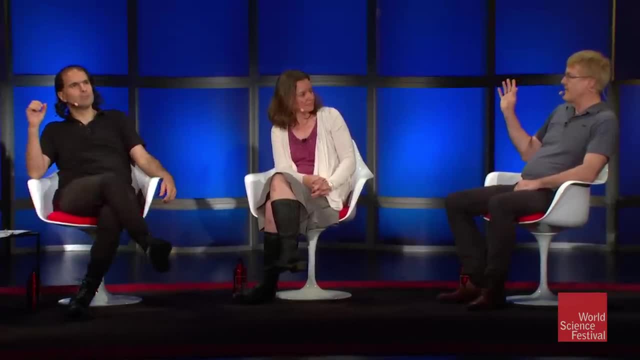 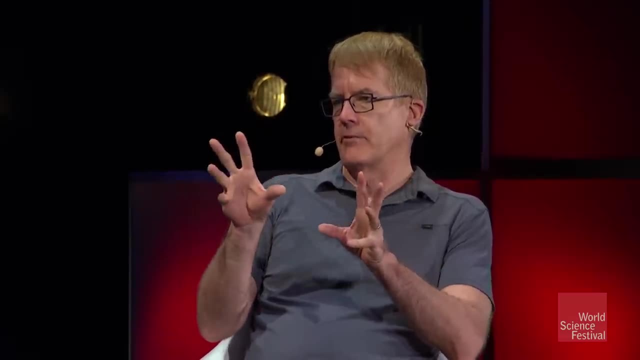 that if the ideas that we've been talking about have any validity at all, if they're not totally wrong, that maybe what we're missing is we didn't quite have a powerful enough tool to see them, And you know what's the probability of that? 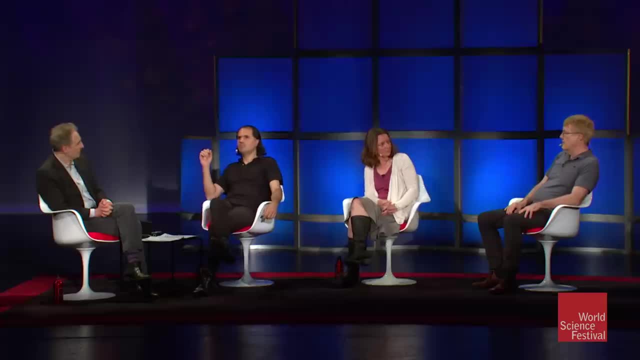 Nobody knows. This is why it's discovery science. You're always taking risks, And Nima can, And you've been actually making an argument to build a new machine- not in China, if I'm mistaken. Yeah, I mean, let me just say 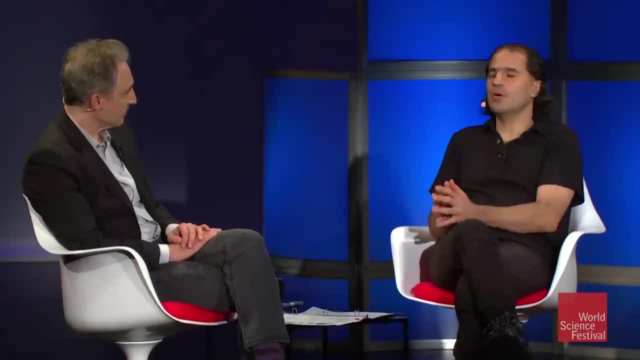 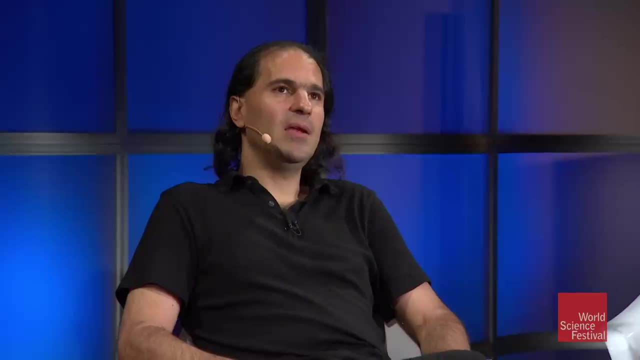 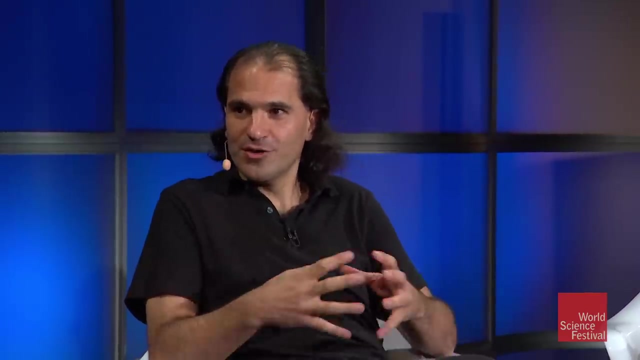 a few broad points. I mean, first of all, we go to the frontier because it's the frontier, So that's the zeroth order thing. But I think, if you think that particle physics is about, uh, discovering new particles, and so you're only 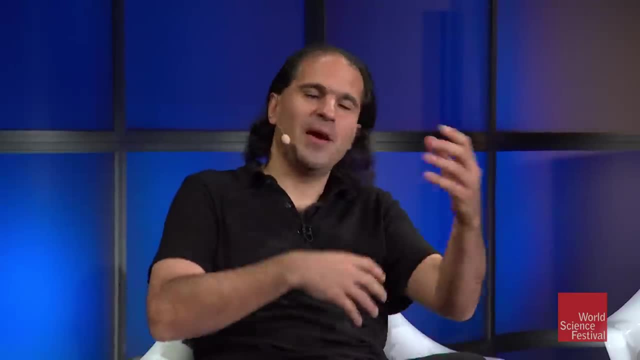 going to build a machine. if you know for a fact you're going to discover a new particle and you have some idea where it's going to be and so on, then this is a perfectly good time to take your ball and go home and do something else. 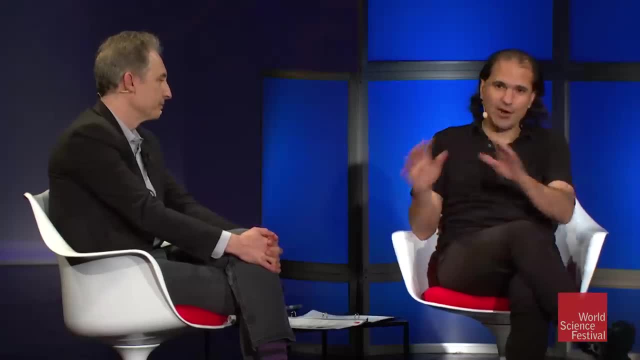 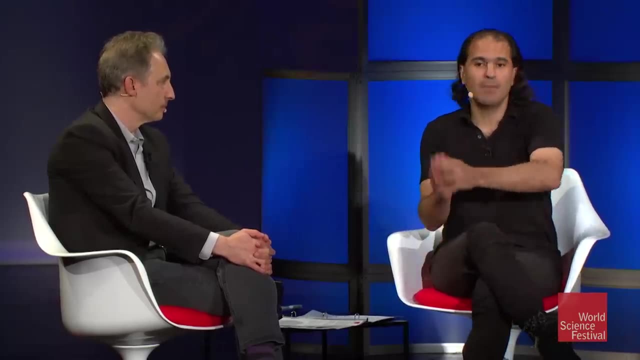 with your life. Okay, Because we have absolutely no guarantee- I cannot stress this enough- absolutely zero guarantee that a new machine is going to produce a new particle. There are some indications for a new phenomenon that would happen at scales. you know, having to do 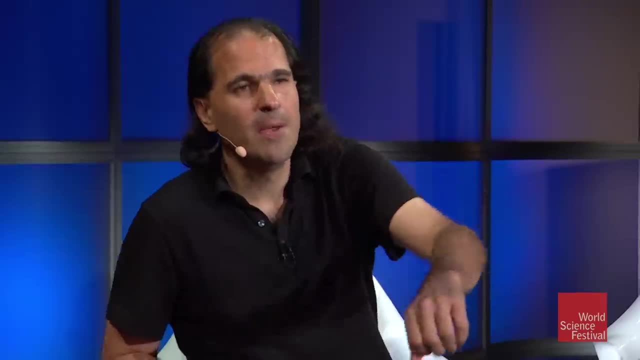 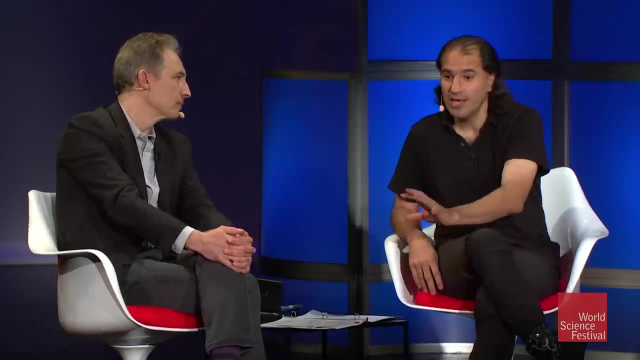 with gravity and things like that, orders and orders of magnitude removed from where we are. But we had lots of theoretical arguments that something should happen right around the scale of the LHC. We haven't seen them, And there were in any case. 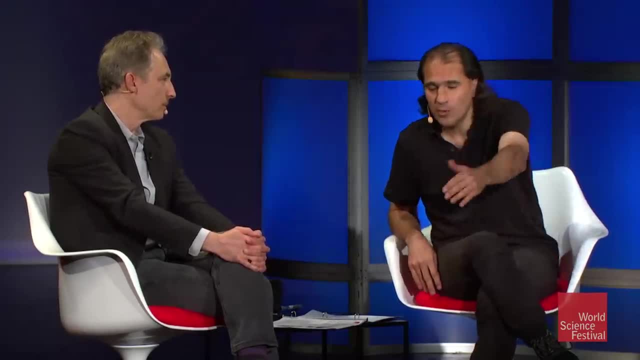 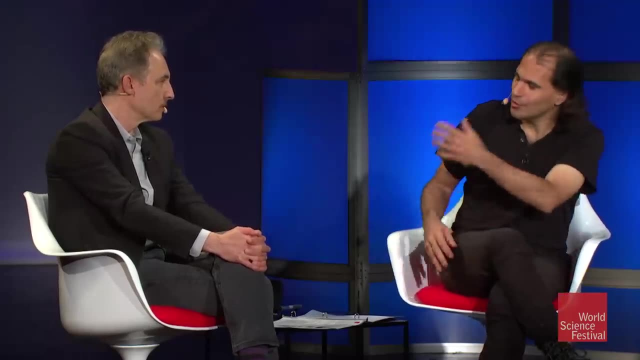 there were circumstantial, indirect arguments anyway, So we there's no guarantee that there are new particles. However, this entire- and this is why I alluded to this earlier when we were talking about the building blocks of matter- picture of the world. 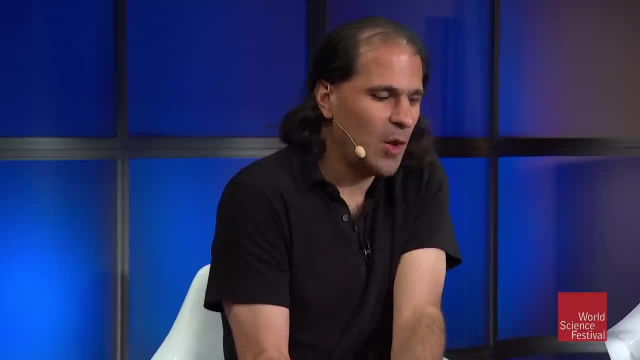 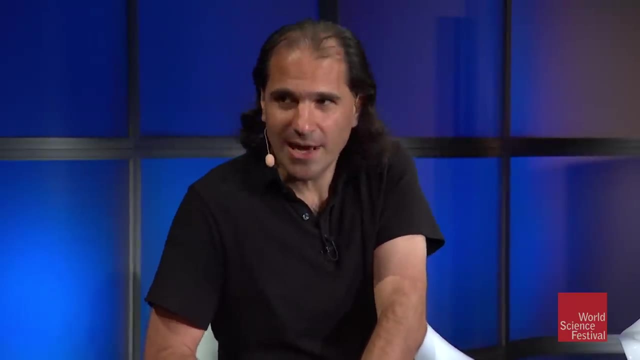 it's maybe a little funny. This is certainly not what drew me personally into fundamental physics. I don't care that much about the building blocks of matter. It's a lot like chemistry. I sucked very badly at chemistry in school And I don't care that much. 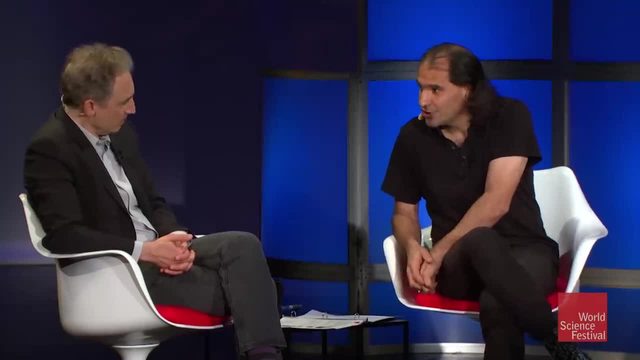 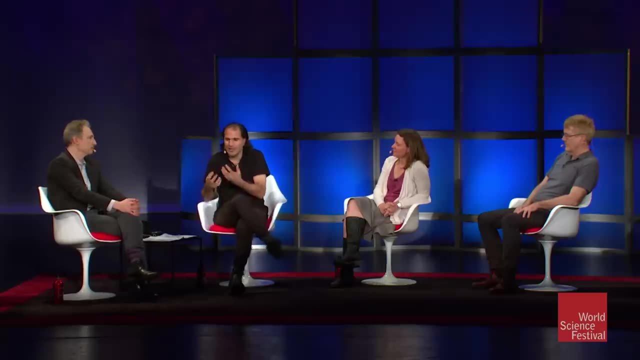 about the building blocks of matter. I care about the structure of the fundamental laws of nature And we've learned that the elementary particles are the letters of the novel that we're interested in the novel, We're interested in the structure of the laws of nature. 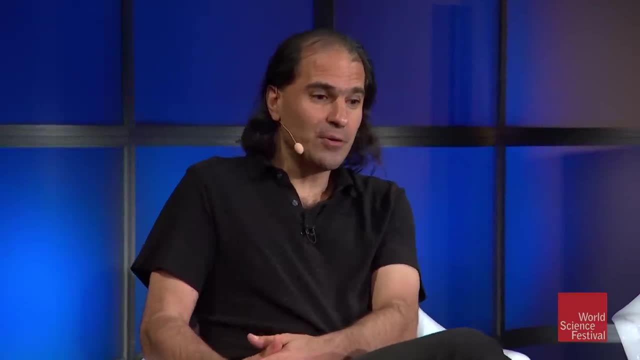 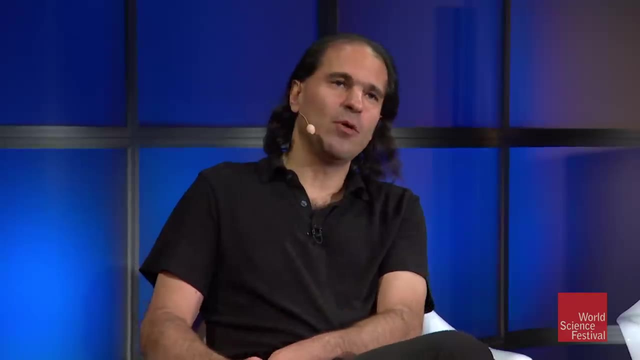 And there what we really care about are new principles, new phenomenon, And from that point of view the Higgs is damn new. It's very strange, We've never seen anything like it before, And so I think the main to me 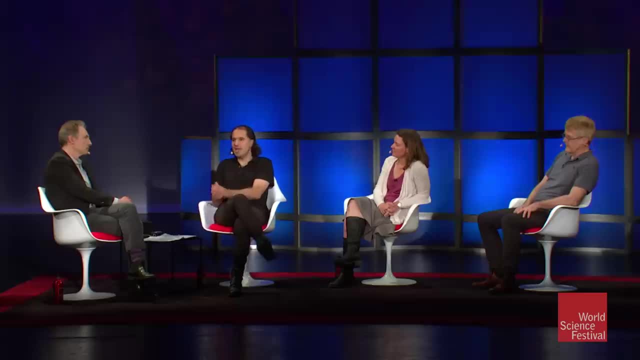 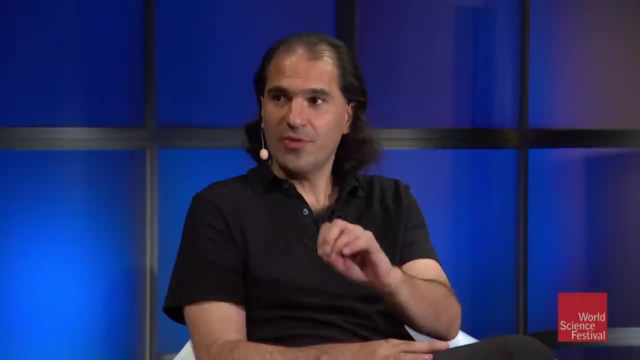 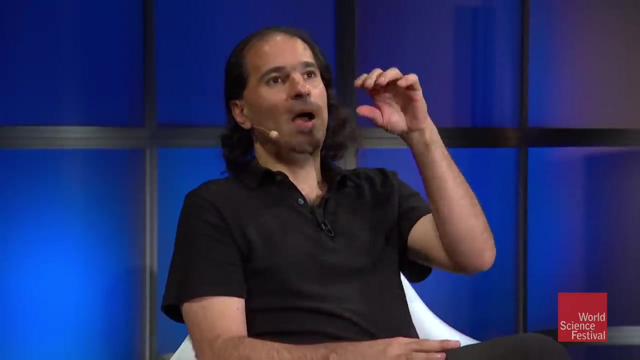 and, I think, to most people proposing these future machines. the main thing we'll learn for sure from doing these new experiments are fundamental facts about the Higgs. We've never seen an elementary particle like the Higgs before. We have to put it under a very powerful microscope. 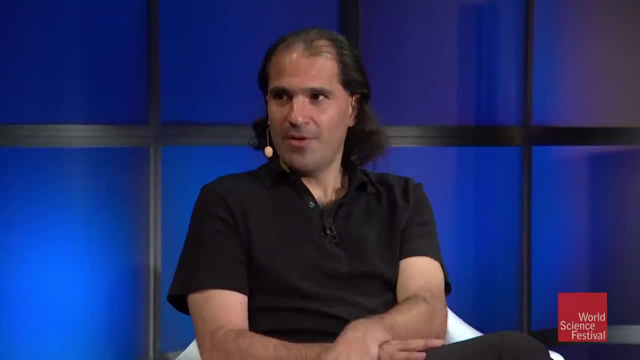 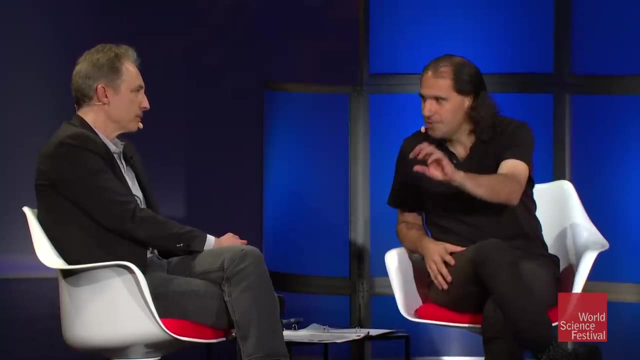 more powerful microscope than we have at the LHC, And the main drama about the Higgs is whether it really looks elementary or not, Whether it really looks point-like or not. From the LHC we're going to get a pretty fuzzy picture. 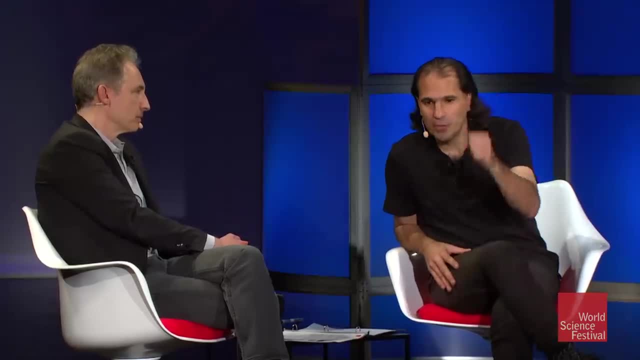 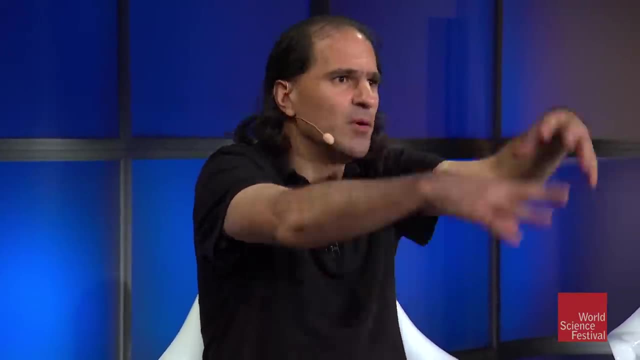 of how point-like the Higgs looks. You really have to put it under, And in fact it's fuzzy enough that we've seen roughly analogous things to it elsewhere in particle physics. Most of you probably haven't heard of this particle. There's a very important 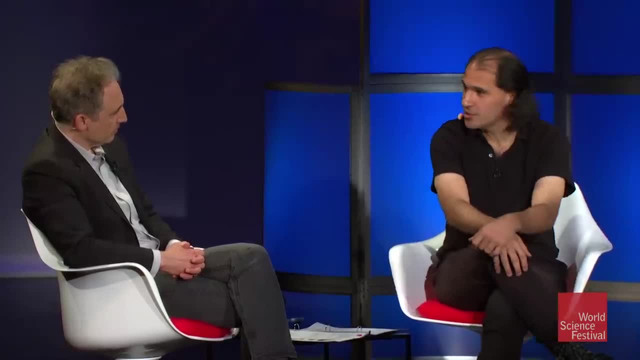 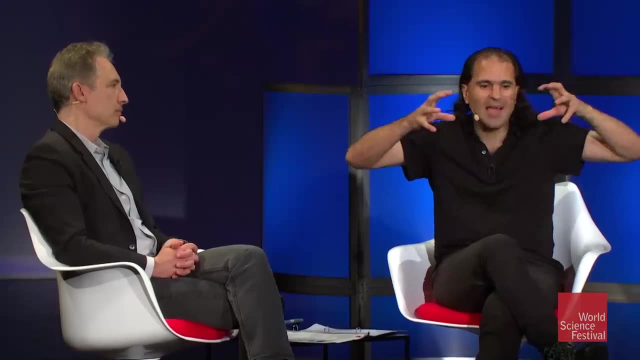 particle known as the pion, that also at first blush looks like it might be kind of an elementary particle of spin zero. But very quickly you see that when you just put it under a magnifying glass with magnification five you see that it's actually. 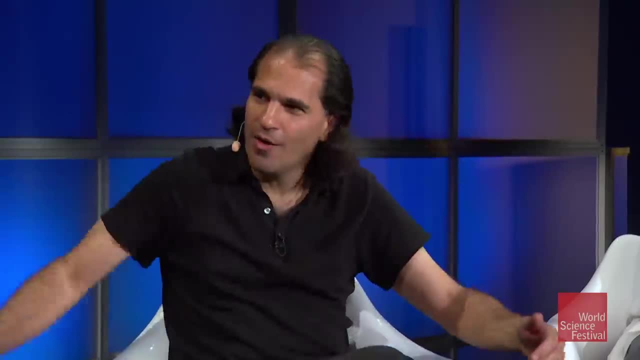 made up out of little quarks held together with gluons. So, phew, all the theoretical drama that could have been there with the Higgs was actually not there with the pion. Well, that's the resolution we're going to get on the Higgs. 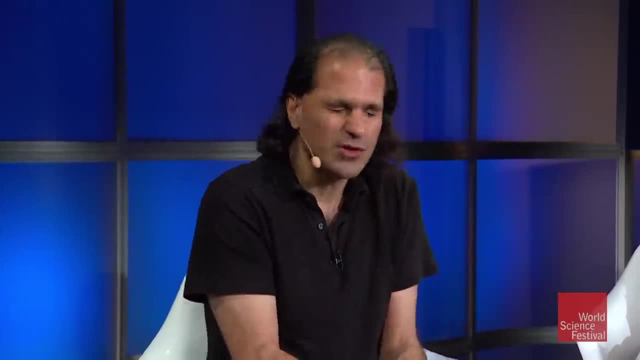 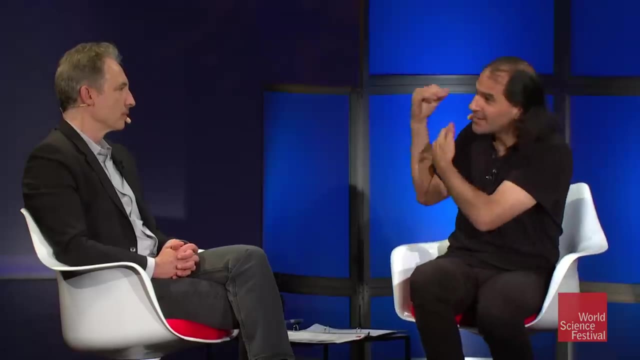 from the LHC, More or less that same kind of factor of five resolution that we had with the pion. We need another factor of 10 on top of that to know if it's something really, really new, if it's point-like, as we expect. 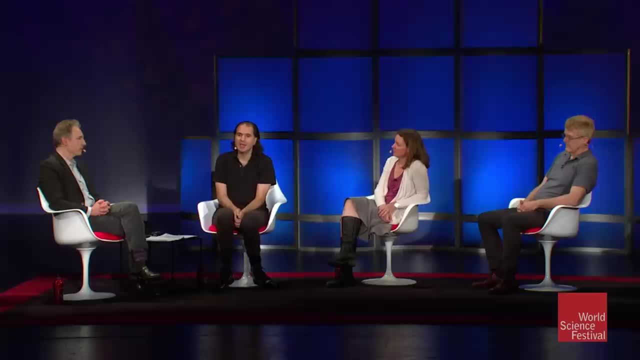 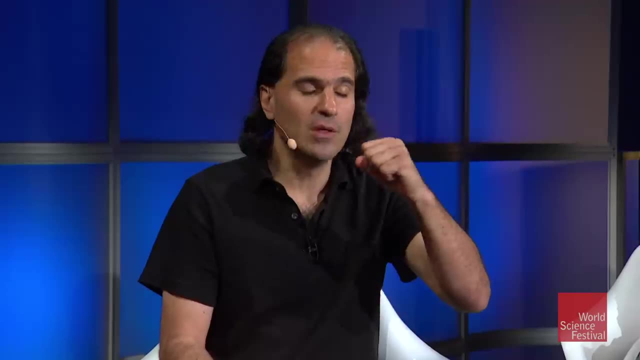 actually in the standard model or if it has some substructure. And so there are two kinds of experiments that we can do. One of them is to see whether it looks point-like to other things. Like, if you literally want to see that it looks point-like. 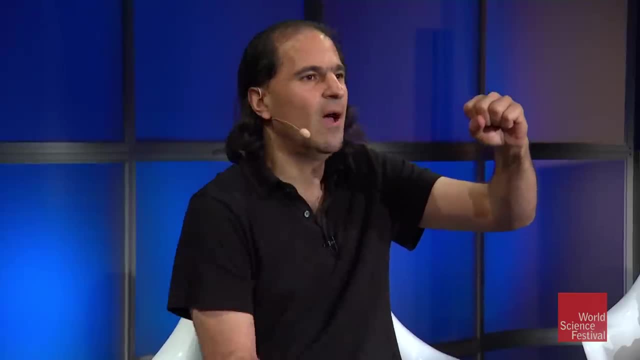 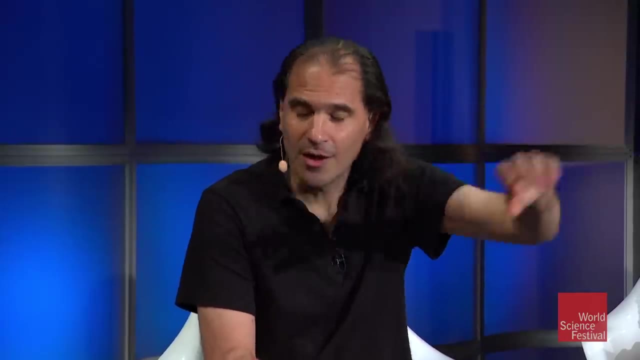 you want to see what happens when a photon bounces in into the Higgs. Of course the Higgs doesn't actually live very long. So equivalently, you look at what happens when a Higgs decays to two photons or into other things. 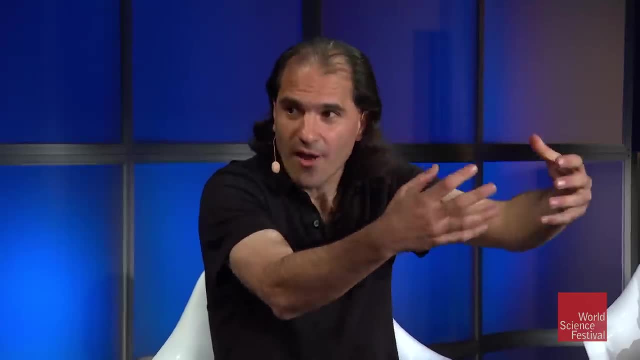 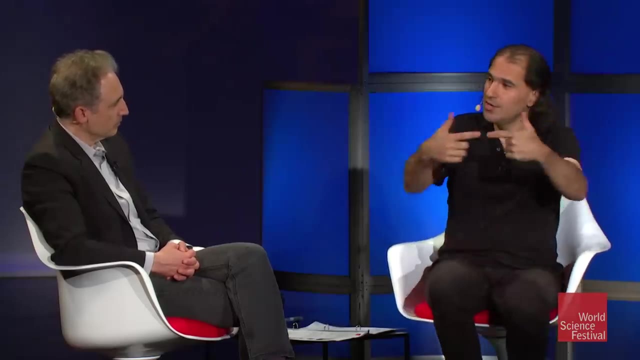 And then you see whether that interaction of the Higgs with other stuff is compatible with the Higgs looking point-like. That's what these so-called Higgs factories will do. The linear machine that Monica was talking about is a great machine to do this. 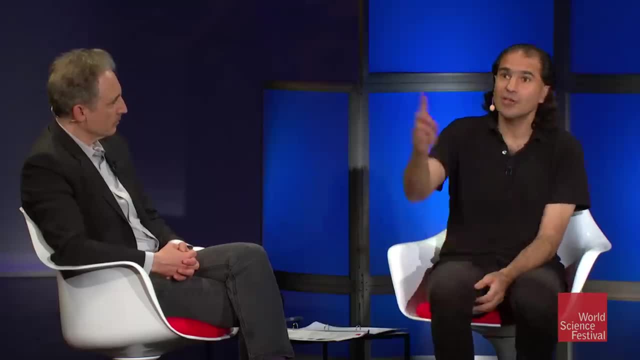 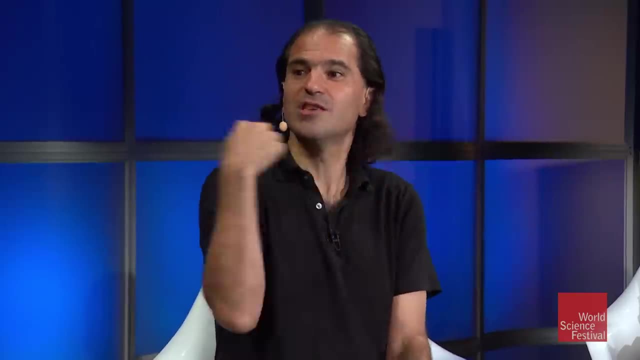 It would produce millions of Higgs particles in a very clean environment. Actually, these circular 100 kilometer machines could do exactly the same thing if you collide in them: the same electrons and positrons. So that's one of the great things about these circular machines. 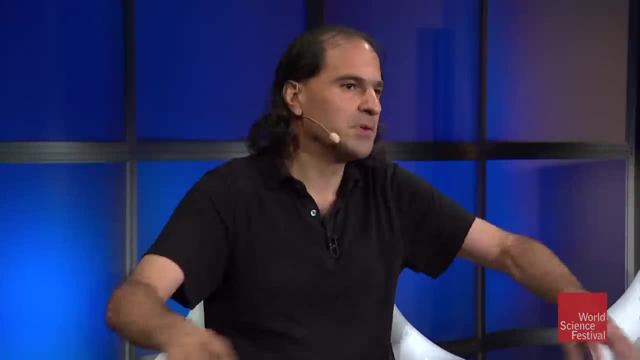 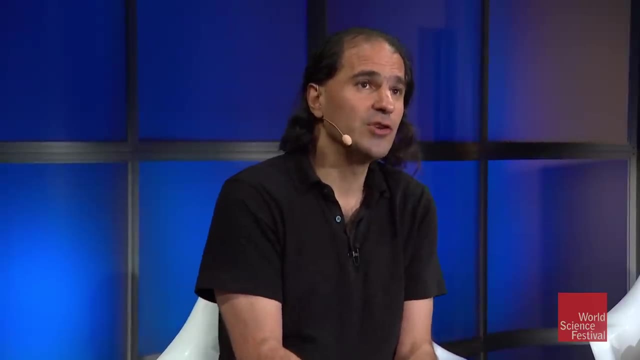 is that they could do double duty. You could first collide electrons and positrons, produce millions of Higgs particles and see whether it looks point-like to external probes like photons and the other things that it could run into, And then ultimately, if you go, 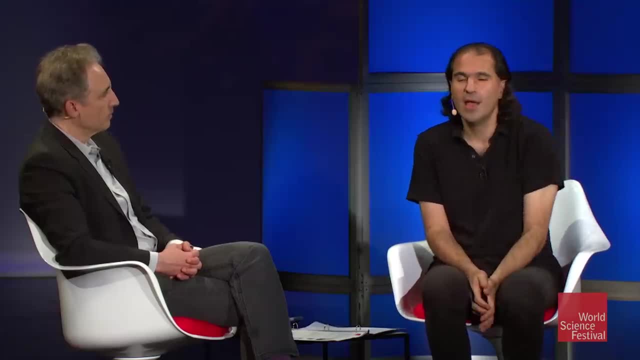 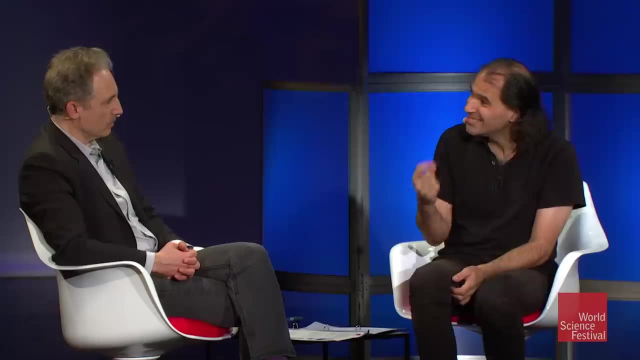 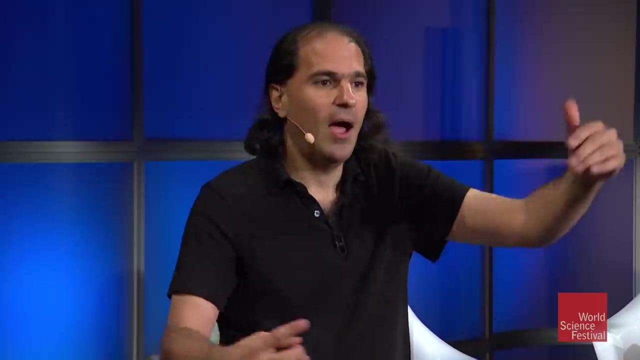 to the 100 TV colliders. if you collide protons in exactly the same machine, you can ask and settle the question whether the Higgs looks point-like ultimately to itself. And that's a fascinating thing, The very simplest interaction elementary particles can enjoy. 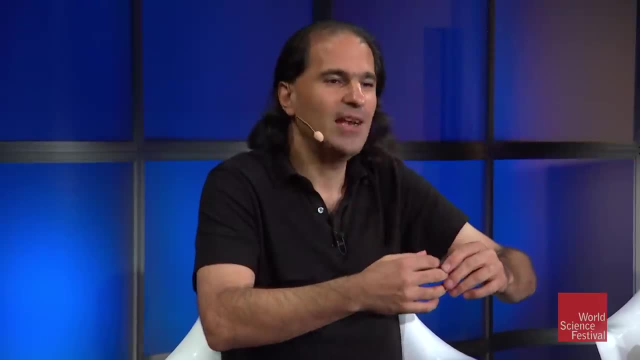 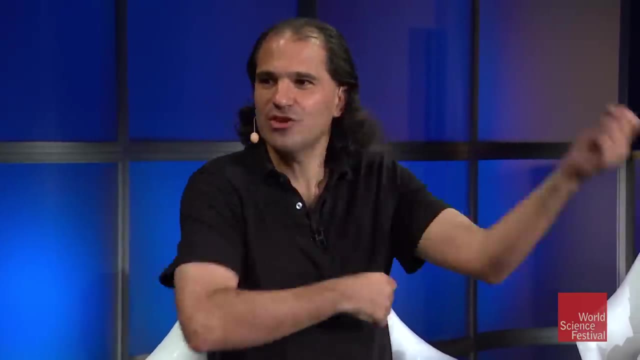 is, with three of them meet at a common point in space and time, And it turns out no other elementary part, single elementary particle actually has this interaction. Every other thing that we know. there's something that changes Some property changes. The Higgs is. 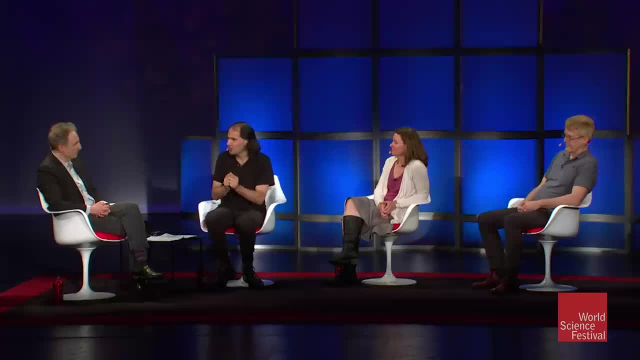 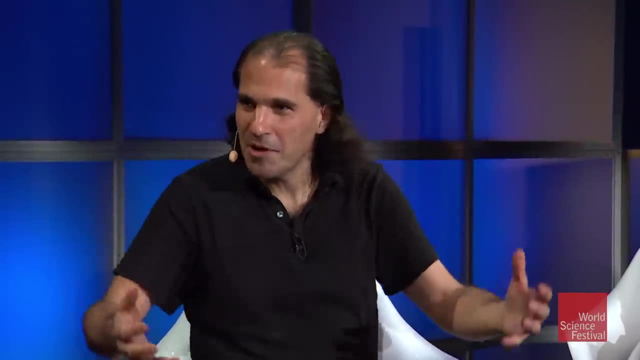 the only elementary particle that can have as its dominant interaction this interaction with itself And therefore, by looking for this interaction, not only for the first time, seeing the sort of simplest possible interaction in nature, but you're checking to see whether the Higgs actually 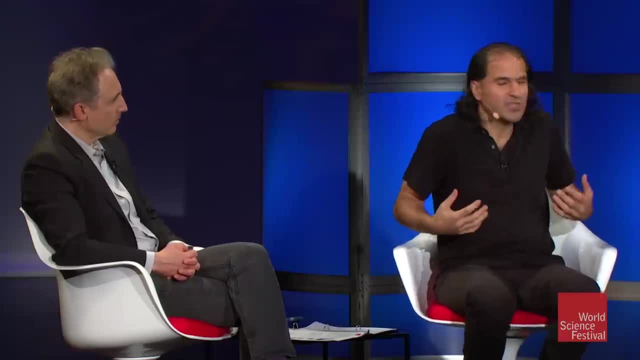 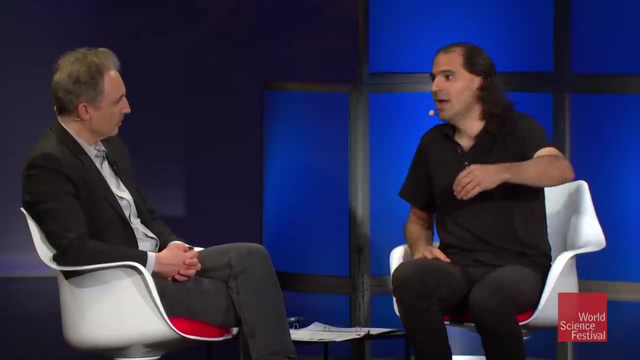 looks point-like even to itself. The LHC is not even going to tell us with confidence whether this interaction even exists, but the 100 TV collider will produce billions of Higgs particles And by doing that will not only tell us it exists. 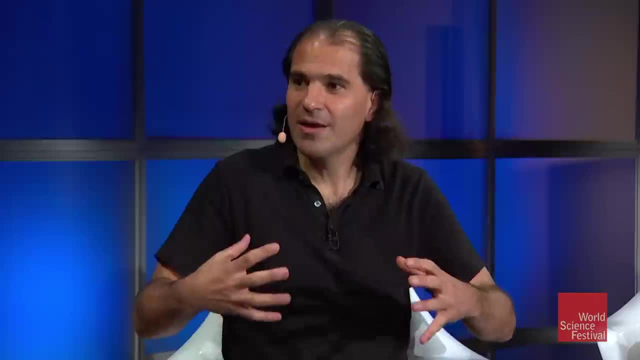 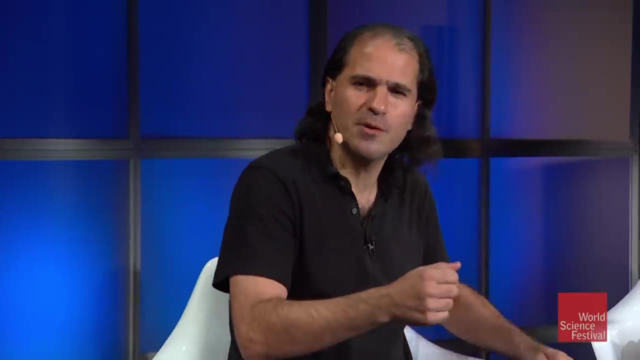 but it'll measure it to a few percent accuracy. So I've just told you what I think of and I think most of the people pushing for this next generation of accelerator- they're not promising. oh, we just barely missed supersymmetry. 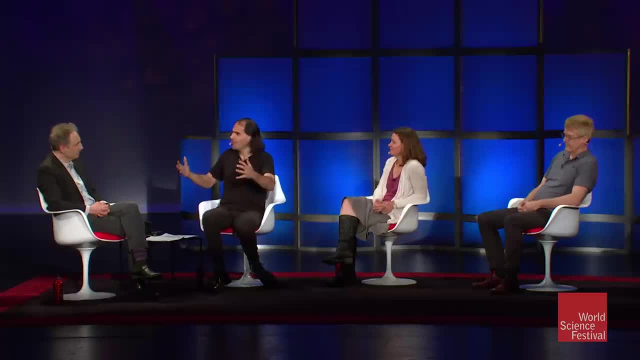 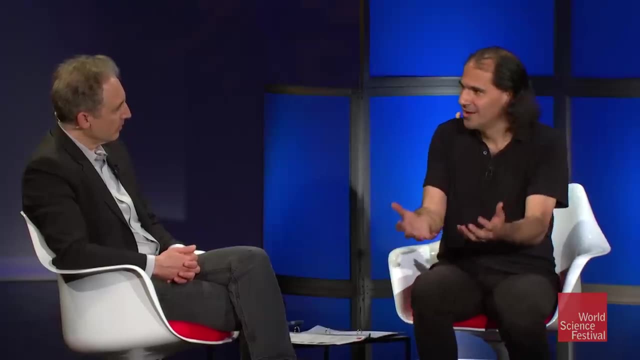 It might be right around the corner. That might be true, OK, But that's not the logic of the argument. at this point, The logic of the argument has to do with the fundamental kind of paradigm-shifting or paradigm-challenging nature of the Higgs itself. 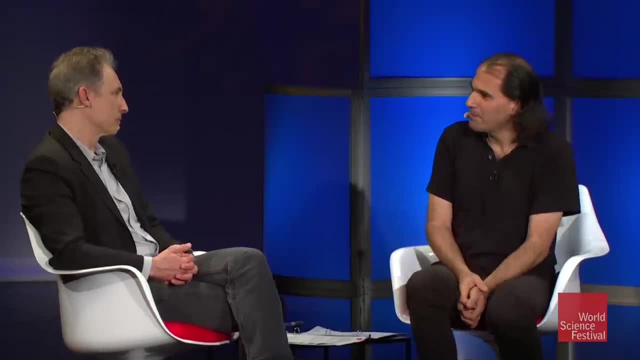 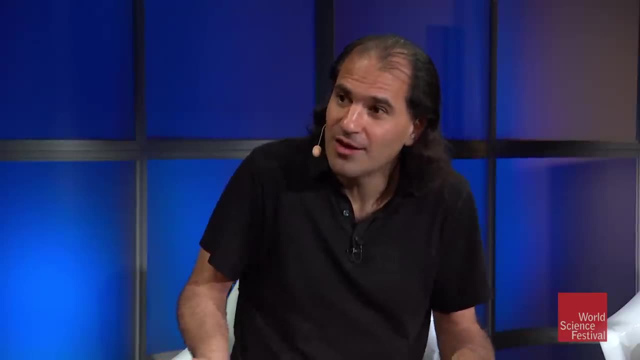 and the fact that theorists are confused. 40 years of ideas for what might be associated with the LHC, but with the Higgs have certainly not been, have not been, uh, amply confirmed at the LHC, not even close. 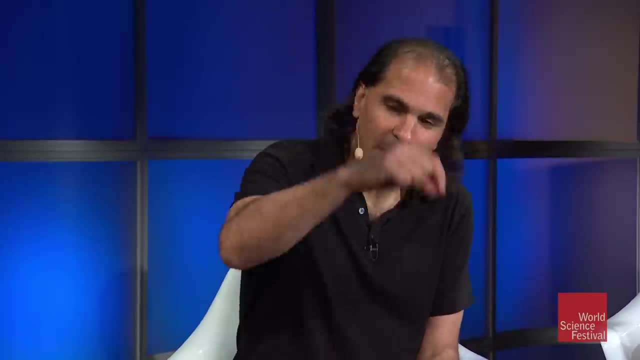 When theorists are confused. you need more experiments, and you need to do experiments on the thing that's confusing. The Higgs is the thing that's confusing, so we have to put it under a very powerful magnifying glass. Very well said. 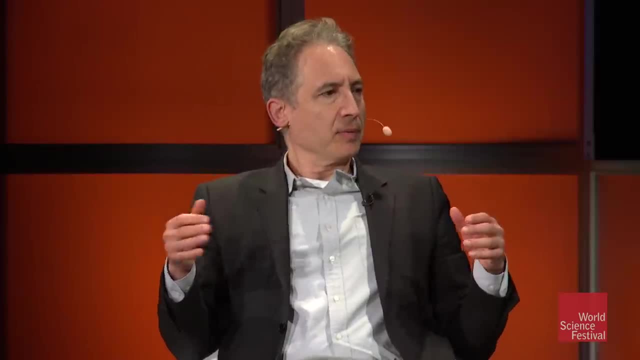 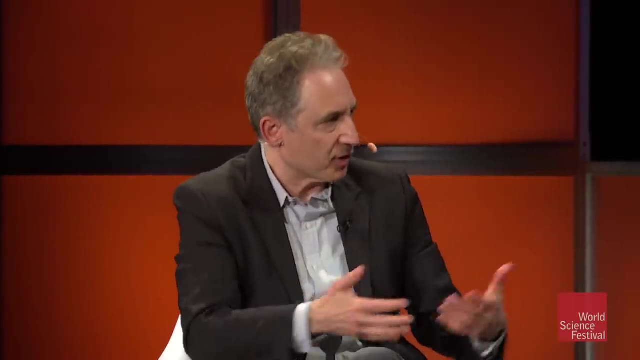 Now when we look at the big principles. so one thing to do is to smash harder, to magnify greater, to try to see fundamental structure that we may have missed, and so on, But in terms of overarching theoretical paradigms, that will 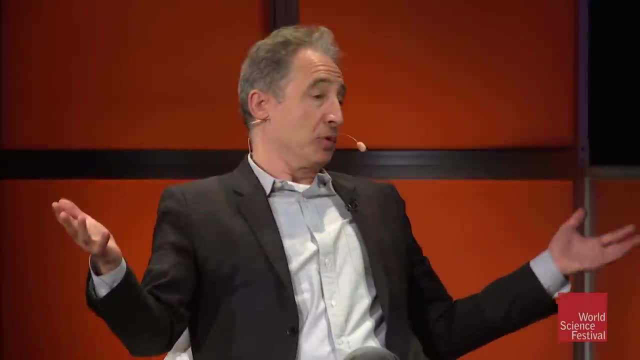 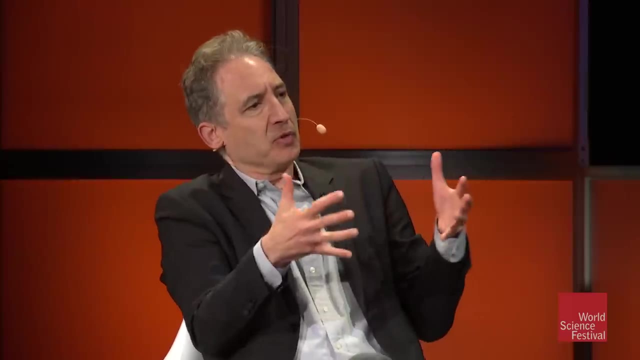 guide us forward. so supersymmetry is not ruled out. It could still be part of the story. but what I mean? maybe just go down the line a little bit, Joe, what would you say? I mean, obviously there are things that people 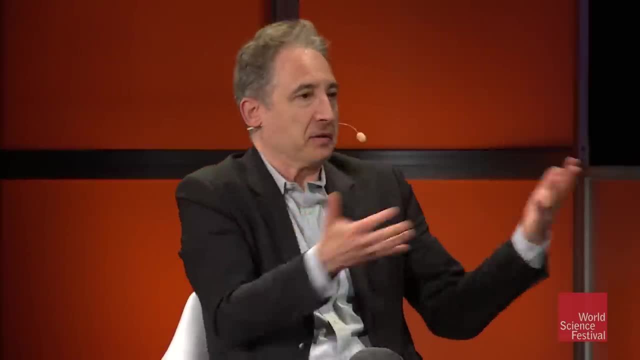 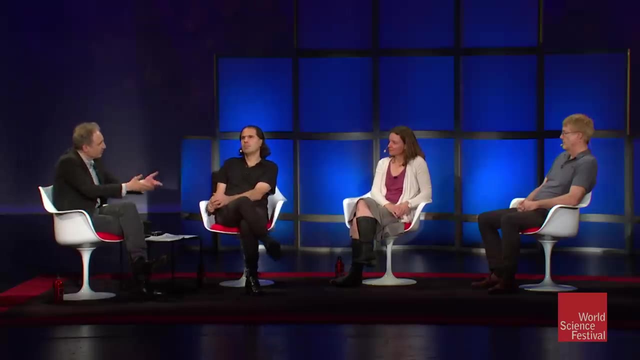 string theory, people, which has supersymmetry. There are other things like technicolor that people have spoken about. Do you feel that we've got the guiding theoretical structure to really give us a clear path going forward as to what we should be looking for? 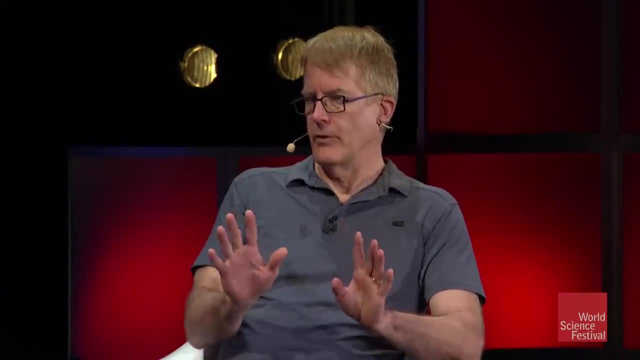 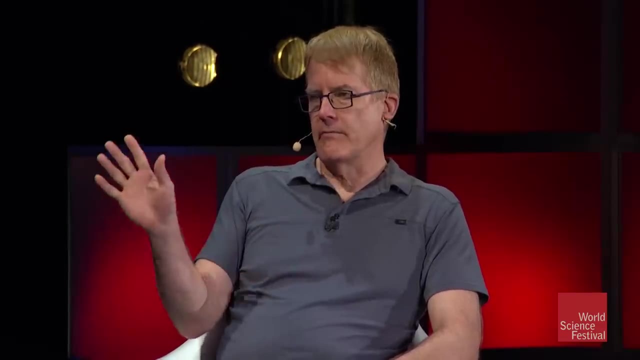 I think we're in one of those periods of physics history where we really need guidance from data It's. we have ideas, Some of them, I'm sure, are good ideas, but we need more. we need nature to tell us more about what's. 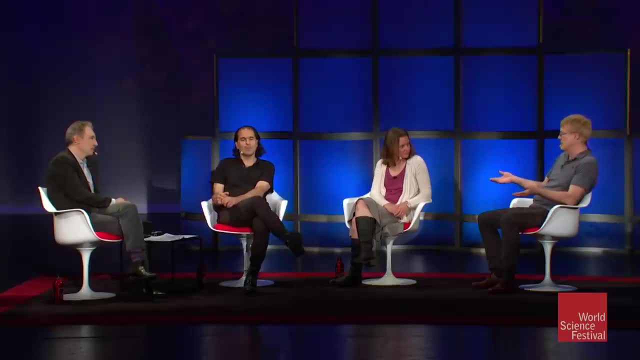 really going on, And this has actually been more the typical situation in the history of physics than having confidence in. you know, Dirac was, as I said was, the lucky guy where he had the idea and then the experiment came right along. 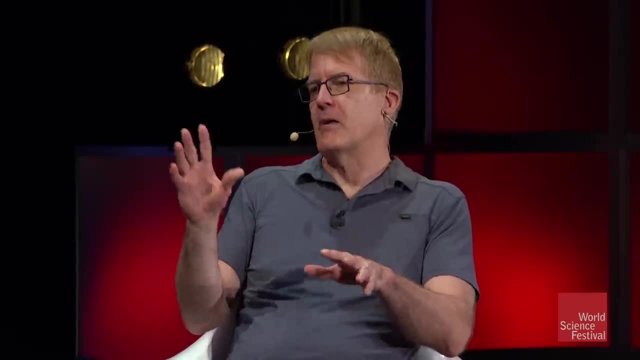 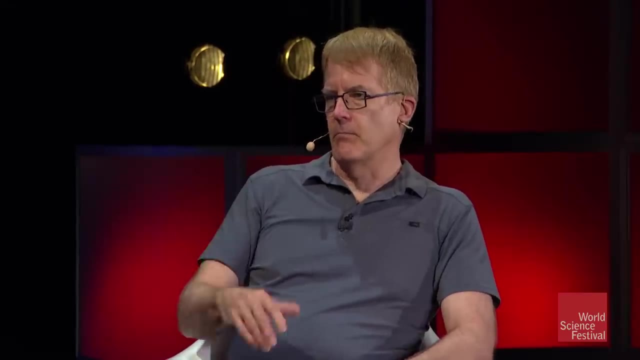 This is the typical situation where we have some ideas, part of it's probably right, part of it's probably wrong. there's probably something missing and we need data to sort that out, And that's what these more powerful instruments are really for. 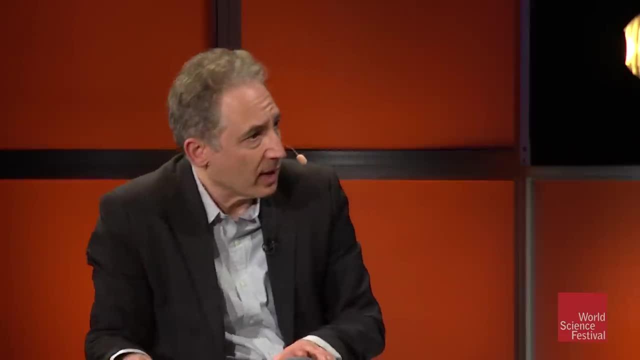 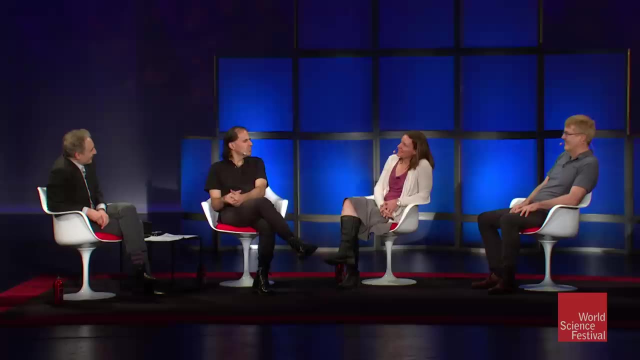 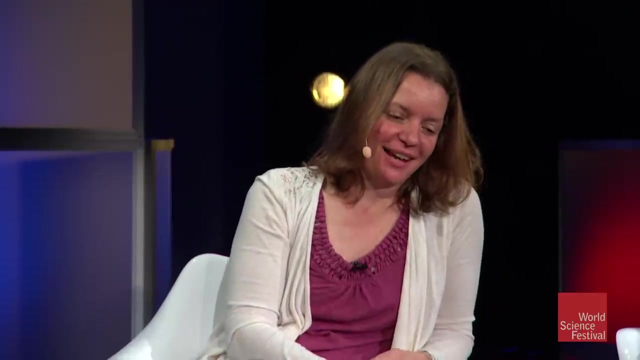 Now there's a nightmare scenario that you described for the LHC. Imagine some next machine is built. What would your nightmare scenario be there? Well, actually, I think that you know, coming back, having looked back now, nine years later, and you know, 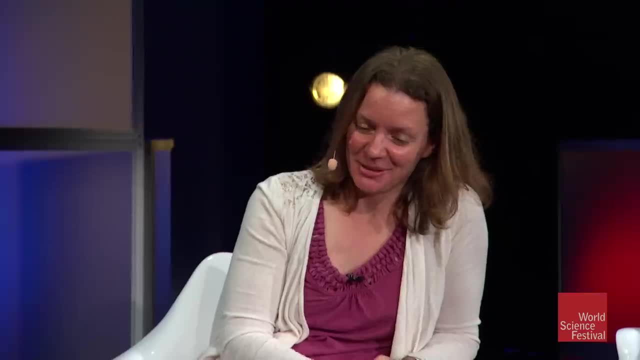 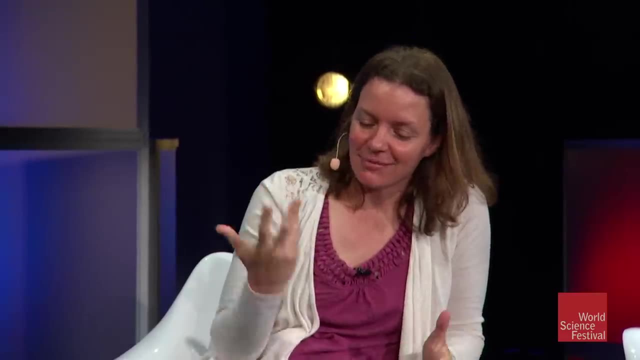 lots of data later. We didn't have any data at that time, right. So we were sort of in a. you know, I definitely have also sort of had, let's say, eye-opening experience out of the whole thing, And I think that you know. 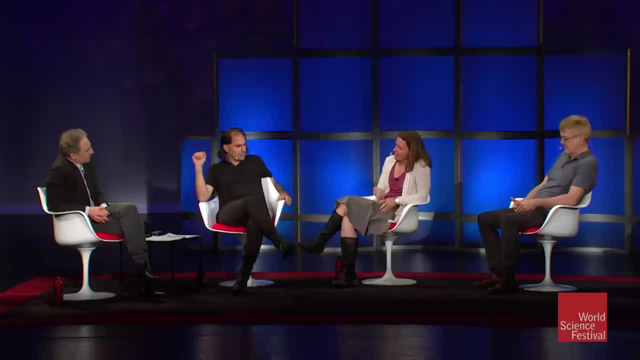 basically supersymmetry basically did us experimentally a disservice, let's say, because it sort of set this expectation that I think that you know that the LHC was going to be the discovery machine in the sense of discovering particles. 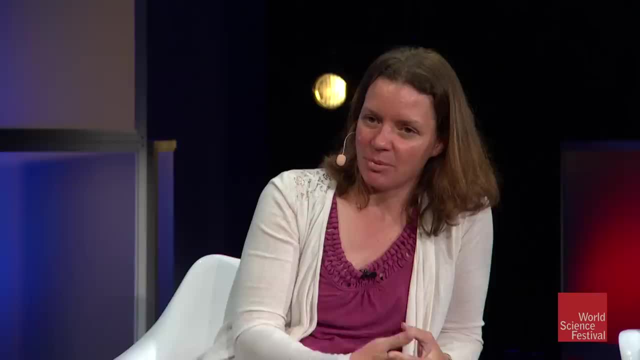 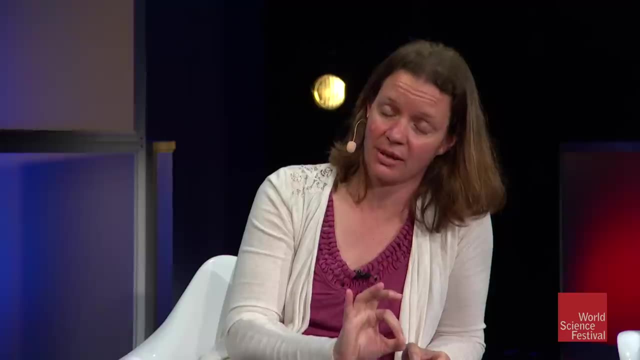 And the LHC has been a discovery machine And I think that you know, because we have learned, you know a tremendous amount. the LHC has given us many, many precision measurements of the standard model, The detectors that we have. 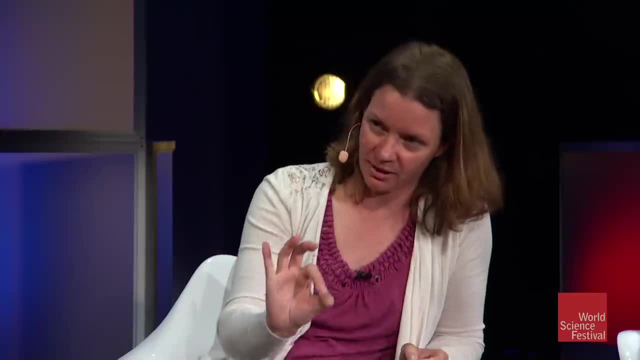 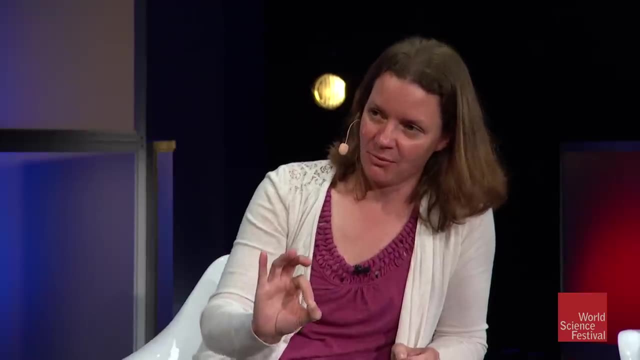 are beautiful. They're stunning. The amount of precision we can get out of these detectors is amazing. It's really been an absolute success in terms of what we've been able to measure And, as I said, we discovered the Higgs in 2012.. 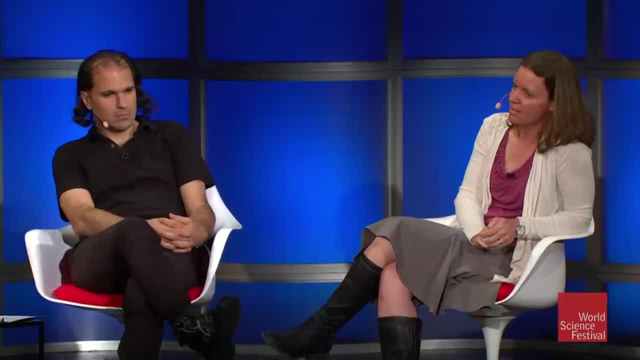 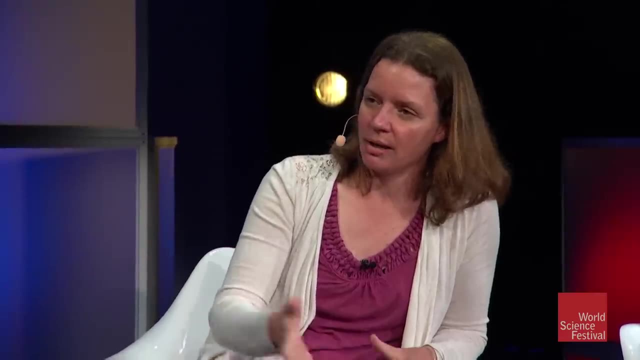 No one expected that our detectors would be at that precision at that time. We've been making measurements that we never thought. I mean Nima says we won't be able to measure the Higgs self-cup cooling, but you know already. 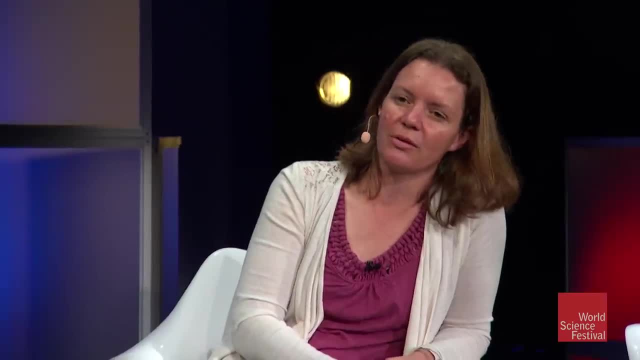 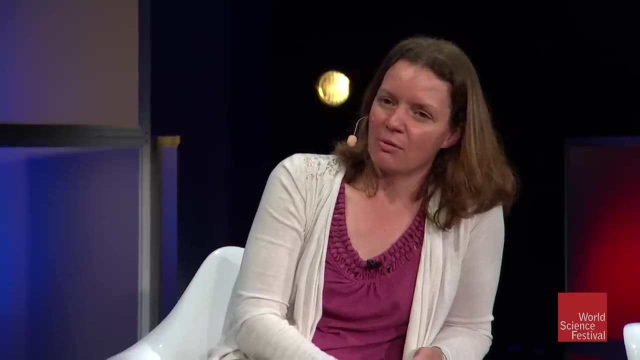 we're doing studies that show that we could maybe start to access it, so forth and so on. So I think that we have made tremendous progress in technology. We've made tremendous progress in precision measurements of the standard model, And I think this idea that you 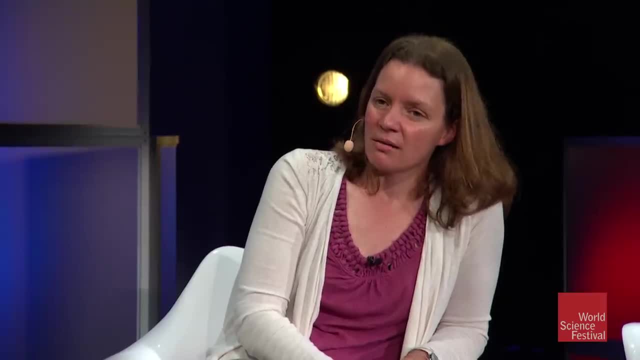 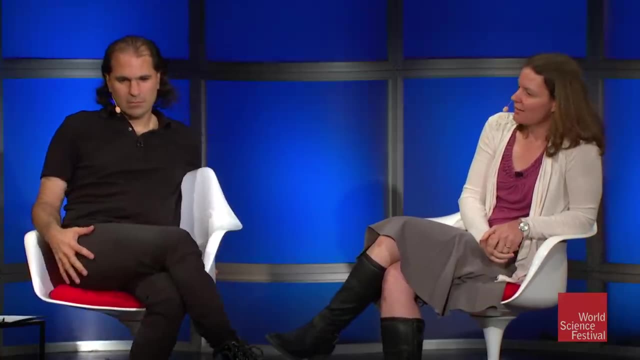 know physics- particle physics was about new particles- was really a disservice to us, And this comment that I made you know 10 years ago, saying it would be Higgs and Higgs only as the worst case scenario, is absolutely a. 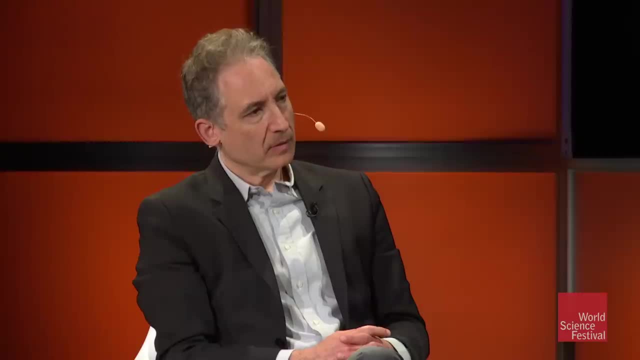 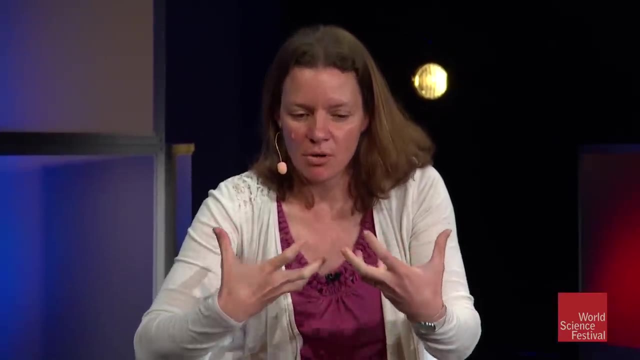 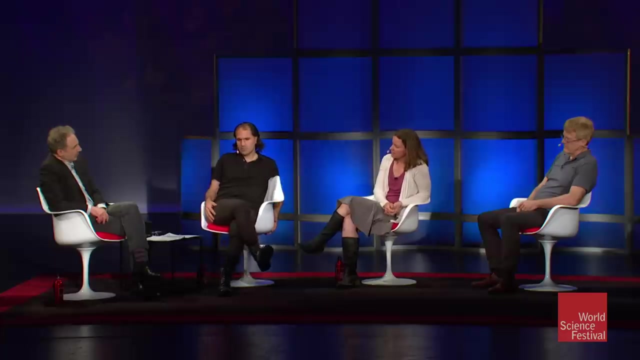 reflection of that time. I think it was a reflection of how we were viewing progress at that time And I think we've all. there has been a big emotional shift in physics in the sense that, exactly as Joe says that we need the data, 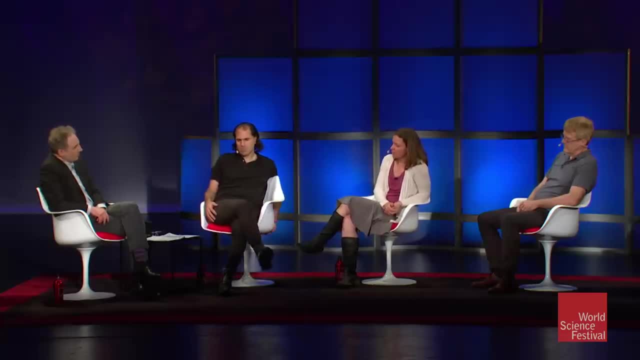 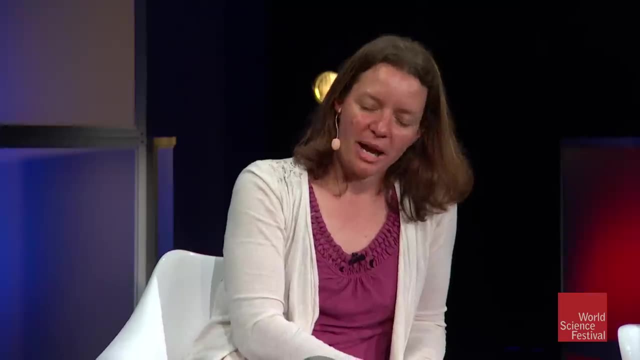 We need to know the standard model better before we can really say: you know, let's go in direction A, B or C And that we're really, despite its successes, despite how much we know about the standard model, we've all discovered that it's. 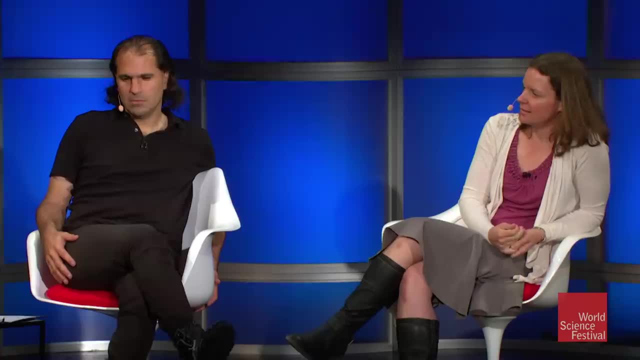 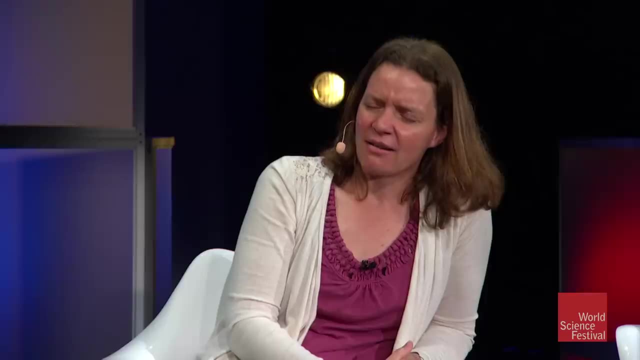 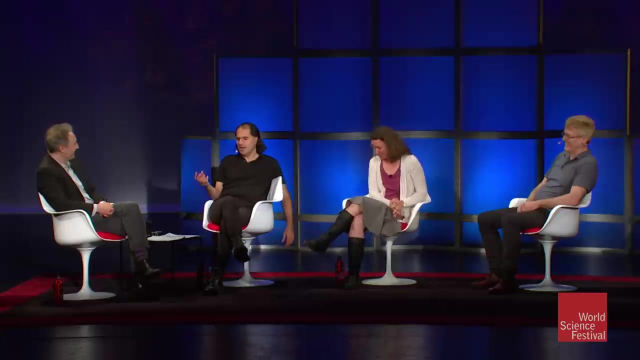 not enough, And these next generation machines are exactly that. So in that sense, my worst case scenario would be pretty much a fire in the cavern, I think. So a real disaster, Yeah, a real disaster. I think we're at a moment. 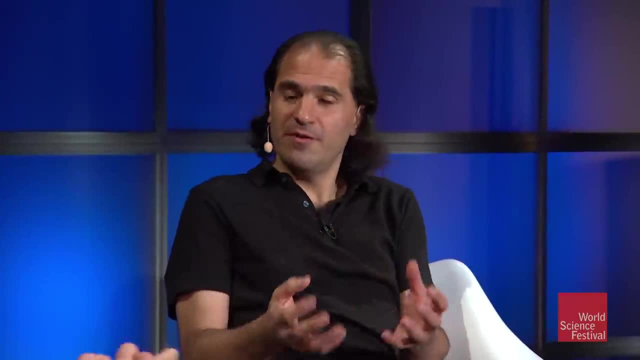 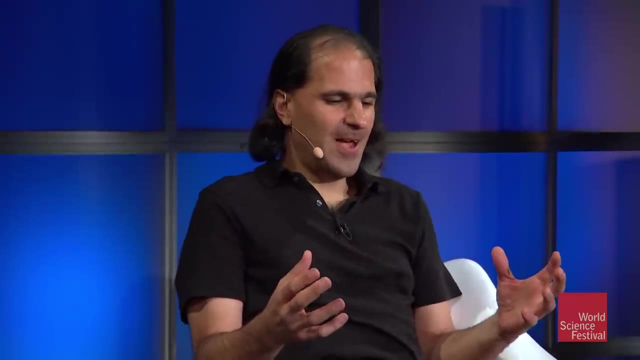 the most important thing is that we've seen this phenomenon that we've never seen before, And so I think it's very funny that, in a sense, seeing the Higgs and nothing else so far is by far the most shocking thing that could have happened. that could. 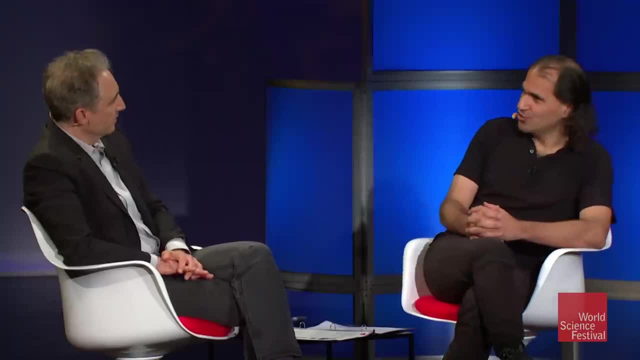 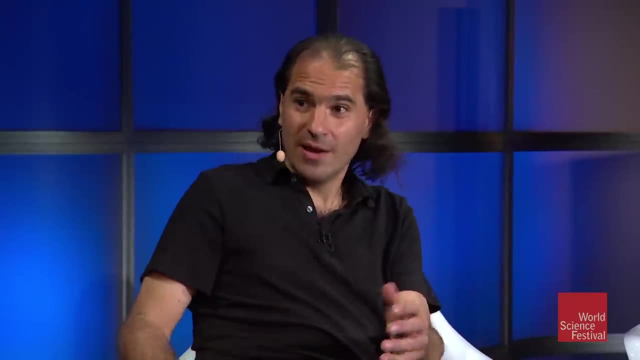 have come out of the LHC experiment. It's the biggest challenge to theorists. It shakes the conceptual grounds under us more than had we seen these things that we've been expecting for decades. It's actually funny. When I was a grad student, 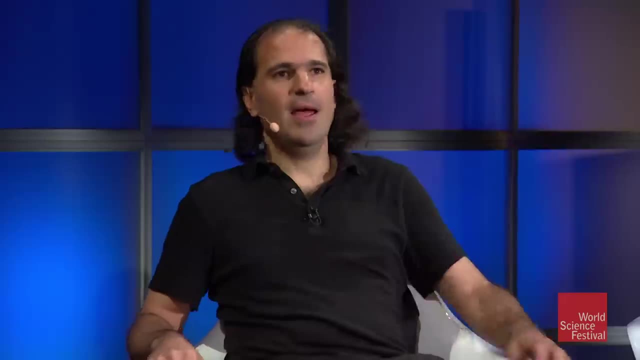 there was such an expectation that something like supersymmetry was right, And that was an idea that people came up with, And I was in the 70s and 80s And the job of my generation was trying to clean up the details. 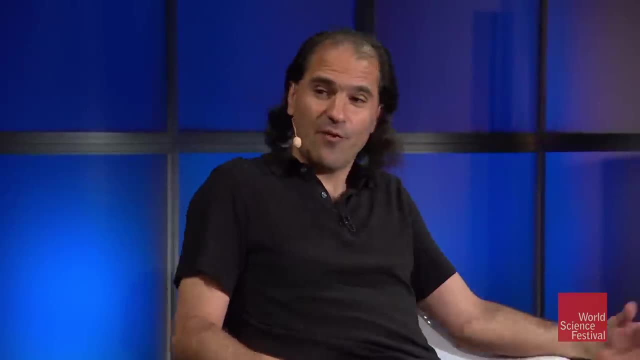 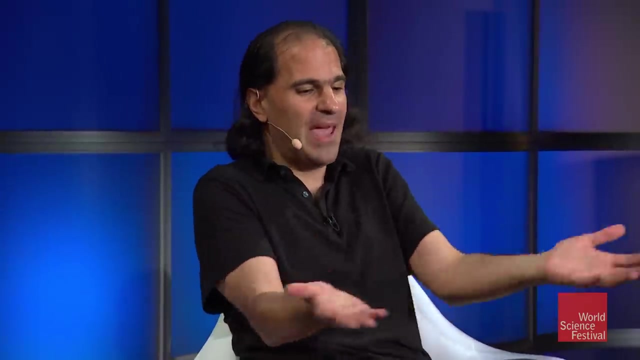 and figure out how precisely it broke and worked out and so on. And that's definitely not how it's worked out. In fact, the challenge just got greater, got much greater. The stakes became more structural, rather than about this or that detail or this or that. 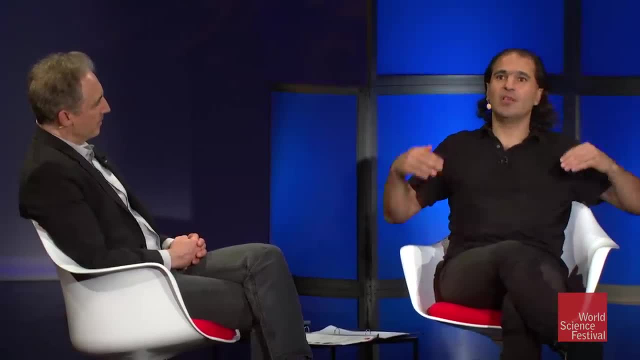 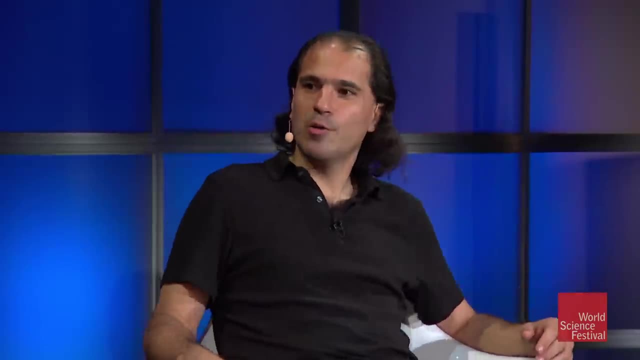 additional particle. I can't stress that enough. I think that the last time a whole community of theoretical physicists have been so perplexed by something and have had experimental results not align with what they expected was when we expected the universe was filled with an ether. 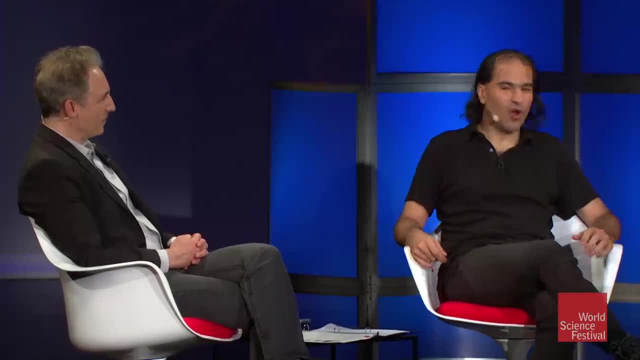 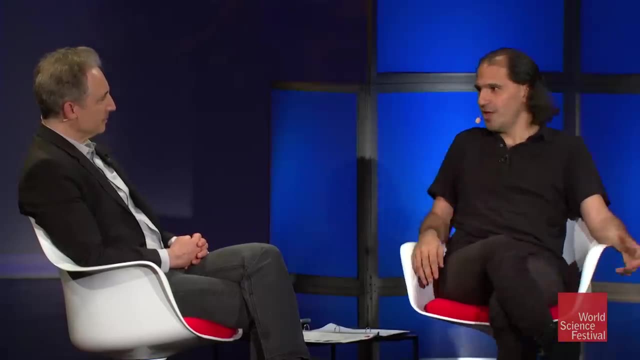 And the absence of the ether, a null experiment, was the harbinger of the revolutions to come. This idea that a whole generation of particle physicists grew up with that, what glory looks like- was the 1960s, with a particle every week. it's true, it was a. 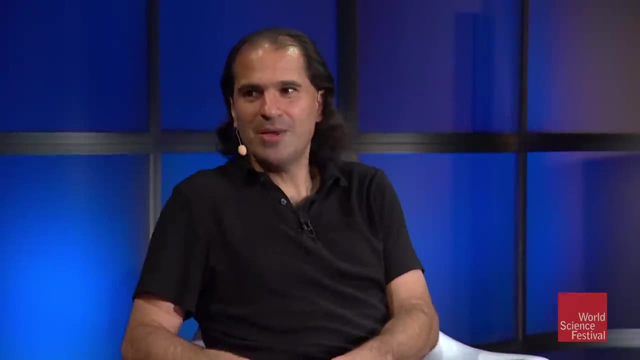 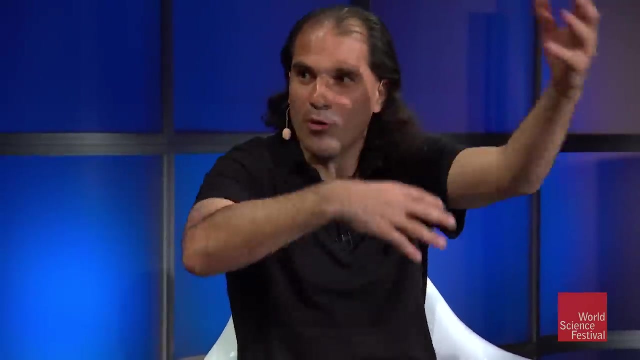 wonderful period, But in 200 years this will not be the great thing about the 20th century. The great thing about the 20th century was the relativity in quantum mechanics, and there's lots and lots of very important details after that. 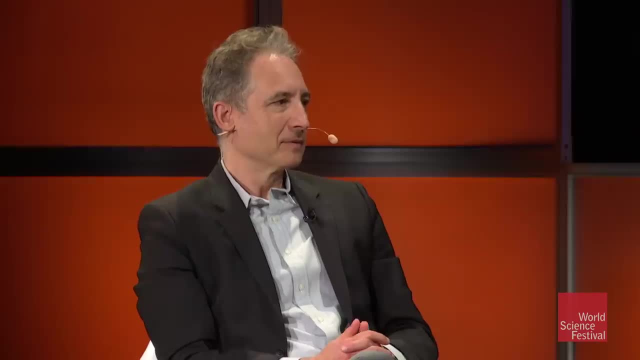 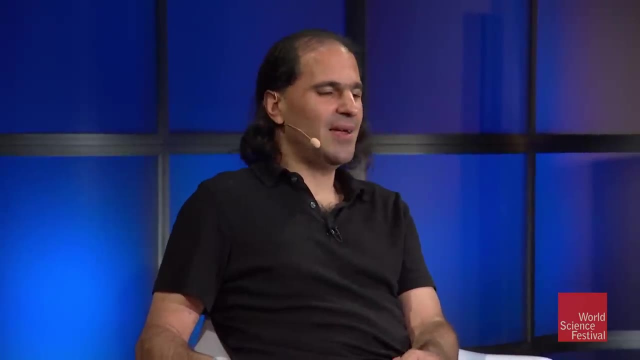 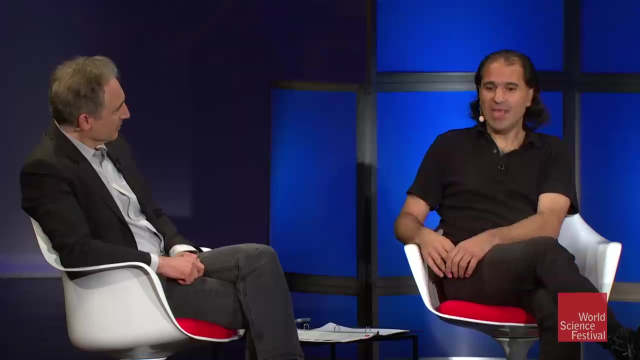 But these very revolutionary kind of conceptually earth-shaking discoveries don't have that character. They're surprising, They involve things that happen that you wouldn't expect, And so I think we're in another one of those periods today, And the Higgs is not the only. 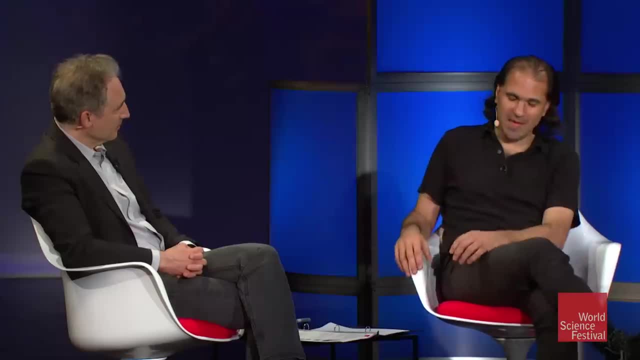 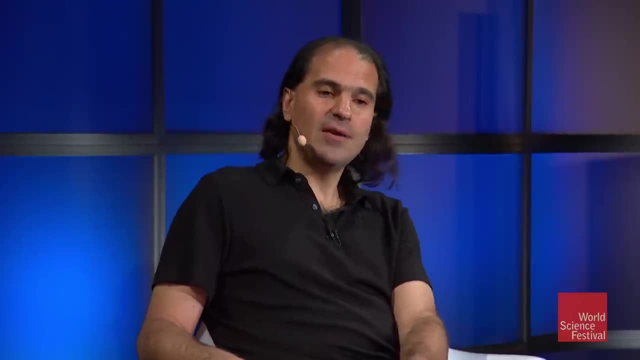 thing You've talked in these programs eloquently over many, many years. There's one other very important experimental shock to the system in the late 1990s when we discovered the universe is accelerating, And these are two different: Accelerating expansion. 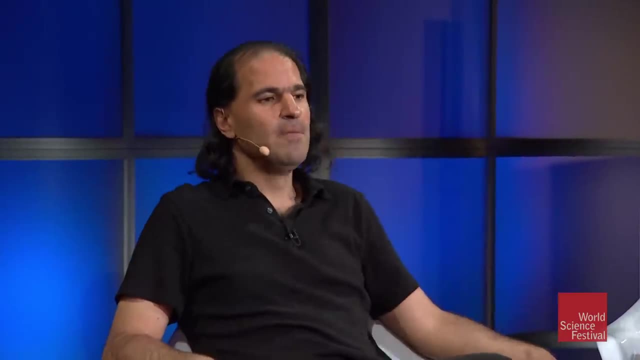 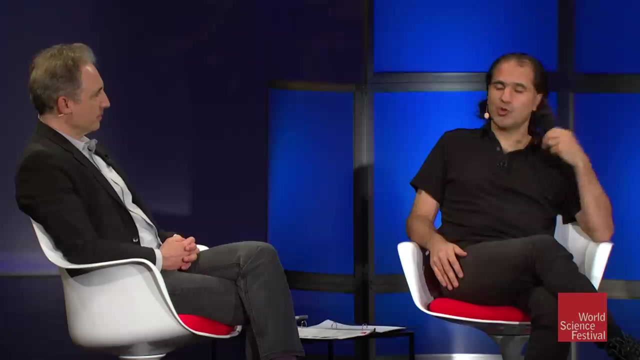 The expansion of the universe is actually accelerating in rate. These are two very theoretically, from a theoretical point of view, they're very closely related- shocks: Our astronomer colleagues want to go measure the heck out of the expansion of the universe And our particle physics. 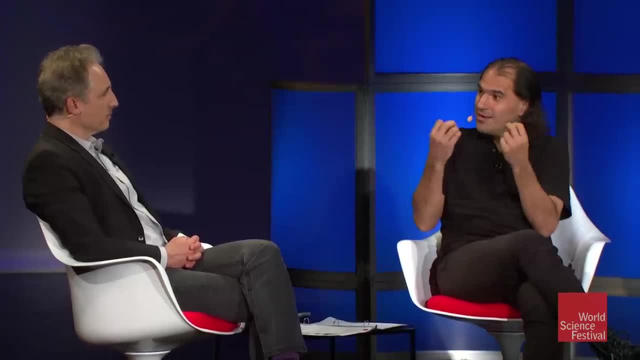 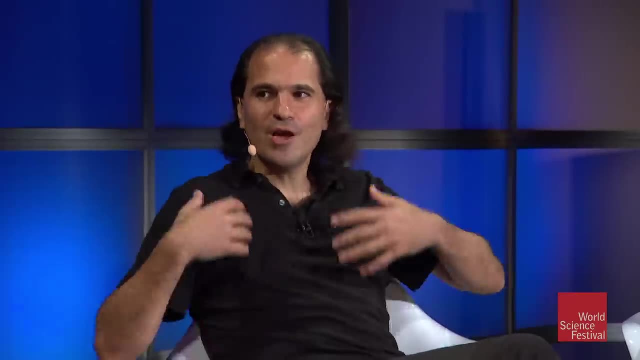 experimentalists want to go measure the heck out of the Higgs, And these are actually very closely related conceptual mysteries. I believe I'm certainly not the only one, but I definitely believe that we're at another one of these periods that comes around every 100 years or so. 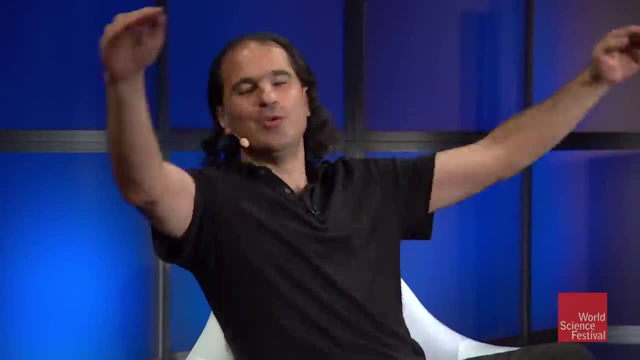 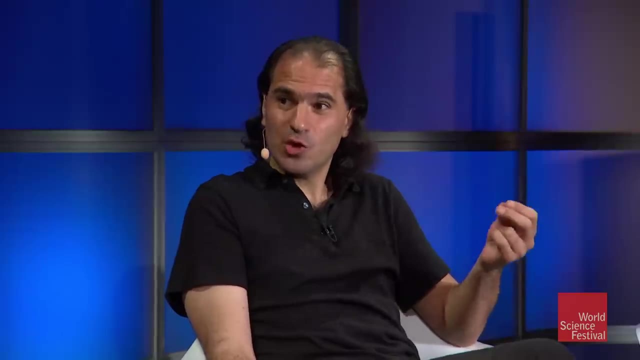 where the issues at stake go up one order of magnitude in sort of structural significance And in many ways the Higgs is the most important experimental actor in the story because it can be put under scrutiny- okay, It can be put under a powerful 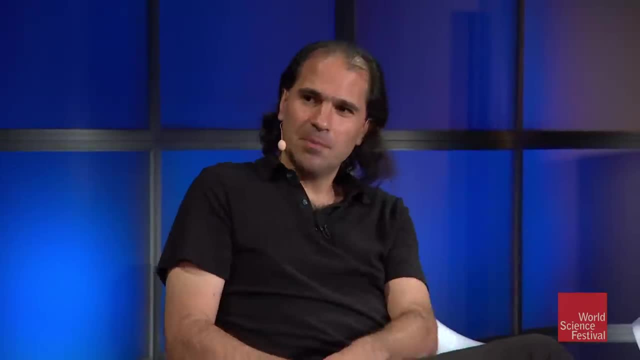 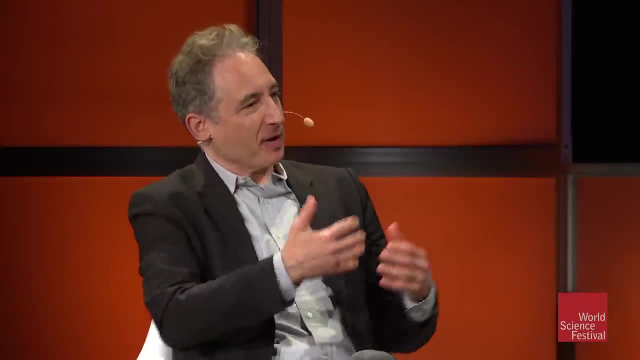 microscope, it can be put under scrutiny. So all this talk of disappointment and nightmares and so on is, I think, kind of crazy. Yeah, And I should point out. I should point out, you know, just because in these conversations I 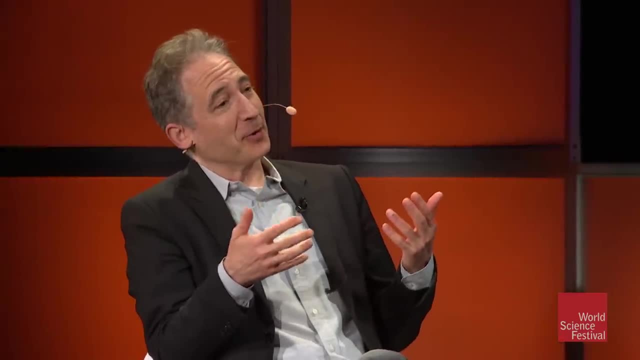 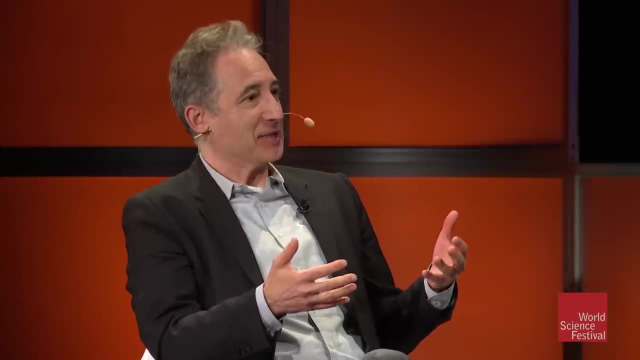 need to sort of play devil's advocate, but in you know, 2010 or 2011, I wrote an op-ed for The Times in which I wrote about finding nothing unexpected at the LHC as being one of the most potent possibilities that could. 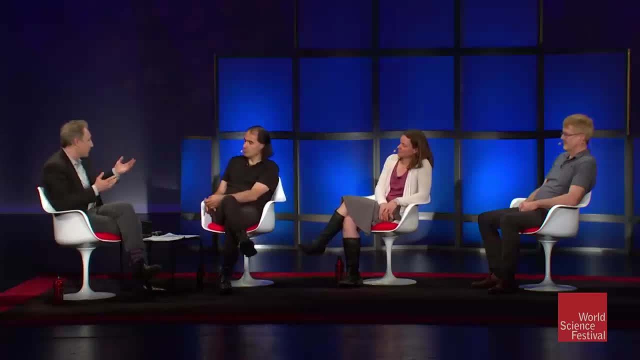 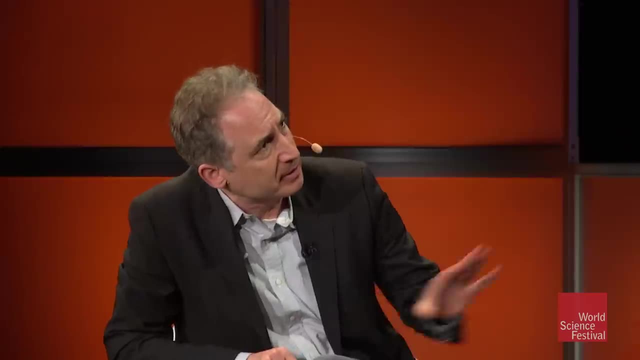 emerge, as opposed to this standard frame of mind that you're articulating, which is particle find, more particles and more particles. So I fully agree. But I want to finish on one point related to the note that you just made about. you know the. 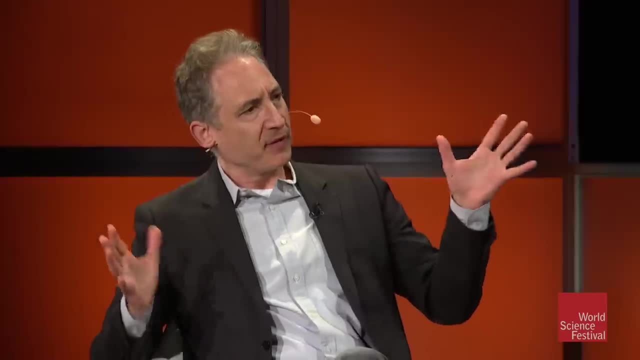 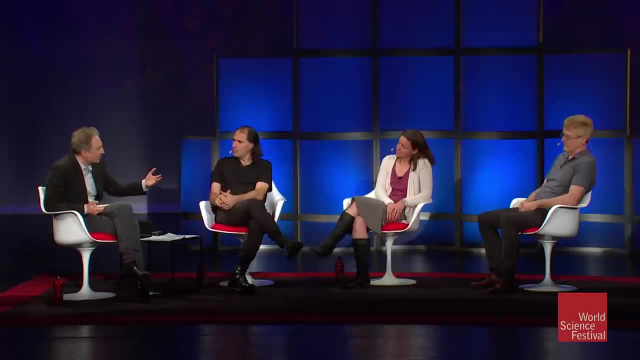 accelerated expansion- cosmological ideas. I just want to finish on a cosmological question. So, Joe, you have written about a curious feature of the Higgs phenomenon, which is that, you know, in the very early universe, at least in many. 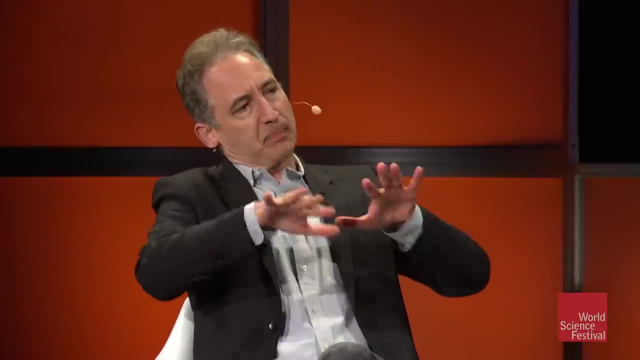 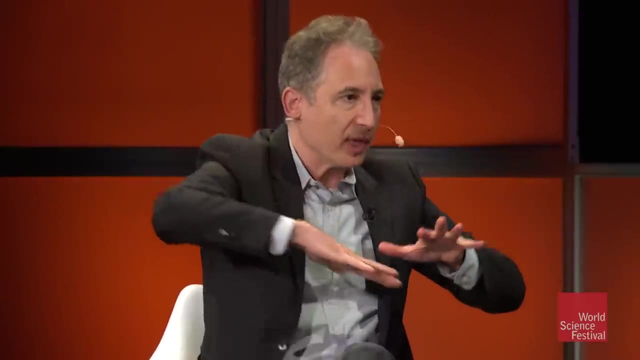 conventional formulations, the Higgs field wasn't actually permeating space. then. It was only a little bit later on that the universe kind of went through a transition where the Higgs then permeated everything. So it went through a phase transition, a change of a 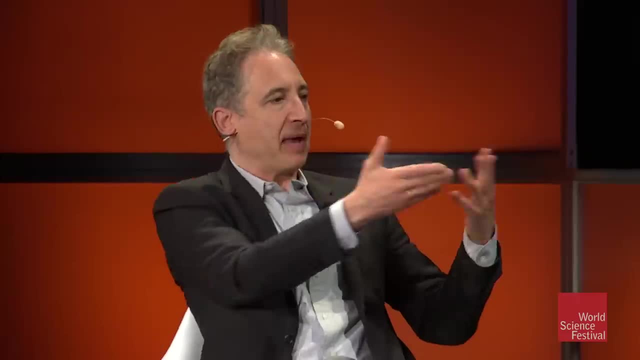 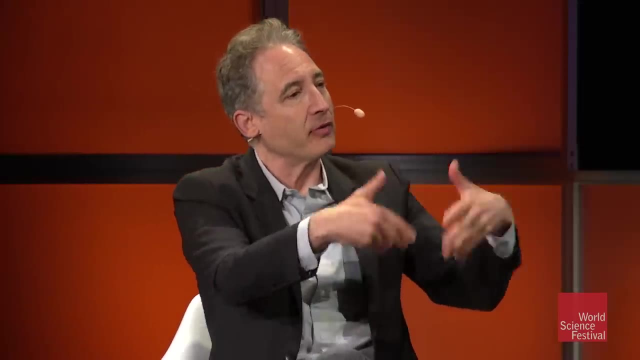 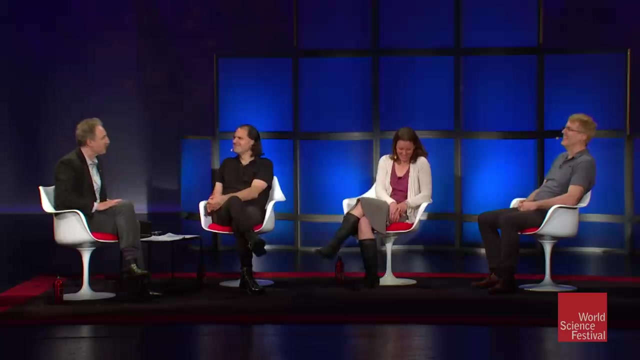 very radical sort. The particular mass for the Higgs field that we found suggests at least the possibility that we could be facing another such cosmological change in our future. So since that's a very bright note to conclude on, maybe you can describe what it is that we're. 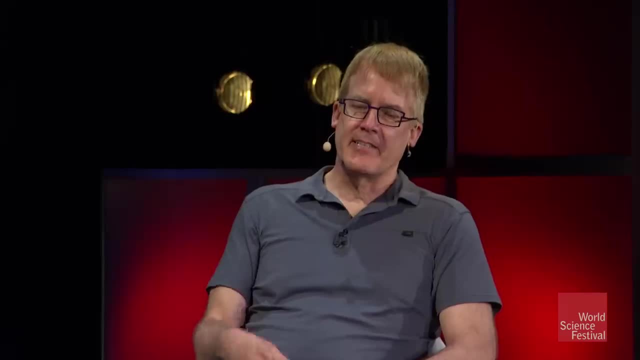 referring to, We can end with the end of the universe. Yes, exactly Yeah. So, as you said, we believe the cosmic molasses wasn't always there. It actually turned the Higgs- turned itself on, if you like itself. At some point in the early universe. That's the phase transition you're talking about, And so you can ask the question: well, is the cosmic molasses just going to stay the way it is forever, Or at some point will something else happen that involves this? 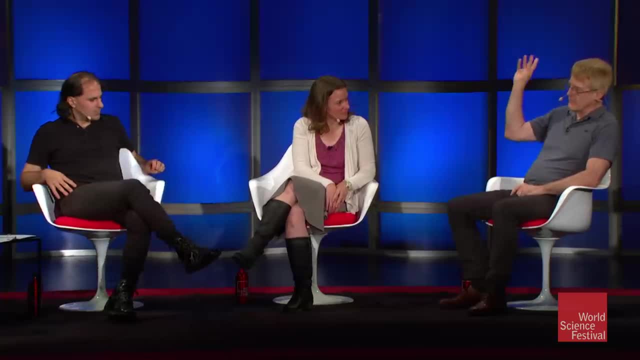 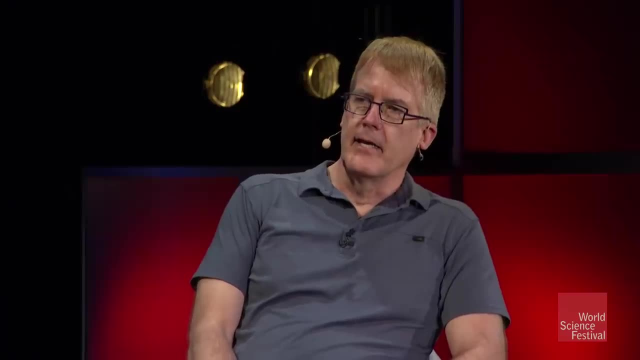 And there is a calculation that you can do, at least with those standard model equations that we have. now that we know the Higgs boson and its mass, We have all the numbers that you need to do a calculation like that, And some of our colleagues have. 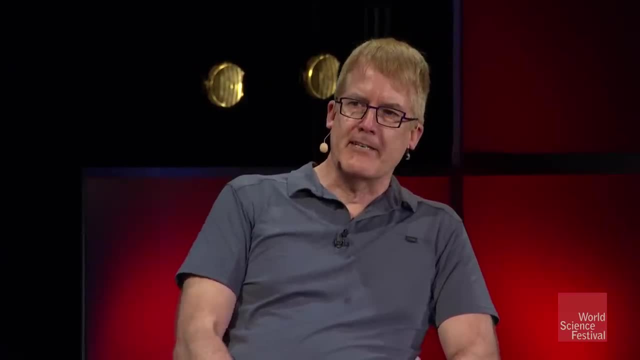 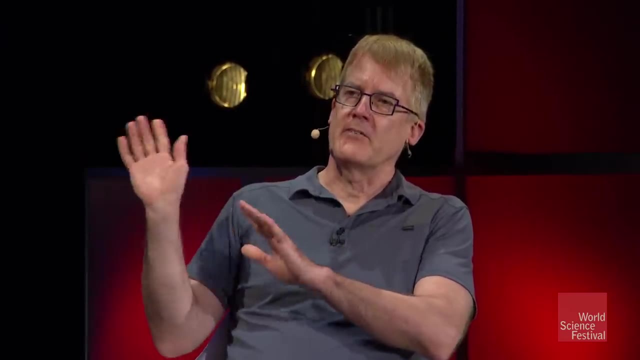 done these calculations very carefully And, interestingly enough, we seem to be right on the borderline of a universe that will eventually want to change into something else. It seems that our universe is slightly unstable to, at some point, a little bubble of something else where the Higgs 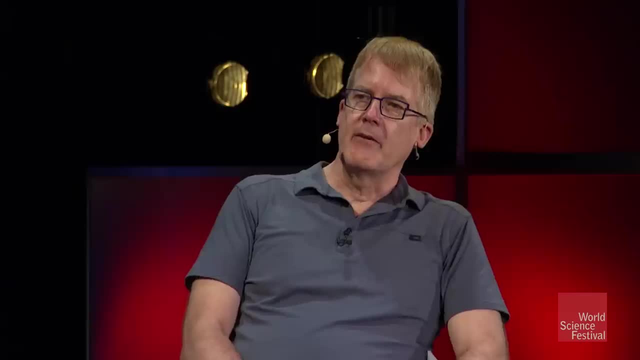 is doing something else will appear somewhere- A different value or something A different value- And once that bubble appears, it will expand at basically the speed of light And eventually it'll get to us. And when it gets to us, what? 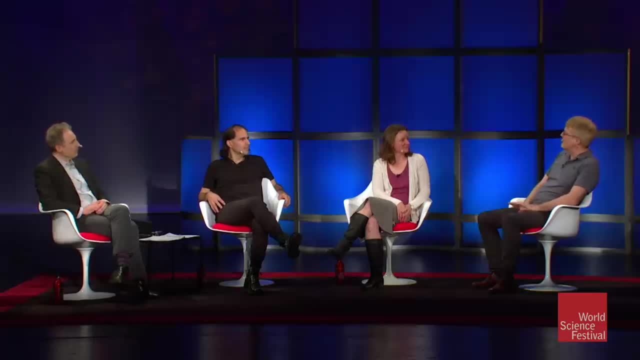 happens And that'll be the end of us. It'll be a different universe, but we won't be there anymore. Now the chance- even if this guy makes the calculation- is right, you would expect this to happen incredibly far in the future. 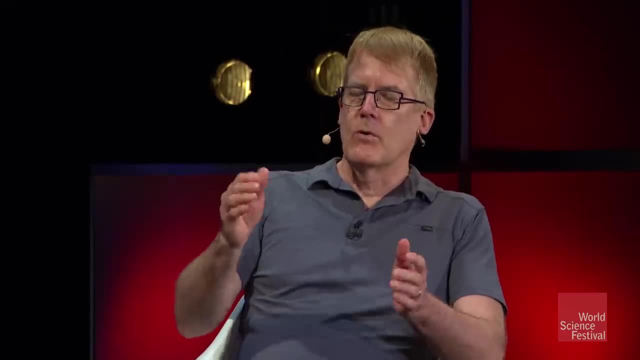 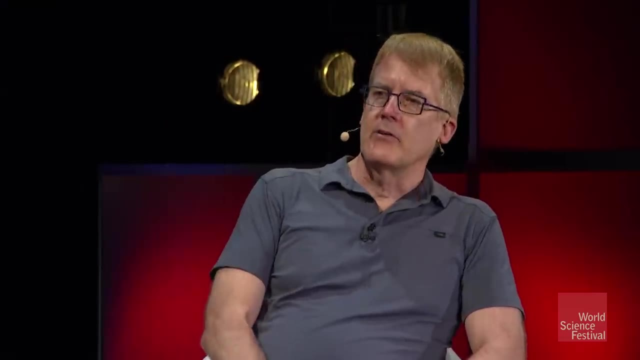 So it's not something. it's on the order of ten to the hundred years from now. So even in the billions and billions of years, it's a very long time, So you shouldn't actually worry about this. I have gotten email from people. 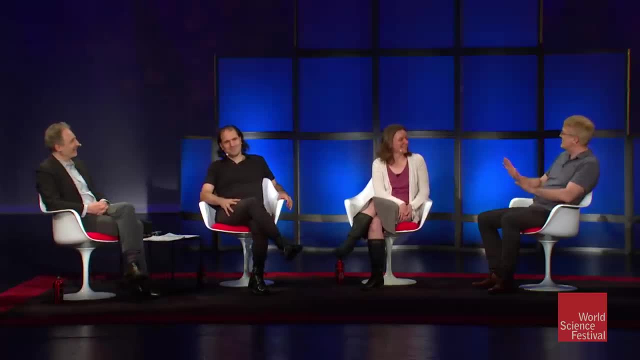 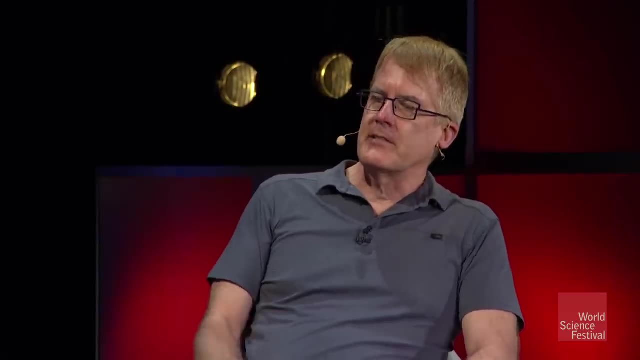 saying I can't sleep at night because I'm worried about this. I always reply: you know you have many other things you should be worried about, but this is not one of them. But to particle physicists this is an incredibly profound thing. 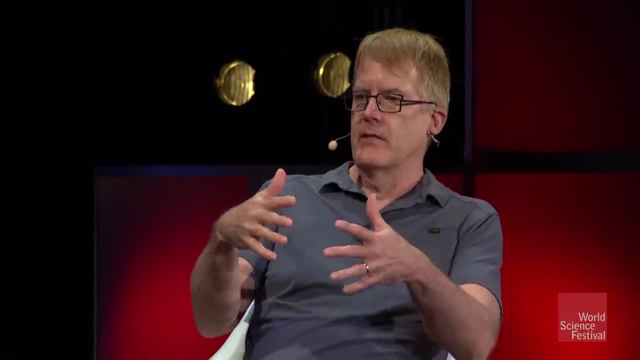 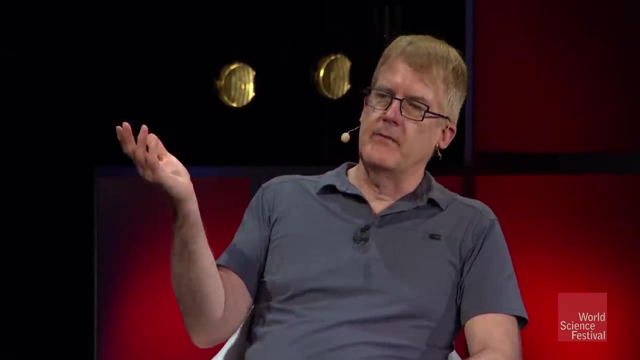 It's the question of what. is the Higgs really forever? And if it's not forever, what does that mean? And one possibility is: again this leads back to ideas like supersymmetry. If you think that nature should make stable universes, then you. 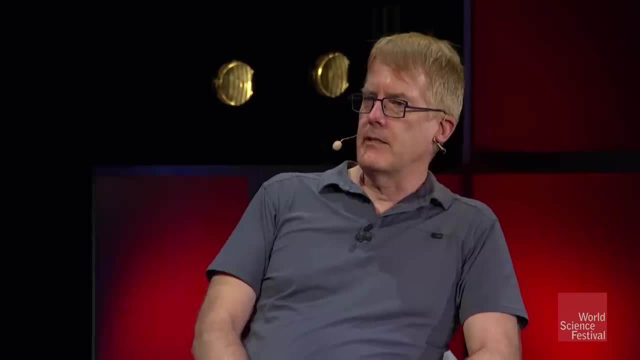 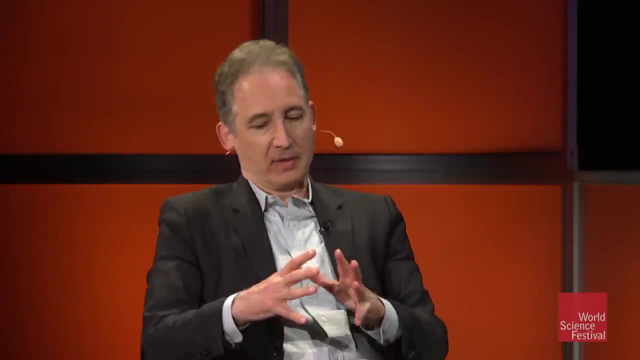 need some ingredient that we need to add, And what is that ingredient Right Now? one thing that you presume you could also write back to people with that concern is, since this bubble of sort of a new phase is expanding at the speed of light by the time you. 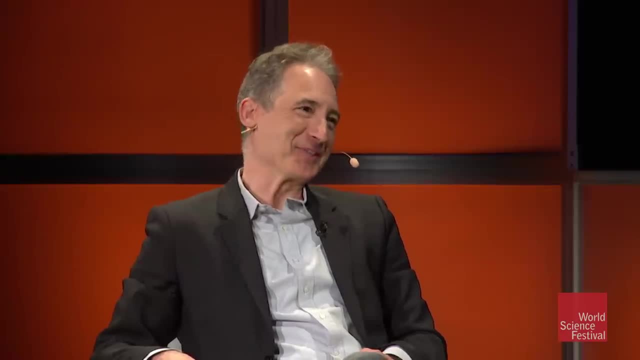 see it, it's upon you. Yeah, You won't see it coming, So you don't have to worry. You won't see it coming, You'll just be a. You know what it looks like inside. I can't resist saying this. 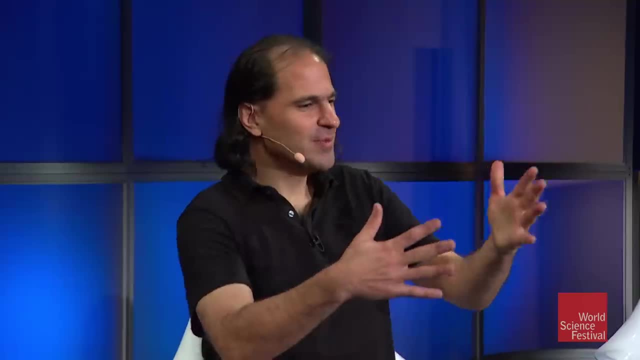 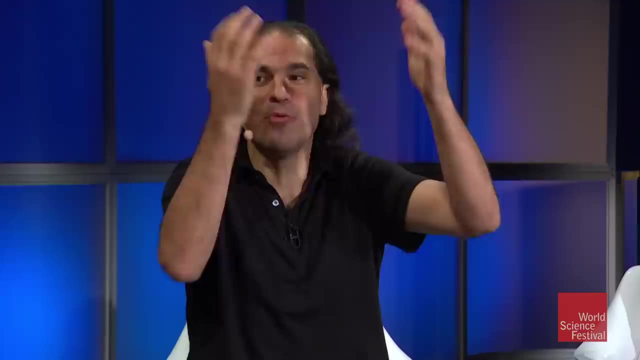 I'm sorry. You know what it looks like inside this bubble. You know because what's going on is that the Higgs gets a lot bigger inside the bubble, So that means that every particle in your body that has a mass gets way more massive. 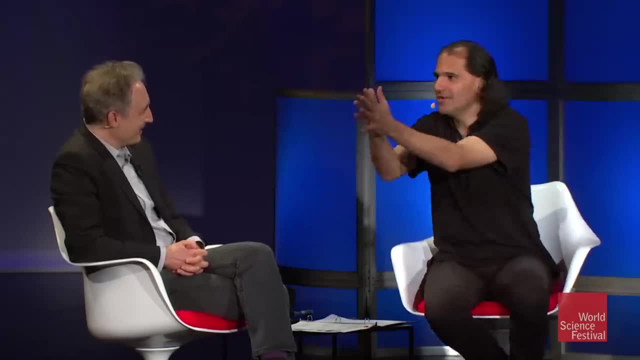 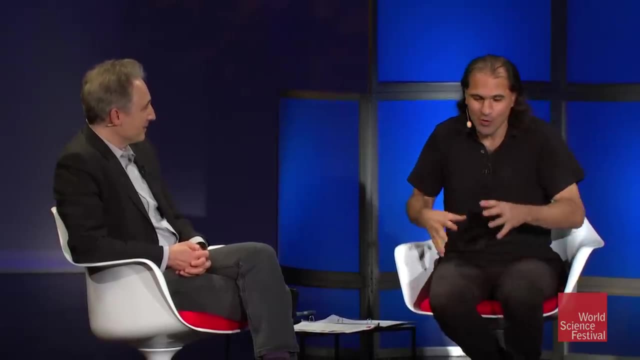 inside. So anything massive goes splat Right, You know, stars, you me, everything. We go splat on this, except light. Light goes sailing right through. So if you or some progeny of yours manages to make it inside, 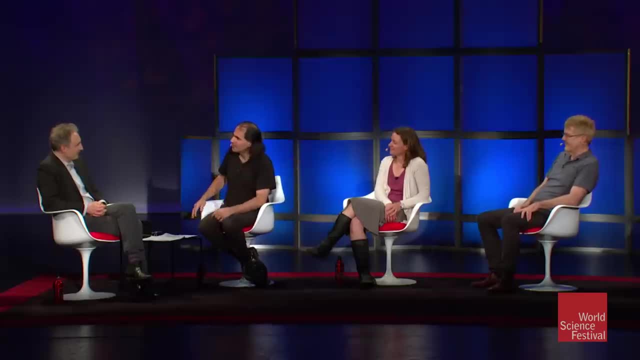 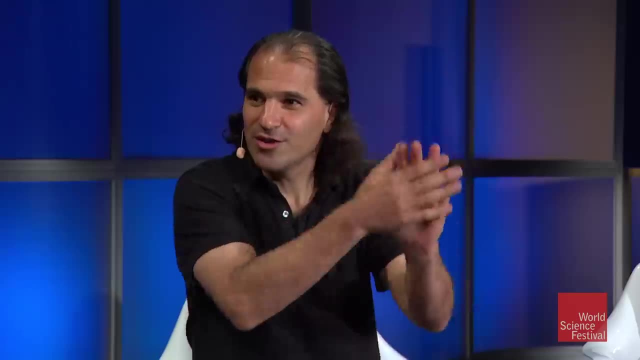 the bubble and run at the speed of light to sort of keep up with the wall of the bubble. it's literally like being on the inside of a car with flies on the windscreen, right, You know. so the whole rest of the universe is just going splat. 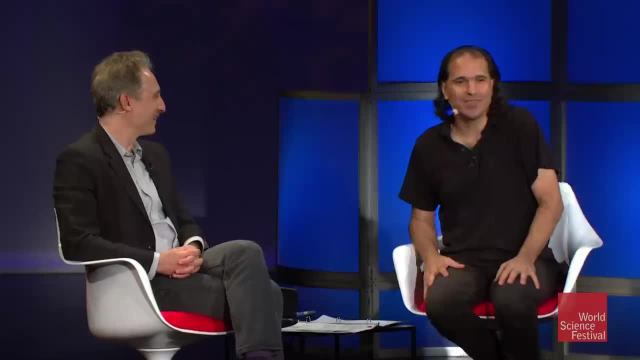 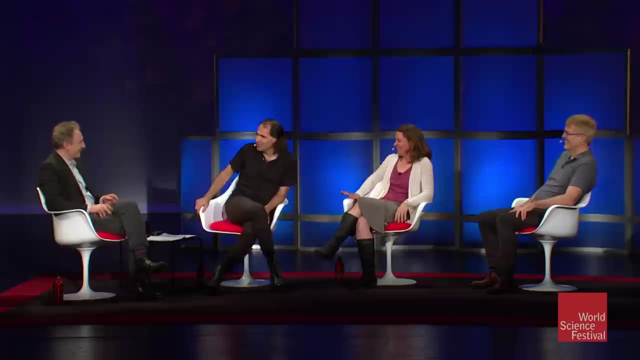 on this bubble as it goes through you. So it's a very cheering thought, indeed Very cheering. yeah, Sorry, Sorry, No, no, Not at all, Not at all. People don't normally talk about what it looks like in there. 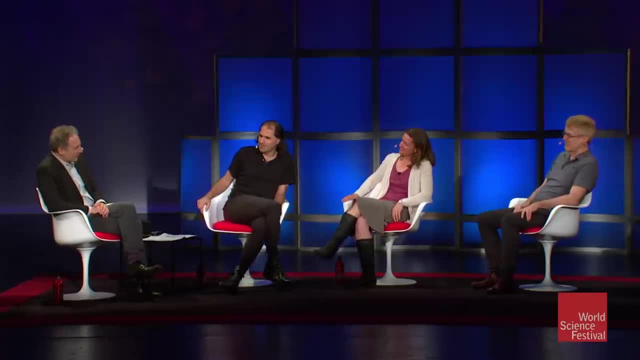 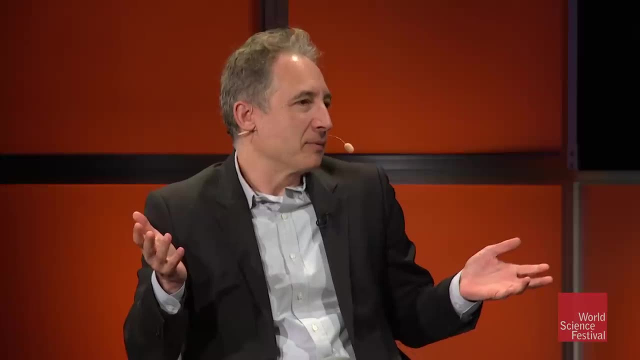 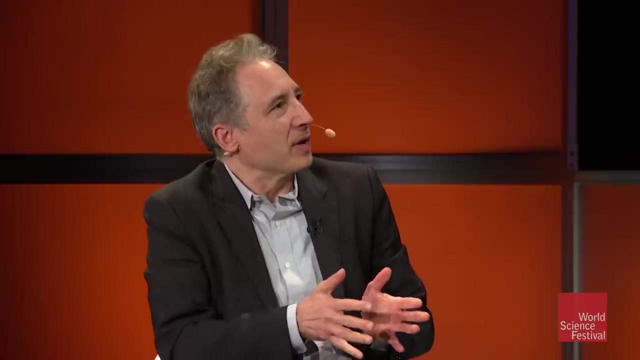 Yeah, So we just have a couple minutes to go and I just want to give you all a chance for sort of a final word. Compared to where we were, say, 10, 15 years ago, do you think that we've gotten to a more? 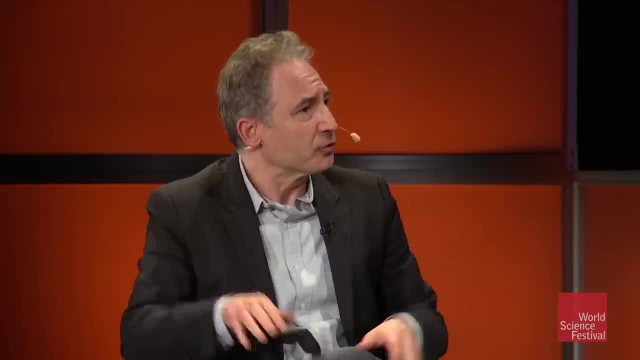 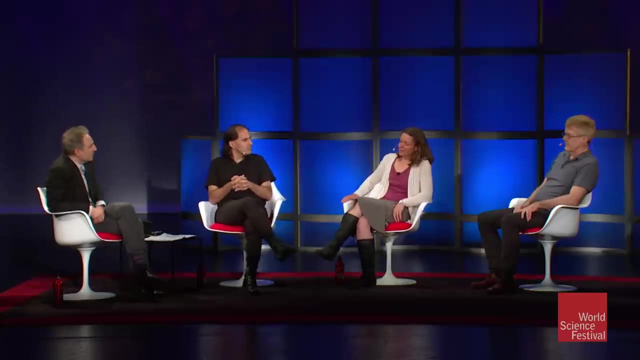 exciting place. Do you think that we've kind of gone through the doldrums? I mean, what would you characterize the state of particle physics to be today? Maybe just write that. Well, I always remember when I was having a really frustrating 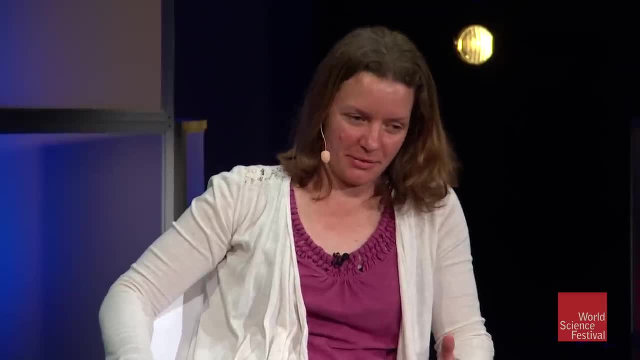 time as a graduate student- a senior graduate student in my group saying if it was easy, it would have been done already, And I think that pretty much really describes where particle physics is right now. There's absolutely nothing about particle physics, that's easy. 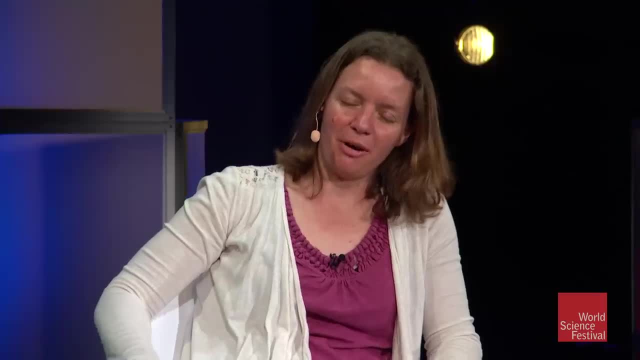 And I think I don't know a single particle physicist who went into this field because they wanted it to be easy, Sure. So in that sense, I'm personally excited about the challenge. It's going to be a challenge. It's going to be a challenge. 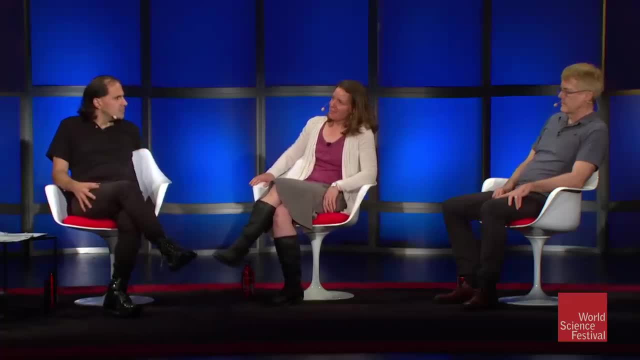 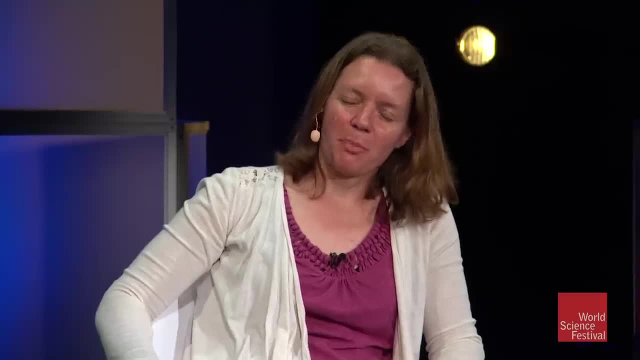 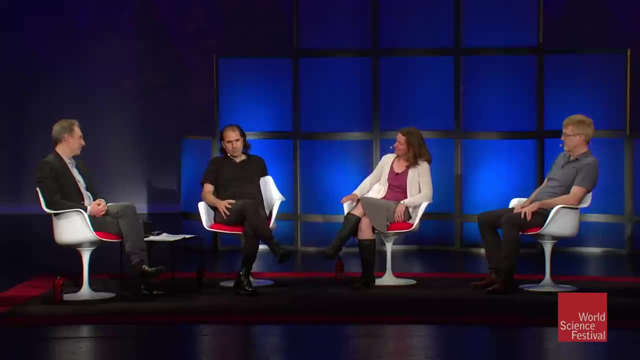 It's going to be hard as hell to build experiments for these new colliders. Bring it on, I'm ready, And I'm ready to take on the measure of the Higgs as well, as we can. All right, Nima. Well, I tell my grad students. 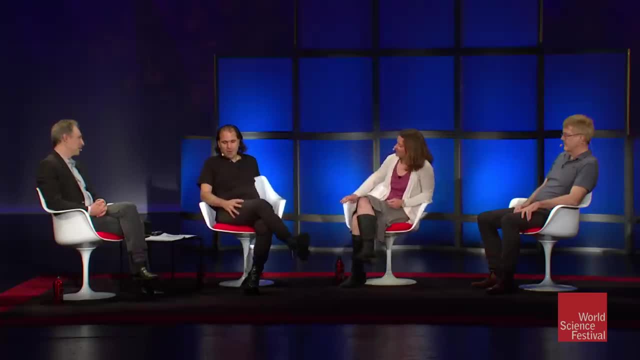 that if I could go back in time and control when I'd be born, I would wish that I was entering grad school today. Really, I really think this is, from my point of view, it's the most exciting time of my life. 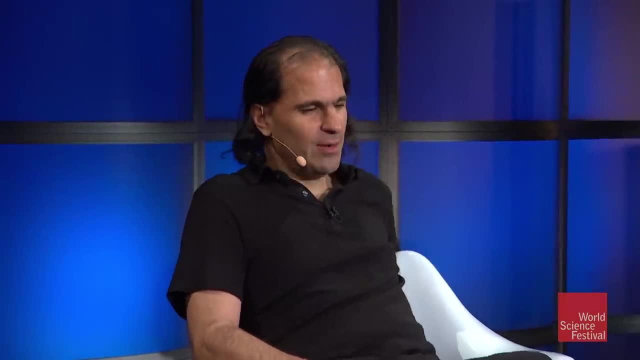 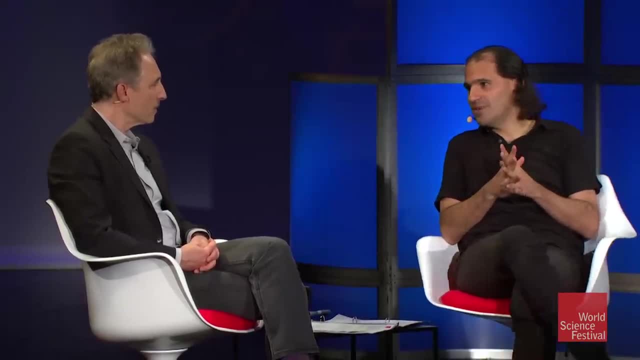 certainly in 50 or 60 years, maybe going back to the time when relativity and quantum mechanics ended up coming into existence, And it might sound crazy, I mean, you know. so again, there are other people who are wandering around. 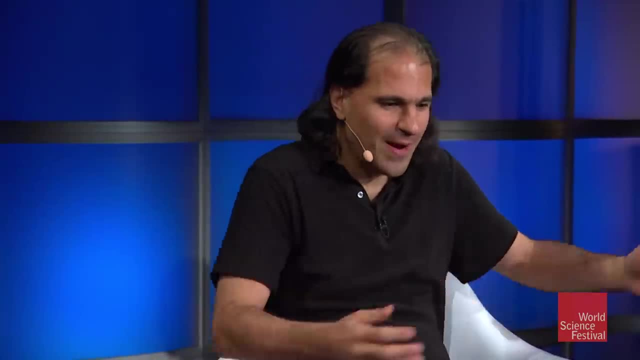 They're sort of depressed. We've seen the Higgs and nothing else. So who's right? You know, am I just on drugs Or are they on drugs? And I think it really depends on why you got into this business, If what really drives you is. 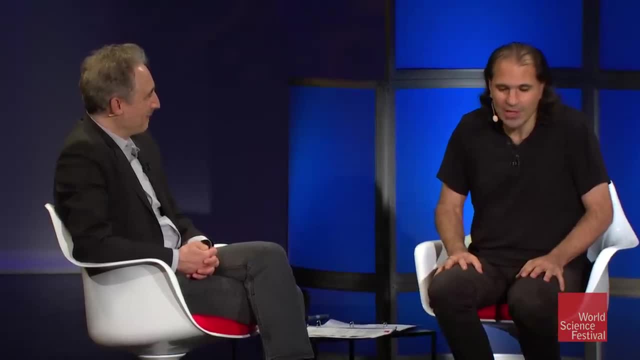 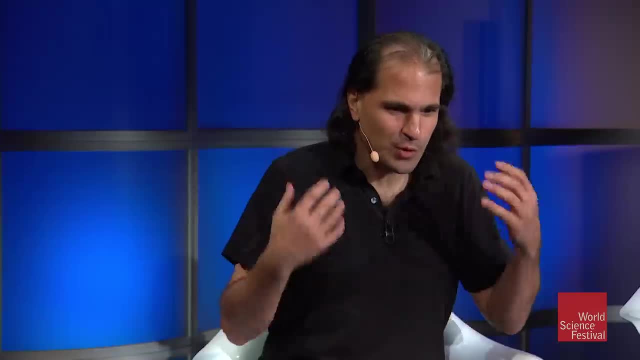 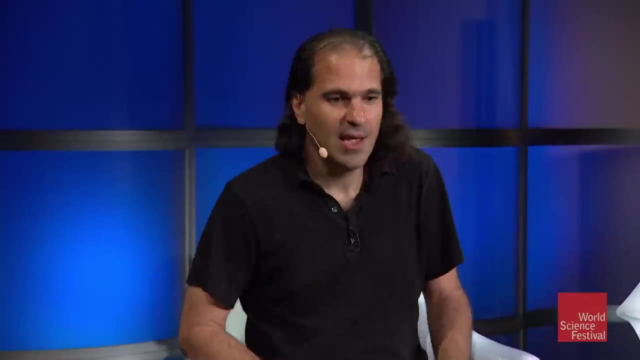 you is trying to understand something deeply, conceptually new about the world. that kind of opportunity does not come along every 10 or 20 years or so. Most people don't get to experience that, And I think we are now at the point after slogging through. 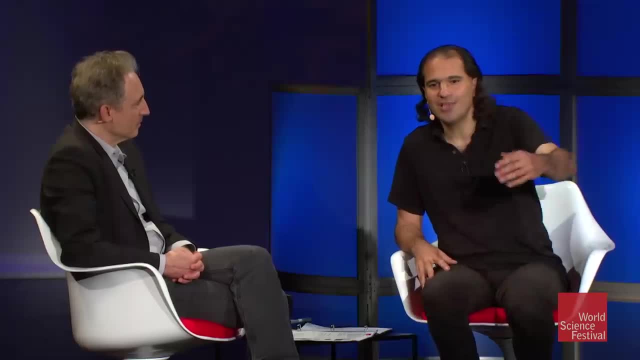 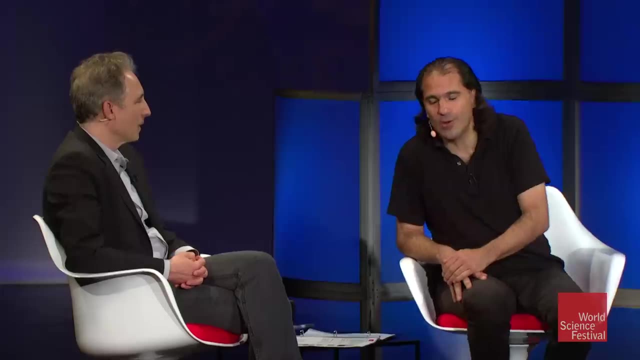 all kinds of easier questions where you know, in science you're motivated by gigantic questions, but you have to work on the next question. You have no choice but to work on the next question. Well, we're finally at the point where the next questions are. 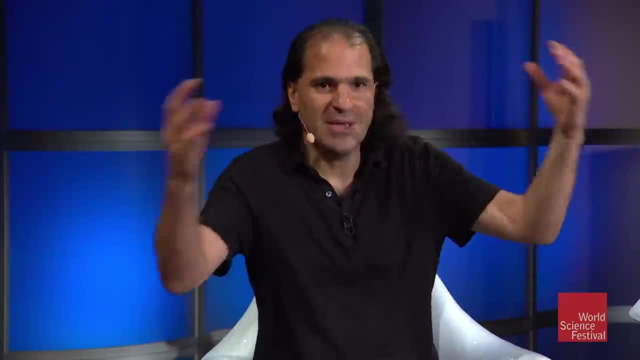 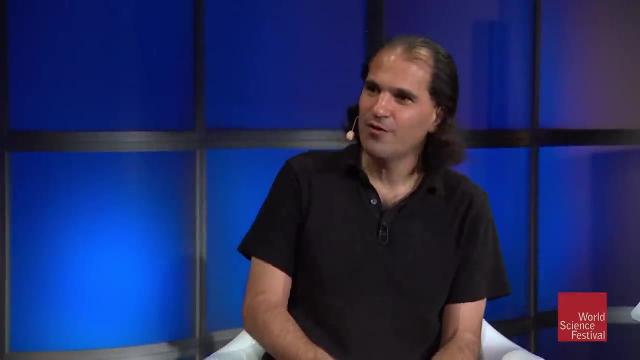 these gigantic ones, or these gigantic questions, These sort of existential ones? What's space and time? What's the origin and the fate of our enormous universe? Why can there be large macroscopic structures when there's enormous quantum mechanical fluctuations that seem to want to destroy them? and 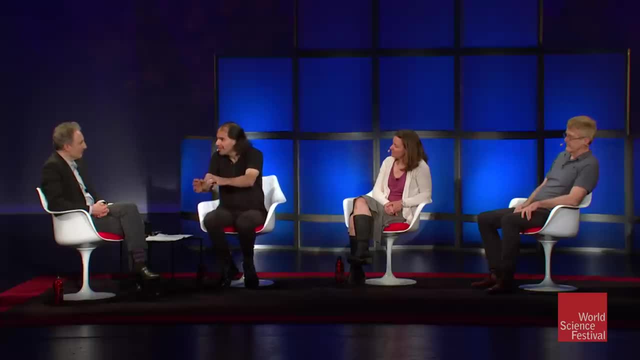 so on. These questions even seem to be interrelated to each other in some way, potentially, And our generation of people are the generation of people who get to work on these questions responsibly. It's meaningful for us to work on them because there isn't. 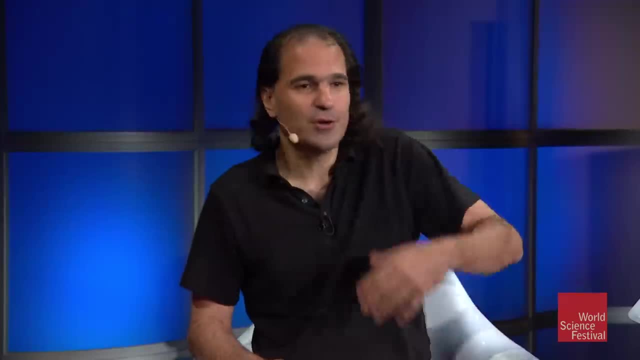 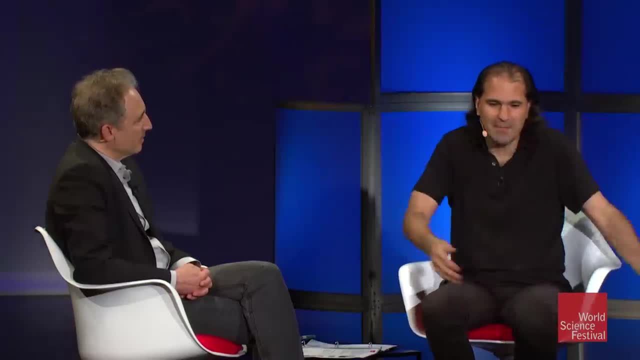 you have to climb Mount Everest first. you have to, you know, get on a plane, go to Kathmandu, find Sherpas, foothills, all kinds of stuff. Finally, you get to base camp, right, And you get to see the beast. 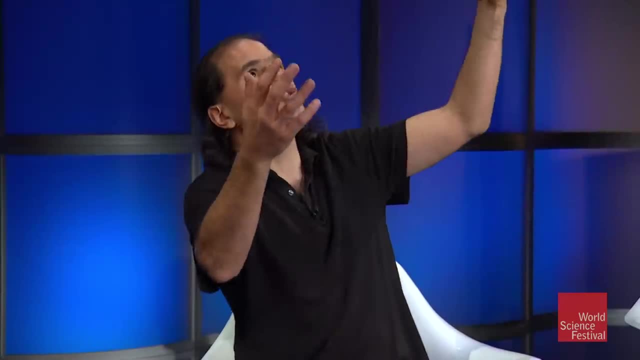 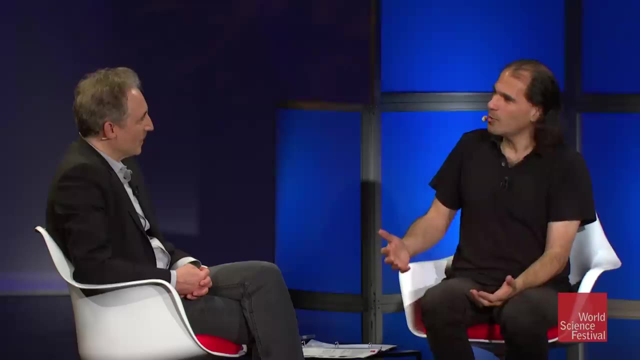 for the first time and then decide what you want to do. You want to wait for oxygen to be oxygen mass to be invented, otherwise you might go up and die, or you start trying to climb in some way. That's where we are, I think. 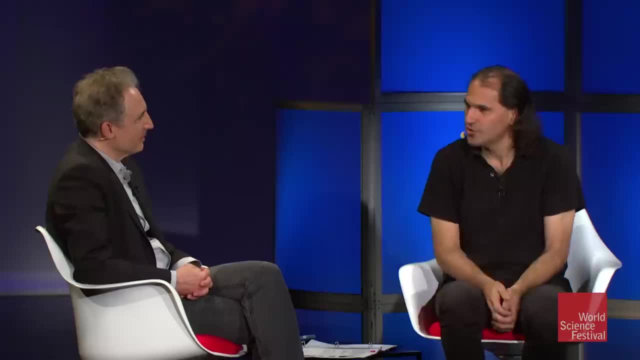 We're at a point where we're finally staring at these most profound questions about the nature of reality, And we get to work on them, And we get to work on them as theorists and we get to, you know, take on the questions that we're interested in. 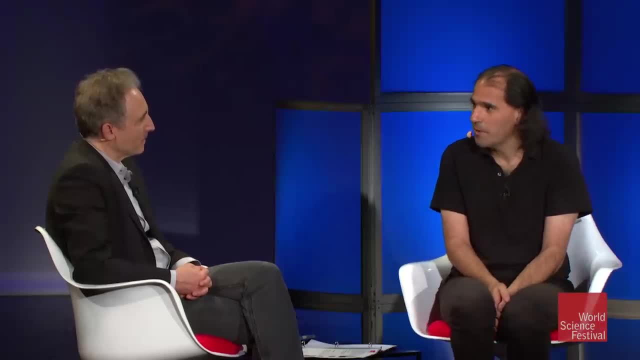 And that's a mighty sort of generation-scale challenge of attacking some of these questions as experimentalists. So I think it's a fantastic time to be a physicist, But you have to have the understanding that you have to be in this business for the long. 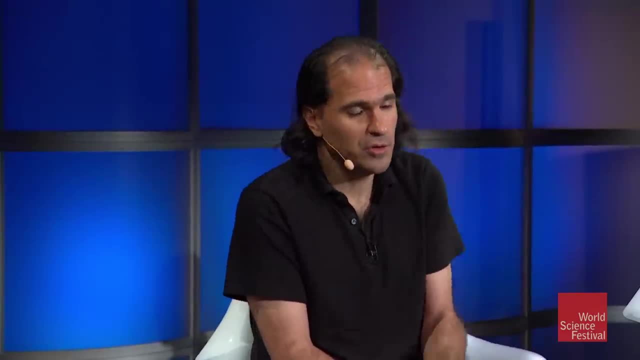 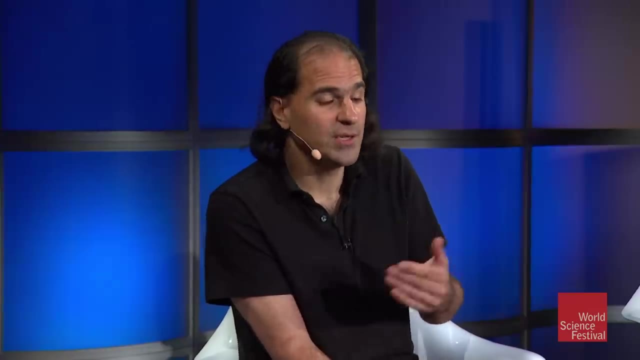 haul, And you may well go 30,, 40 years. You may easily die without having made substantial progress on the questions that you are interested in, But that's what you have to do if you're interested in this kind of thing, Joe. 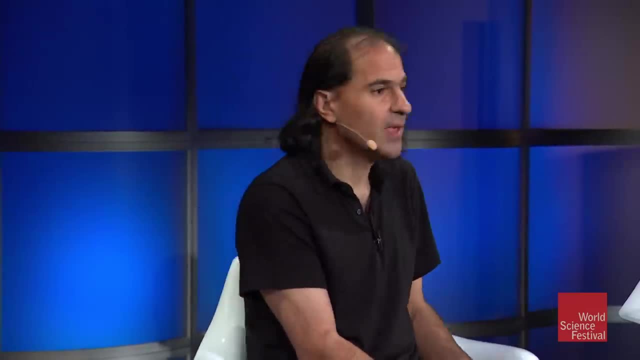 Along the same line, speaking to somebody that's at a big national lab. if you look at what our young people are doing right now, they're doing a lot of research. They're doing a lot of research. They're going out to these. 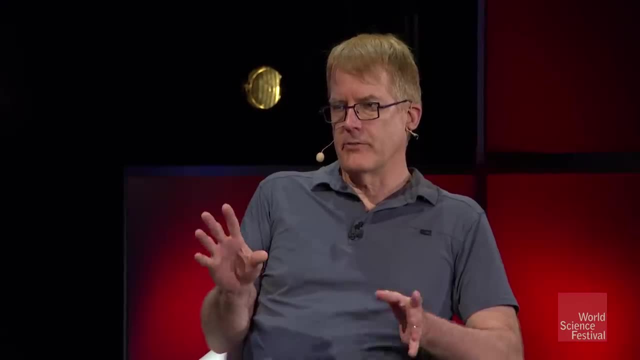 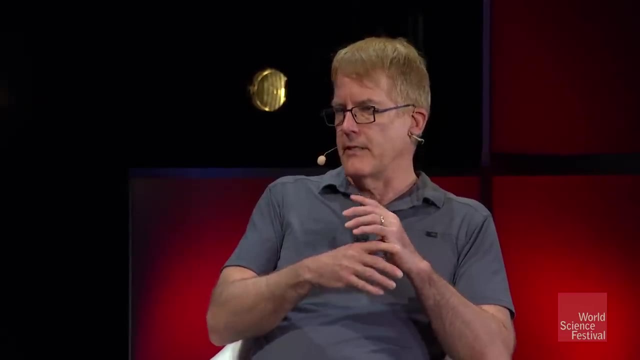 labs. They're motivated by the big scientific challenges. They're trying to develop new technologies to build us these better microscopes that we know we're going to need to make these discoveries, And so those technology challenges are equally fascinating and interesting as these scientific questions that 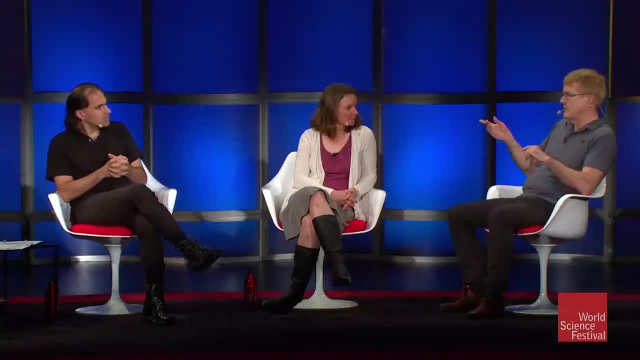 are motivating them And I think that sort of cycle of the big science questions motivating us to push the technology so that we can do the experiments that we haven't been able to do yet. I think that's a very virtuous cycle And it's one of the things that 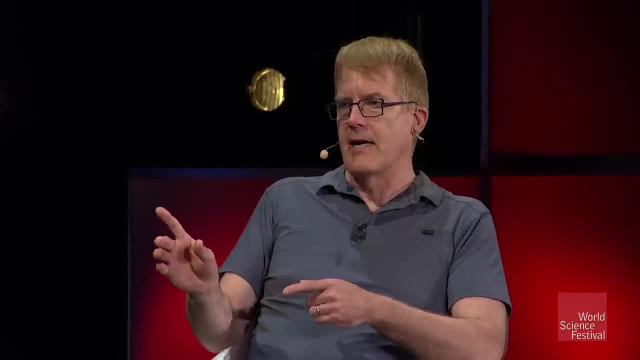 we do for society that's important to us, And I think that's one of the things that we need to do, And I think that's one of the things that we need to do, And I think that's one of the things that we need to do for.